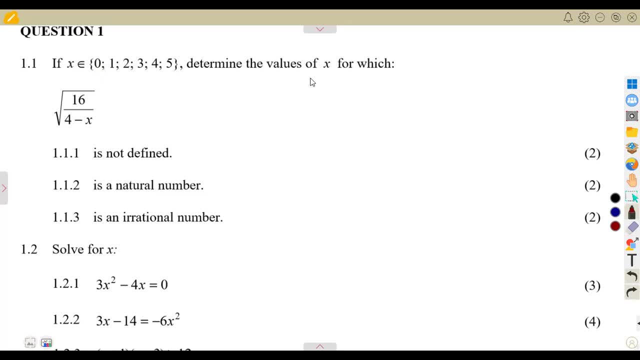 Only these Determine the values of x. from these values that are here Determine the values of x that when you substitute here the value of x, 1.11 is not defined. This one is a natural, this one is an error. So they are simply saying: substitute the value of x, any value of x here. 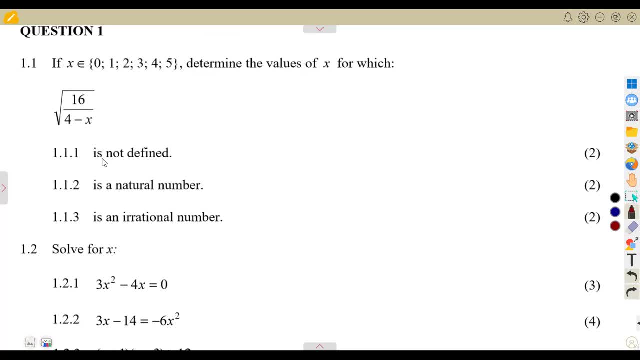 that you are given and see where it is Not defined. Okay, that is, that is guess. So if you are someone who is into like calculations, you can see that. okay, I'm dealing with a fraction there. Yes, it's a square root, I know. 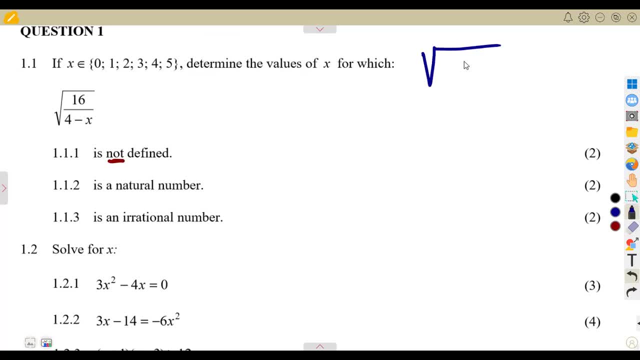 that I'm having a square root there And I know that the square root cannot be of a negative. The square root of a negative value does not, does not exist. This one does not exist. It is not there. We do not have the square root. 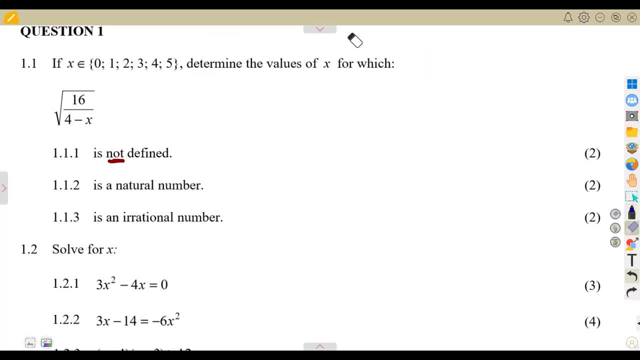 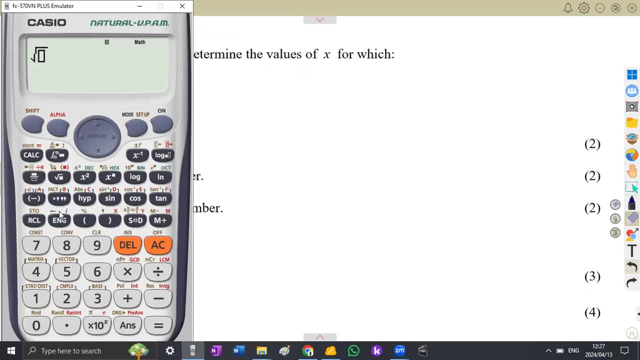 So what it simply means is that: all right, I want you to do this so that you understand me. This is you and your calculator. You are going to say that, all right, let's just try the square root of a negative five That is met error to this, to show that this does not exist mathematically. 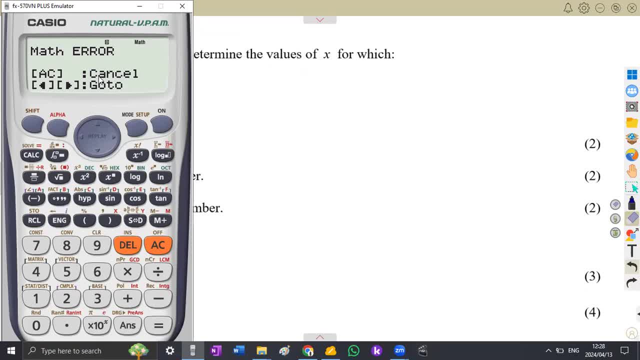 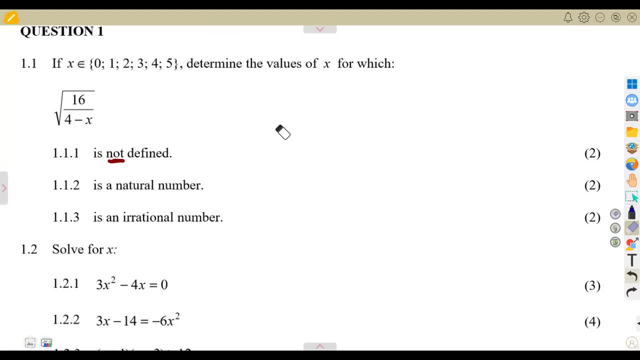 A square root of a negative does not exist. So the question is: where are we going to have this as a negative? That's the question. Where are we going to have this as as a negative value? Where are you going to have it as a negative? Where you have it as a negative, that's the X. 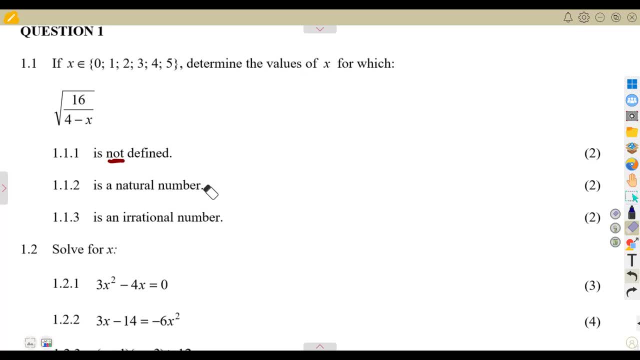 value They are talking about. that is the X value The question is referring about. Okay, So this is just a substitution that you are going to make, So I just, I just want you to see something so that we can properly answer this question quickly. 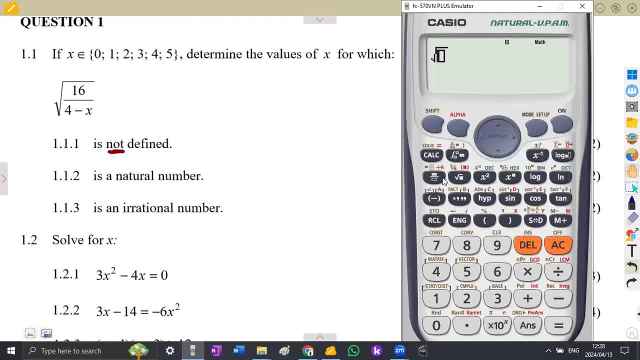 So you just substitute your values. If you do not know, just substitute, because you know that not defined means cannot be simplified. So this is the square root of 16.. So you just put your fraction, already You have your X value. So you just have to substitute for minus the first value. 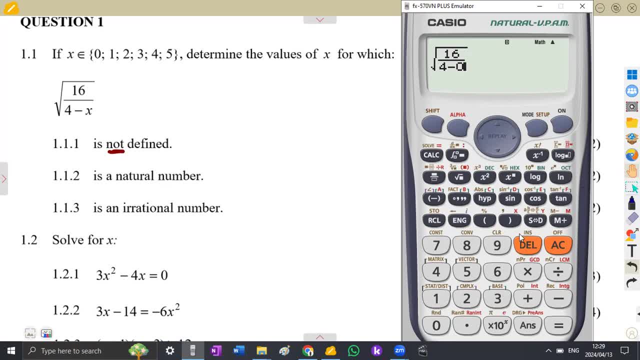 It's a zero there. So if you check, you have got an answer there. You move on to. when X is a one, you substitute a one there. You see that there is an answer there. Guys, not defined means there is no answer. This one is an answer. It's a decimal, whatever that you 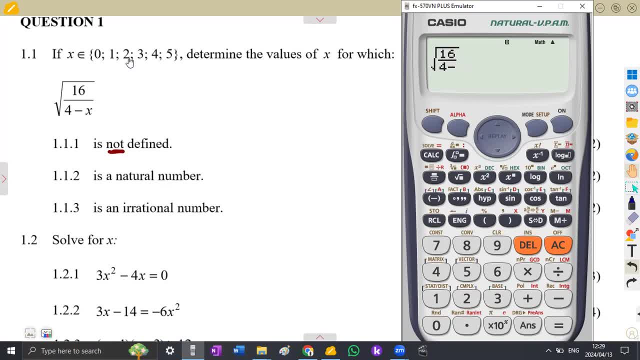 have there. That's an answer, meaning to say it can be defined: When X is two, you move on to two. This is going to give us this two square It, all these values. they can be simplified, All right. 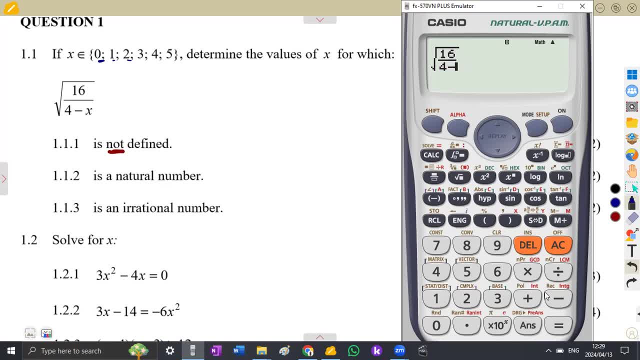 let's move on to three. You put on a three here. That's a three in place of X, That's a four. All right, Meaning it can be simplified. We put a four in this case. All right If we put a four. 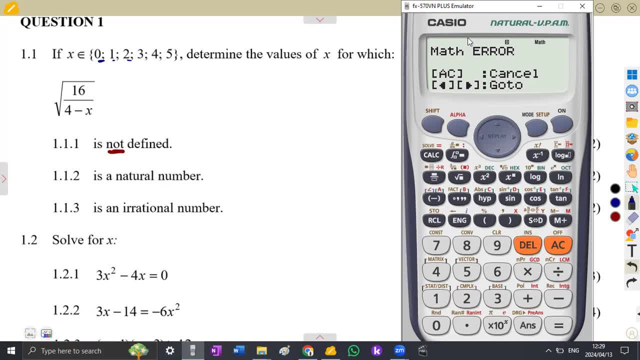 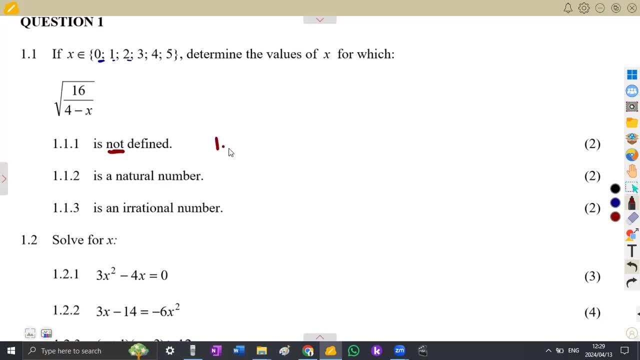 four minus four. meaning to say this cannot. as long it gives you a met error like this, It means it can not be defined. So if you do not know, that is the way that you can use. So meaning to say: in this case, our X must be a four. All right, Let's move on to another X value again and see All. 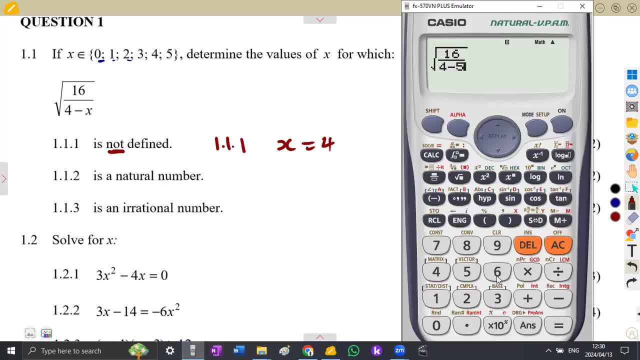 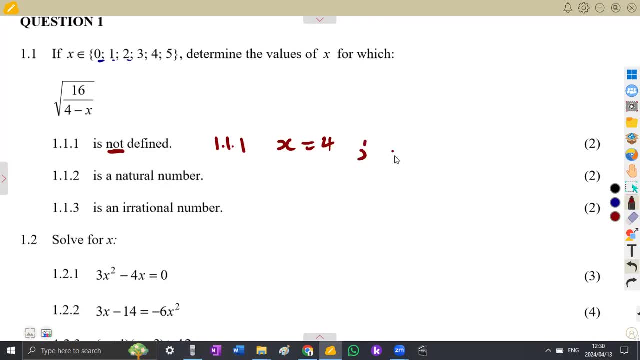 right, If you do the same, when X is a five, you substitute a five. This is going to give us again a met error. I mean, you say this cannot be simplified when X is also equal. All right, Let's move on to five. So these values of X that we have in this set, that we are given 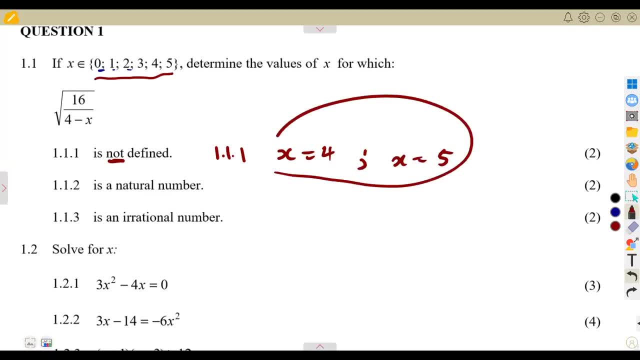 of X. these are the values of X. that will give us something that is not defined. So since we have got X, which is four and five, you can also write it this way: X is going to be an element of the numbers that are going to represent X. It's four and four and five, just like that, All right, So 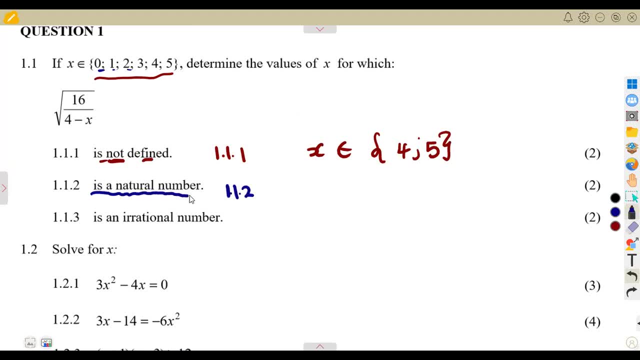 this was your condition, When this is an natural number. So the question is: what is a natural number? A natural number is a counting number excluding zero, meaning to say, zero is not supposed to be there. So what I want you to do is: 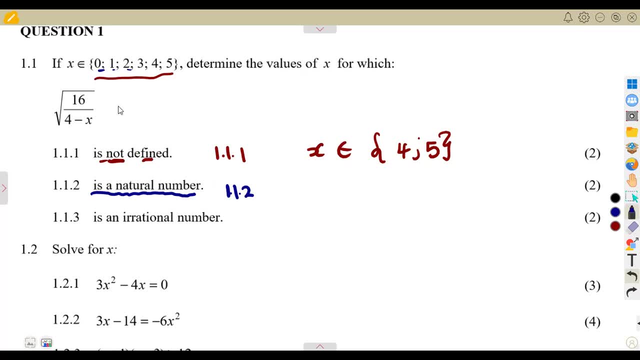 to substitute. you're going to substitute when X is zero, then you're going to substitute, meaning to say that's where you're going to have that four that way. So, okay, guys, we talked about these values, So you are going to see that where we are going to have exactly the count. 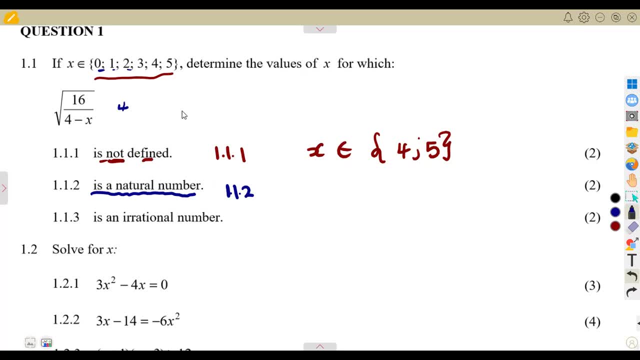 counting numbers, That is, when our X is a zero. we saw that time. when we substitute a zero, then we got a four. So meaning to say X must be a zero, Okay, Also, when you substitute numbers such as one, two, you know, you saw, we got the square root. the square root there. 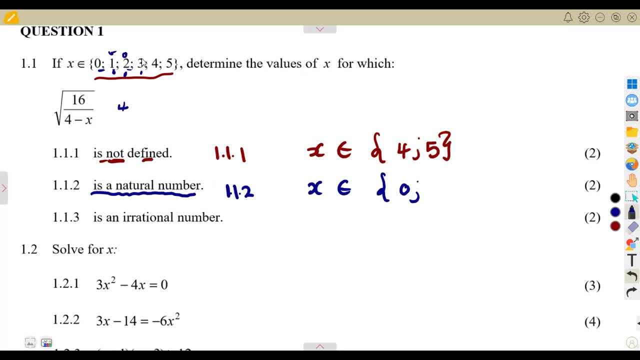 Okay, if we move on to three, we got a four again there, meaning to say a three is going to give us a counting value if you substitute this. So I want you to substitute a three and see what you are going to have at the end is a counting value because we saw previously. 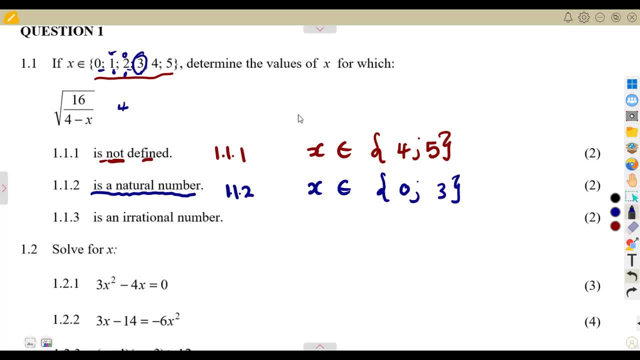 that this gave us a four. A four is a counting value. We saw that at four and five. then this was not defined, So it can't be a natural number, because a natural number is a counting value. So we can't use the four and five. So this is the only part that we have. 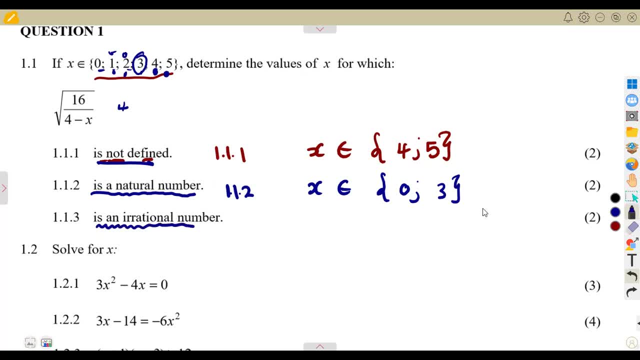 all right, Then, when this is an irrational number, remember, an irrational number is just the opposite of a rational number. A rational number is the one that we are used to. A rational number is the one that you express as a fraction of the. 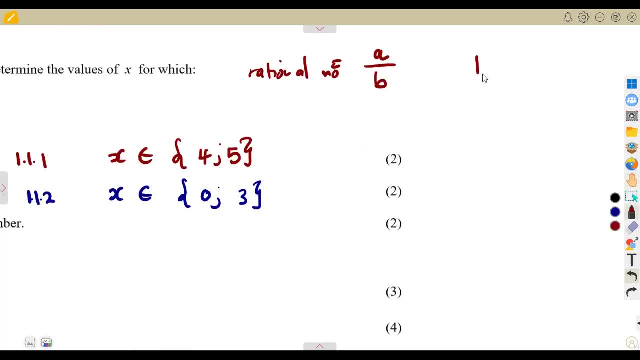 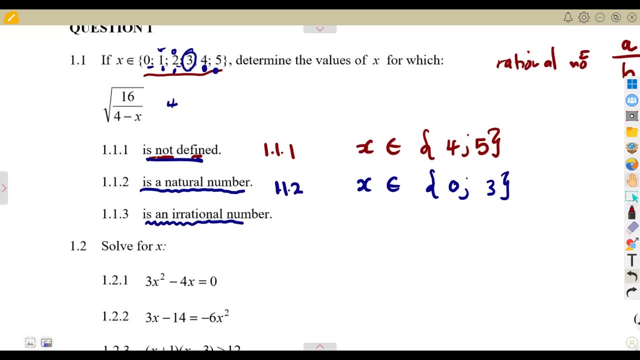 form of A over B, where these are all numbers and B cannot be equal to zero. So meaning to say we just want a condition where we are having that. that is an irrational. But now they're saying this is an irrational, So it's the opposite now of this meaning to say irrational. 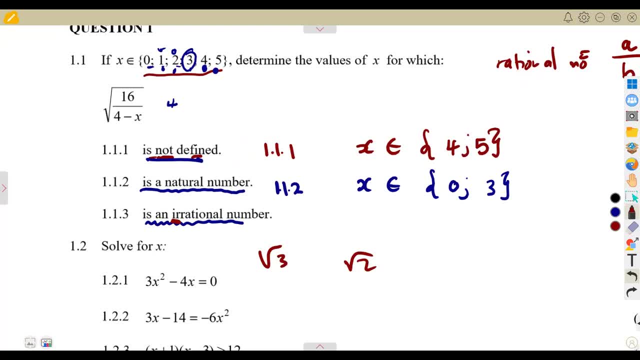 that is when we are having those square roots. Now, the square root of three, the square root of those square roots that we're having, those are irrational, the opposite of a rational number. So we can't use this four because it gave us a natural number. A natural number cannot be. 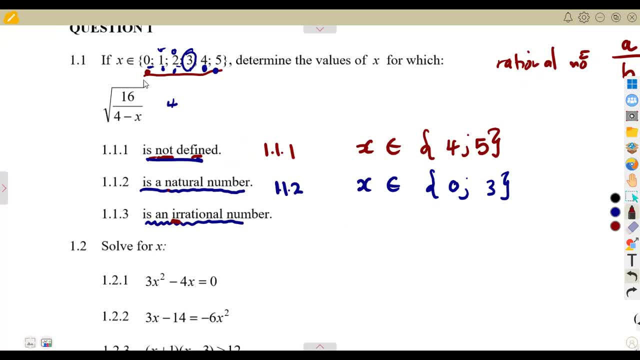 an irrational number, because a natural number is a counting. So where x is a zero, we saw that it was a four. We're not going to take that, So the value was going to be at one. Remember when you substituted one, guys. 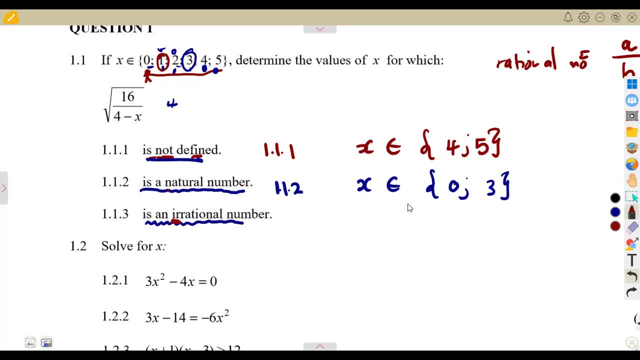 I showed you. we saw something like four square root of three over three. that's an irrational number. So meaning to say at this point, our x must be at what our x must be at one. we also saw this happening When we substituted a two. we got two square root of two. two square root of two is: 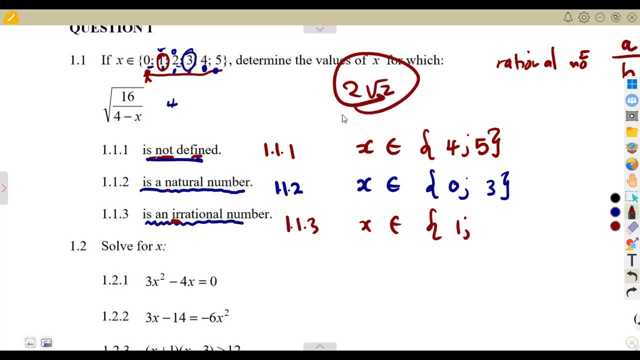 an irrational number, But we got this from which value of x? when our x, when our x was a two, sorry, when this x was a two. All right, if you move on to these three. when x is three, it was a natural number, So it can't be an irrational number. 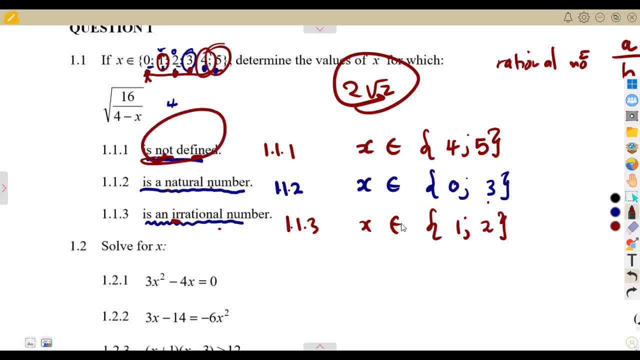 When four and five- these are not defined, So meaning to say these are the only numbers that will give us a irrational number and irrational number, Be careful, you have to substitute. So when it was like this, you had to substitute so that you see these numbers. how are they? 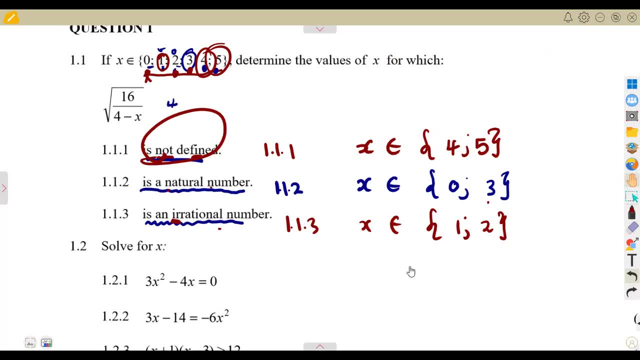 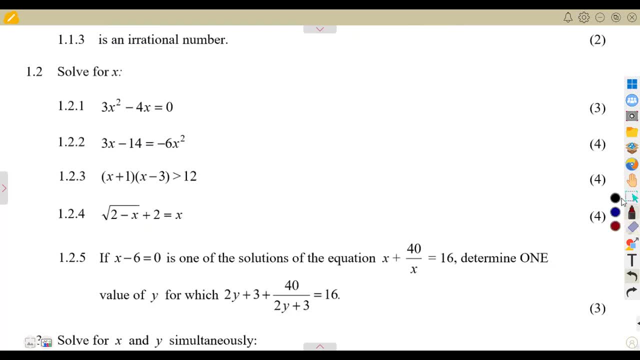 So this is your grade 10.. Remember your grade 10 maths. on those numbers I want you to also revise that part so that you have an idea. So this is just six marks for that. All right, let's move on to the other part of our question. 1.2 solve for x, So three marks for the. 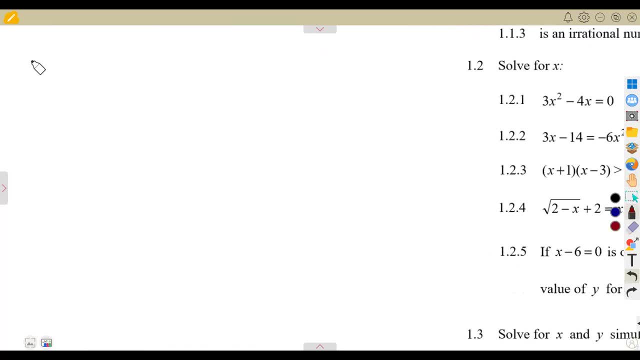 first part: 1.21, we are given to solve for x. that is 1.21,. we are given this is three x squared minus four x, which is equal to zero, and that is three marks for that. All right, that's a. 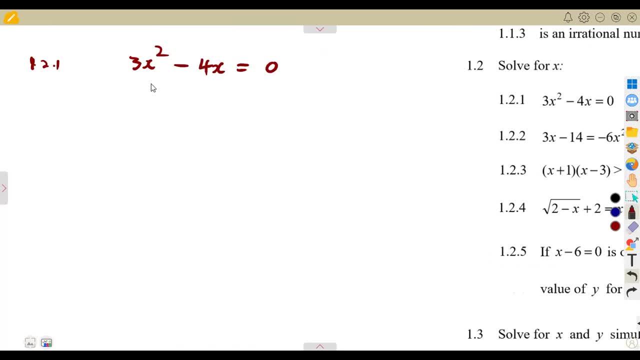 quadratic equation. And the fair part of this quadratic equation is that they are just two to terms. We know from our factorization that if they are two terms, I can just factor out the highest common factor, which is x. By factoring x, I can divide three x squared to x. this will be: 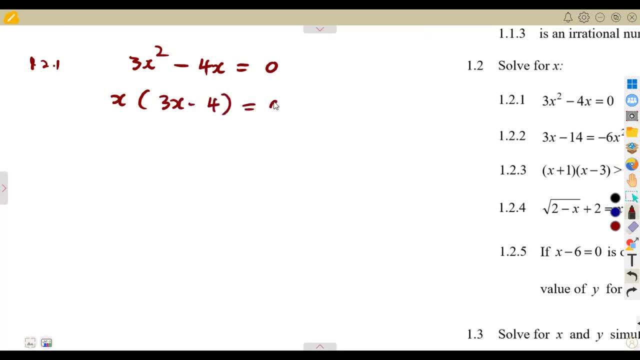 three x minus four, x to x, that will be minus four, that's equal to zero. Remember, from the zero concept, one of these from the product must give us a zero. So it's either x it must be a zero, or the bracket of three x minus four is equal to zero. So from this, if we are to solve for x, 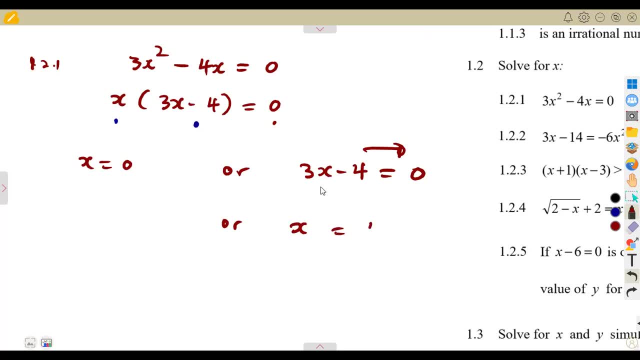 transpose this to the other side, that was going to be a positive four. then you divide by a three, So meaning to say x was going to be a zero or four over three. You can use a quadratic formula if you want. that is your choice, but that is three marks for that. 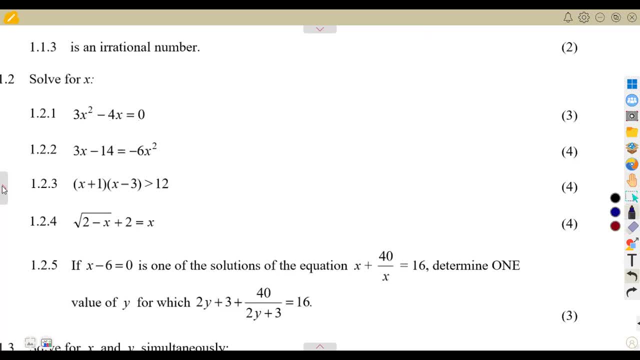 All right. so for x: four marks. So if you see these four marks, in most cases we know that it's going to be a quadratic formula, All right. So we have to apply the quadratic formula. So we have to apply the quadratic formula. So we have to apply the. 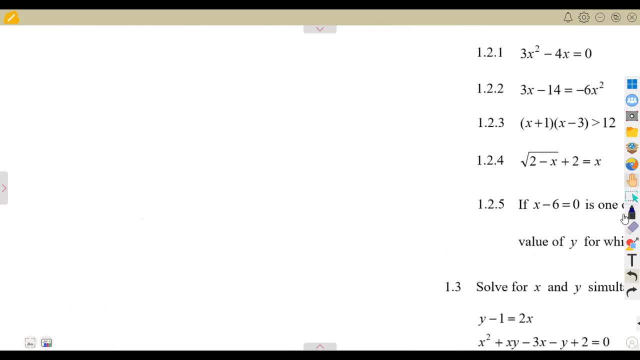 quadratic formula, completing of the square method. it's your choice again. So this is 1.12,, where we are given three x minus 14 is equal to minus six x squared. So the first thing is the format of our quadratic equation, which must be, and the form of a x squared plus v, x plus c is: 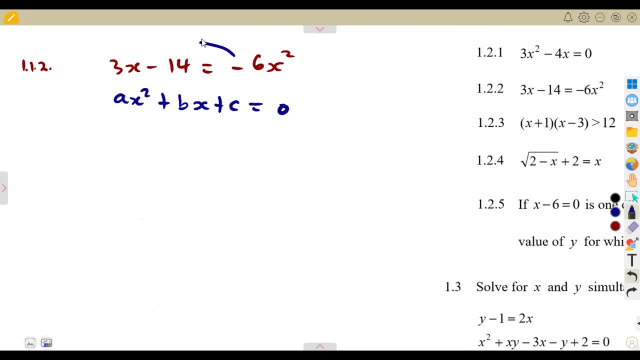 equal to zero. So if you're to check this format, we can transpose this, because what we need is to have one of the sides equal to zero. So transpose the minus six- we have to have one of the sides to the left hand side makes this one to be a positive. that's six x squared, because it is: 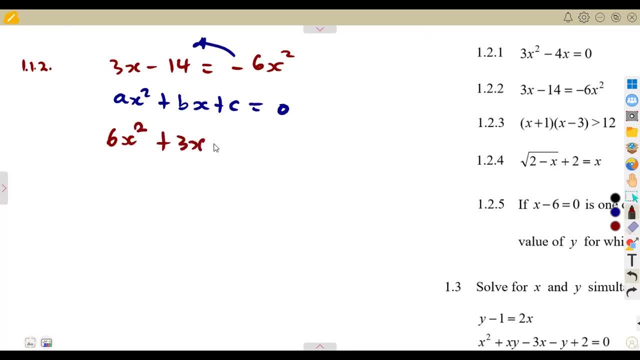 crossed with the equal sign. So the sign changes: plus three, x minus 14, which is equal to zero. So, as we can see, we have our normal quadratic equation that we can solve using our quadratic formula from the format of a- x squared, b, x plus c. it means our a is six or b is positive three. 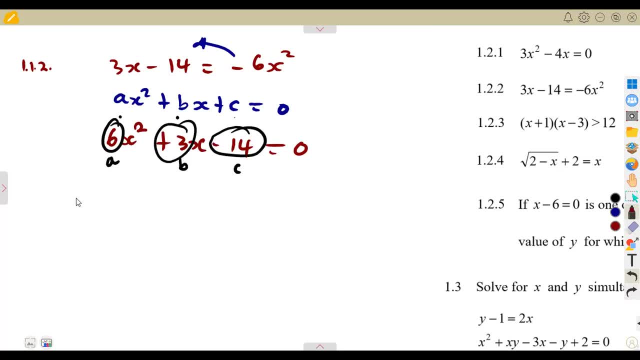 our c is the constant. So using the quadratic formula we know that our x is equal to minus b, plus or minus the square root of e, squared minus four ac, everything over to a, that's going to just substitute b. So that is minus b, which is positive three, plus or minus the square root of b, which is positive three. 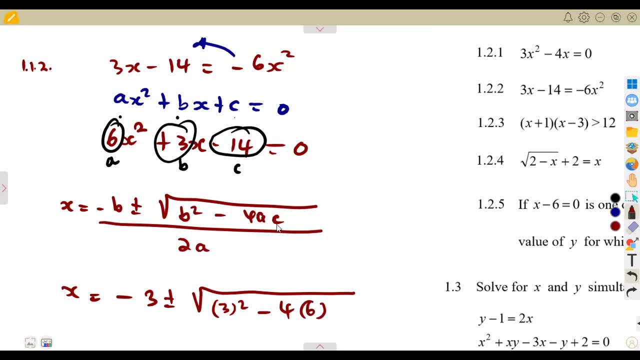 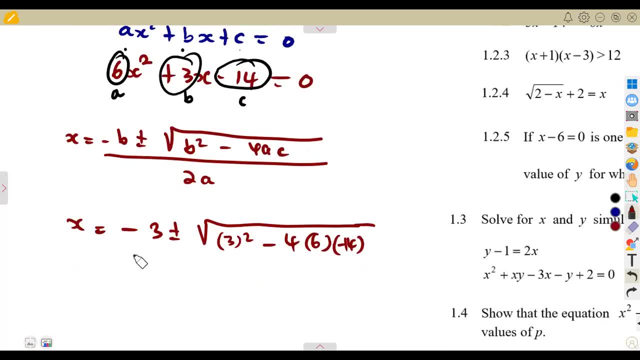 squared minus four times a, which is six, and our c, that is minus 14.. All right, that's a minus 14, then you're going to divide everything over two times a. that is two times a, which is six. So what I would like you to do is to at least 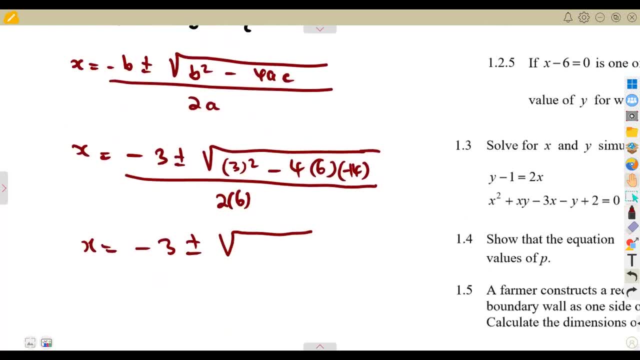 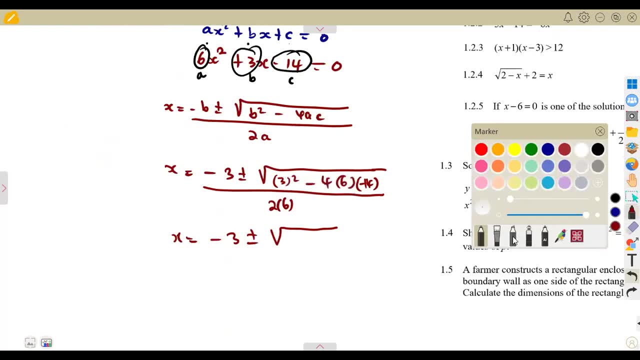 try to simplify this part that is under the square root, just the part under the square root. I know, I know you can simplify this direct, I know that you can do that, I know that you can do it, But just simplify, try to just simplify this part here under the 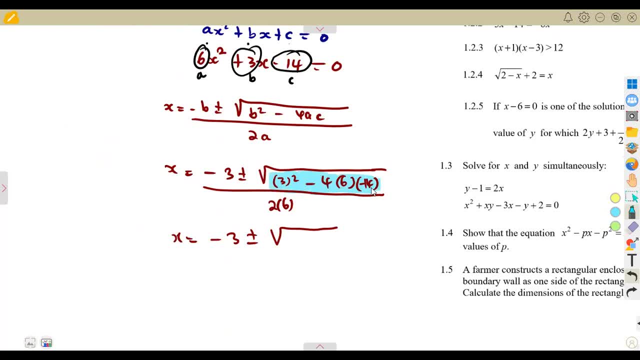 square root. this part alone. Don't put any square root, don't put any, just these numbers under the square. these ones Don't put anything, just those numbers under the square root. just try to simplify that part alone. Okay, this is what I'm trying to say. 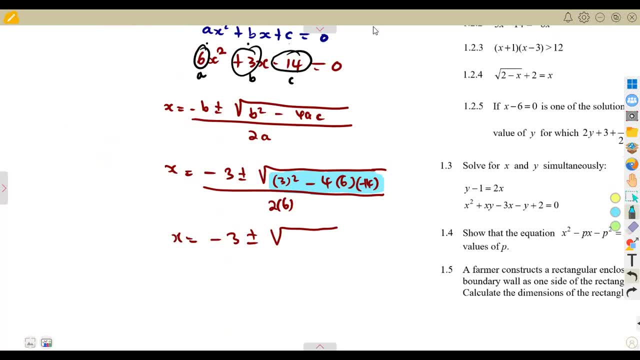 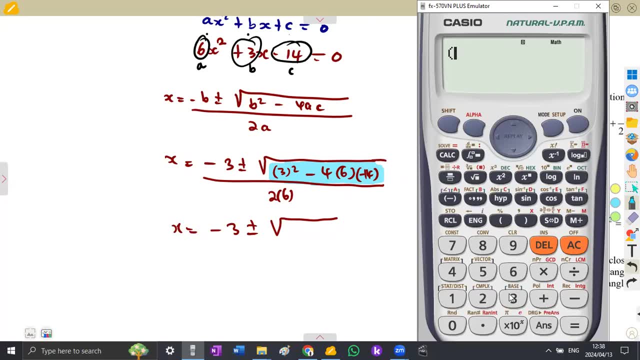 This is your calculator, So you're just going to see what I'm trying to say here. So this is it: the numbers that are under the square root only. So there's a bracket there, three squared, All right. so we're going to have three squared, All right, minus. so the calculator is not as 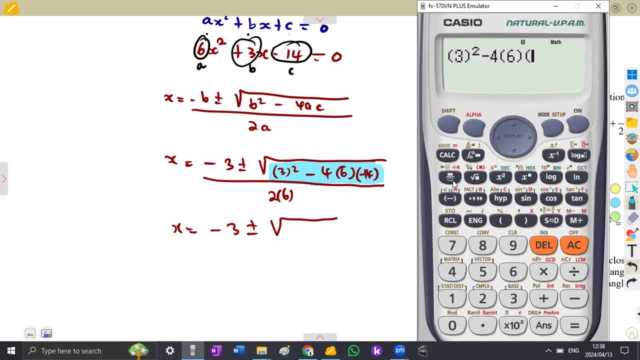 fast as I am, just so this calculator was so fast. So, anyways, this is it, guys, what I'm, what I just want you to do: the numbers under the square root only going to obtain 345.. So meaning to say, from these numbers, we are having 345,. 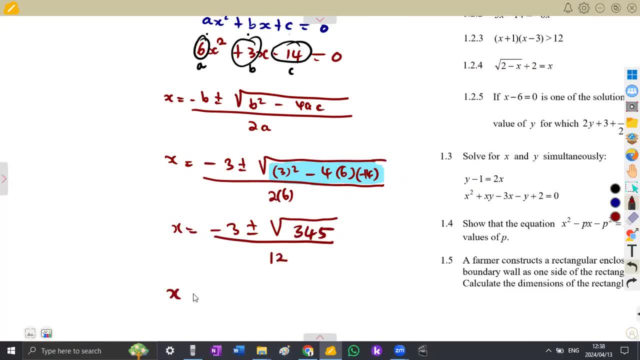 everything over 2 times 6, which is a 12. Then from there you can separate. I don't care how you're going to do that, But at least we see this, this, this number. try to do that, All right. 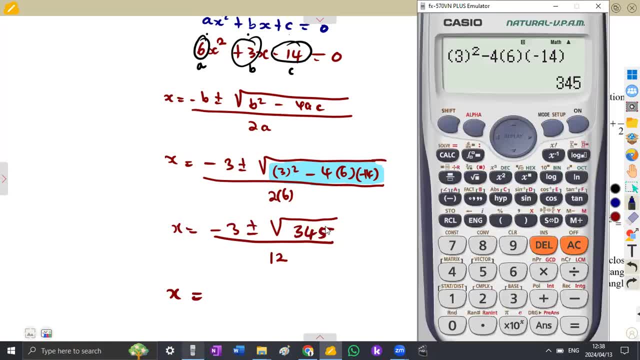 then you're going to separate plus or minus. So this is what you're going to have on your calculator. Even if you don't show that, just write your answers. No problem for that. Minus 3 plus the square root of 345, everything over what? over a 12.. So this was going to give us this. 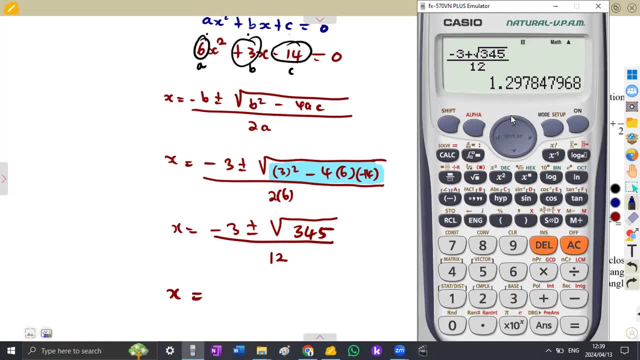 then pressing this SD is going to be 1.29.. So to two decimal places, as we are given on the instruction of the question paper. So you can do that on your calculator shift. you go to the set up, So this is fixed. on number six, they press six. it can round off to two days. 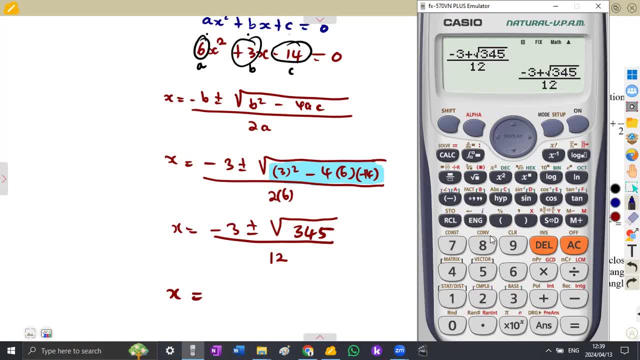 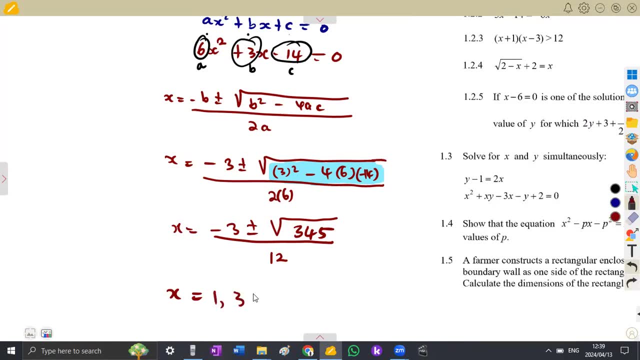 small place from zero to nine. So we want two decimal places. press a two, So change again. So that's two decimal places, 1.30.. So that's 1.30, or x is equal to. again you go back and change. 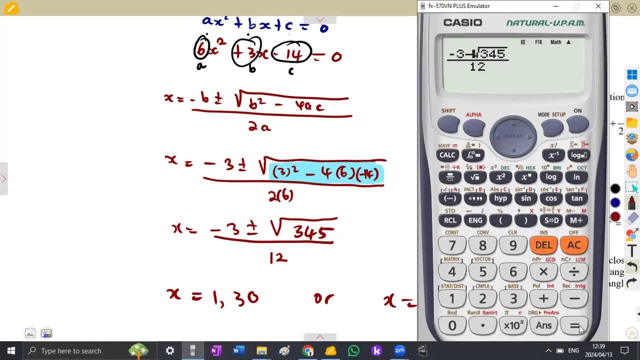 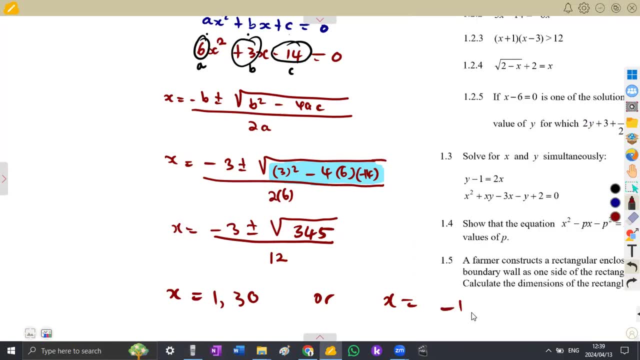 this to a negative. Alright, so already our calculator is fixed to two decimal places. That means whatever that I'm having is to two decimal places, which is negative. 1.81.80 to two decimal places. make sure that you follow. 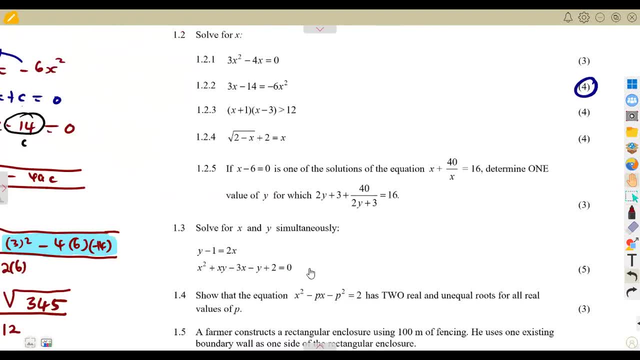 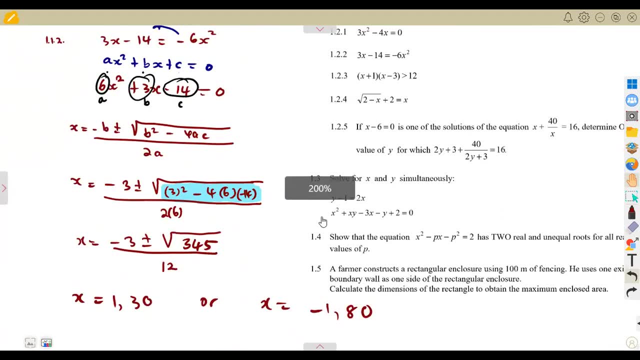 The instruction that you are given. So in this case we are not given the instruction. here we use the instruction that we saw from our information sheet to two decimal places. So these were the possible values of x which satisfy this quadratic equation. All right, 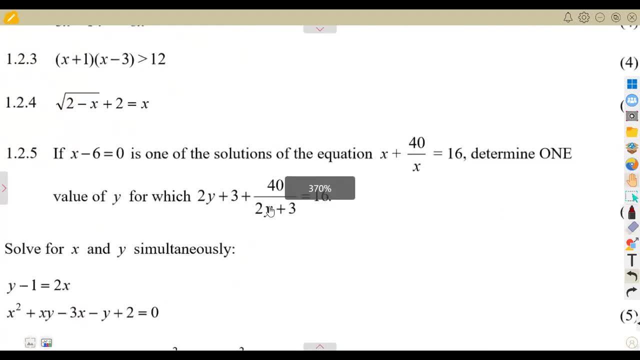 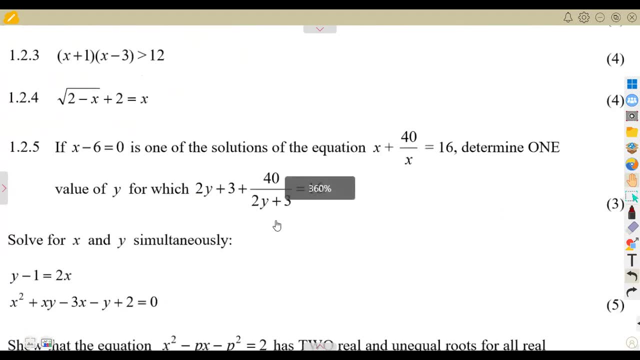 let us move on to another part, which is 1.23.. So again for x, and that's an inequality which is four marks for that. Alright, so they were given an inequality for max. let us see how we're supposed to have this. 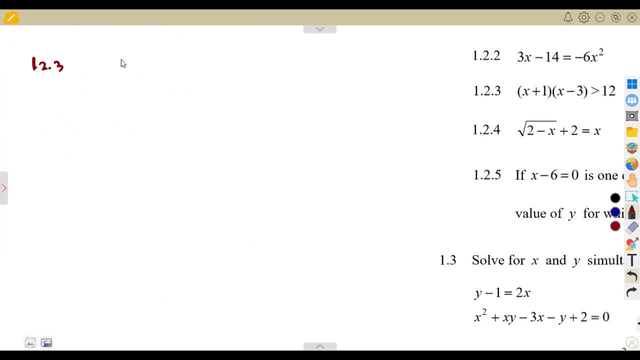 Inequality. Thus, we're given 1.23, the bracket of x plus one into the bracket of x minus three is greater than 12.. So that is the idea there. So if you're to simplify, if you're to solve, 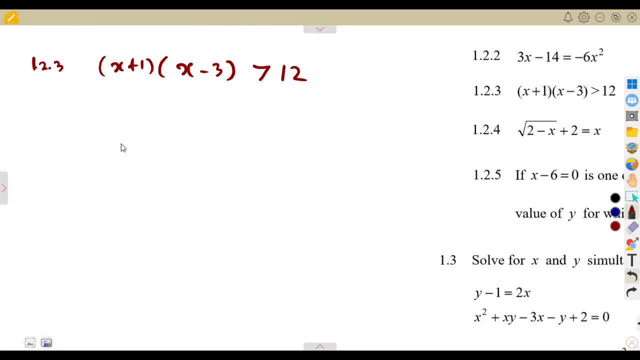 this inequality. we know that we're going to need the critical values, But before that, the same thing that we talk about this is if we check the two brackets there. So by expanding these two brackets we can see we're going to have a quadratic. So at the end of the 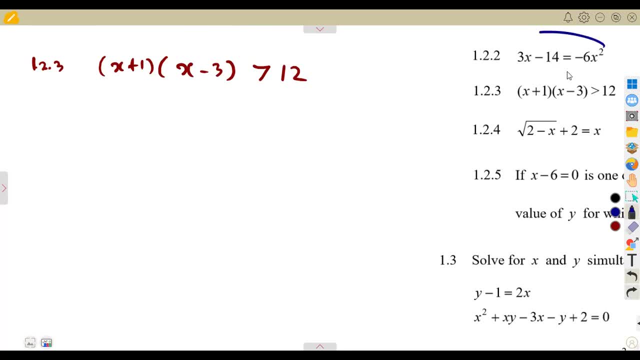 day we're gonna have the same format, just like what we had on this part. It was a quadratic, Yes, but we had to also focus on the format, So the format also plays a role. The format also plays a role. So you're going to expand brackets, then this: you have to transpose it to the left. 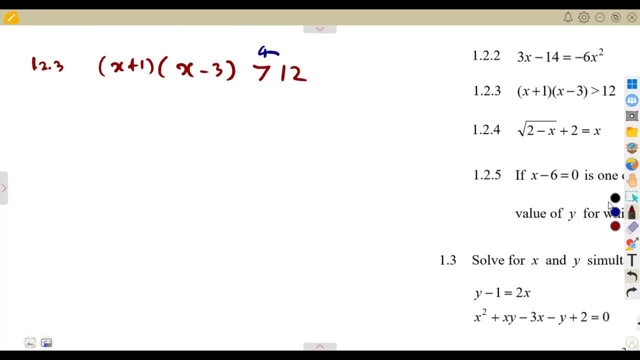 hand side, so that we remain with a zero on this side. Alright, so expanding our brackets using our FOIL method, x is going to multiply With x. that is going to be x squared x times minus three. that's minus three x. make sure that. 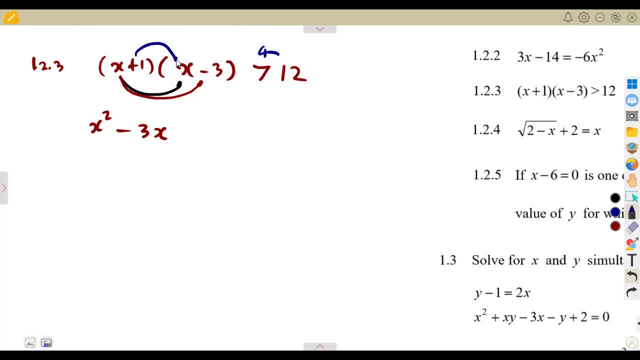 x multiplies everything in the second bracket, then one multiplies also everything in the second bracket. that's one times x, which is positive. x minus three, right, one times minus three, that's a negative three. So if we were to transpose the 12 to this side, because it's a positive, 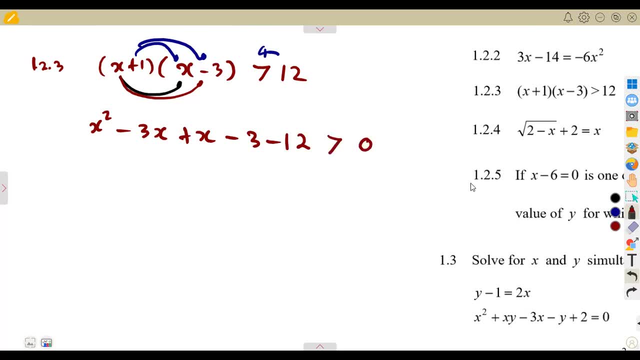 it was going to be a minus 12. That is greater than a zero. transposing this does not affect anything. It doesn't affect and it does not affect anything. So meaning to say what we just need is to have a zero on one side of the inequality, just like what we had on a quadratic equation. So this is x. 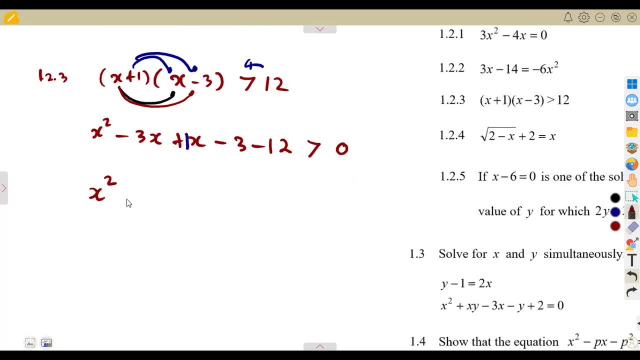 squared, collecting our like terms: minus three plus one, that is going to be minus two, x minus three. minus 12, that is going to be minus 15, is greater than zero. So at this part you can talk of the critical values, which is fine, Or you can even go on to the next part, which is the critical. 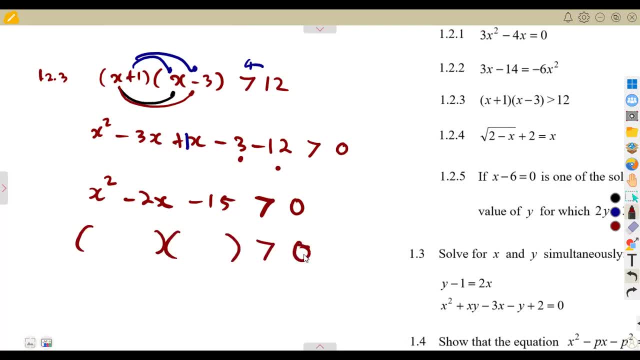 values, which is equal to the factorization before the critical values. it's up to you. Alright, since this is a quadratic, having the coefficient of x squared is one. it means we are going to have x in this bracket, x in another bracket. then you consider the factors or the products of minus 15,. 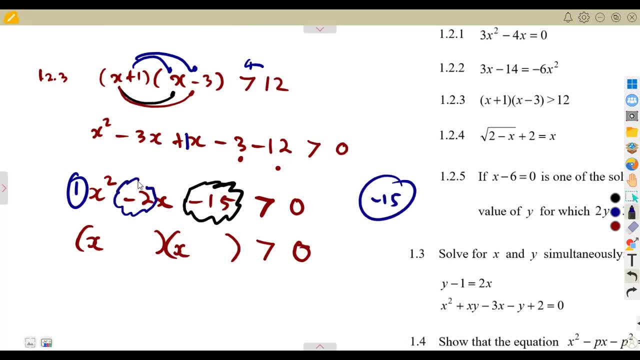 the products of minus 15, that will add up to negative two. There are so many numbers that you can put into consideration minus five and three, five and minus three. so where are we going to have a negative two? if we add, if you multiply, you get a positive. 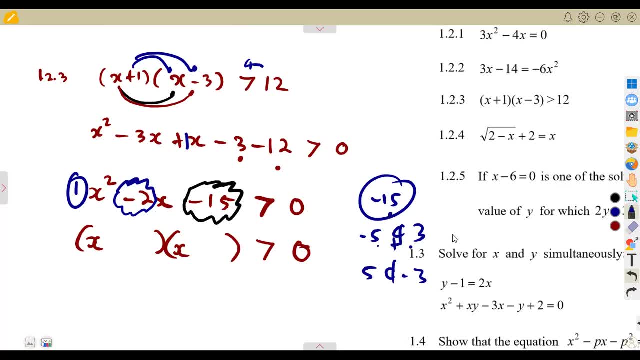 which a negative 15 is fine. If you add, you obtain a negative two. If you add here, you're going to obtain a positive two. So the part that gives us a negative two is on the minus five and the positive three. So meaning to say, on this bracket we are going to have minus five. 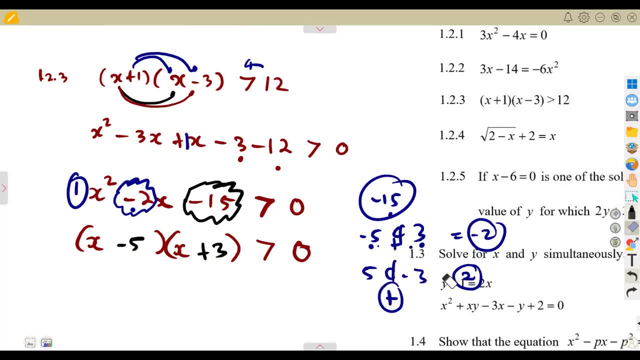 All right, this one, we are going to have a positive three. So that is where now you can think the critical values of this condition. The critical values: what is it that we're talking about? These are the solutions of an equation, not an inequality. no, 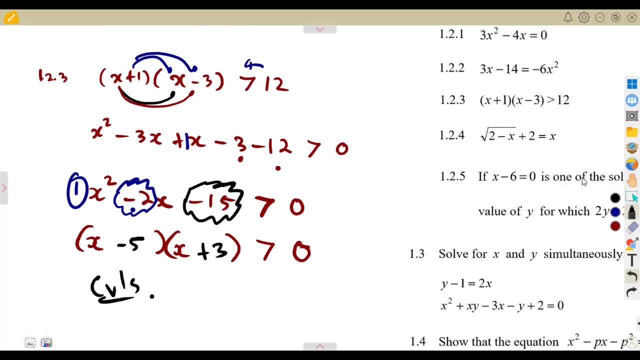 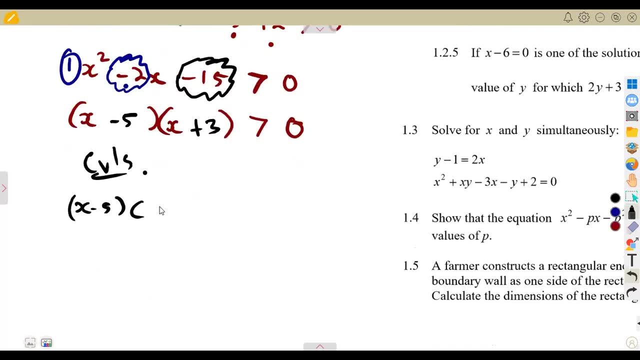 No, not an inequality, an equation just like. just like you are having a normal, a normal equation. you take it as a normal equation. x minus five into the bracket of x plus three must be equal to it's now. 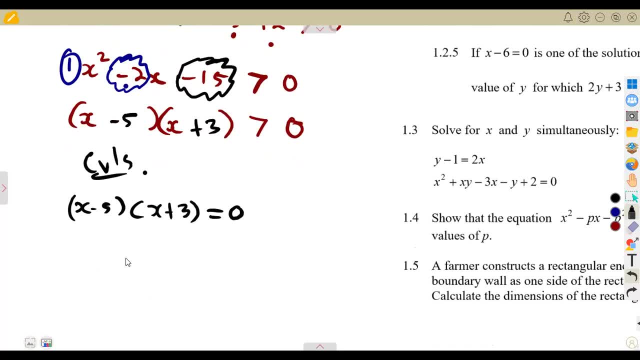 an equation. These are the points, the solutions that we have when our function is equal to zero. add the critical values. These are the solutions. direct, it's an equation, this one. So remember that from the zero concept, one bracket must be equal to zero, So it means x. 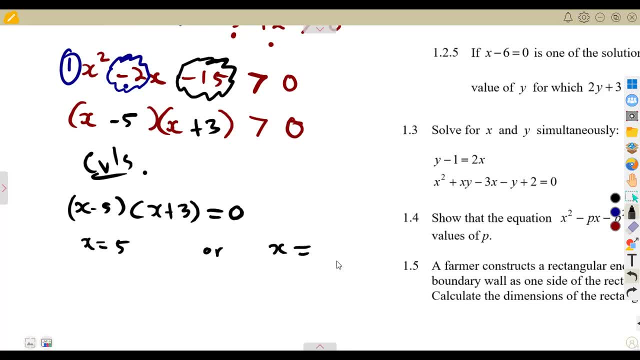 was going to be a positive five on the other hand, or x was going to be a minus three at the other hand. These are critical values. Then, from the critical values, you now need the absolute solutions, which are the exact solutions of the inequality, not the equation. 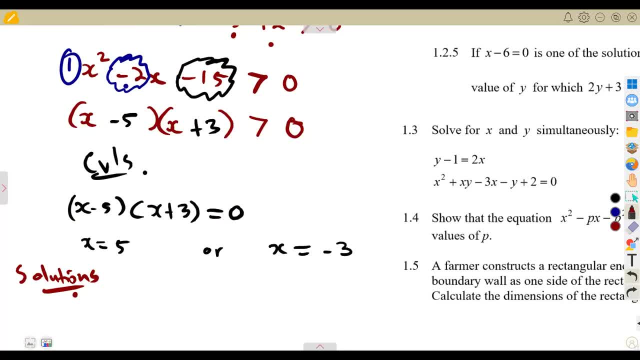 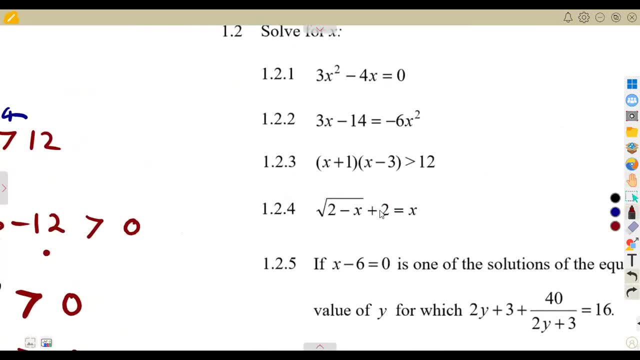 The critical values of an equation. an equation is an equation. that's here. this is an equation: where there's x is there's a zero. there, x is equal. there's an equal to whether there's a zero. whether there is any, there's an equal equal to The moment there's a inequality side. 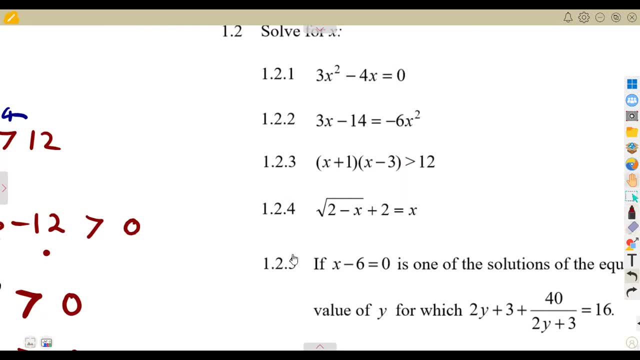 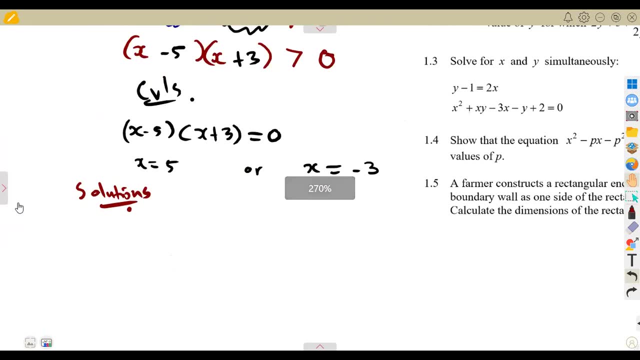 there it's no longer an equation. So we took something that is not part of our question, These brackets here. they're not part of our question. I mean, this is: this bracket is equal to zero. To equate to zero, to say is equal to this, is not part, because 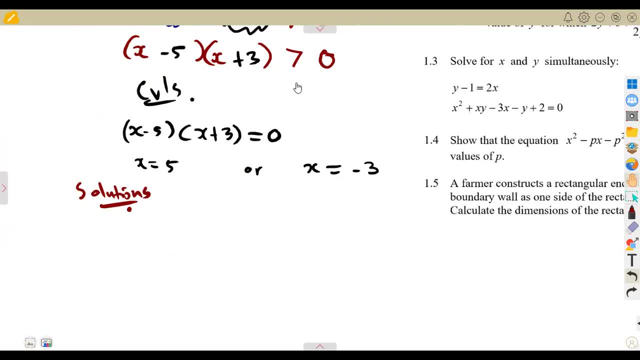 it must be greater than, not equal to, zero. So that is why we call these critical values. So, from there, you need the solutions. You need the solutions. So how are you going to determine the solutions That that? that that is the question now. 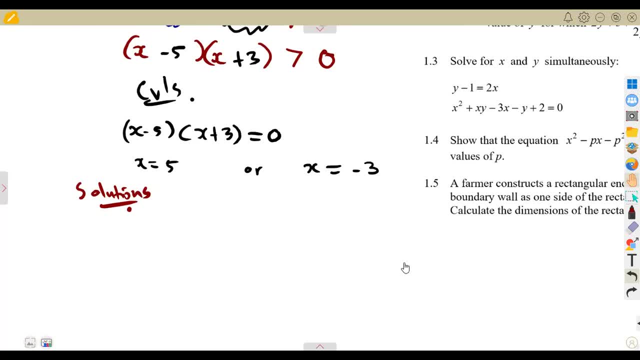 That is the question. That is, how are we going to have these solutions of the inequality? Whether you're going to use your number line, you're going to use the graphical method. it's up to you. So, using the graphical method, this is what you do. You go back at this stage. 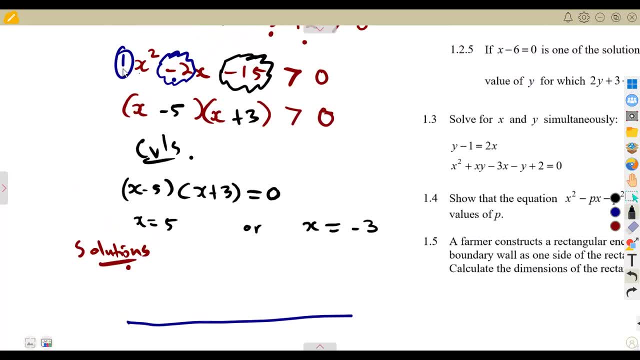 as we can see, the coefficient of x squared is one which is a positive, And we know that if it is a positive, it's a negative. So we're going to use the graphical method. So we're going to use, if a is a positive, we're going to have a smiley shape like that. So that will be a smiley shape. 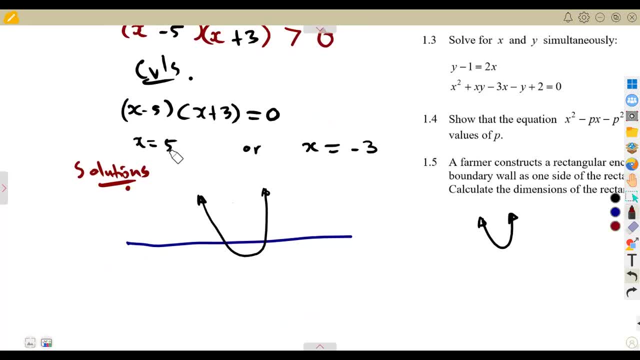 at a point where this function crosses x must be five or a minus three. So negative three will be on the left side and a positive five on the right side. So representing or talking about the x values, These are the ones that we need on our solution. Where is this function greater than zero? where our function is greater than zero and where our function is greater than zero. So we're going to represent that. So representing that is what we're going to do, And we're going to do the push pesabytes, We're going to do the push pes prompted. So we're going to do the push pesbery ones that we're going to do. 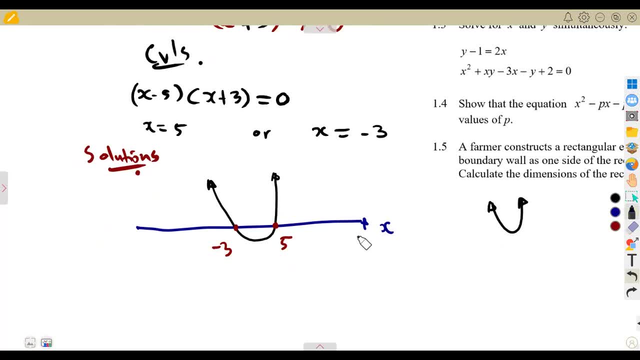 questions here in a really easy way. We're going to take on sum And what we're going to do is we're going to take on some is greater than zero. it is when this function is above the x-axis, above the x-axis, that is when 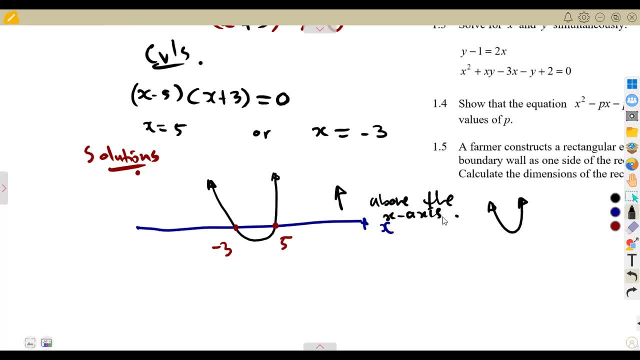 it is greater than zero, When it is less than zero. that is when it is when it is less than zero, that is when it is below the x-axis. When it is like that, you have to consider that it's below what Below the x-axis, So it can be a condition like that. It can be a condition like that When 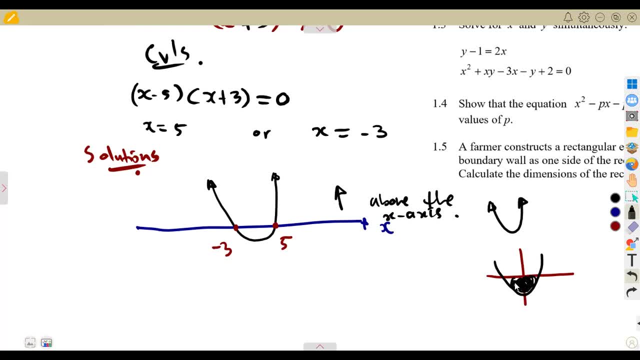 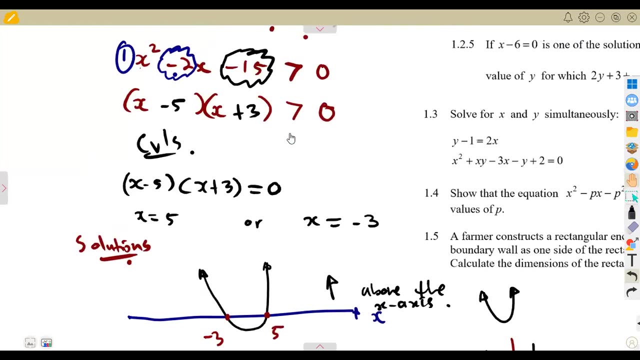 it is less than zero. you consider something below the x-axis, below the x-axis. that is what you need. So, each part, you have to be very, very careful. Where is it that you're taking your solution? So in this case, we are talking about something that is above the x-axis. that is a 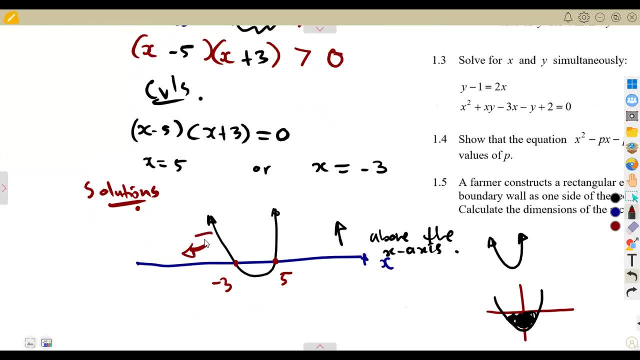 positive. So, above the x-axis, our solutions can be this side of our function or this side of the function. We cannot take something that is open like that, Just like there, there's nothing. What are you considering? What is it here? There's nothing there. So our values on this side, always you. 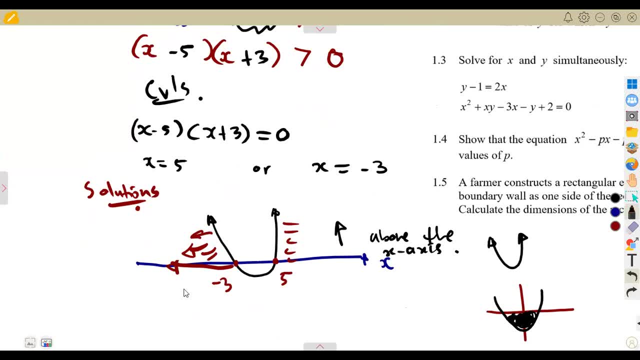 take a less than These values. they are less than minus four, minus whatever that you have, minus 1,000. They are less than this value that you're given. That is less than what Minus three, Or our x values on this side. they will be greater than. 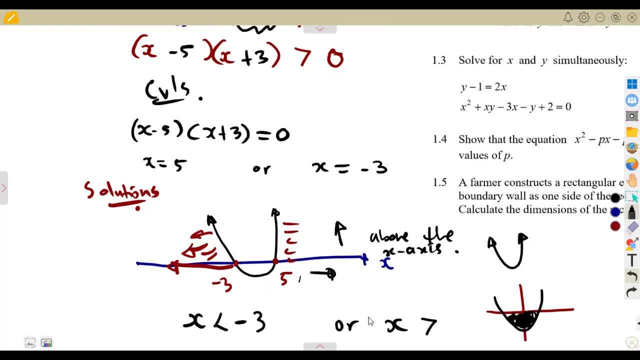 the value that you see here. Always it will be greater than that value that you're going to see there. I just hope I talked about this on the inequalities. If so, if not, we're going to talk about this introduction so that we do not waste much time when doing press and papers, But I just 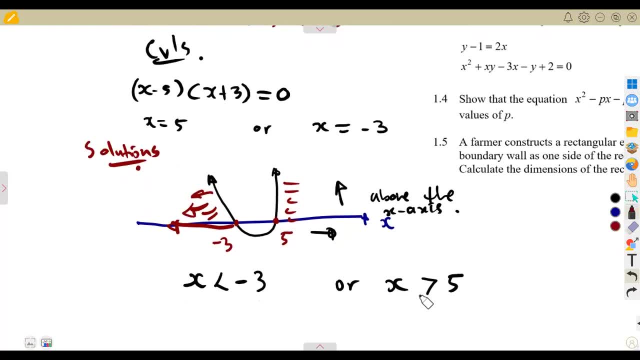 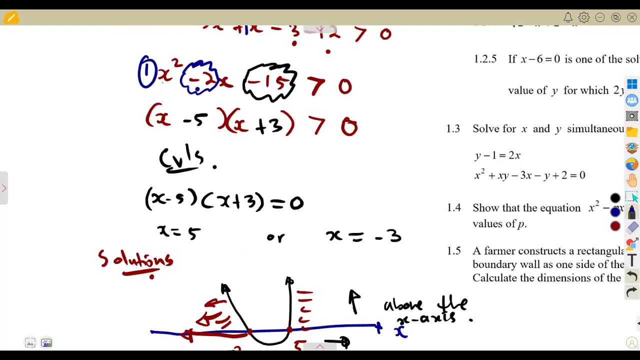 hope you understand the concept. So, in short, this is what I want you to do. We're going to talk about this. Whenever you have got these solutions, all this side, they must be greater than. And also, you consider here: if there is an equal to here, let's say there was an equal to there. You also 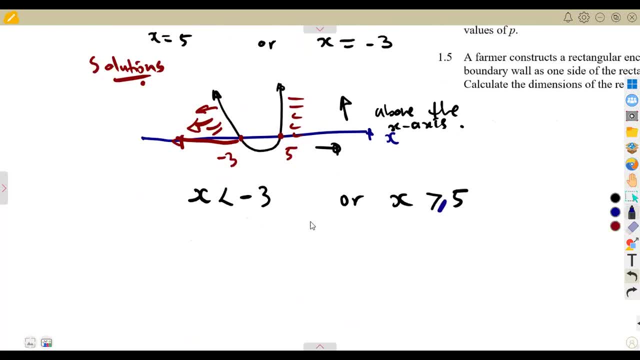 do the same thing on your answer. You also put what An equal to there. But in this question there is no equal to. You, just put greater than, just like that. If the solutions are within here, let's say it was a less than and these solutions are here. 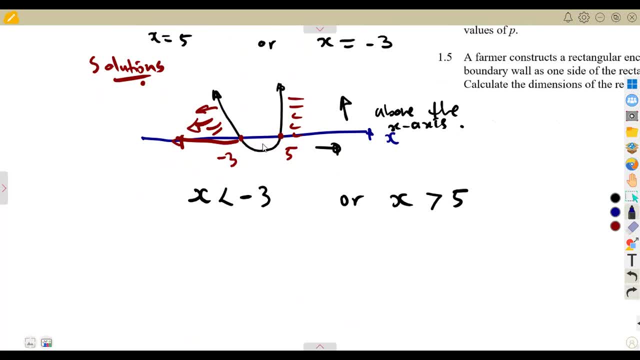 These are the ones that you want. How do you present this region, This region? always, it will be: x is greater than or x is less than these numbers on the boundaries at the critical values. So it will be greater than the lower value, which is minus three, less than the bigger value. 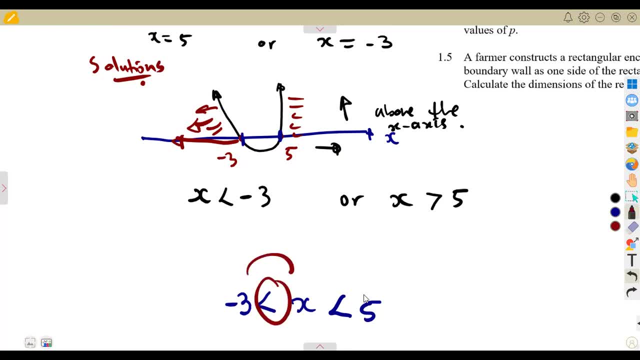 which is five, Always. never give these signs interchanging or you see these signs facing each other like this. It won't be like that. It will always be like that x is bigger than that smaller value, but x must be less than what Your bigger value. 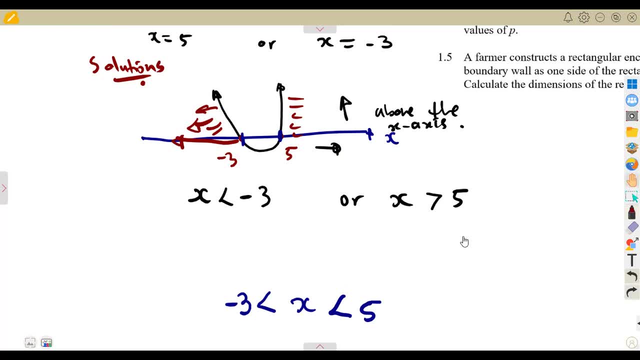 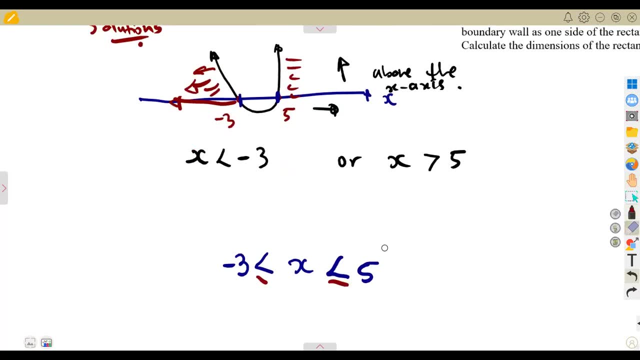 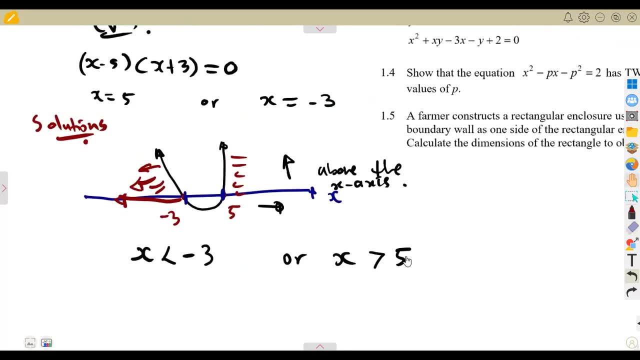 That is the condition Always. So if also there was an equal to here, you also put an equal to on your what, On your answer. But in this case it wasn't like that. So I'm just saying this because of time. But on our introductions, we hope that we're going to talk about this. 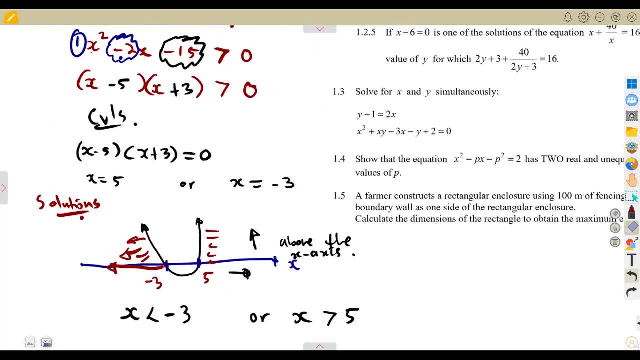 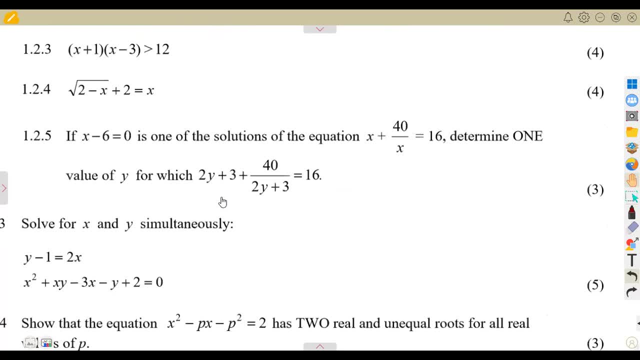 If we talked about this, then it's an advantage. All right, So that was the question of the inequality. Then we move on to another question, which was 1.24.. Again, solve the equation. This one is an equation We are solving for x. It's an equation because we have 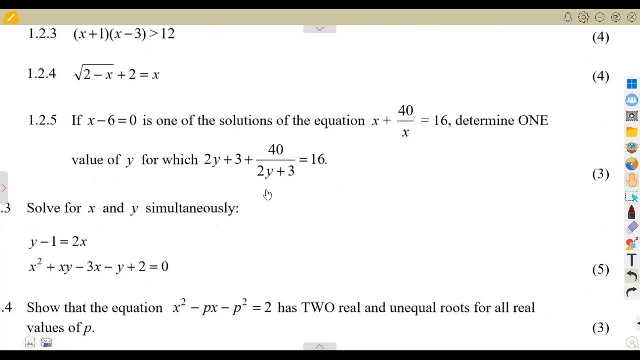 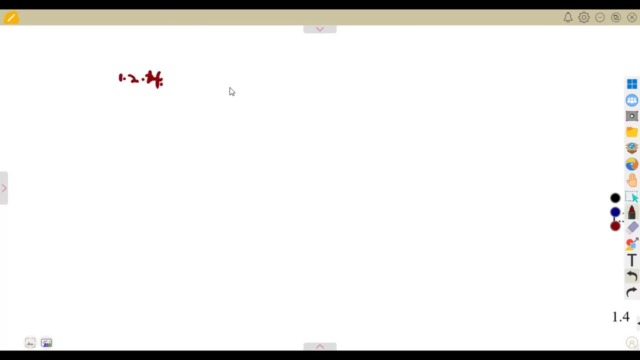 got an equal sign. That's four marks for that. I'm just going to rewrite this equation. So we've got four marks there, So 1.24,. you are given the square root of two minus x plus two, which is equal to x. So these are said. 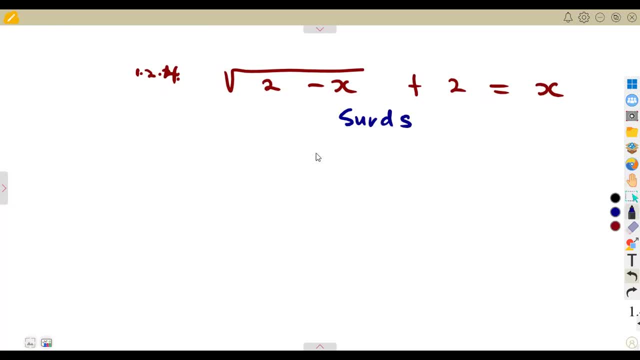 You are working with the sets like this. How do we solve these sets where there's a square root? What you need is to make sure that you remain with a single set on one side. You must have a single set on one side of the equation, meaning to say: I have to get rid of these two. Two is not. 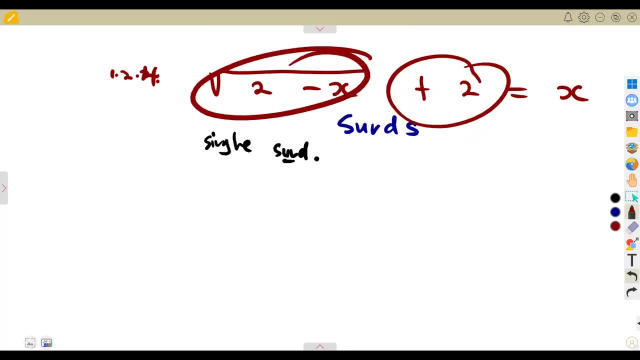 inside of the square root. It's just a number added to the square root, So we need to remain or we need to have a single set On one side of the equation and this is our set, this one, this part that is under the word. 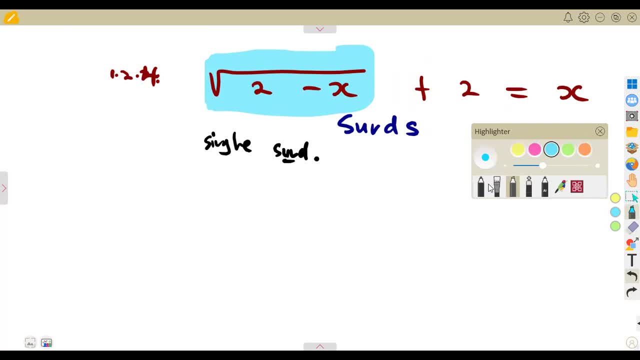 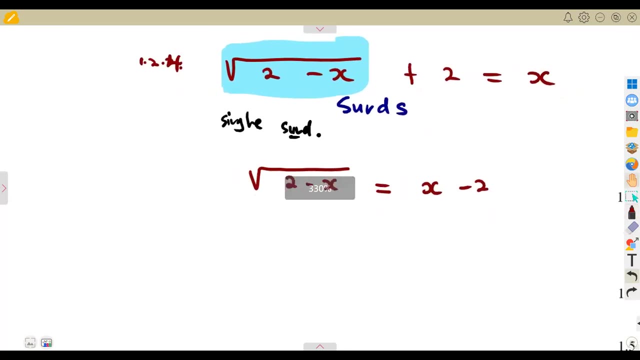 that is having the square root, So we need to make that the subject. So we are going to have the square root of two minus x is equal to transpose two to the other side, So it's going to be x minus two. It was a plus, So on the other side it will be a minus. So how do I get rid of? 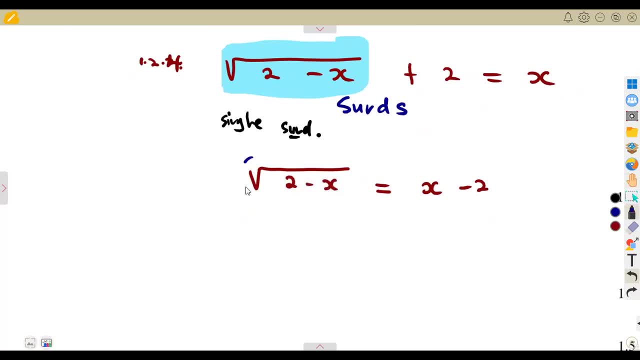 this by having a single set. I square both sides. On both sides, you are removing the square root, All right, So the square and the square root neutralizes. So meaning to say we are going to have two minus x, which is equal to x minus two. 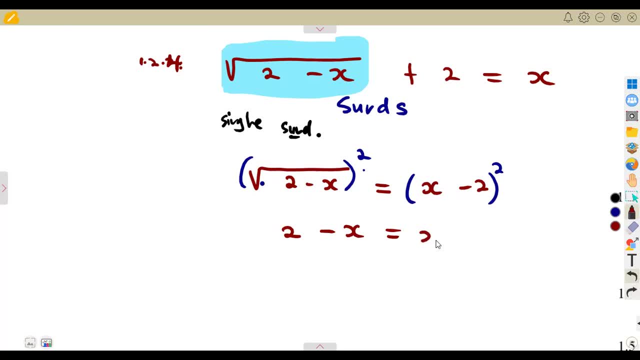 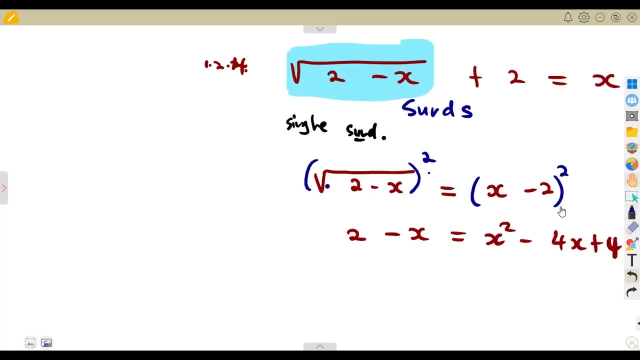 squared and x minus two squared. You're going to expand as we're going to two brackets: x squared minus four, x plus four, So you can use your identities or you can expand brackets as usual. There's a bracket of x minus two, a bracket of x minus two, So x and x. 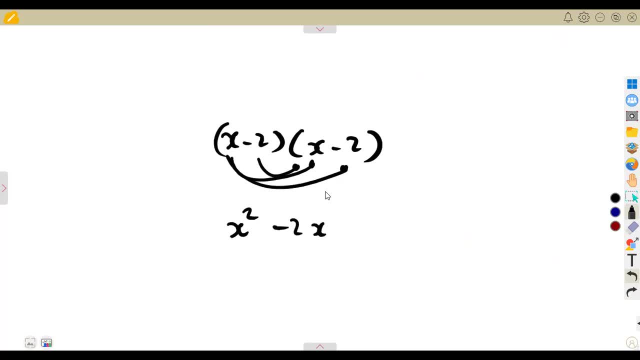 that's x squared- x minus two minus two, and x minus two and minus two, that will be a positive four. So these add together, that will be x squared minus two minus two. that's minus four, x plus four. you can do that- This one is up to you- Or you can just use your identities, Remember. 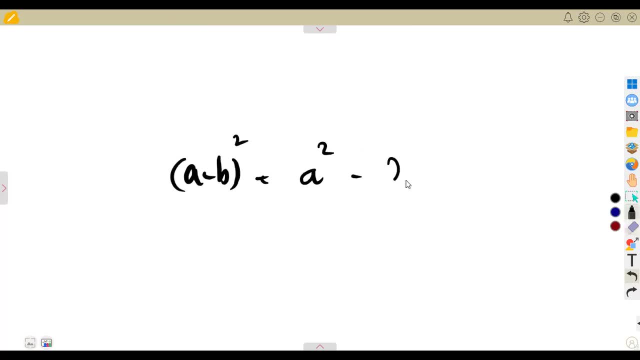 we know that a minus b squared is equal to a squared minus two, a b plus b squared. So we can use that, which is the one that I just used there. You can just use it in your head and expand A quadratic equation. we saw that in the previous case that we're supposed to have the format. 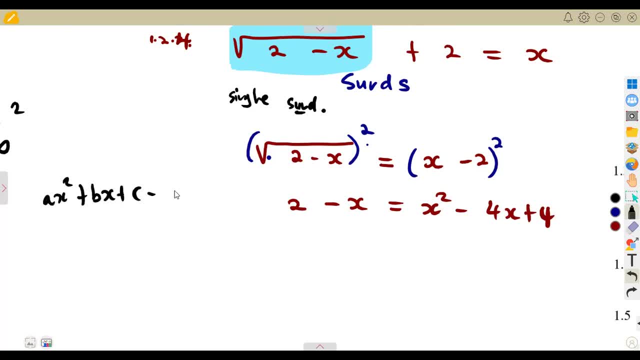 of a, x squared plus b, x plus c, which is equal to zero. So, having this, we can transpose this so that this side remains as a zero, And this is where we have a lot of terms. So it's better that we transpose these terms to the other side of the equation, So that's, zero is equal to zero. 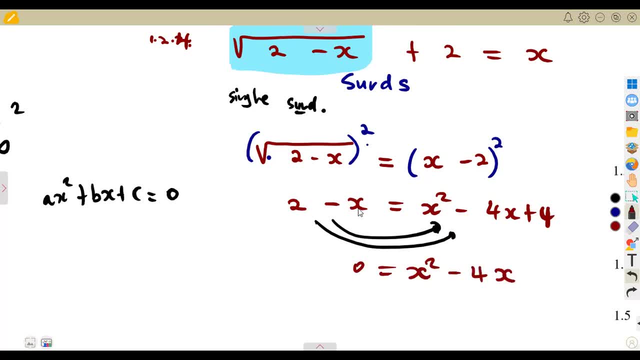 x squared minus four x. So if I transpose the minus x on this side, it will be a positive x. okay, the sign changes. a two will be a minus two, So that's four minus two, So that's zero is equal. 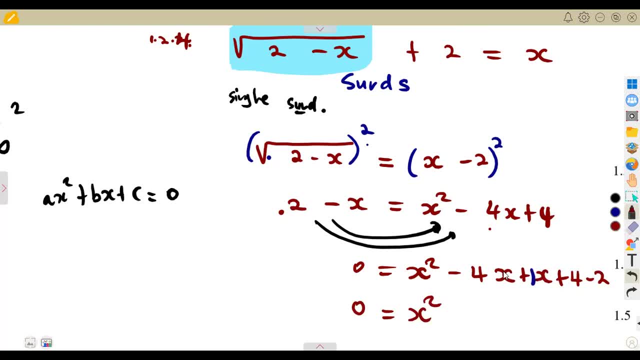 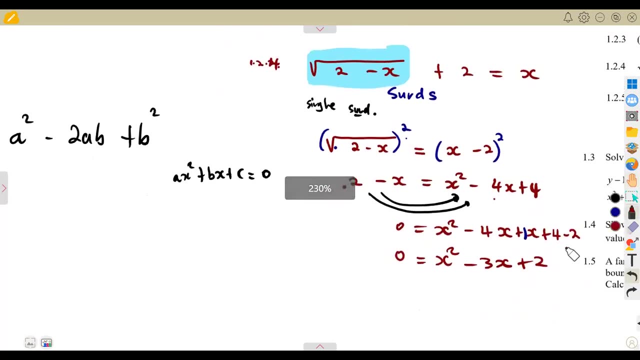 to x squared. If we add this, what are we going to have? minus four plus one, that is minus three x four. plus four minus two, that's a two. We are used to this Simplification. So from there now we can solve our equation, knowing that if a is equal to b, 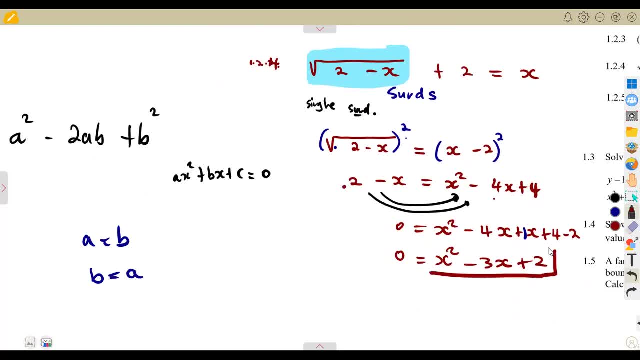 it means b is equal to a. So this does not stop me to take this and write it on the right hand side, I mean on the left hand side, without affecting anything, does not stop us to do that without affecting anything. Without affecting anything, we can do that. So, meaning to say at this stage: 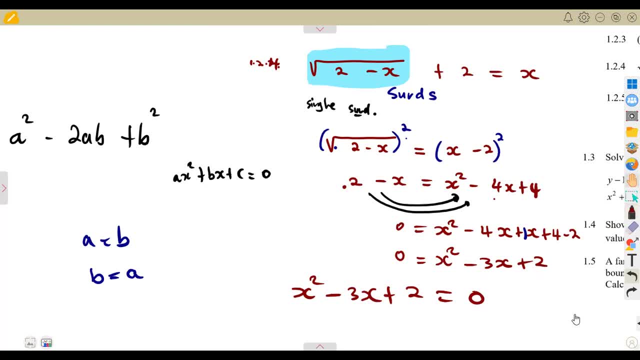 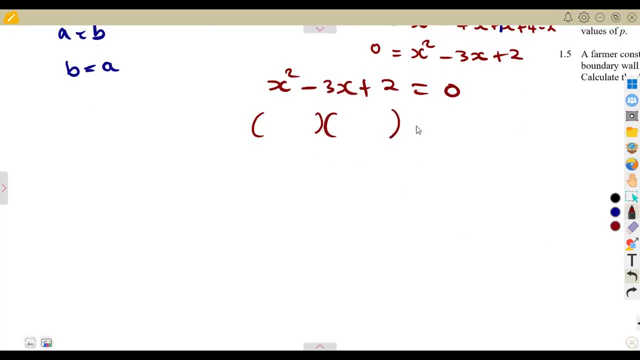 method. So in this case I'm just going to use the factorization method, taking advantage that the coefficient of x squared is one, So it means one bracket must be x, another one x, so that if you multiply x and x you've got x squared. So, taking the factors of positive two, factors of two, 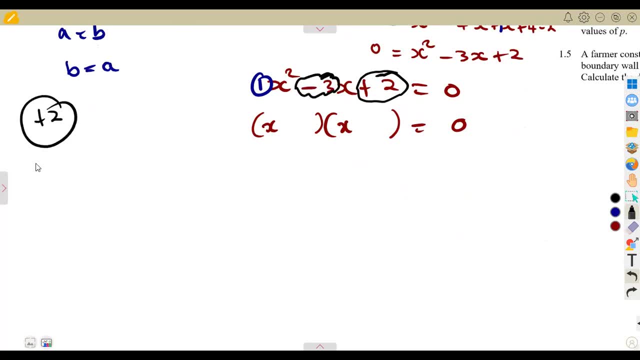 and these factors must add up to minus three. Since this is a positive, it means we are supposed to have our numbers as negative, all so that we get a negative. this one is a negative, this one. So if you have minus two and minus one, you multiply, you get. 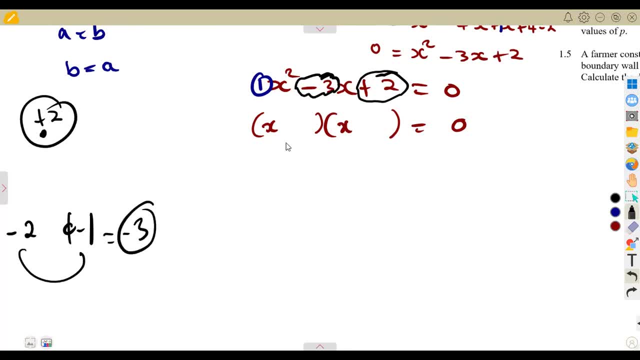 a positive, But if you add you get a minus three. So these are the numbers minus two minus one. So from this, x must be equal to what a positive two, or x must be equal to a positive one. So these are the x values. 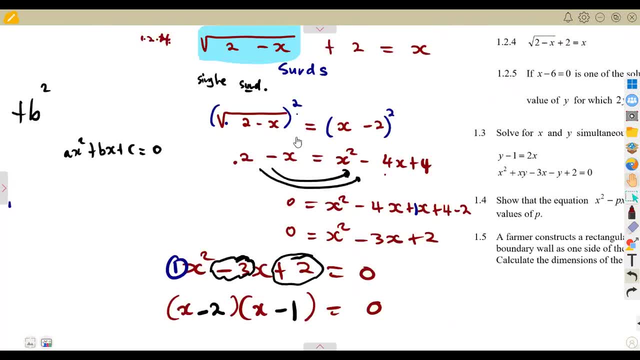 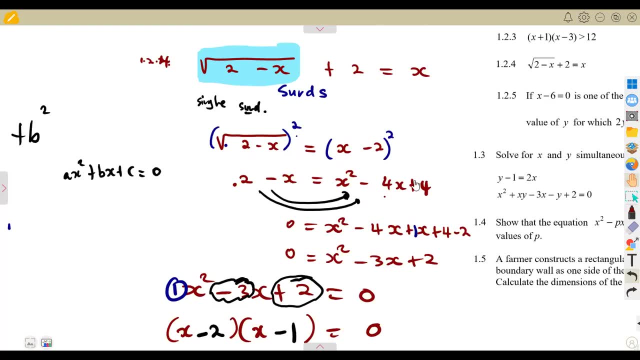 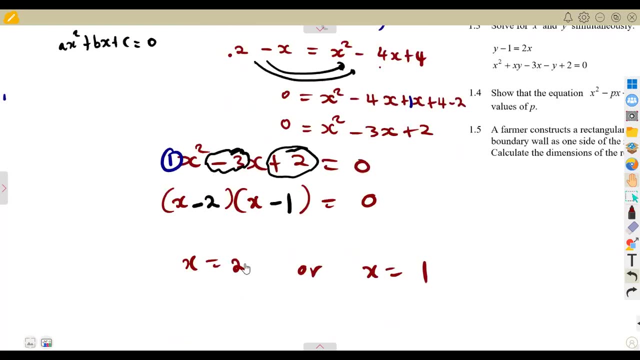 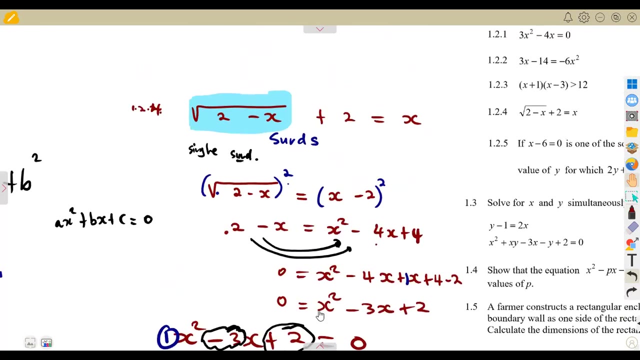 that we have. but as long you are working with a sad equation, test your solutions. Does this make sense? Does this make sense If x is equal to two? does this make sense? If x is equal to one, does this make sense? Okay, this is what I'm trying to say. If we are to substitute the x, 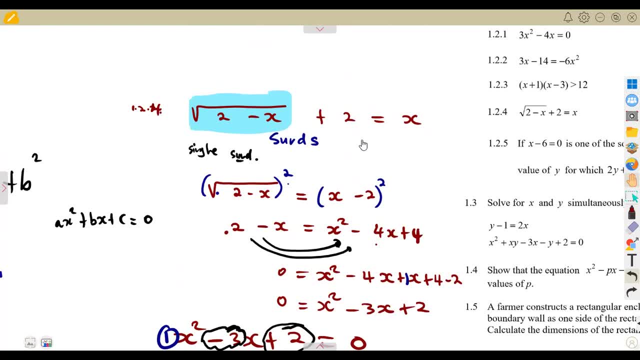 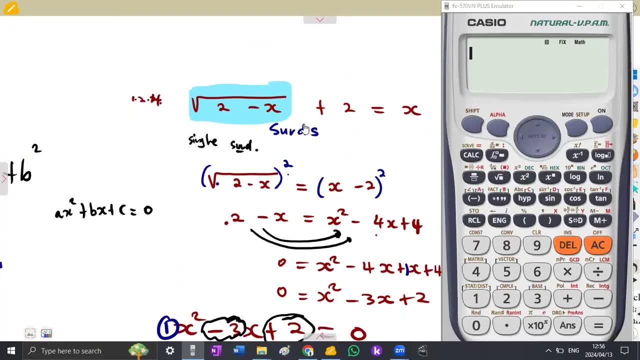 value that we had, the first value that we had the first value that we had. the first value that we had, there was a positive two. Alright, so this is it what you're going to have on your calculator. Remember, we fixed our calculator last part to two decimal place, So let's just go. 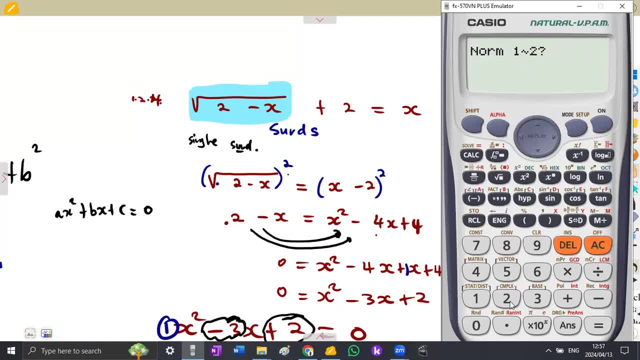 to the normal function eight. So you're going to press two, Alright. so this is the square root of two minus x. So this is two minus x. when x is two, Alright, then we move aside, there is a plus. 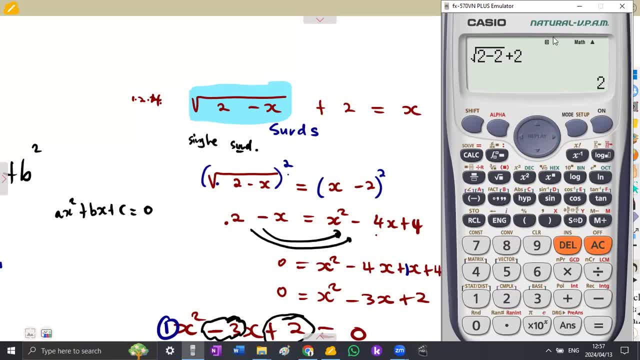 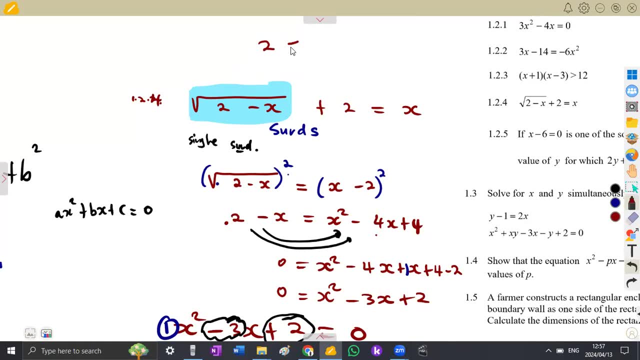 two also there, plus two. This is going to give us a positive two. So this is going to give us a two. Alright, so we are saying: this is two. the left hand side gave us a two. When x is what? when x is two on the right hand side, there's x. we substitute a two. So x is two, So two is equal. 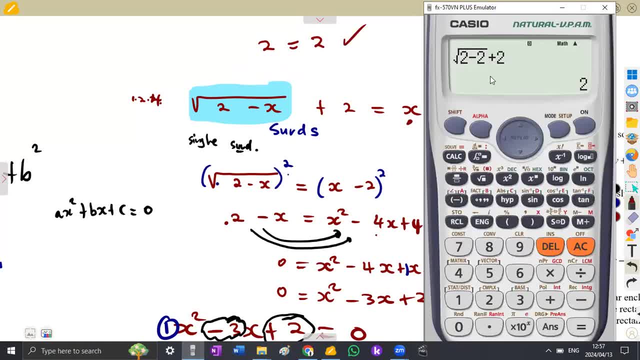 to two. This is good, This is correct. Okay, let's move on. When this x is one, remember, another solution is one. we substitute a one here. this will be the square root of two minus one plus two, which is a three. So this is giving us a three when x is the one. 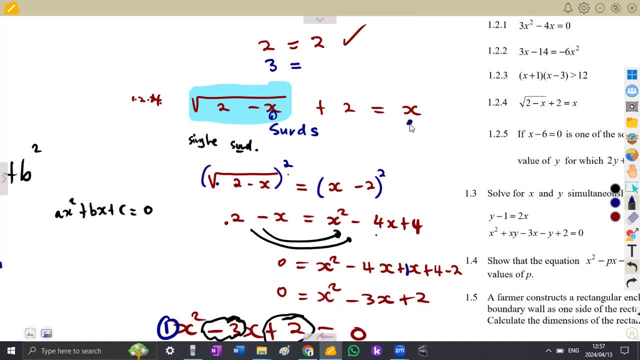 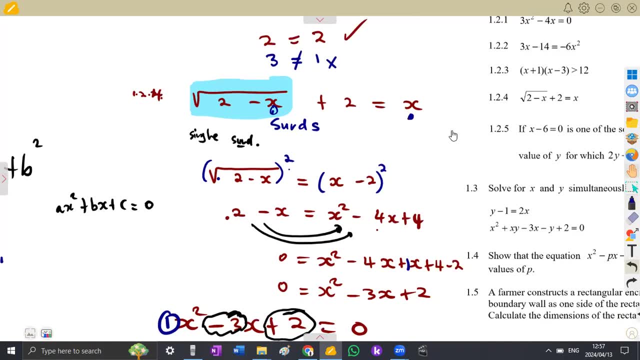 We get a three is equal to when x is a one. you subject a one three is equal to one. no, three cannot be equal to one, So meaning to say when x is equal to one. this is false, So x cannot be. 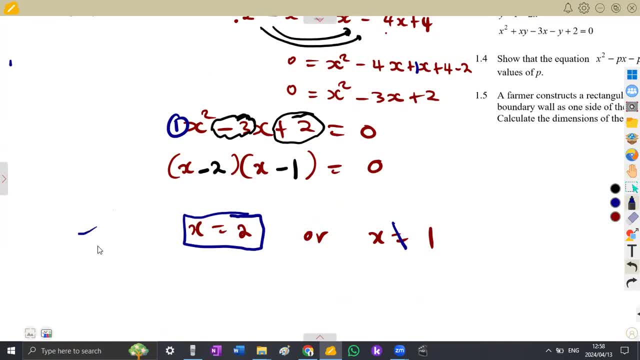 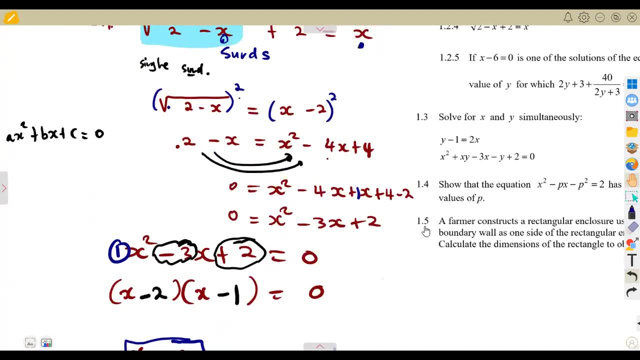 equal to one, but x can be a two. So always when dealing or working with a said- unlike any other quadratic equation that we are having here, where we never tested our solutions- when you're working with a said you have to test your solutions at the end. does the value of x that? 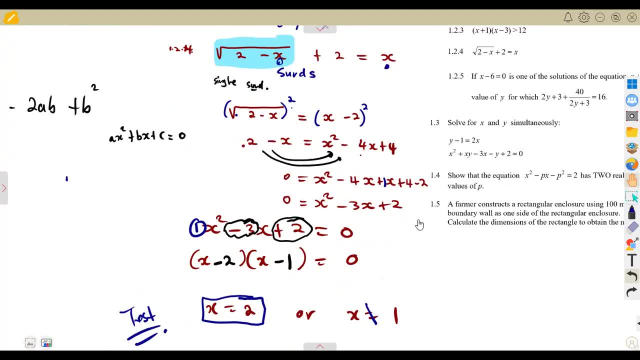 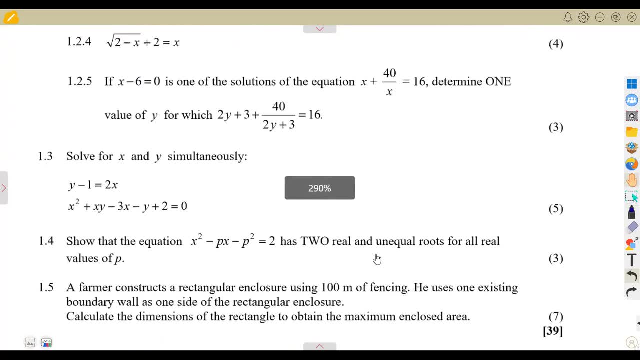 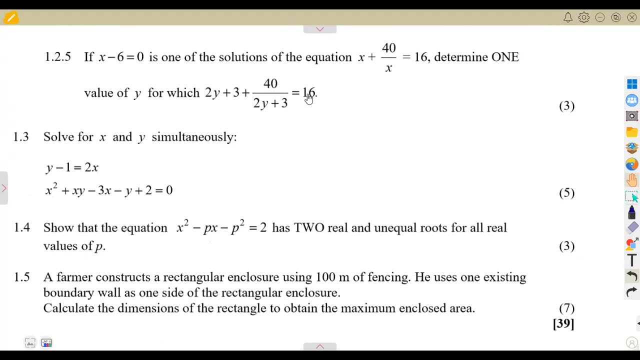 I'm given, does it satisfy the condition that is given? That is the case, All right. number 1.25, which is if x minus six is one of the solutions of the equation, this equation determine one value of y, for which this must be equal to one. So if x minus six is one of the solutions of the 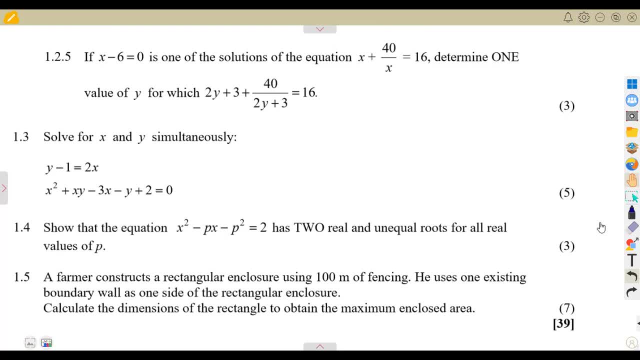 equation. this equation determine one value of y, for which this must be equal to 16.. So these guys, they are just playing around. they want to confuse you here. Take note: x minus six is equal to zero is one of the solutions of this. take note: this is x, this is 40 over. x is equal to 16.. 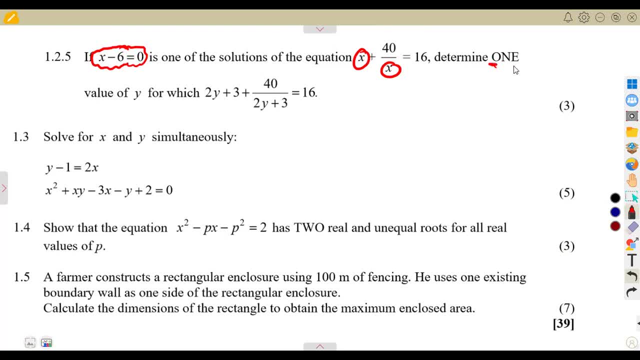 Now they're saying: determine one value of y for which take note, take note what is happening. Two, Two y, Take note, this is two y plus three. If you check, if you check the way that it is given. 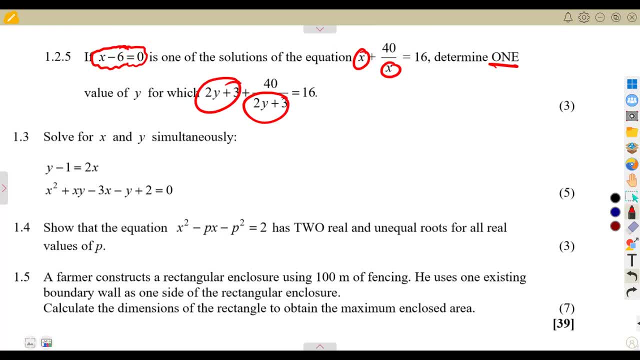 it is given as two y plus three, two y plus three. This is something that we are supposed to just have. a single term, x, Where there is x here. look here, guys. look here this one, this two minus y, is in place of x plus 40 over x. It was x here, but look here what they put In place of x. 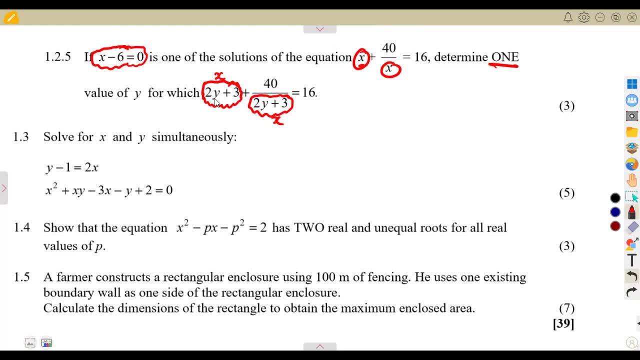 they put what? Two minus y? again This two, two y plus three. the same two y plus three. the same two y plus three. they are putting it in place of x. The 40 is the same as this 40,. the 16 is the same as this 16.. 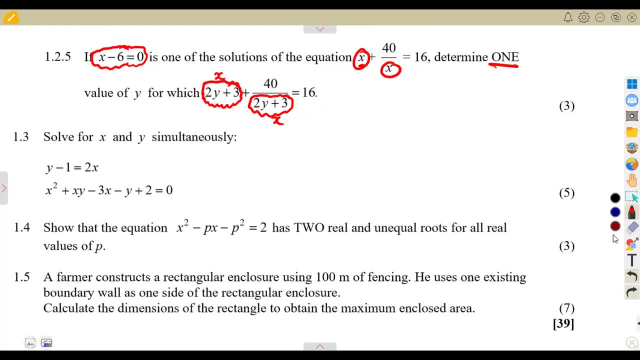 They are just repeating. So if this equation where there was x here, if the solution of this equation is given like this, what's the solution? The solution is: x minus six is equal to zero when this is x. So what is x there? It means x is equal to what. 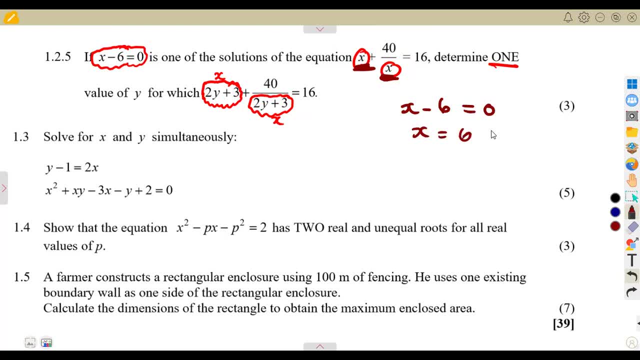 transposed to the other side, x will be a positive six. Please listen to me. When x is equal to six, this is the value which satisfies this equation, when this is x here. But look now where x is, which is the same x, which is six. 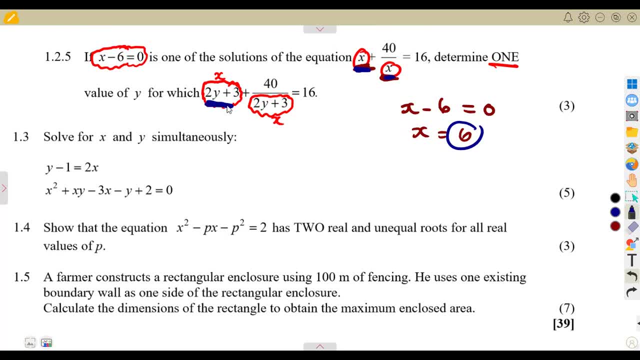 Where x is. this time it's no longer x. They are now putting this as two y plus three. So we are simply saying: if they can write two y plus three in place of x, it means two y plus three is equal to x. They just substituted what is equal to x as an expression. 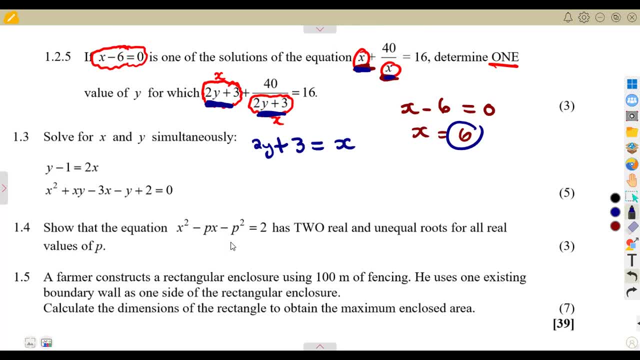 Just like that. They just substituted something equivalent to x, but as an expression of y, And now we have got the numerical value from this equation that they told us that x minus six is what It's a zero, And we saw that x is six. So if x is six, it means two y. 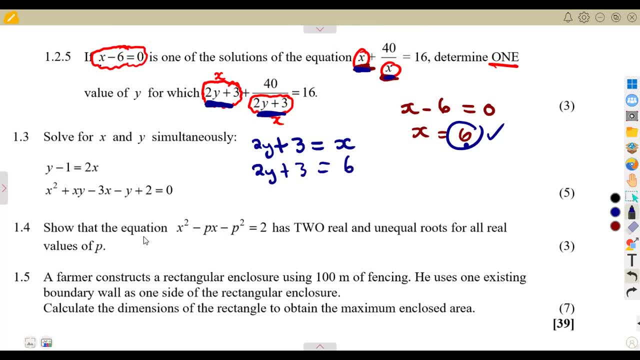 plus three also must be equal to six. So what is the value of y? That is what they are testing. They wanted you guys. They wanted you on this question. They wanted a lot. So be careful, Very, very careful. So two y is equal to. 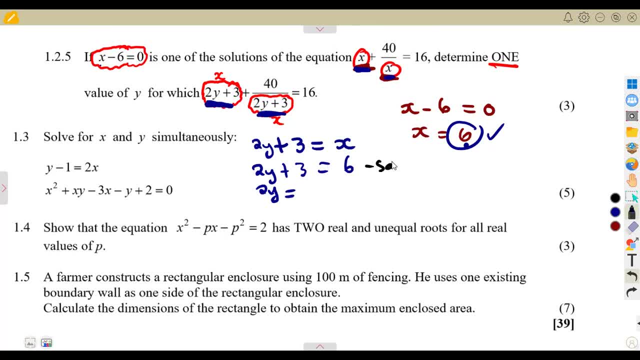 transpose. we are now solving for y, in this case an equation. So you can now solve for y. Transpose three to the other hand, it becomes a negative. So that's six minus three, which is a three. How do we solve two y? It's a multiplication, So you divide by two. So therefore y is equal to. 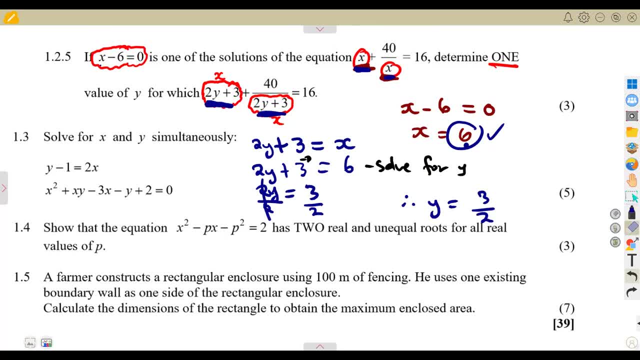 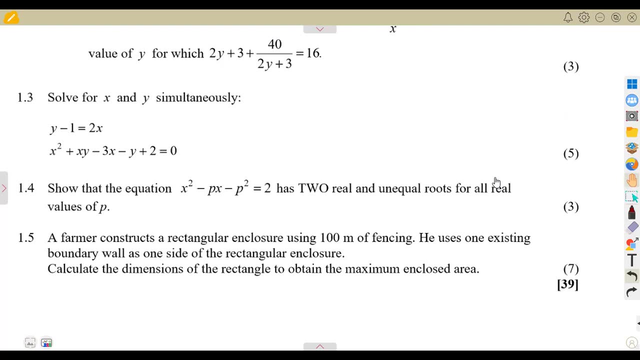 three over two. So that's a single solution, one solution that we are having there, which is the value of y. So you see how do they try to to manipulate what you know, just to confuse you guys. So don't tend to be confused whenever you. 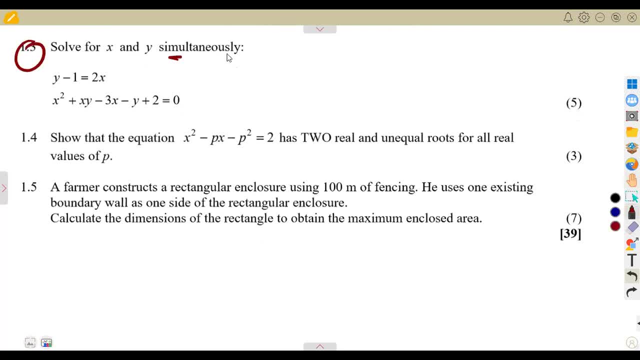 see something like this: So for x and y simultaneously. so they were given two simultaneous equation equations: y minus one is equal to two x. So this is, let's say, our first equation. then we are also given x squared plus x, y minus three, x minus y plus a two, which is equal to zero. 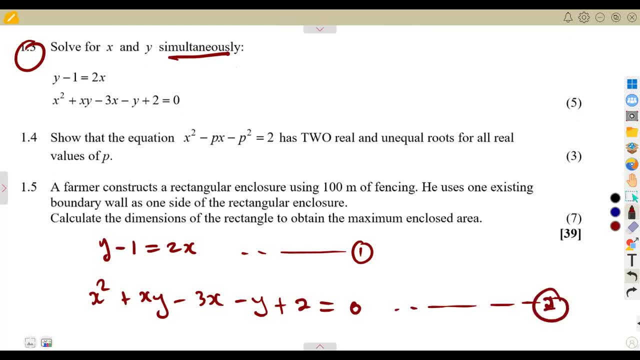 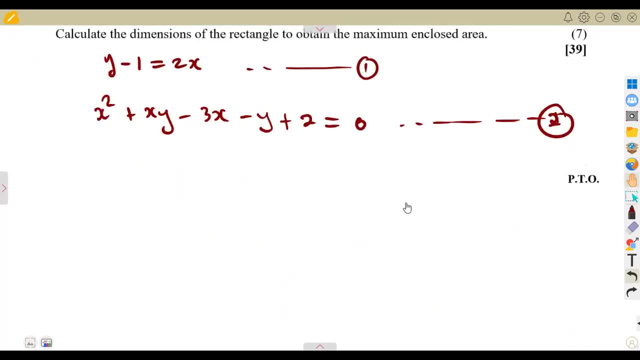 So this- let's say this is our second equation- and five marks to solve for x and y. All right, so that is what we have there, 1.3.. How can we solve for x and y? That is the question. 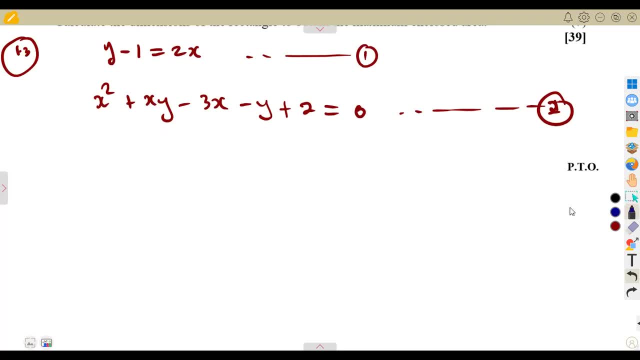 If we are to consider this, we know that it is the best way to use our substitution method ways. either I'm going to make x the subject substitute in another equation, or I make y, the subject, the subject substitute in another equation. So there's your choice. which part are you going to to use from these two? 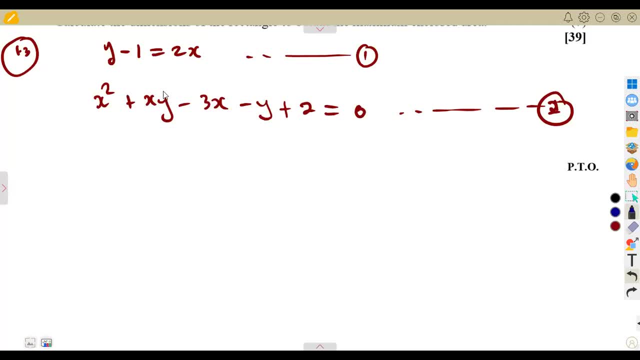 So if you were to consider the first equation, it is easier for us to work with the first equation. in the first equation, we can just make why the subject transpose the minus one on the other side. That's a positive one. That's a positive one, Although it's easier. 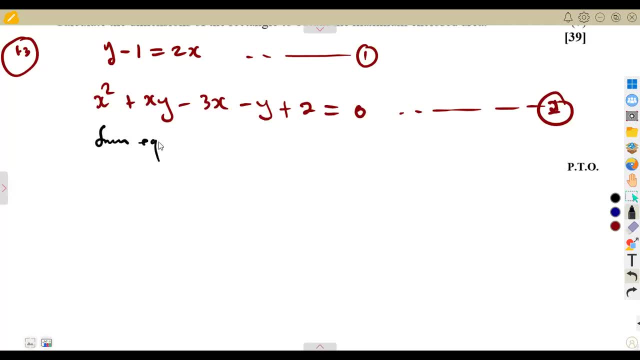 for us to make y the subject So from equation, So from equation one gonna make y the subject, so y will be equal to 2x transpose 1.. On the other hand, minus 1, it will be a positive 1.. 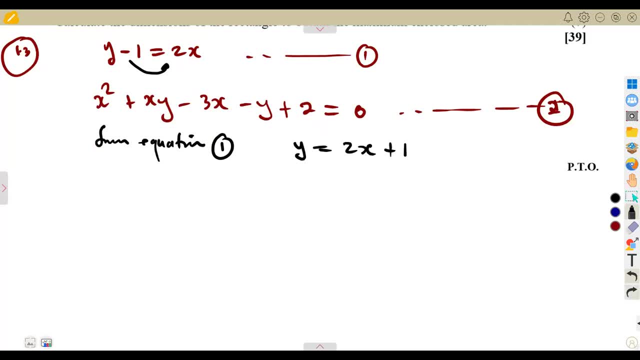 So this is another equation that we never had, but we have to formulate it from another equation So we can name this now our equation 3.. So this is the whole idea of your solving of this simultaneous equation: Just work with the easiest path. 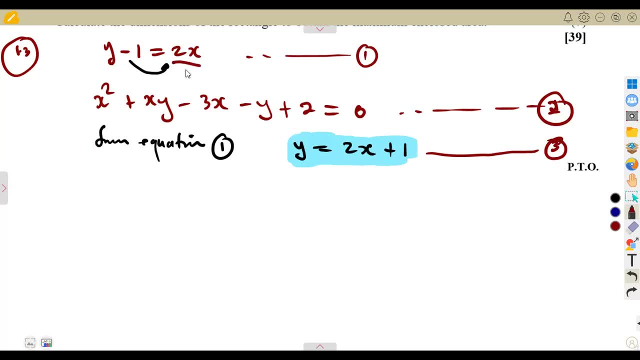 Just imagine you want to work with x. Yes, you can divide by 2.. Just look, you're working with a fraction there. You are working with a fraction and when you substitute, there's an x squared, meaning to say you have to square. 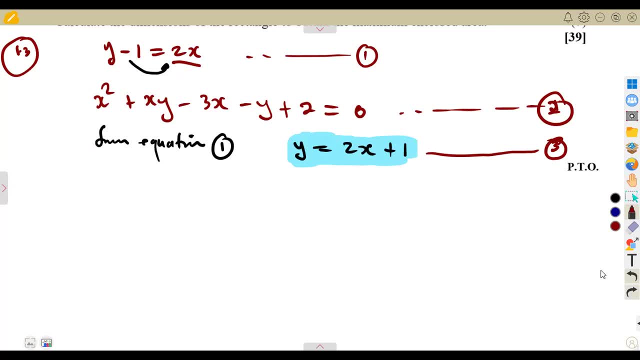 So be careful, also Analyze your equation. It's not just I have to make the subject. Analyze and see what's easier for you to work with, Not to say you're not going to have the same answers. You will have the same answers. 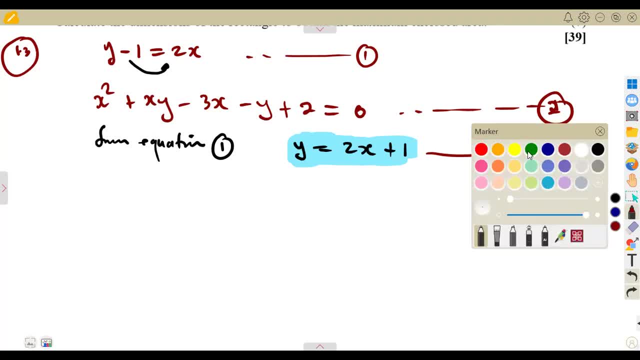 but avoid working with complicated situations. So just analyze Before you do that, then you can solve All right. So from the equation 3 that we now have, you are going to substitute in the other equation, not the first one. No, because that is where you made why the subject. 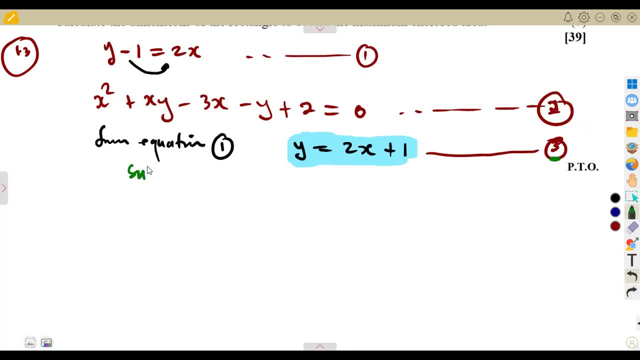 So you substitute into the other equation. So you are going to substitute equation 3.. So now I'm just going to write in short. So I'm just going to write in short: Substitute equation 3 into equation 2.. All right, 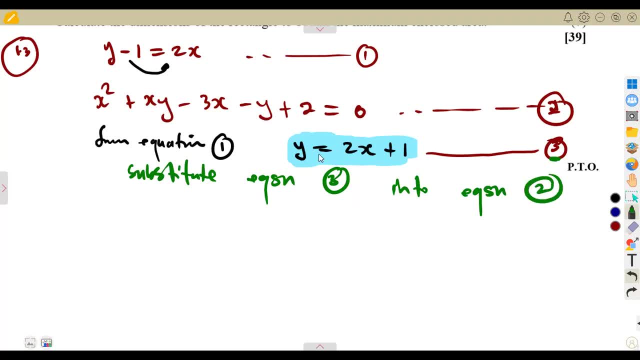 So you're going to substitute this into equation 2.. That's in equation 2.. Wherever there is a y, you are going to substitute the equivalent of this, which is 2x plus 1.. All right, So this is x squared. 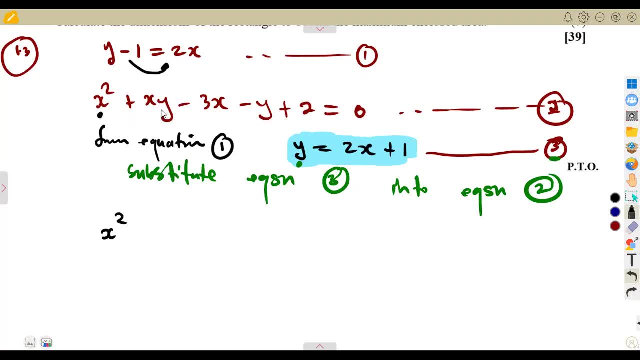 There's nothing to be substituted there. Then we've got plus xy, Where there is a y. here you substitute what is y, So xy means x times You multiply to what is representing y, which is 2x plus 1.. 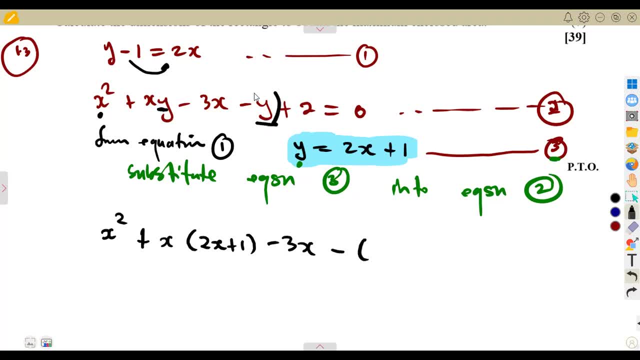 Minus 3x, minus y. in this case, Where there is a y, just open a bracket. Substitute what represents y there Plus a 2. That's equal to 0. Always substitute properly. Okay, Open brackets whenever it is very, very necessary. 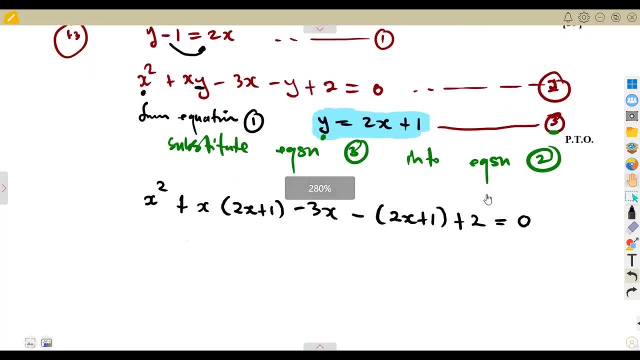 All right, Whenever it is necessary, do that. And with this equation we can see that we are just left with x, So we can solve for x. So expand the brackets. x squared, that's x and 2.. This is going to be 2x squared x and 1.. 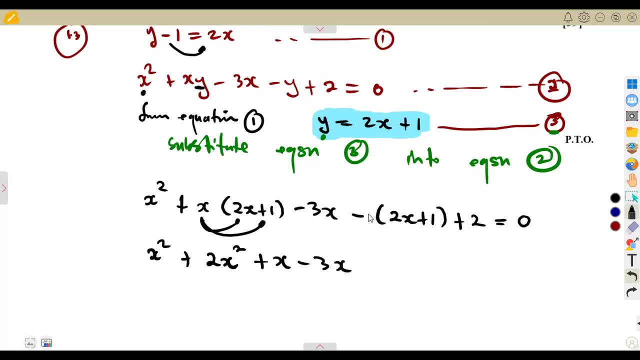 That's plus x minus 3x. Then here there's a minus 1.. If the number is not indicated invisible, there's a 1.. So it means minus 1 times 2x minus 1 times a 1.. So you're going to have minus 2x minus 1 and a positive 1,. 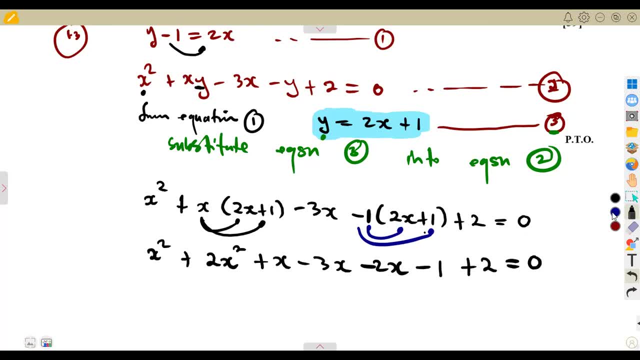 a minus 1 plus a 2. That's equal to 0.. So what I want you to do is to solve, I mean to combine the parallelism. you have x squared. this is 1 and 2.. So 1 plus 2, that is going to be 3x squared. 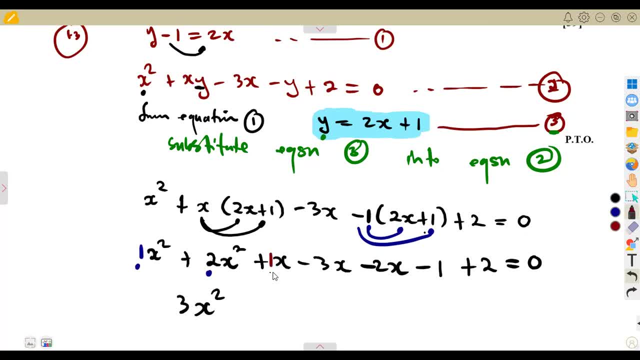 You do the same thing on the x. This is 1x, So this is 1x minus 3x minus 2x, So this will be minus 4x, So you are going to obtain minus 4x there. 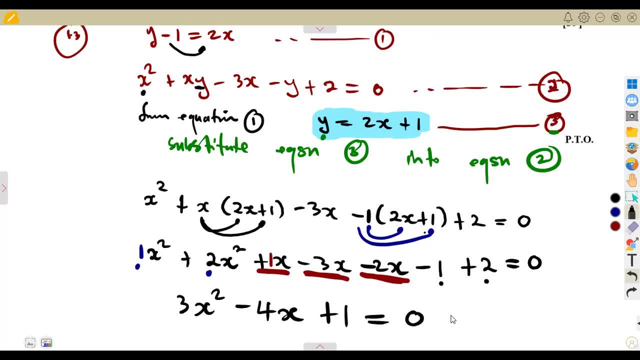 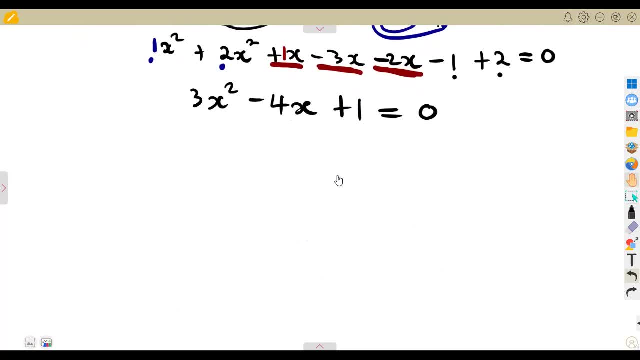 Minus 1 plus a 2. That's a positive 1, which is equal to 0.. So you're having these equations And that you are seeing here, Solve that equation. To solve it is your way, Use your quadratic formula: factorization. 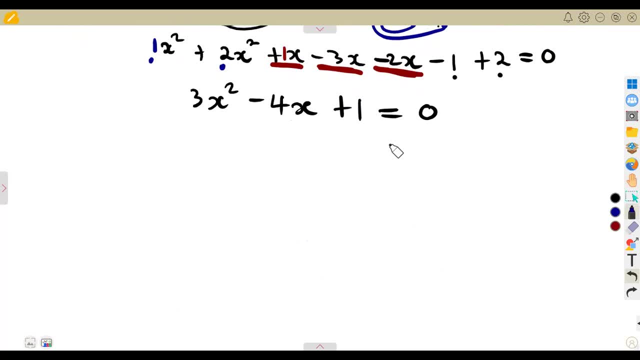 So in this case, I hope we used the quadratic formula. We used the factorization before, So this one is our choice. I'm just going to use the formula in this case. Most of you guys, I see you have a confusion whenever you see a number like a 3.. 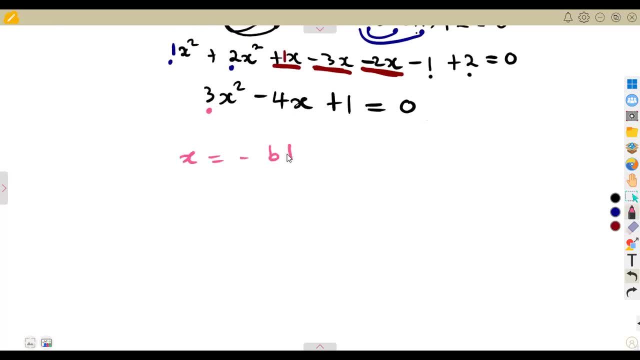 So if you have that, just avoid that. Just avoid. use your formula minus b, plus or minus the square, So you're going to have minus b, plus or minus the square root of b, squared minus 4ac. substitute your values, You are done. 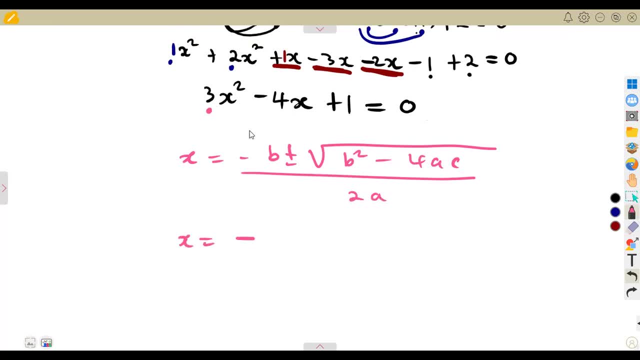 So x will be equal to minus. Remember this is our ax squared, bx and c. So our a is 3 or b is minus 4 and our c is plus 1.. So you're going to have minus b, So b is a negative 4.. 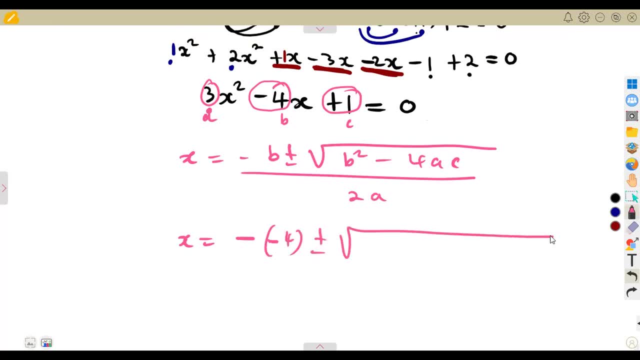 That's why, when I have minus, minus there, plus or minus, the square root of b squared our b, which is minus 4, squared minus 4 times a, which is 3.. So you're going to have minus b And our c, that's a positive 1.. 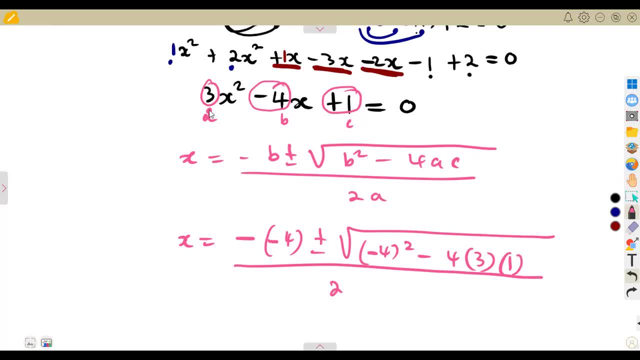 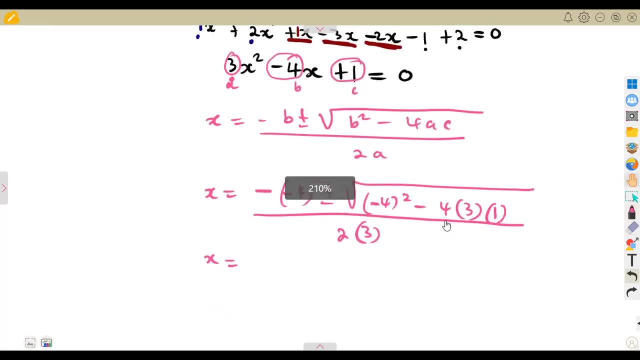 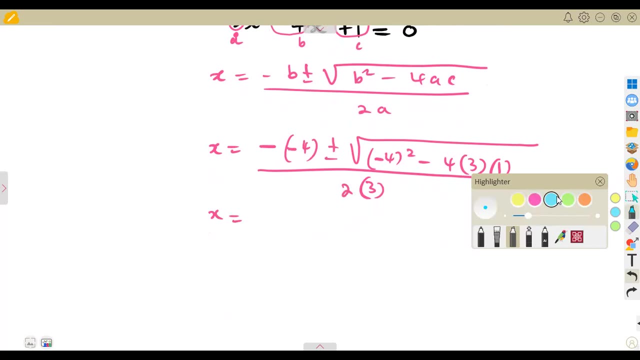 All right, Everything here is over 2 times a, our a, which is a 3. So if you were to simplify this so that you avoid confusions, like I said, just simplify what is inside of the square root. But this one is not part of our question. 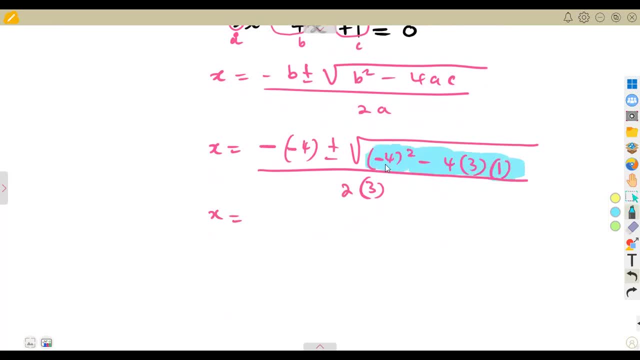 So you can even avoid that, But just try to simplify this part under the square root. So let me just be a coach to show you what I'm trying to say Here. this is what I'm trying to say On this part. you are going to do it like this: 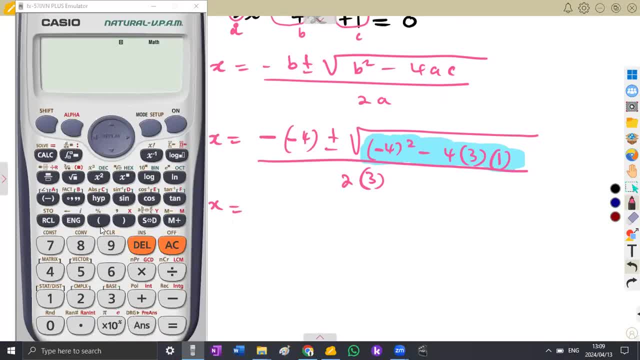 So just simplify: This will be open a bracket. It's just going to be minus 4 squared. So that's minus 4 squared minus 4 times 3 times 1.. So that's it Times a 1.. All right, 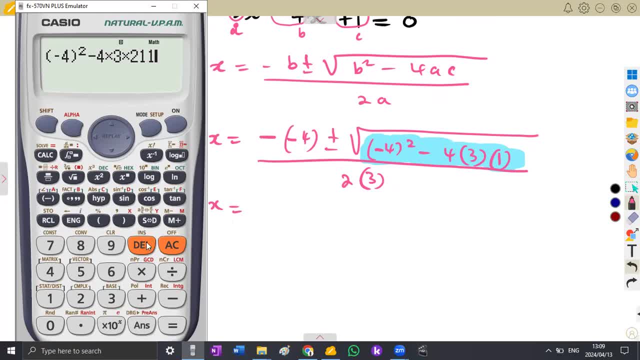 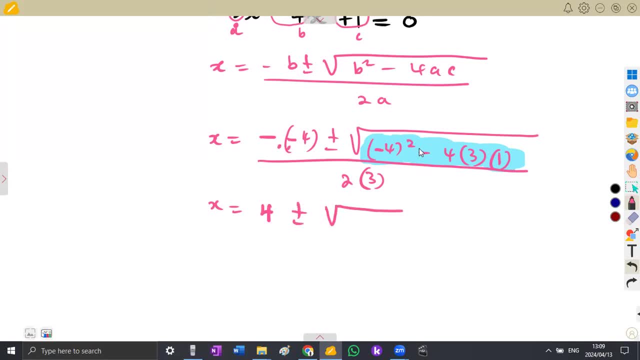 That's a positive. So it's 4 plus or minus the square root of. So you simplify the whole part here You've got a 4.. Everything over a 6.. 2 times 3. That's a 6.. 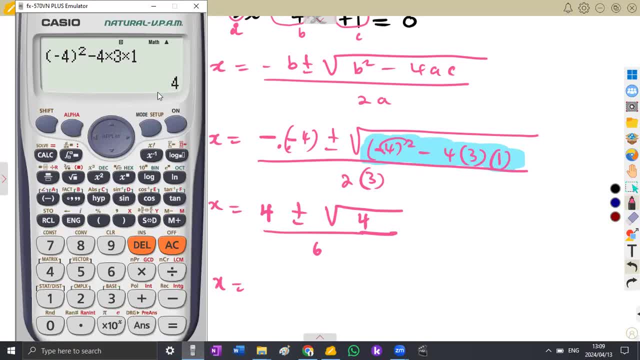 All right, So meaning to say x is going to be what. Now you can do whatever that you want in this case on your simplification. All right, So they're going to have a fraction. Then you have 4 plus. you go back here or you just use this one. 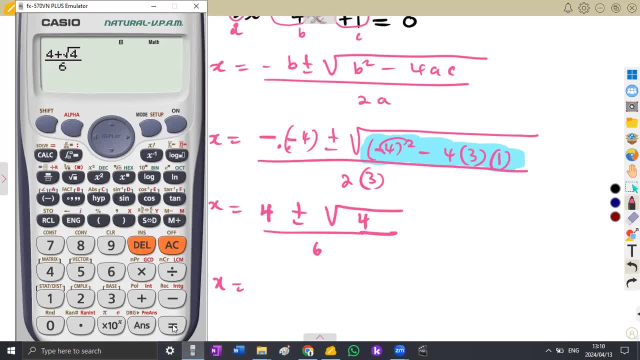 It's up to you, The square root of 4 over a 6.. So the first solution is giving us a positive- 1 or x is equal. to move on to the other solution, which is just going to put a negative, And this is going to be 1 over a 3.. 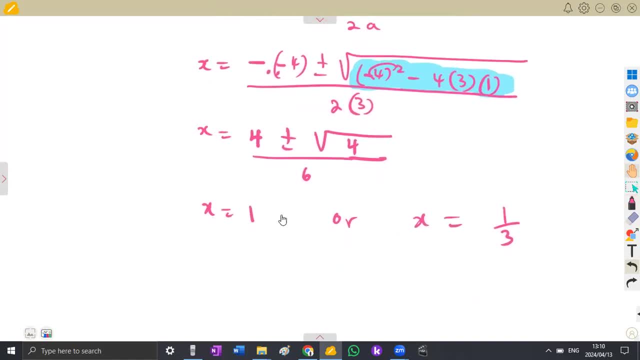 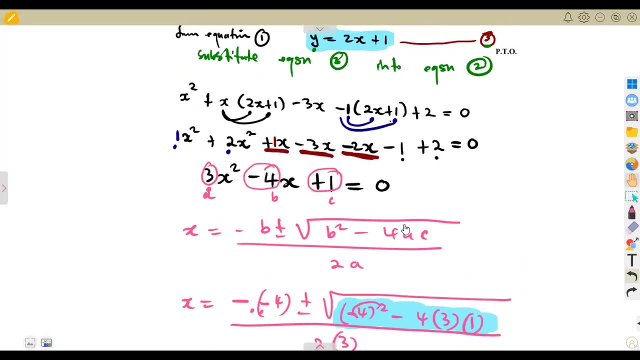 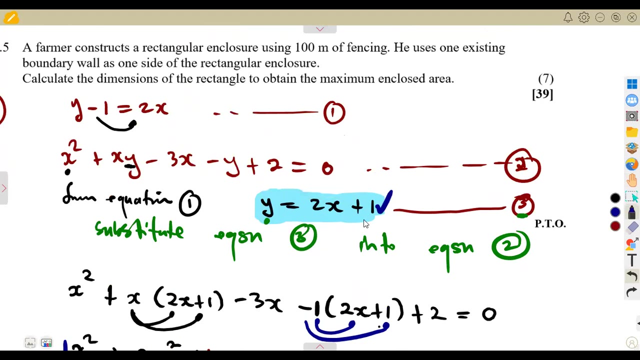 So we are obtaining two values of x: X which can be a 1, or x which can be 1 over 3.. And with these values of X you cannot substitute where in equation 3, because if you check, equation 3 is the best equation to substitute to find the y values, because already y is the subject. y is equal to 2x plus 1.. 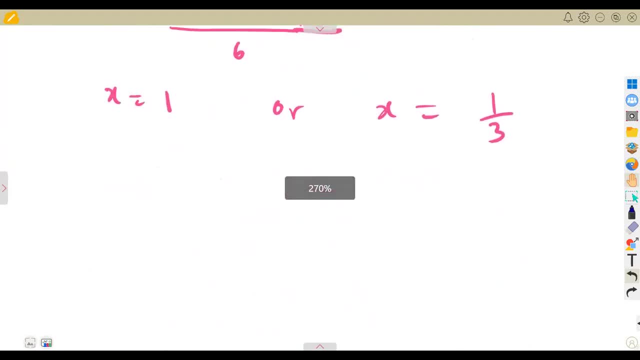 So, taking that into consideration and also as an advantage, that y is equal to 2x plus 1, you're just going to substitute when x is equal to 1.. You substitute here, So y was going to be a positive 3.. 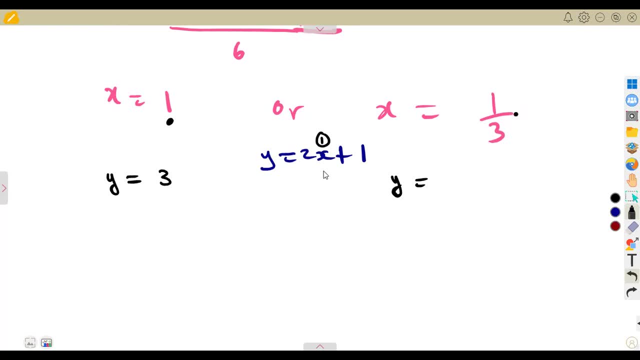 If you substitute when X is 1 over 3, on this part you substitute 1 over 3.. You are going to see that your y value was going to be 5 over 3.. So this like a pair, You're simply saying when x is 1, y is 3.. 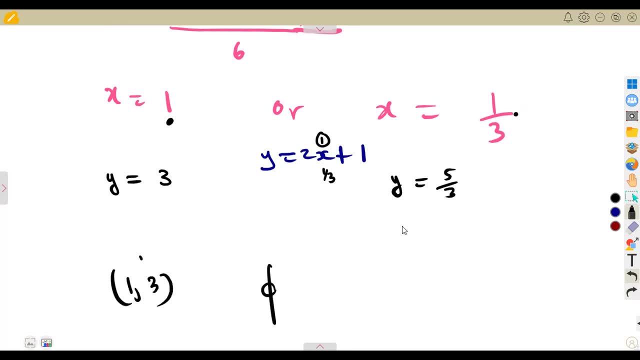 You can even write as points 1, 3, like this, and another point where x is 1 over 3, 5 over 3.. This presentation is up to you, Up to you. Writing this: that x is this value and y is this value at this point is enough. 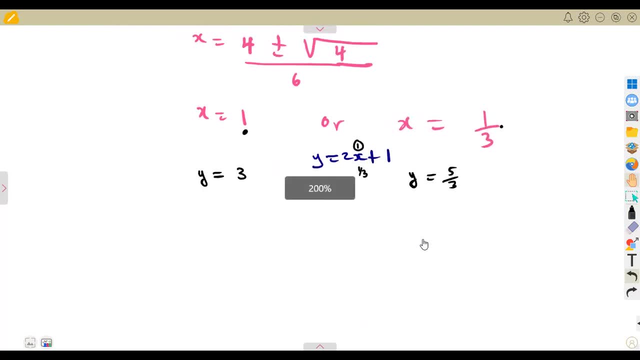 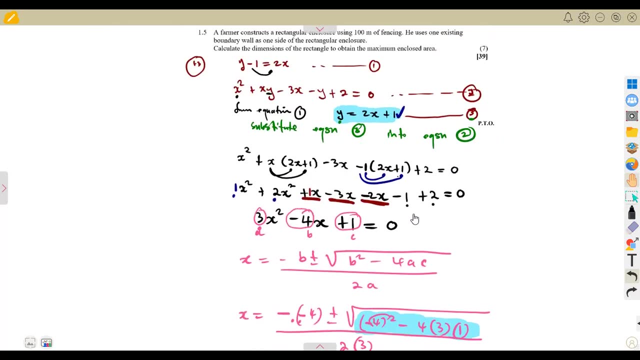 So writing, Writing as points. it's another bite up to you unless, if the question was determined, the coordinates of point of intersection You have to indicate in point form. when it is like that, You do not have a choice. when it is like that, 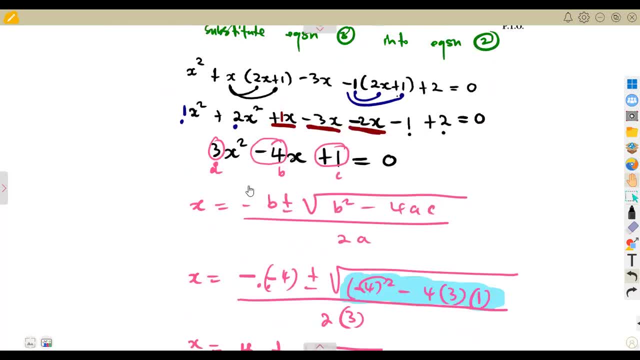 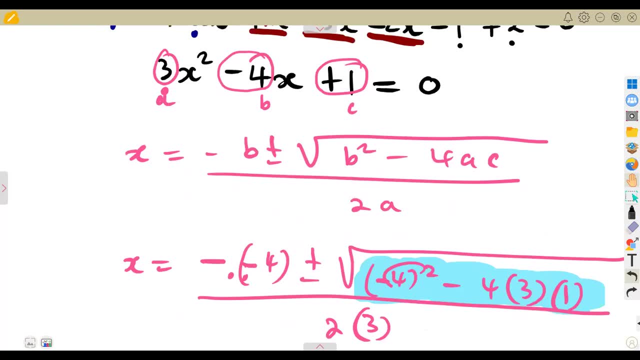 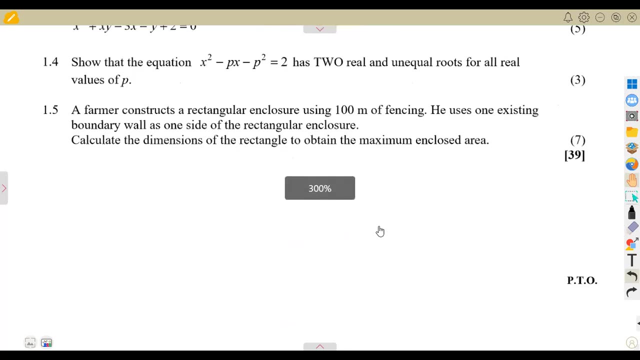 So, like I said, you could have used factorization. So I want you to use the factorization and see if you are having the same answer on this part here. Use a factorization to prove if you are having the same answers, Because on the values of x, if not, then that means there's something that you need to be worked on on that part. 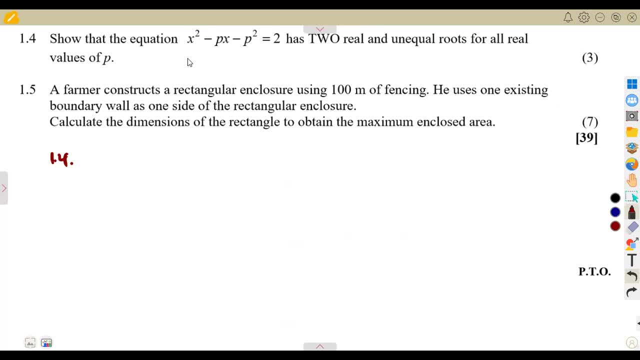 1.4.. We are given show that this equation that we are given is two real and an equal roots. The first thing is they're supposed to be real roots. Real roots, That is any real number. It can be any real number. 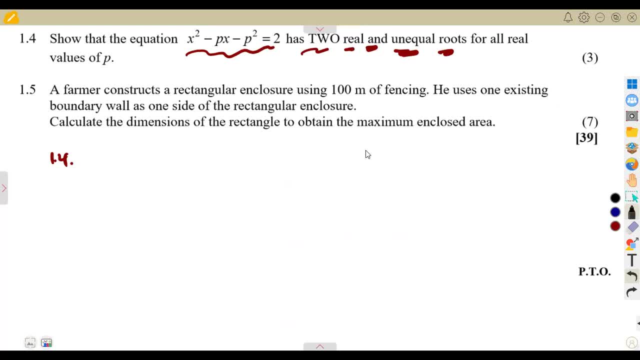 Meaning to say what we are talking about. when it is a real number, We talk of the solutions. It means our discriminant or our delta part. Just for having real solutions, it must be greater than zero. So they are saying now, is this going to be the roots? 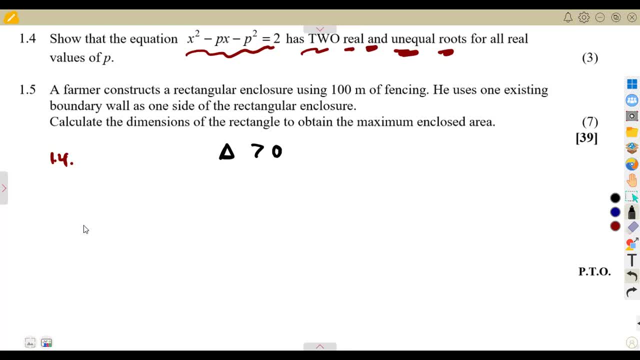 They are real and unequal. They are not equal. OK, so what is the case? now? The discriminant, what does it? what does it mean? Or our delta. It is taken from the equation ax squared plus bx Plus c, And we know that, if we are given this nature, this discriminant which is our delta is supposed to be b squared minus four ac. 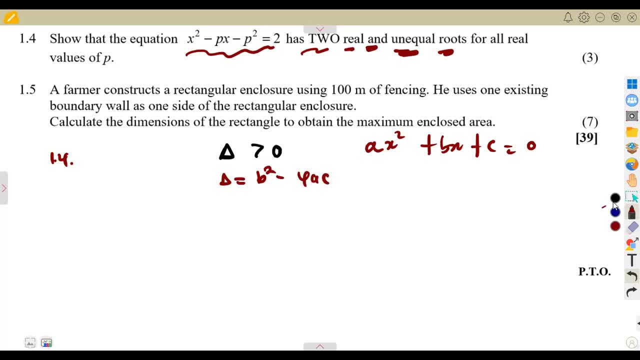 So we could be squared minus four ac. But we need the format from this. We need first the format because it must be of this nature, equal to zero. So this equation we are given as x squared minus px minus p squared is equal. It's not equal to zero. 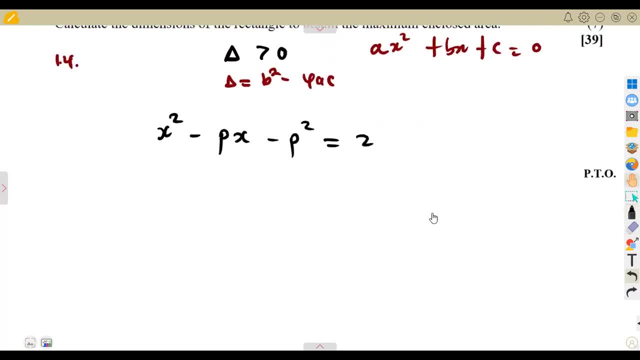 It's equal to what? To two, This Must be equal to zero. So what you're going to do is to transpose the two to the other side, and x squared minus px, minus p squared minus two is equal to zero. So it was a positive. 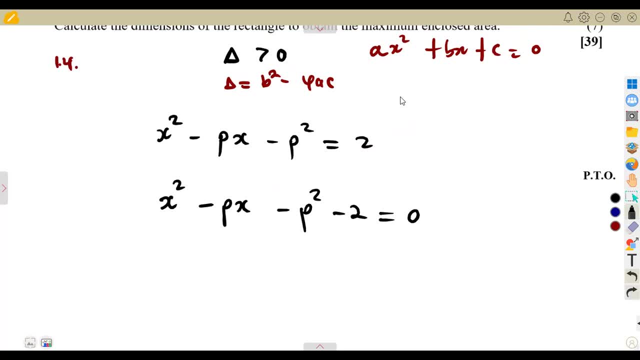 It will be a negative. So this must be a x squared, a x squared. So our a is the one plus bx, b, b, b x, x. There must be x, So our bx- we're talking about b. This is our b. 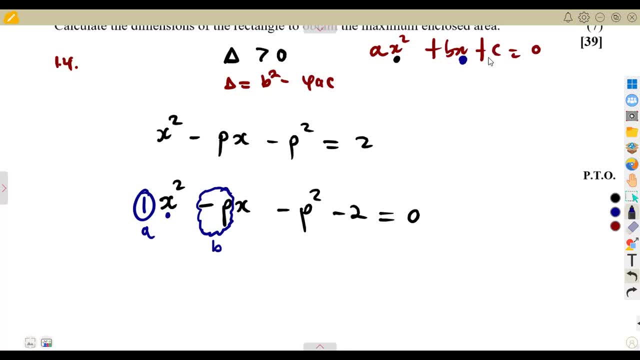 So this is our a, This is our b. C is the constant. On the constant there is no x, So they can put any letter what they want, But if there's no x, this whole part is our constant. This is our c. 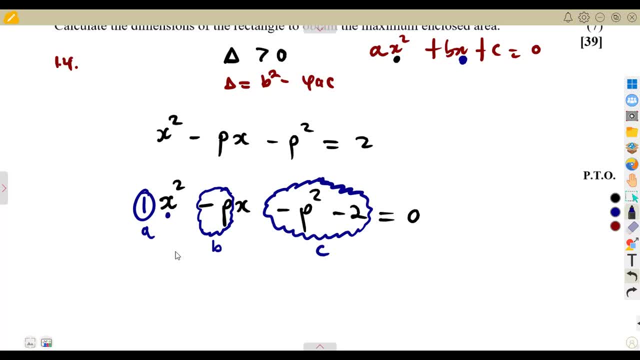 Where we do not have x, Where we do not have a variable, Like the variable is x, P is a constant. Now we treat p as a constant, even though p is a letter, But we are treating it now or we are taking it. 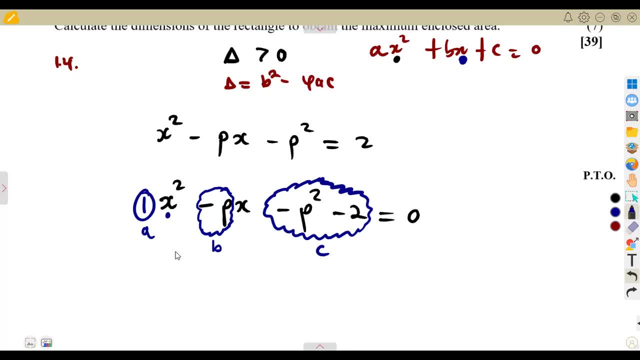 As a constant for now. So meaning to say, if I am to use the b squared minus four ac, Let's check our. b is p minus minus p, So that's b squared minus four ac. A, b, which is going to be minus p, squared minus four times a. 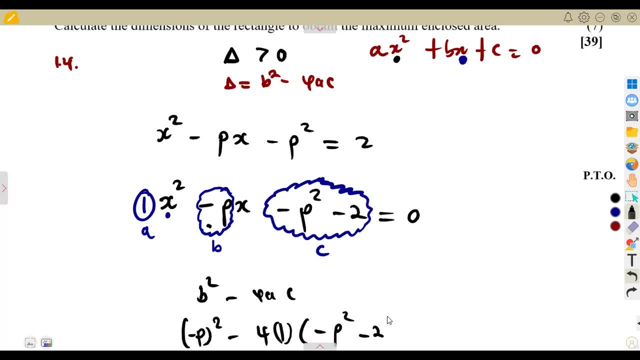 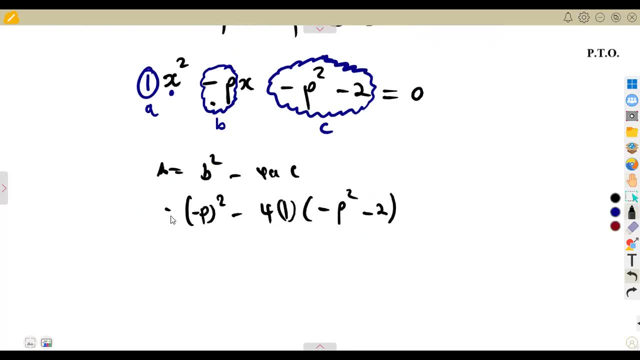 Which is one, our c. That is minus p squared minus two. This is our, our delta, Which is our discriminant. So minus p squared- Remember a negative from our grade nine. when raised to an even number It becomes a positive. So that's p squared minus four times one. 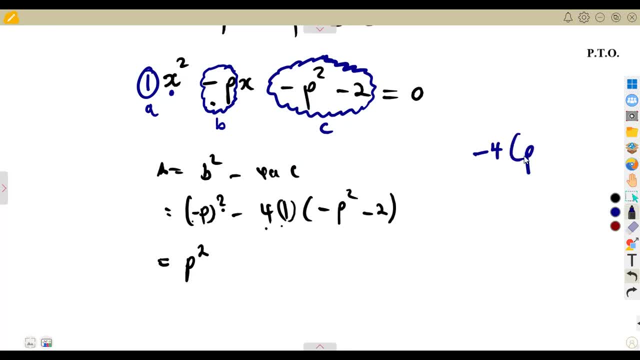 That's minus four. So it means we've got minus four into the bracket of minus p squared minus two. So that's minus minus. That will be a positive Four. p squared minus minus, That will be a positive eight. Four times two, which is eight. 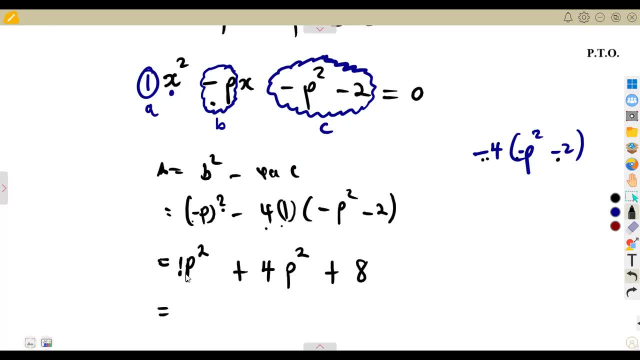 So if we are to Add- this is one p squared, One is invisible- One plus four, That will be five p squared plus eight. So the question is: Are the values of p that we are talking about here Going to maintain that this is great? 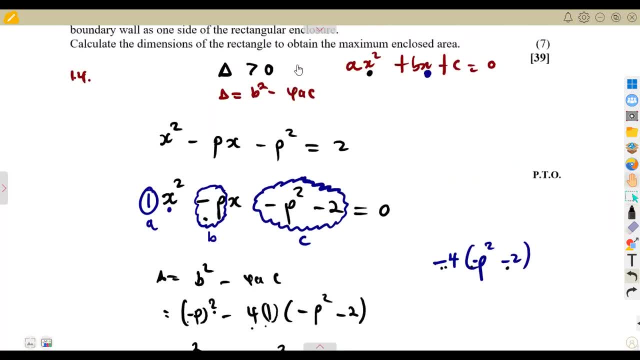 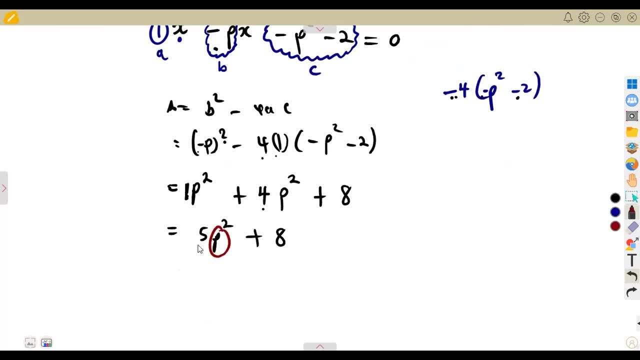 Because we said it must be greater than zero. It must be greater than zero. All right, This is it. Oh, I want You to think of any value of p, of your choice, Any The moment that you square a value, whether it was a negative, whether it was a positive. 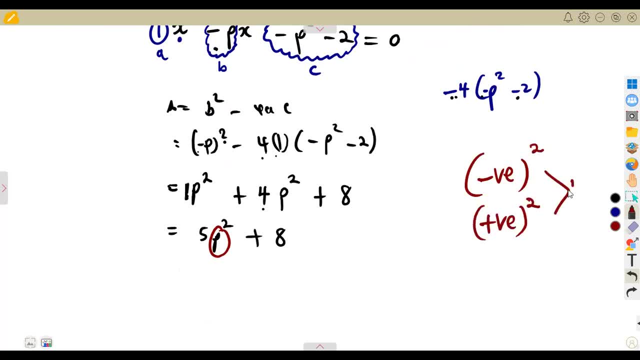 The moment that you square this, it remains, It becomes a positive at the end, Becomes a positive at the end. So five is positive, Eight is positive, P squared is positive. So There is no way, this expression that we are having- there is greater than zero p squared. 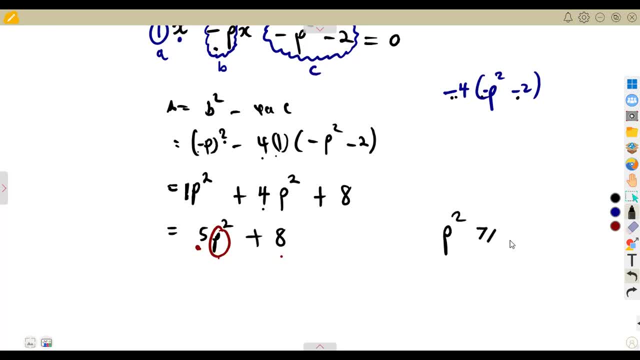 It is a number, that is. It can be great. It can be p. P can be a zero. You square a zero, You get a zero. P can be a one. P can be, So meaning to say, if you square that p, it can be equal to zero. 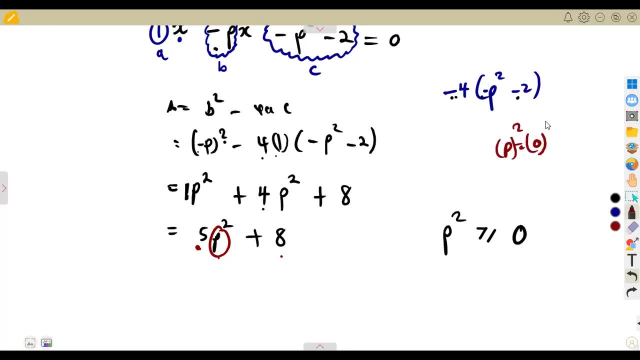 Because if p is equal to zero and you square this, that will be a zero. If you have minus one, you square minus one, It's a positive. If you have a one, you square it's a positive. So meaning to say: whatever p you square, it is going to be something that is greater than or equal to zero. 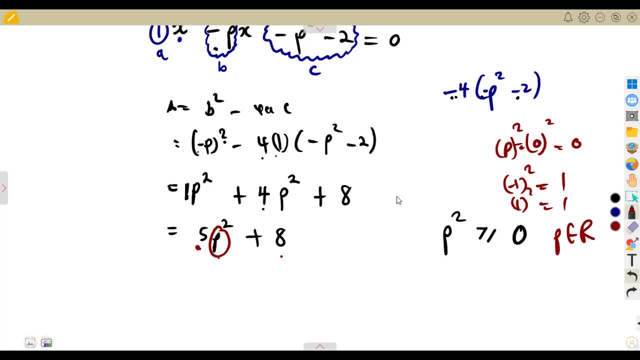 For any p that represents every real number that we talk about. So if it is like that p squared is a positive and you multiply, guys, a positive times, a positive is what It's a positive. So meaning to say, if I multiply five to p squared, what am I going to get? 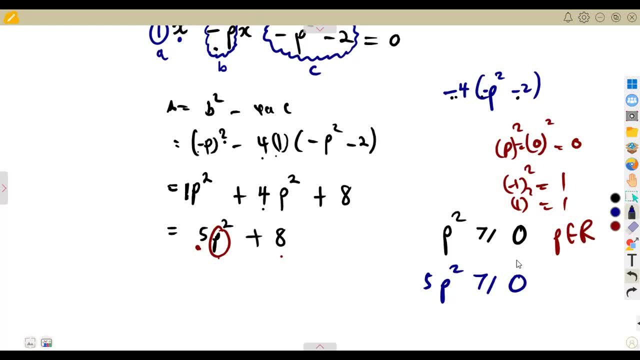 I'm going to also get a positive value Greater than or equal to zero. What if I add a positive to a guys? I add a positive to a positive value. The answer will be positive. So the moment I add this- five p squared plus eight, this one that I'm having here, this whole thing here is going to be what. 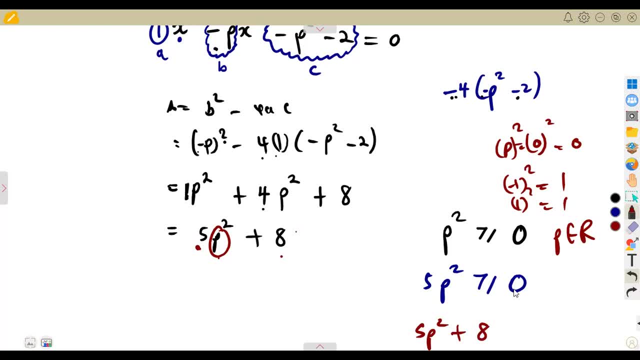 Greater than also five p squared plus eight. Now it won't be greater than or equal to zero, because you are now adding eight. So if it was a zero zero plus eight, it's no longer Greater than or equal to, is just greater than zero. 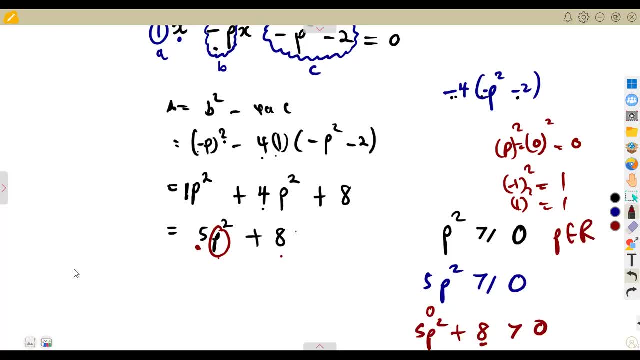 Now take note, because you have added that if you are at zero, you add eight. Are you still at zero? No, you are no longer at zero, So it's no longer equal to zero, but it can be greater than zero. So, as we can see our discriminant, at the end it is something greater than greater than zero. 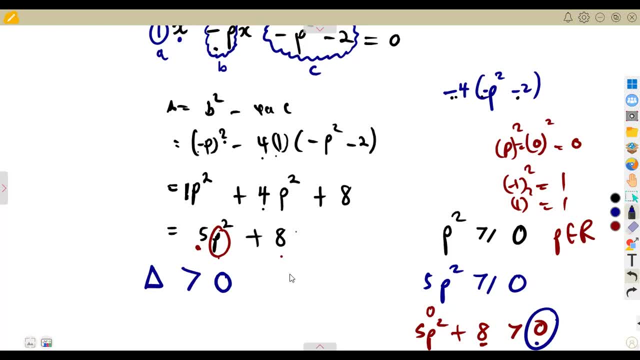 And if it is greater than zero for any p value, which represents a real number. Therefore, what does it? It means? it means that these roots are equal and also these roots are real and unequal. So therefore, the roots Are real. 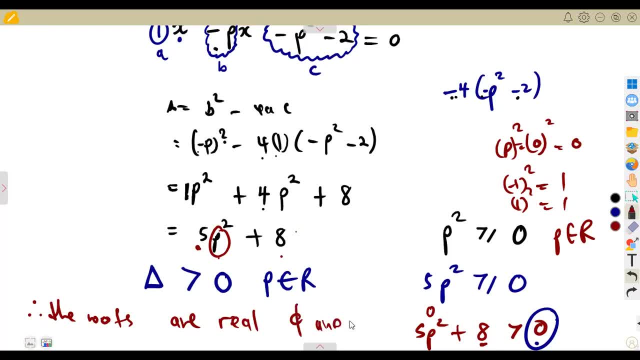 That is the first thing. They are real and unequal. All right, So you need to know the conditions. that makes the roots to be what To be real and unequal on your quadratic Uh equations there, when you are dealing with your quadratic equations, 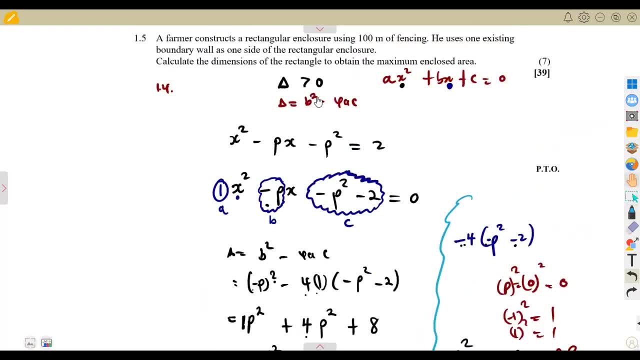 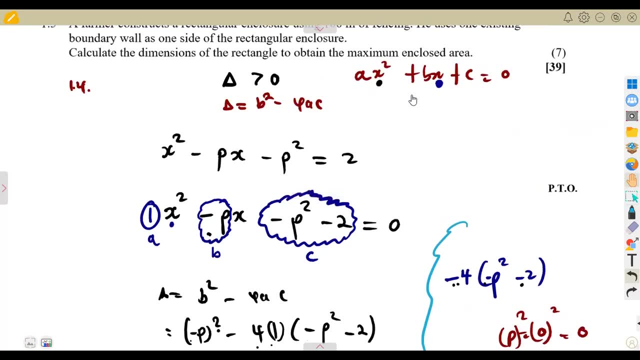 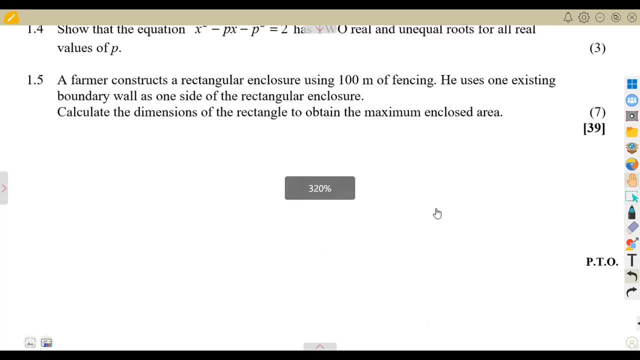 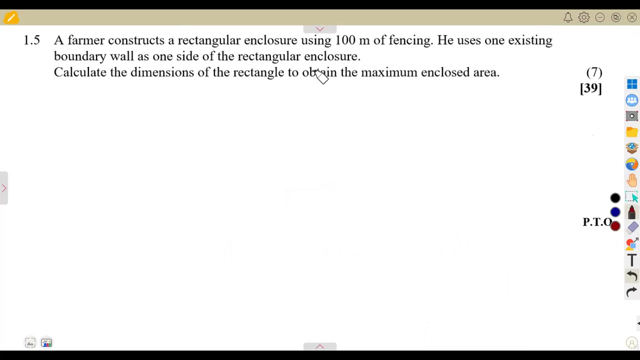 So the format first, of a quadratic equation. we need the format before you talk of the B squared minus four AC. The format is taken from the format. That is the idea there. All right, So on question 1.5, you are given a farmer constructs a rectangle enclosure using 100 millimeter of fencing. 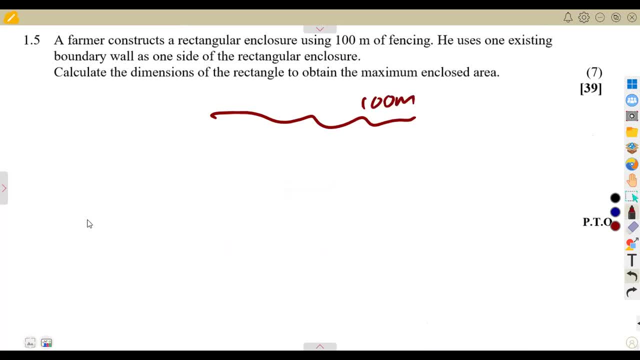 The first one is a rectangle. The fencing that is used, it is 100 meters. He uses one existing boundary wall as one side of the rectangular enclosure, meaning to say, as you are making, uh, as he was making his rectangular farm another part, it was to be covered by a wall. 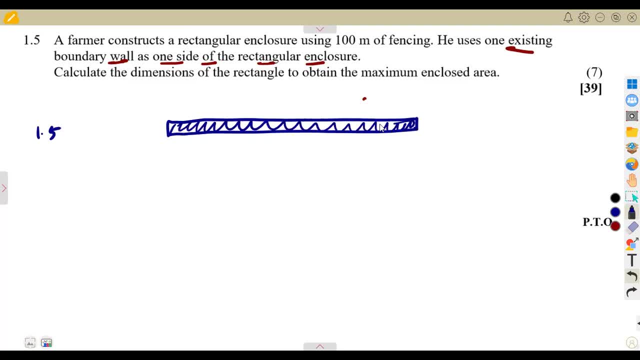 Another part yet to be covered by what? By a wall, not a fence. So the fence Is this one, This is our fence. Remember, it must be a rectangle at the end, But as you are forming a rectangular field, uh, one of this part is covered by a wall. 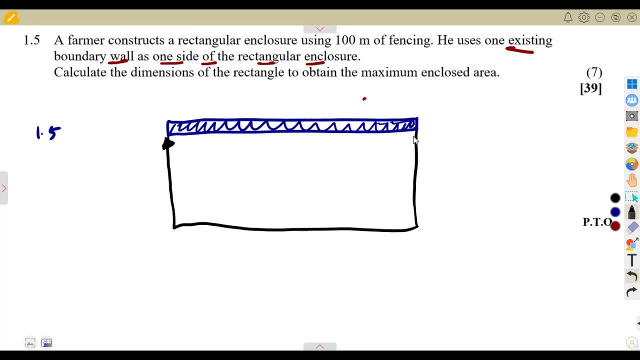 But this is so many to say: this is our, uh, this is our fence. So this fence that we are seeing here, it is 100 meters long. So let's just say, uh, because this is a rectangle, So you can consider the length and breadth. 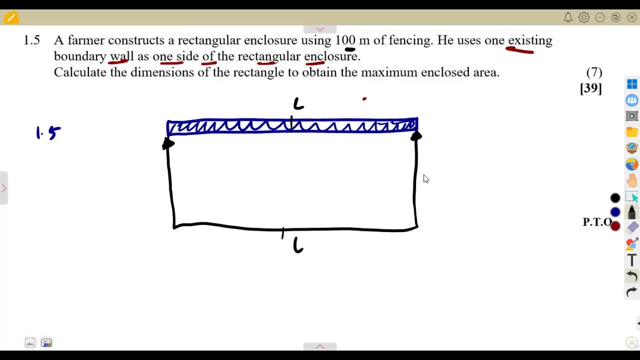 Concept the opposite sides of a rectangle. We know they're equal. That's our length and breadth, or you can consider length and width. So let's say this is what we have. What it means is that if you add this part of this, well, this is your fence. 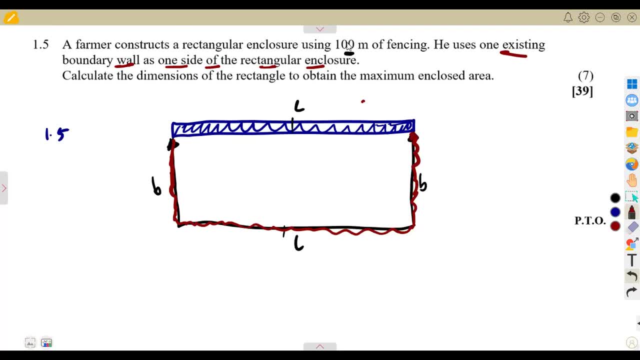 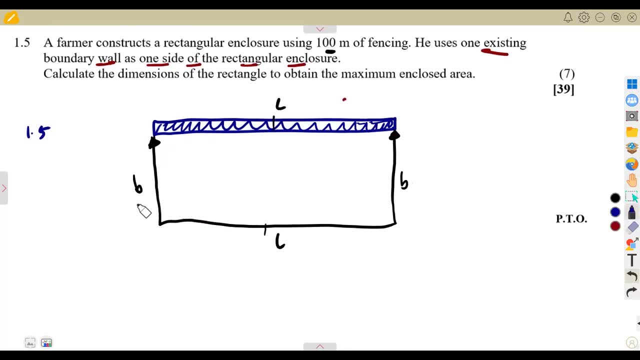 This one. this is the fence. How long is the fence? It is 100 meters, So many to say. if we add where the fence is from, it's from B to L- To this other B, we must get the 100 meters, which is of the length. 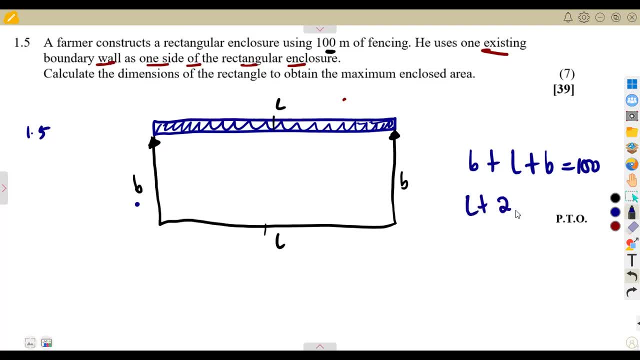 So many to say we are going to have L plus B plus B, That is, 2B is equal to 100.. This is just an equation that you're obtaining from the fence, the way that you are given, and also from the properties of a rectangle. 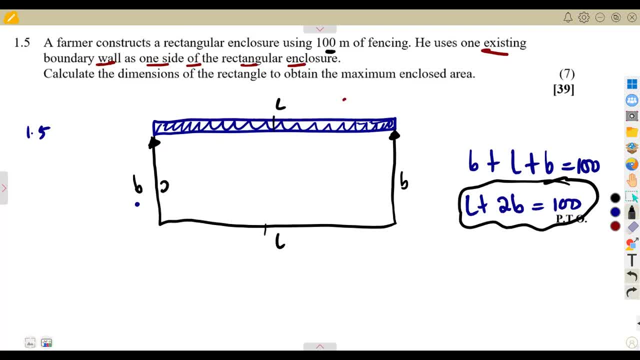 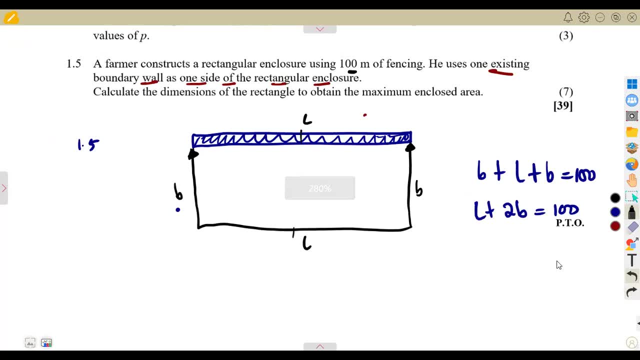 I don't know, maybe used X and Y. It's up to you. So it will be X plus Y plus X. So at the end you have to. You have to form the same equation or a similar equation, All right. 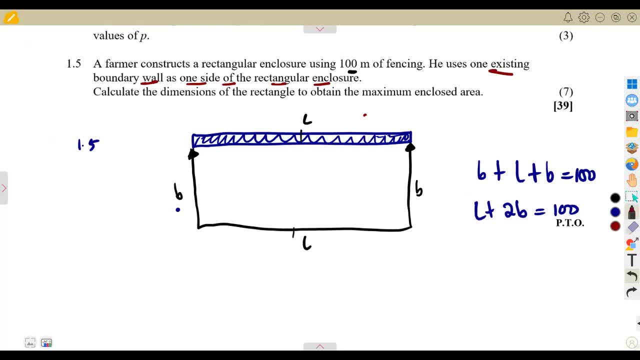 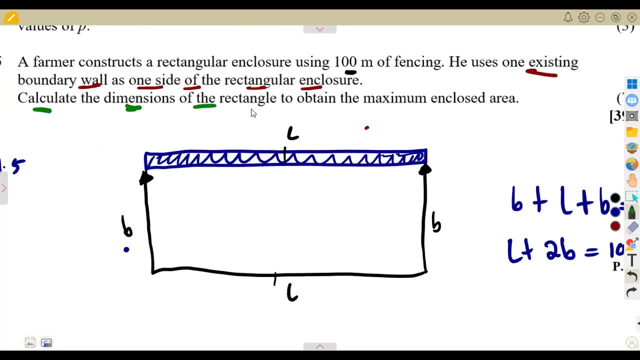 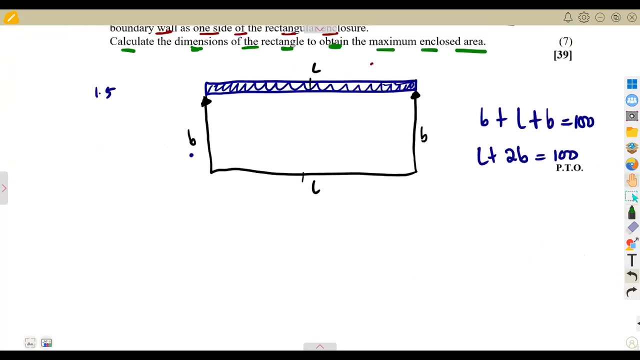 So this is not about our question. I'm just talking about what this statement means. So the question is: calculate the dimensions of the rectangle from this rectangle that we are seeing to obtain maximum enclosed area, Maximum area. So we are talking about the max to obtain. 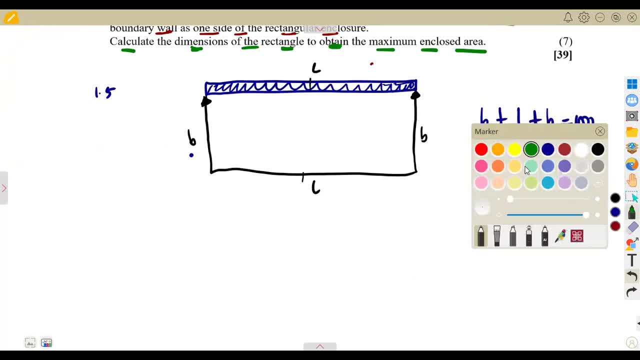 What are the dimensions to obtain the maximum area? So what you need are the dimensions there first, But these dimensions, that gives the maximum area. So how do you answer this type of a question Whenever you hear about maximum area, maximum, surface area, minimum. 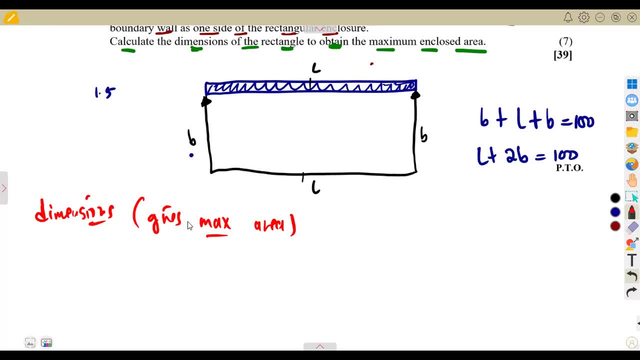 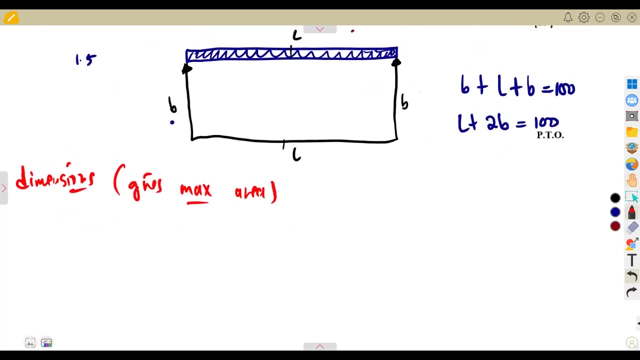 these are maximum and minimum. Minimum values, Maximum and minimum values. If you are to consider this as you continue in your grade 12, we shall talk of the derivatives, where you can use derivatives to determine maximum and minimum values. So, in our syllabus, how do you consider the maximum and minimum value? 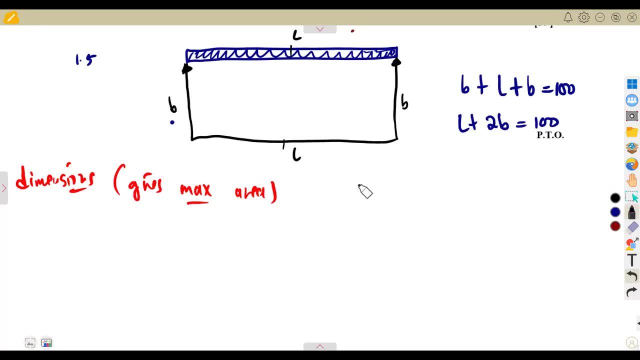 We know that from a quadratic function, if Y is equal to F of X, in the format of AX, X squared plus BX plus C, as long you have a quadratic equation and it is of this nature, at X is equal to minus B over 2A. 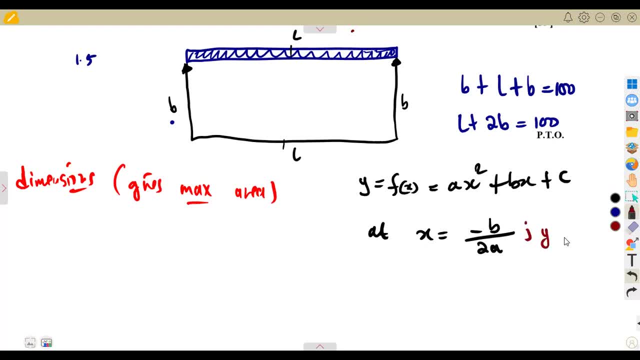 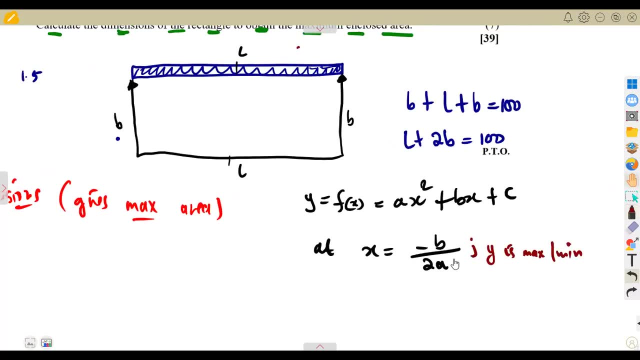 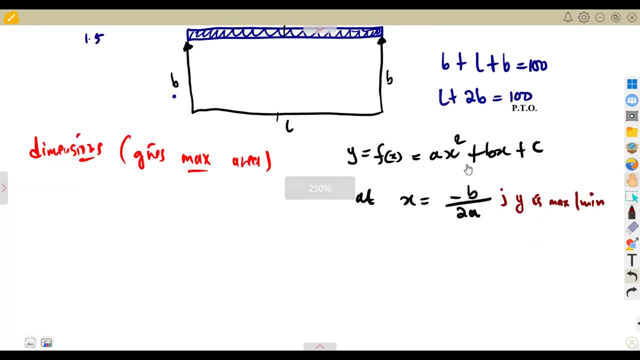 that's Y is. at this value, Y is maximum or minimum. That's it. So, at the maximum or at the minimum, X must be equal to minus B over 2A, as long your equation is in this format. So they are talking about having an area as a maximum. 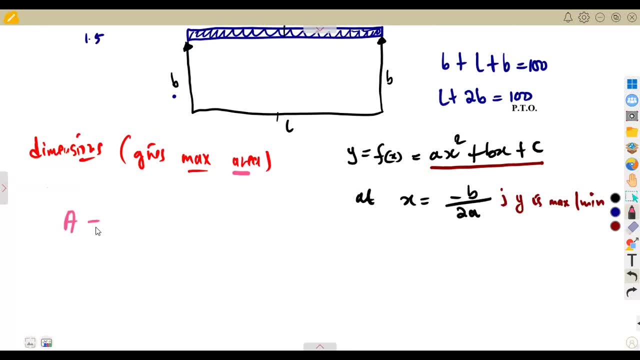 Do we have the expression for area? No, we do not have, So let's find it. We know that the area of a rectangle- because the shape that we are given there is a rectangle- is determined in the term of length times breadth. 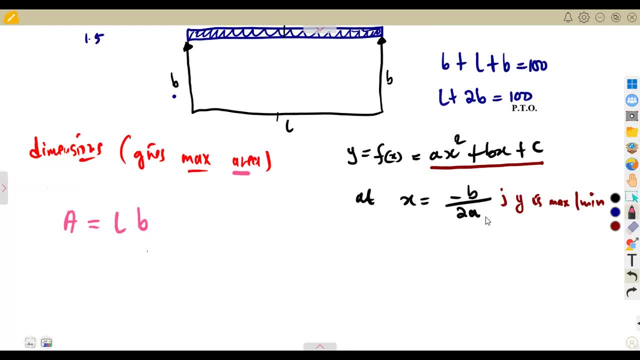 So with this expression, there is nothing that we can do. We can't have minus B over 2A. We must have the same format of a quadratic and also having the same letter. If this is X, let it be X. So how can we have this? 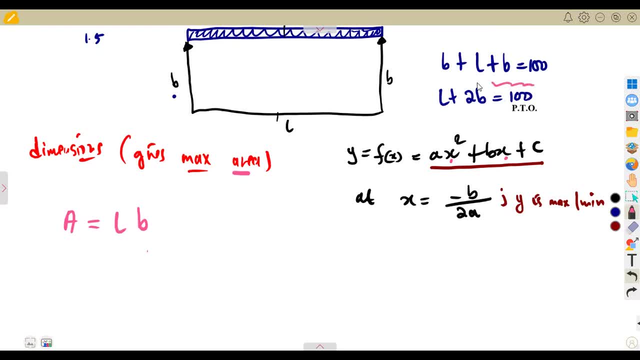 It's: either we can write from this equation of the fence- Remember, the fence is 100 meters. So from that equation that we wrote, it's: either we are going to make L the subject or you are going to make B the subject. 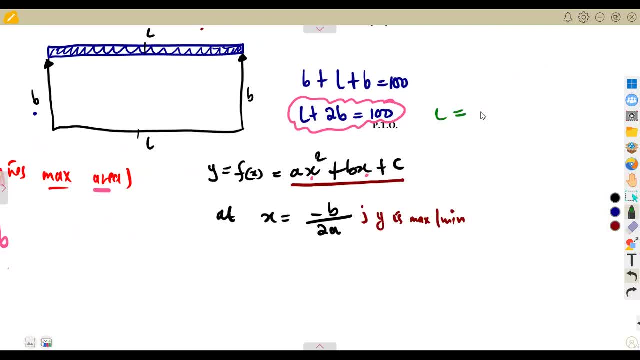 So let me make- I'm going to make- L the subject from here. It means L is equal to 100 minus 2B. It's easier for us to have L as the subject. So if L is equal to 100 minus 2B, 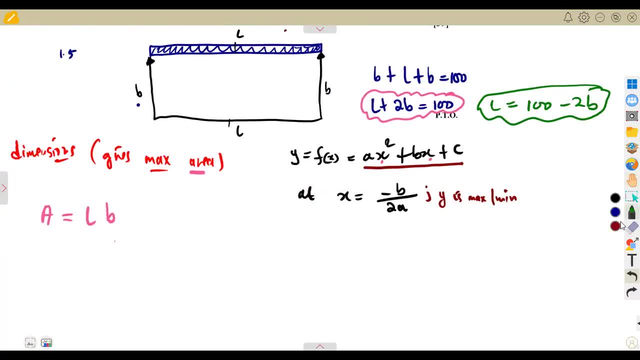 let us substitute it back here. This is what it means. It means this area can be given or can be written as the area is length, where our length is 100 minus 2B times the breadth. We're not going to change the breadth. 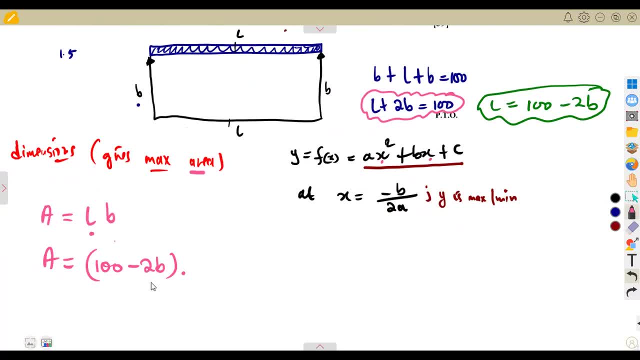 because you want to write the length, You want to write area in terms of the same variable. Is it B or is it L? So B is not going to change. We change the L to be a B, So B remains as it is. 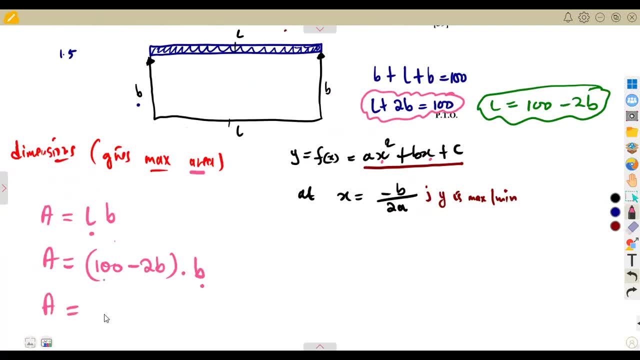 As you can see, these are now brackets. You can expand the brackets times B, That is, 100B times B. here This will be minus 2B squared. Having a closer look, we are seeing exactly the format of a quadratic equation. 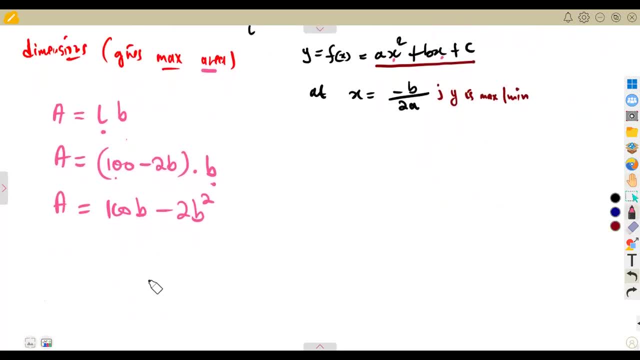 in the form of AX squared plus BX plus C. So it means It means our area can be given as minus 2B, squared, taking the highest power into consideration, followed by X, which is followed by what? By 100B, then followed by the constant. 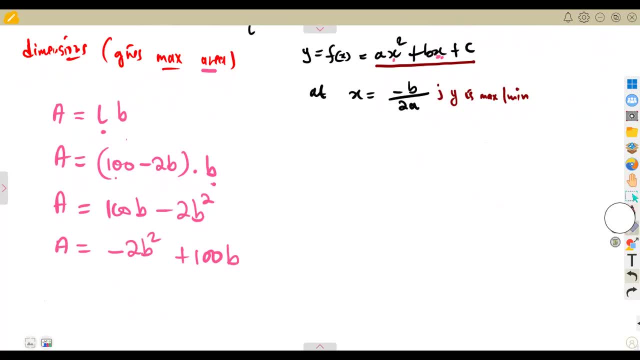 And in this case, the constant, if not given, it means that's a zero. So this is it, Exactly the format. So at this point, at this, at this, for a maximum value, for a maximum for a 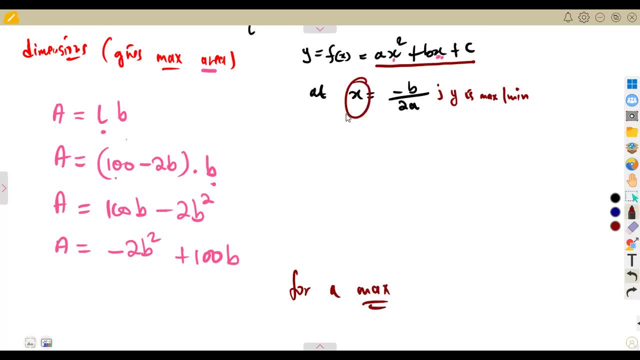 Not to say X is our maximum. no, Y is the one that will be maximum or minimum. So we are saying, for any maximum value, X at a condition was supposed to be minus B over 2A. from this formality that we have, 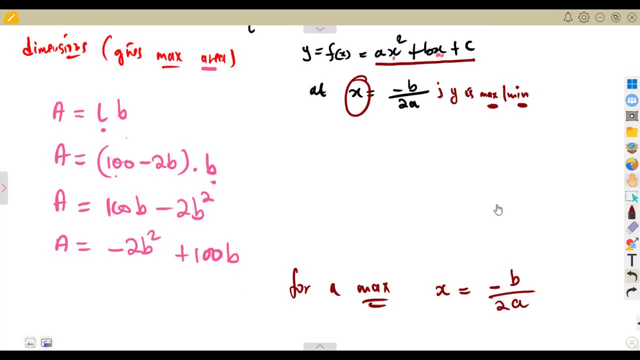 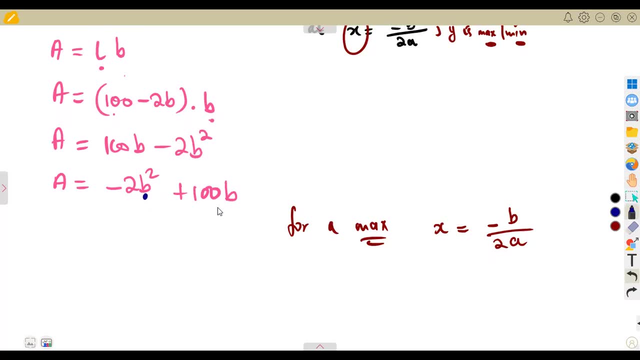 Our X, So we are no longer having it as our X in this case, because- So just don't confuse guys- It's no longer X, This is now a B, So meaning to say, at our maximum value, our B. as of this equation. 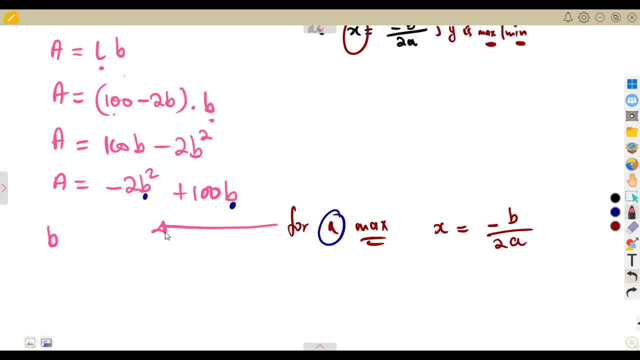 B at maximum value. for maximum value now, B is equal to what? B is equal to minus B over 2A of the? This one is of the formula when we are writing this in the form of AX squared plus BX plus C. 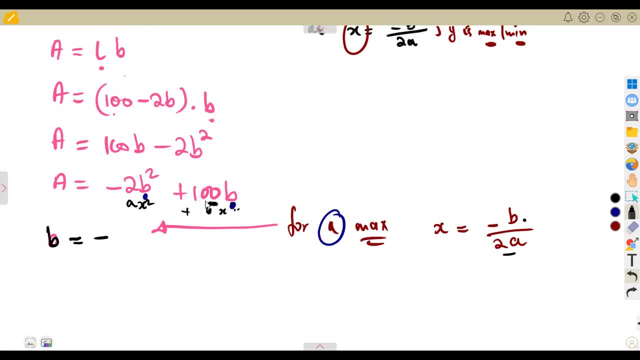 So our B, there is the coefficient of X, which is the coefficient of B, which is this one 100.. So it's going to be minus 100 over 2 times A. A is the one that affects what B squared from X squared. 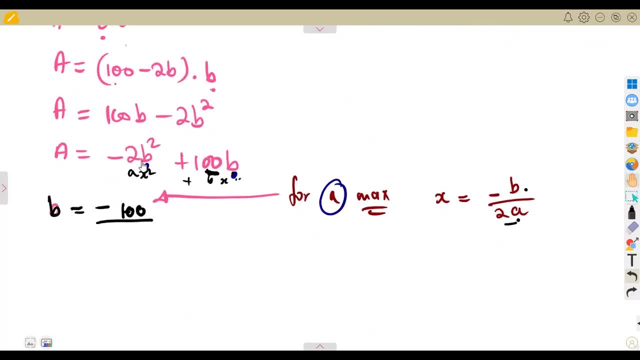 A is the coefficient of what Of X squared, And what affects our square is minus 2.. So it's 2 into minus 2.. So this will be the value of B at the maximum value. For a maximum value, this must be equal. 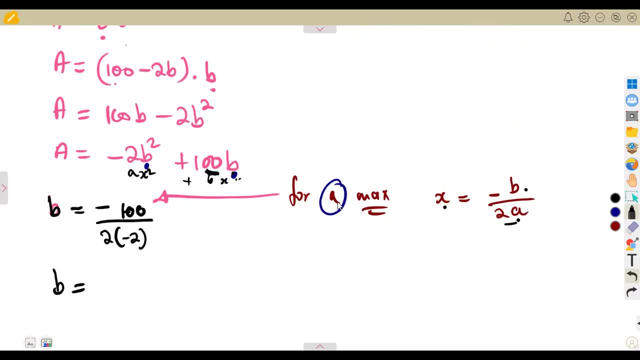 Minus B over 2A. And what represents that X? It's no longer X, It's now a B. So B is equal to minus 100 over 2 times minus 2 at the maximum value. So it means our B at the end was going to be 25. 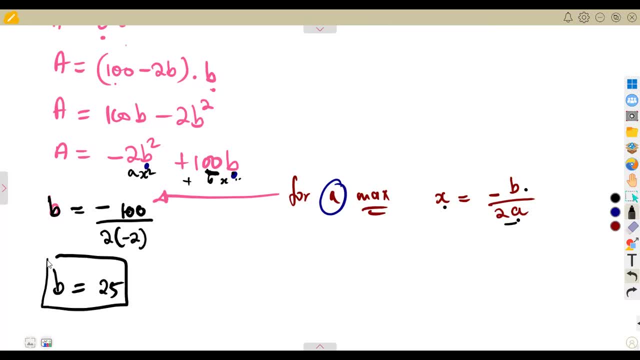 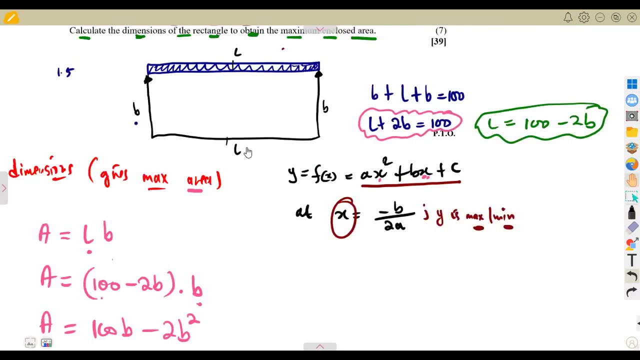 at the maximum value. So if B is 25 at the maximum value, what about the value of A? I mean, what about the value of the length? B is the breadth. What about the length? Remember I said the length is 100 minus 2B. 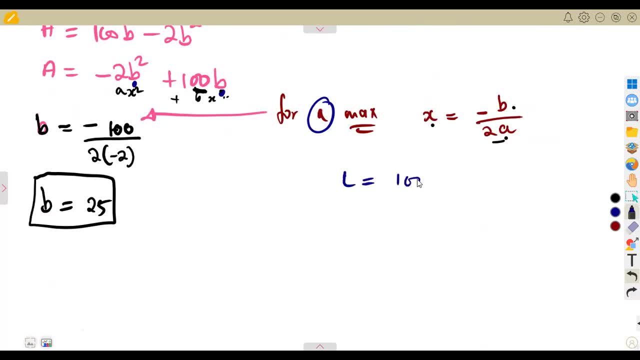 So it means we can Determine our length from there, because this is 100 minus 2 times the breadth. So that is 100 minus 2 times the breadth that we calculated, which is 25.. So our length at the end was going to be 100 minus 50,. 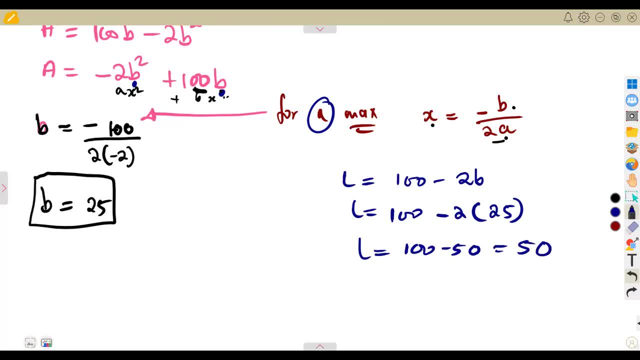 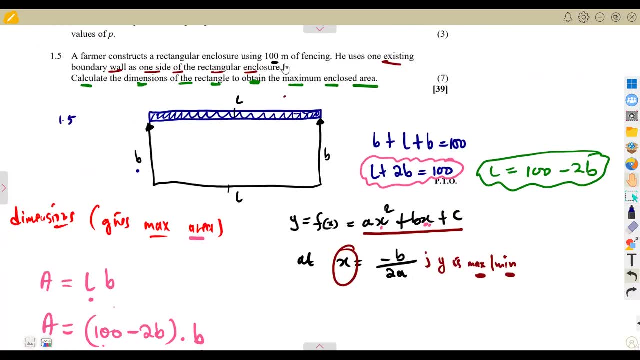 which is going to be 50.. So that is it. These are the dimensions that will give us the maximum area. So, if we take a closer look, the other units that we're given, the units of the fence, it's meters- 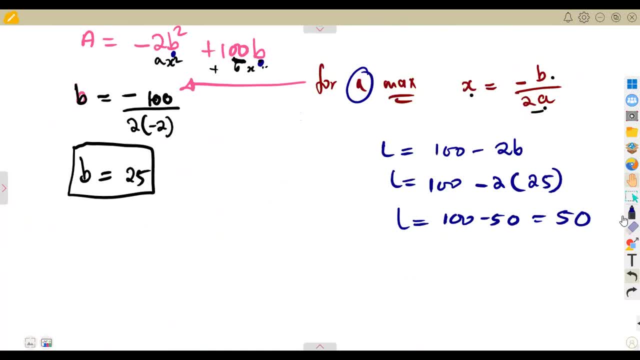 So it means this: B, this length, breadth, are also in meters. Our breadth is going to be 25.. Our length is going to be 50 meters. For this value, our area must be maximum, Or you can use completing of the square method. 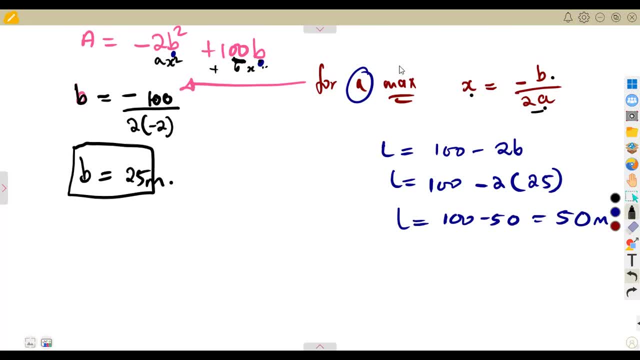 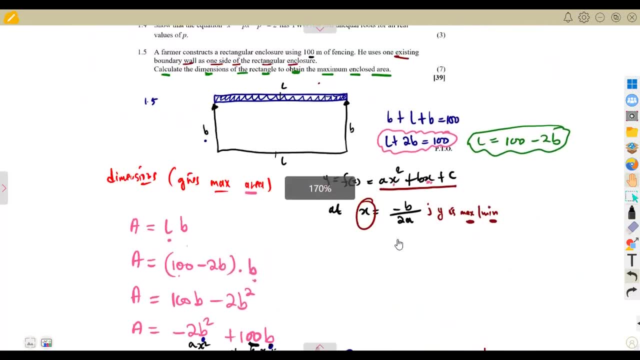 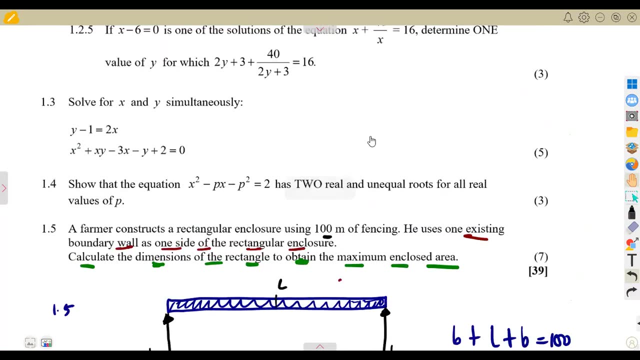 which is another way out to your simplification. If you want to use that, you can also work with your completing of the square method. So that was the first part of our question, which is question number one. We're going to consider what follows next. 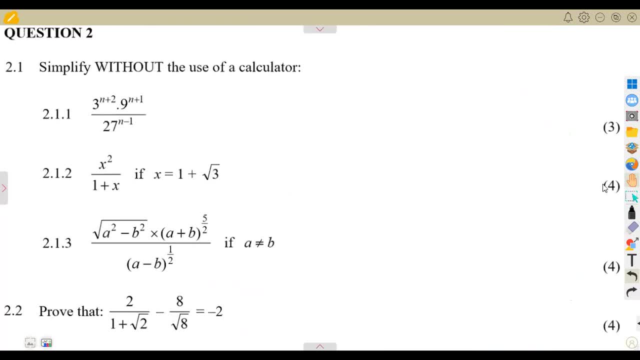 on this question paper: June 2023, paper two. All right, that's a nice question paper actually that we are having in hand at this time. So what is it that we are given? Simplify without the use of a calculator? 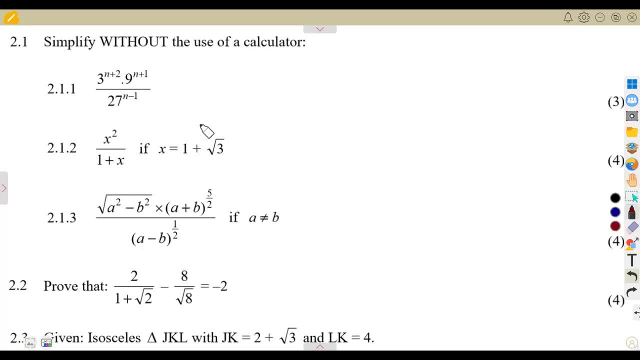 Meaning to say a calculator is not needed in this simplification. You are not supposed to have a calculator. Yes, you can just use for your verifications, which is fine. 2.11, we are given, that is. let us just have it here. 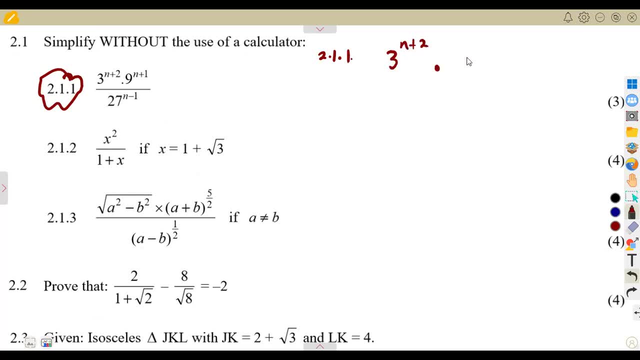 Three to the exponent of n plus two, multiplied to nine to the exponent of n plus one, This here is over 27 to the exponent of n minus one. So we're given 2.11, that is, let us just have it here. 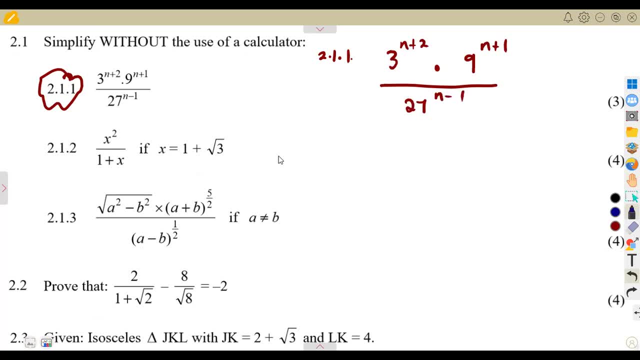 That's one, that's three marks. So if you had to consider, you were seeing that I said when we are dealing with our exponent, remember The best way to work an exponent is to work it as the simplest number And the simplest number. 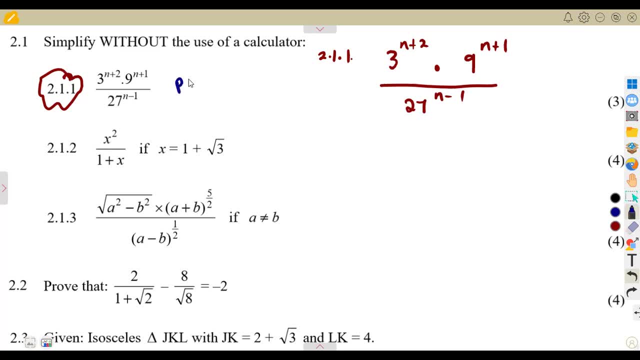 we are simply talking of prime numbers. We are simply talking of prime numbers. These are the simplest numbers that you think of when working with your exponents. If your numbers are in simplest form, everything will work smoothly. Okay, what am I trying to say? 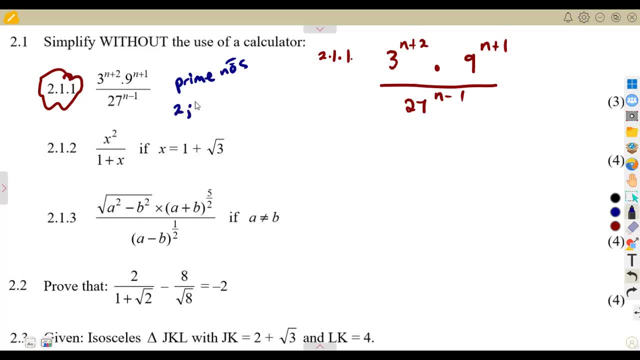 Prime numbers. we are talking about numbers such as two. Okay, when you divide by, I mean it's just divisible by one and itself, Divisible, exactly divisible by one and itself. So examples: we've got two, we've got three. 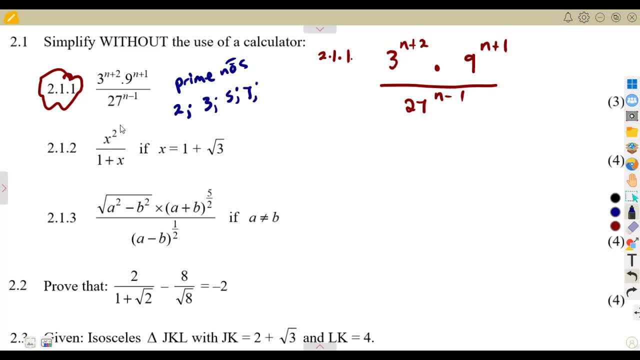 all right, we've got five, we've got seven. All these are prime numbers. So you are going to think of these numbers to say, all right, I'm given this expression. So three is already a prime number. It's already in simplest form. 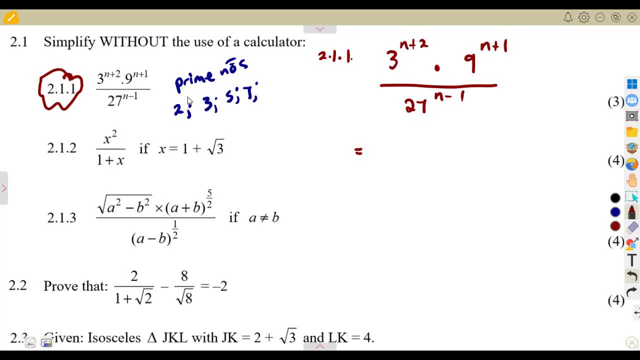 Remember I want to write these numbers in or in its simplest form. So already, three is in simplest form. I'm just going to rewrite: as it is Times is nine a prime number? No, So how can I rewrite the nine? 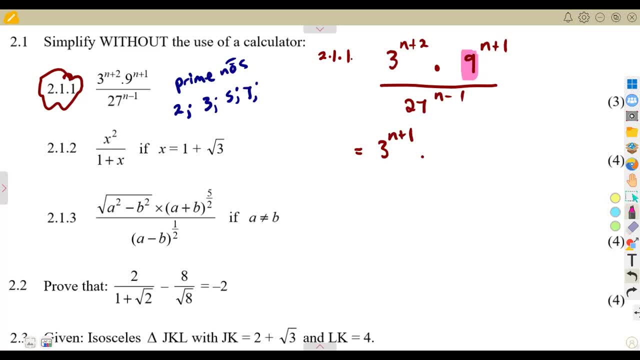 Okay to be a prime number, but remains, it must remain, as a nine, as it is. So we think of a three. Three to the exponent of two gives us a nine. So meaning to say, in place of nine, we've got three to the exponent of two, multiplied to n plus one. 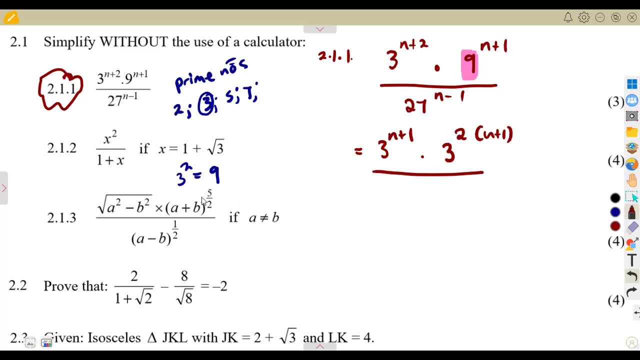 27 again is not a prime number. There are so many factors there. but it can be written again in the best of three as three to the exponent of three into n minus one. So you can also use your calculator to check if you are not sure about your numbers. 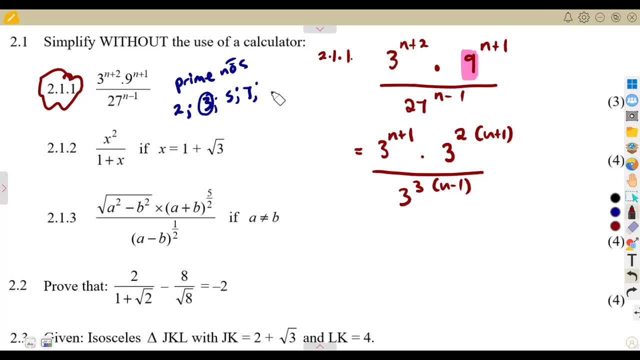 Just try your numbers: three to the exponent of one, three to the exponent of two, and so on. This is how you just try your numbers. You just have to make sure you work with each part that you are given until you get that number. 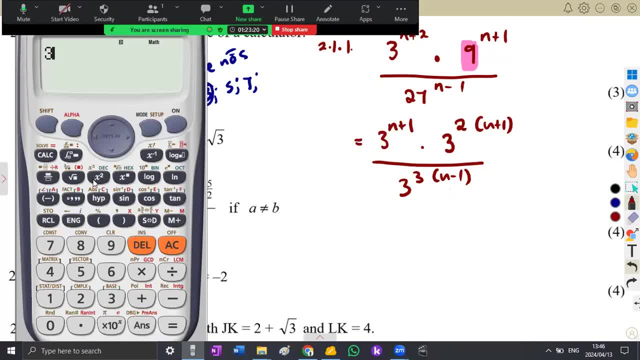 At least you have an idea that I am in the best of three. So you can try. three to the exponent of two, That's a nine. So I know that okay to have a nine is. three to the exponent of two. three to the exponent of a three. 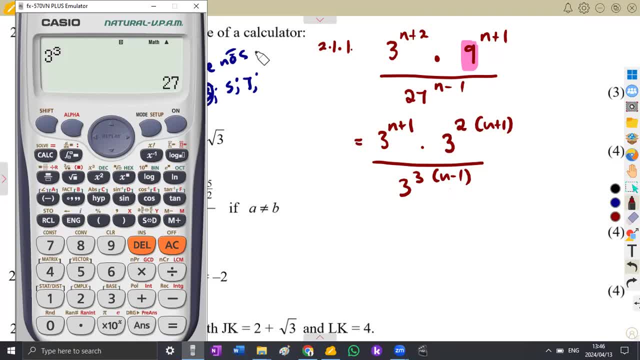 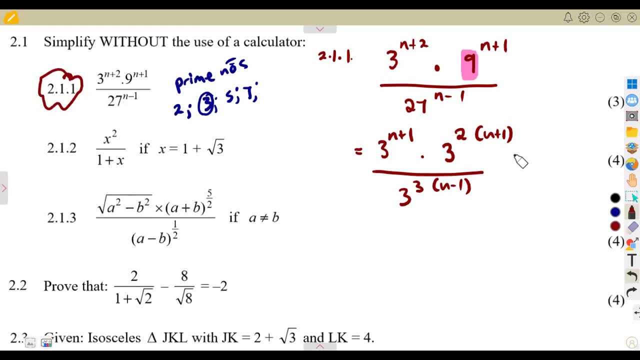 You can use your calculator. No one is going to actually understand what you're doing there. All right, this is it. We know that an exponent, an exponent, can be simplified together, Exponent to exponent. If I am given, this is x, maybe. 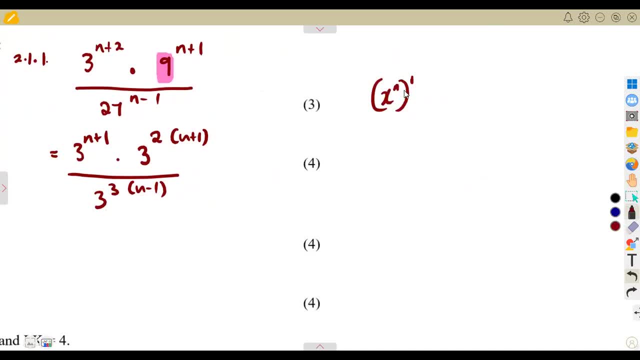 whatever that I'm given raised to a certain exponent And also there is another exponent, You can simply multiply the exponents together in that situation, So meaning to say three to the exponent of n plus one, there's nothing. also, just leave it like that. 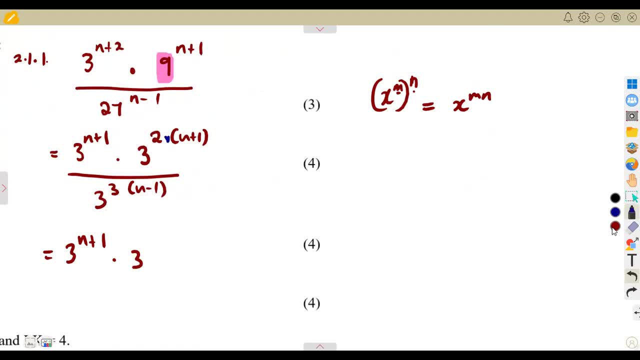 Three to the exponent. there is an exponent, an exponent. So multiply by two, distribute by two times two, That'll be two n times two here, That'll be a positive two. Okay, the same thing. three, distribute in this bracket: 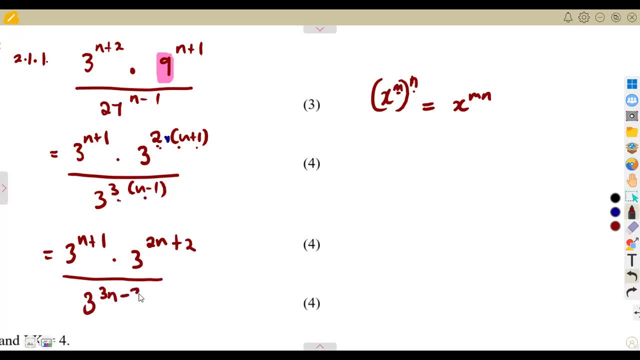 So it's an exponent of three n, three times minus one, which is a minus three. So now that we have got the bases, which are the same if we check on the numerator, you can consider to say that this is the best of three. 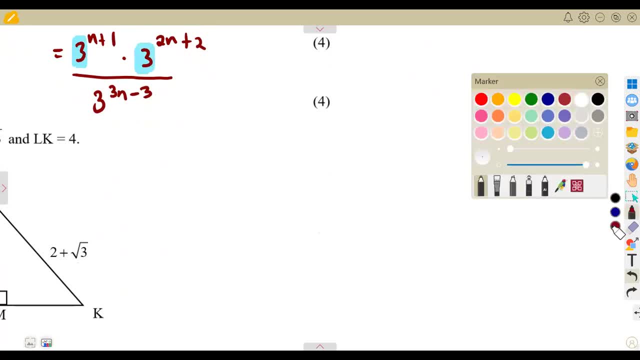 This is the best of three. But what is happening? You are multiplying. the best is that are the same. So if x is being raised to the exponent of m and being raised to the exponent of n being multiplied, we add the exponents. 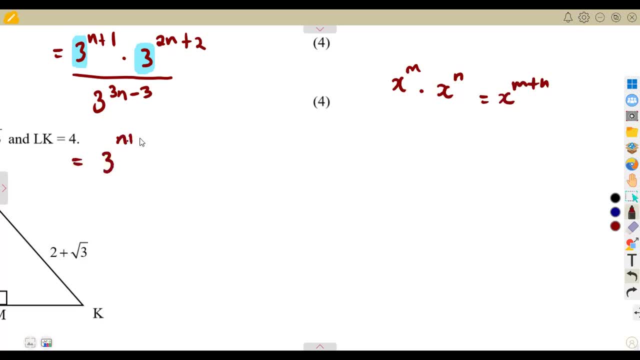 So meaning to say this was going to give us three to the exponent of n, plus one we add. So when you are adding, don't worry about the brackets. all right, It does not affect anything. So you can just write: plus two, n plus a two. 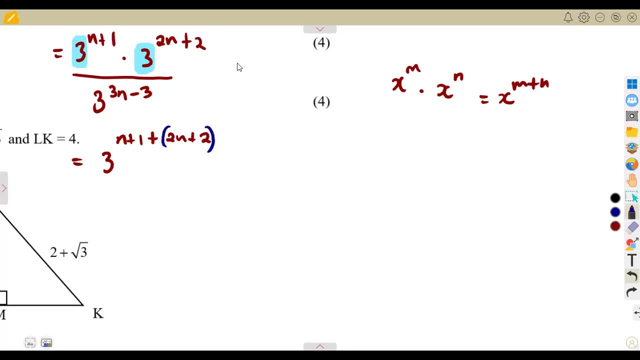 But in actual sense you were supposed to have a bracket there. But, like I said, addition does not affect anything. Checking again in the denominator, there is also a three in the base And this time we are dividing. all right, We are dividing everything that happened. 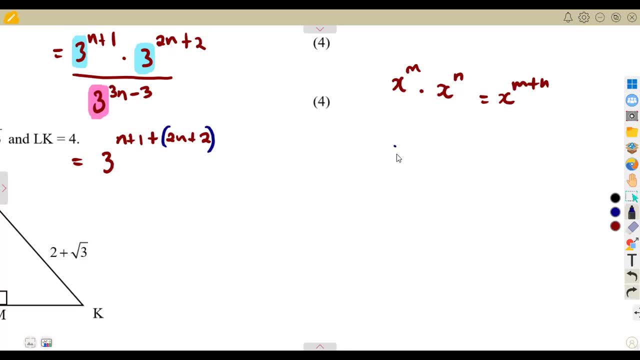 There is a division. So what is going to happen? if you are dividing x to the exponent of m, this time being divided to x to the exponent of n, you are going to subtract the exponents, So meaning you are going to subtract n. 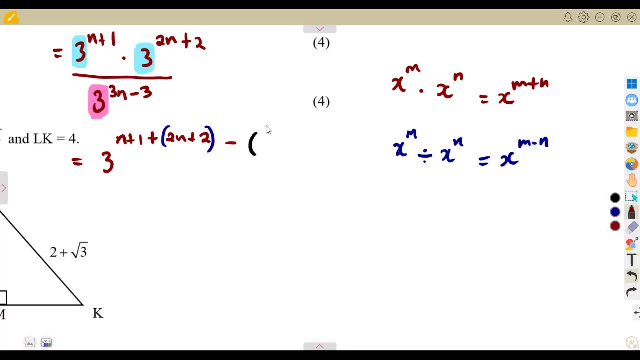 For a subtraction: always open the bracket because the negative it affects everything. So for you not to have a confusion to say where am I going to open a bracket Or where am I not going to open a bracket, Just whenever you are working. 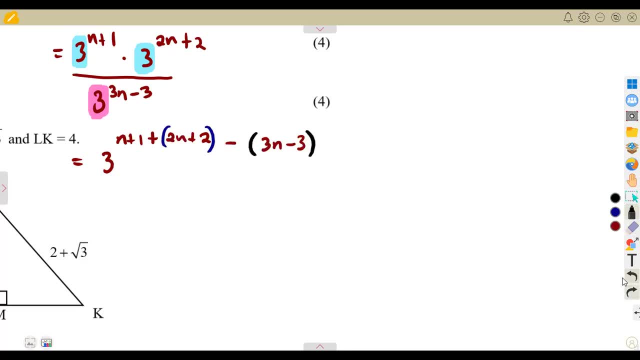 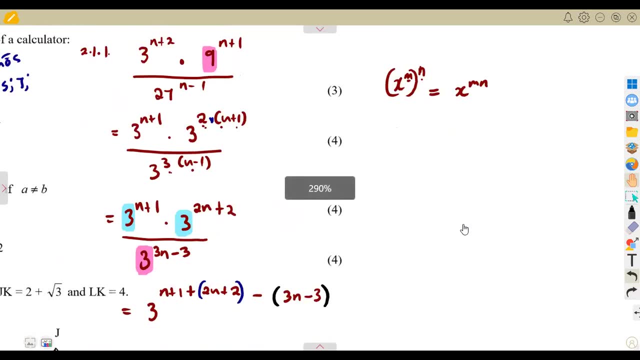 with an algebraic expression. open a bracket in simplification so that you won't make any mistakes. So this is where we are. We could have simplifications. we could have simplified the numerator on its own. We get our answer, then we move on to the denominator. 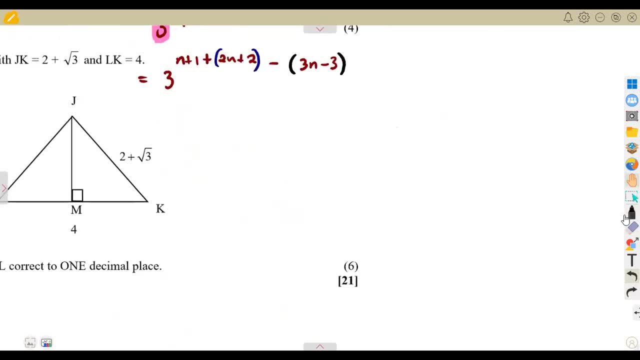 It's another way You could have done that, But you can also simplify at once. So, maintaining the same base of three, this will be okay. let's just expand here. So this will be n plus one, That's a plus one times two n. 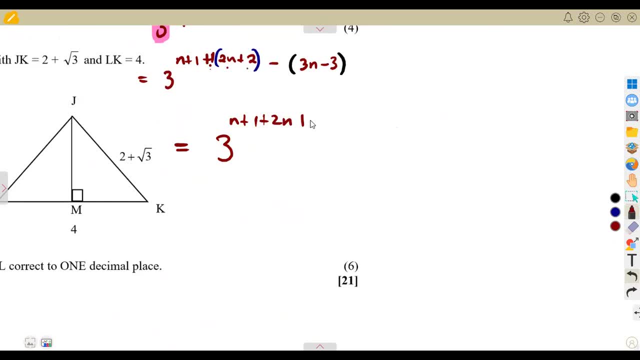 as you can see, that would just remain, as it is Plus one and plus two, that's a plus two. But if you check on the negative, this is a negative one. So if you distribute this by negative one, negative one times three n. 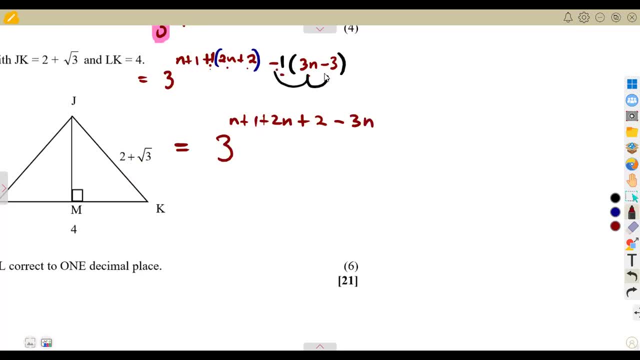 that's minus three. n. As you can see the negative changes, negative. negative, that's a positive three. So we are going to collect the terms together of: n. This is one, n, all right, plus two n, You move on. 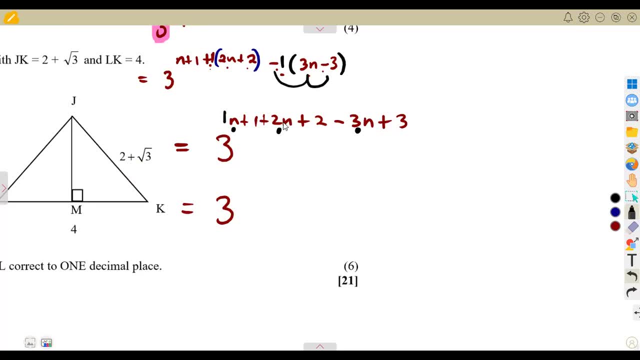 there's a plus two, n minus three n. So one plus two, that's a three. three minus three, that's a zero there. So you're going to remain with a zero. You move on to the numbers. This is one plus two. 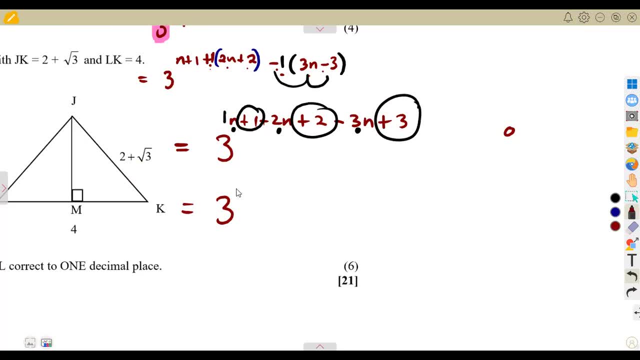 which is three. Three plus three, which is a six. So that's three to the exponent of a six. All right, guys, this is what we are going to have at the end. All right, There was a two there. There was a two. 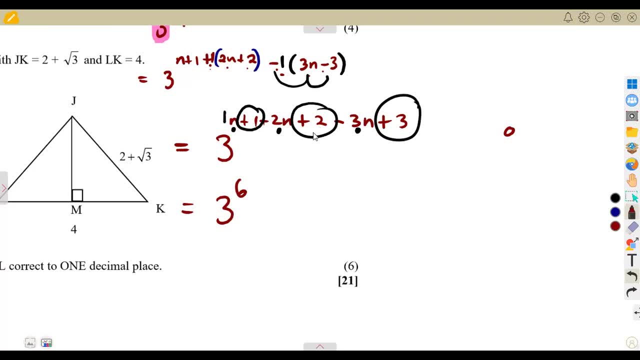 All right, this is one plus two, which is a three. Okay, then, three plus a three, that is going to be a six. All right, guys, in my preparation, you see, I got something else, So I just want to check here. 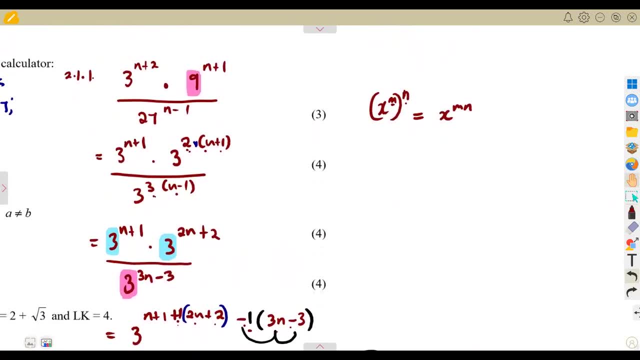 what actually transpired. This transpired here. It transpired here here. on this one: This is supposed to be a positive two there. a two there. We are still having a two. Just correct this, guys. So that's a two here. 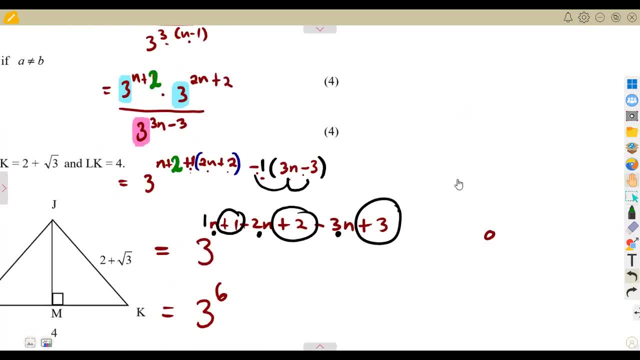 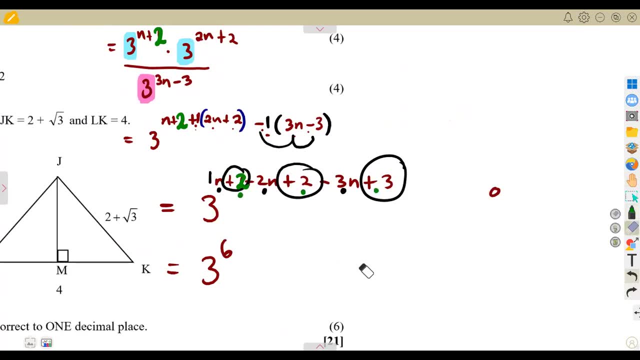 That's a two here, All right. so my preparation actually tells me something. That's a two here, All right. so two plus there's two plus a three. That was going to be a seven, not a six, So let's correct this one. 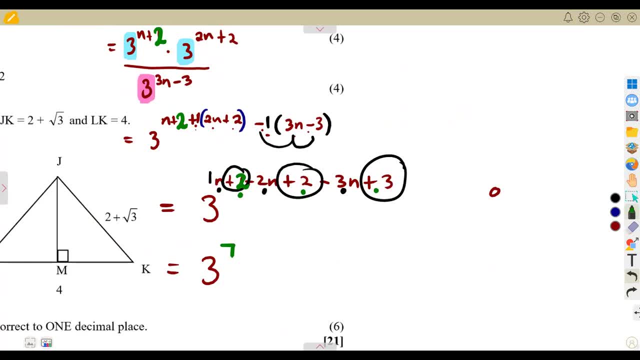 That's a seven, All right. So, since the calculator is not needed, don't waste your time trying to multiply three. There are so many numbers. Just leave it like that. All right, just leave it as it is, You are done. 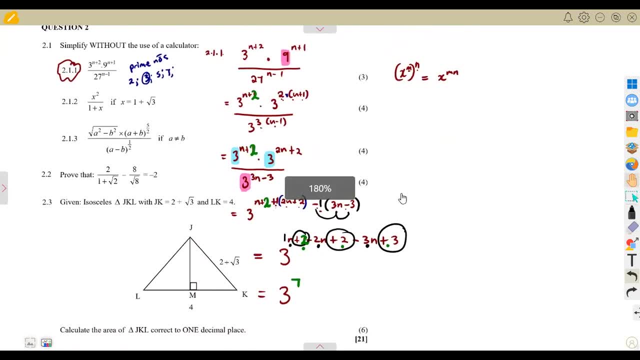 So this is all you're supposed to do. So these are some of the errors that you are supposed to get rid in exam. Try to simplify properly your calculations. You'll see that you won't even go wrong. All right, Two point one, two, four marks. 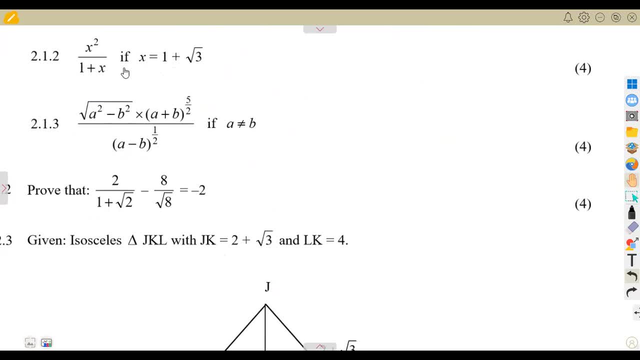 It is given that x squared plus one over x. Simplify this. if x is equal to this, All right, let's. let's see what we are given there. This is a two point one. two. We are given a certain expression: x squared over one plus x. 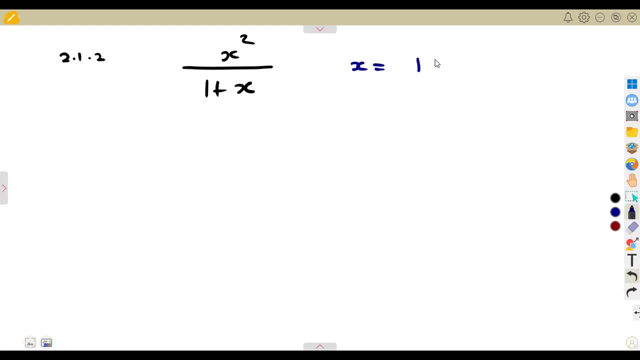 So we are supposed to simplify this, given that x is equal to one plus the square root of three. So these are just simply said. we are back to those sense that we talked about before, that this whole expression that we are given of x, squared plus one over x, is equal to, in place of x. 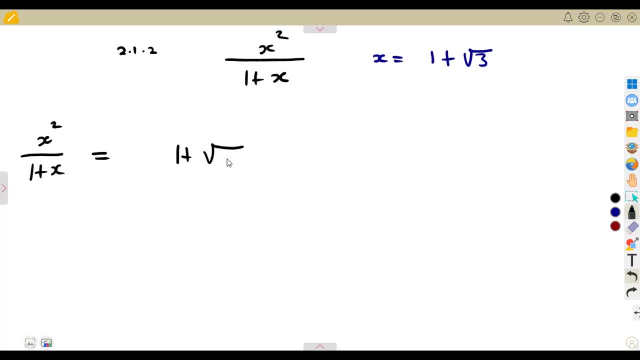 We are going to substitute what represents x, which is one plus the square root of three squared, And this is over one plus x. Our x is Given as one plus the square root of three. So, like I said, if you're ever dealing with an expression, 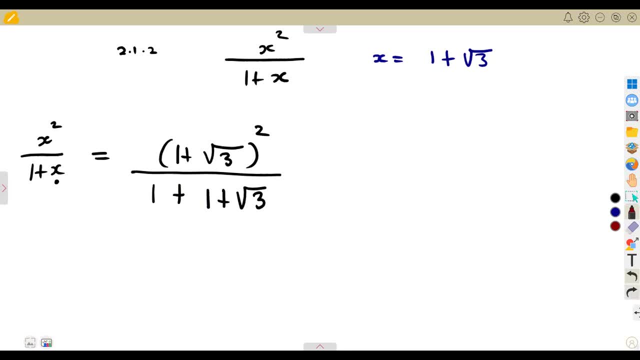 one plus just open a bracket. but looking at the plus does not affect anything, So you can even ignore that. So these are said. as we have got laws that govern these sets, we are supposed to make sure we maintain those laws. A square simply means you are expanding the two brackets. 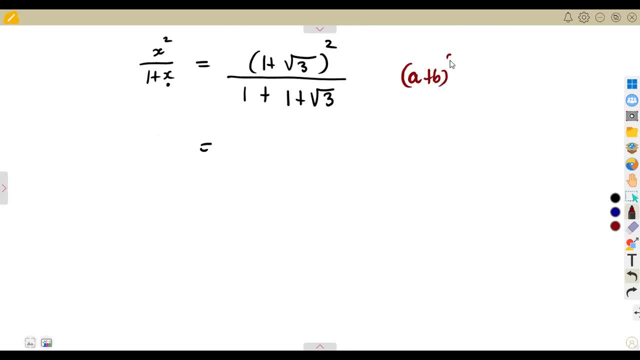 or you can use the concept of a plus b squared, which is equal to a squared plus two, a, b. Remember your identity from grade 10 plus b squared. What does it mean is that we've got a square, a and b. That's first and last time. first, last time. 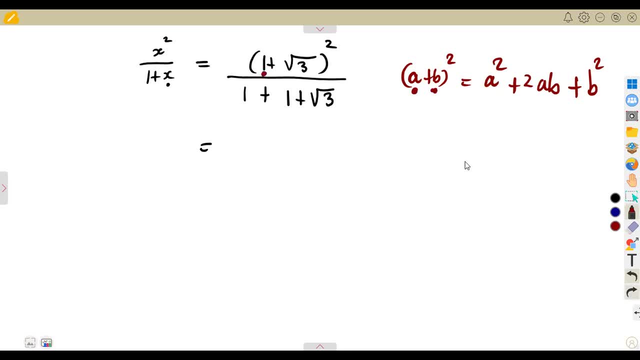 So this is your first time, So it's going to be first squared, which is one squared and one squared. That is simply a, one plus two a, b, That is two times our a, which is the first time, which is one b. 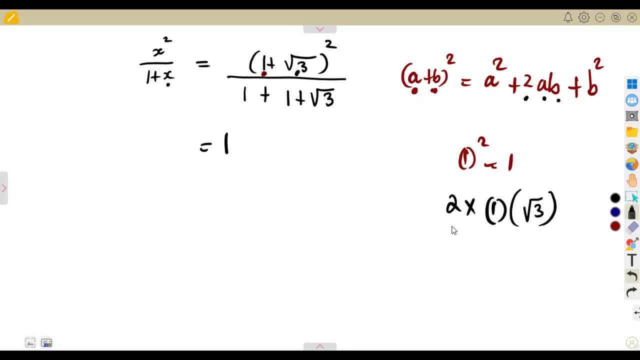 which is the second or the Last term, which is the square root of three. So two times, one times, the square root of three was going to give us two square root of three. Then we move on to the last part, which represents b squared. 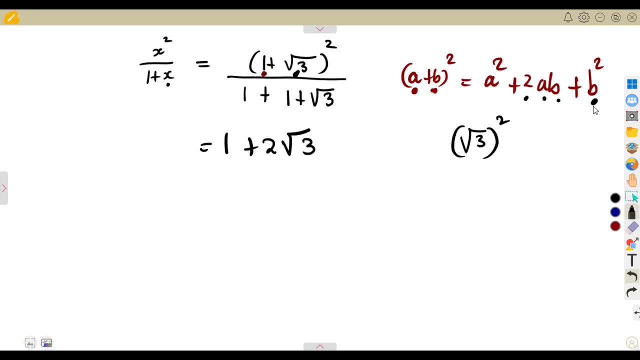 B is the square root of three and we've got the square root of three squared, That is b squared. If you do not know this, you can just use your calculator. No one is going to know that you've used a calculator there. 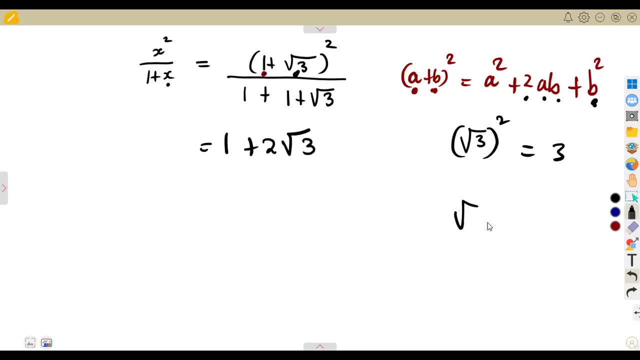 The square root of three squared is equal to three. The square root of three times the square root of three, That is, from the law, square root of a times the square root of a, we obtain a. or you can multiply the numbers three times three, that is nine. and the square root of 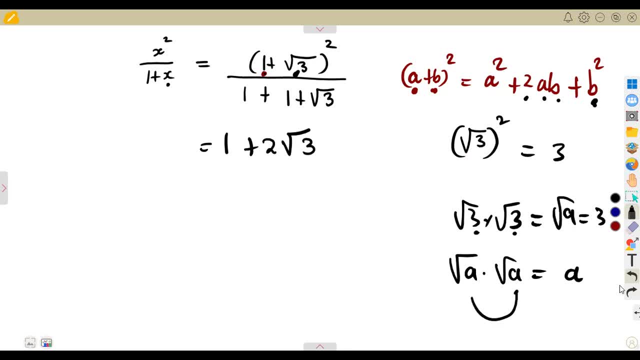 nine is a three or this law states that if you're multiplying the numbers that are the same, as long you're multiplying the numbers that are are the same. the numbers are the same under the square root, right? you obtain that number under the square root, so meaning to say the b squared. 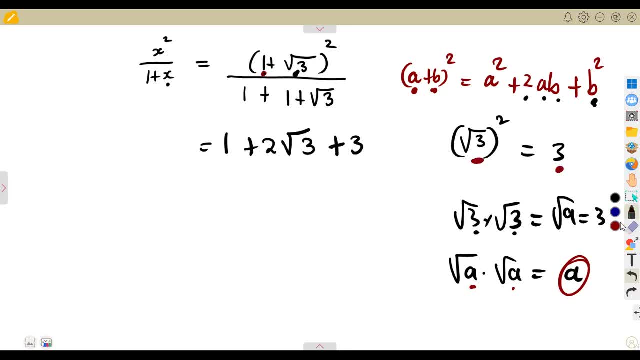 which is the square root of three squared, was going to give us a three at the end or just expand your brackets. if you do not understand this part of the a plus b squared, these are your brackets: uh, one plus the square root of three into the bracket of one plus the square root of three. 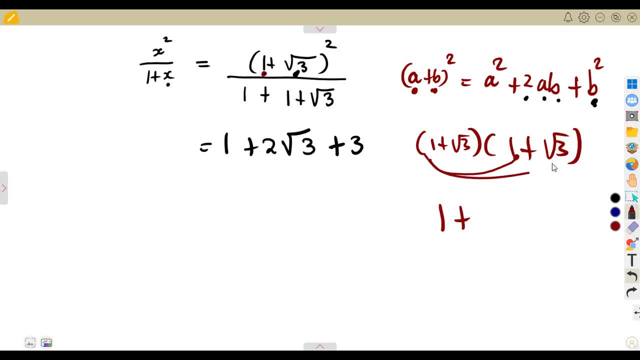 one times one, that is going to be one plus one times the square root of three, which is the square root of three. the square root of three times one, that is the square root of three, the square root of three times the square root of three, which is our three, or the square root of nine, which will 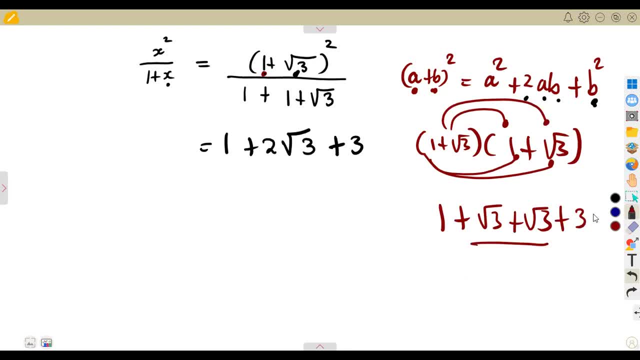 give us a three. you simplify this. there's a same. you simplify this: there's a same, and you simplify this. there's a same and you simplify this. there's As there's a 1 and there's a 1, so 1 plus 1 is going to be 2.. 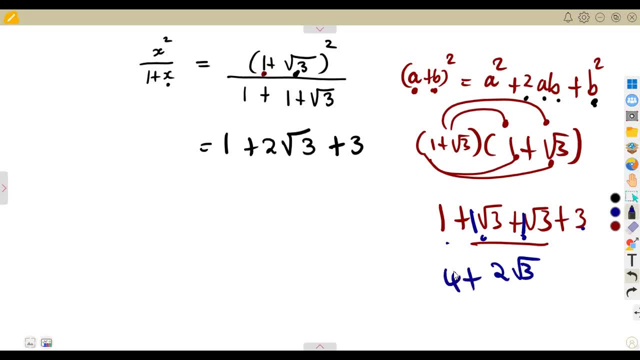 Square root of 3,, 1 plus 1,, that will be a 4.. So that's it. You can also expand your brackets. In this case you can use this concept, But at the end we can see that these numbers can be simplified together. 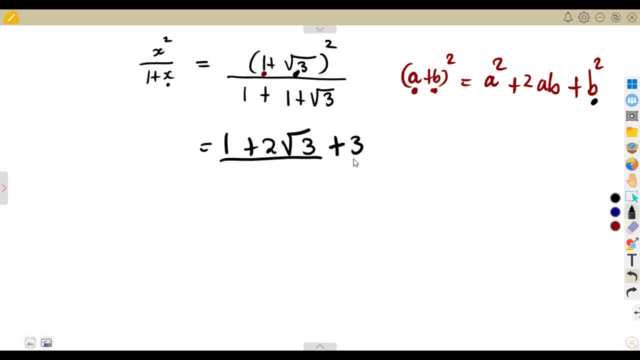 The 1 and the 3, we're going to simplify that, Do not worry. All right, So everything over here we can simplify 1 plus 1.. That is a 2.. So we've got 2 plus the square root of 3.. 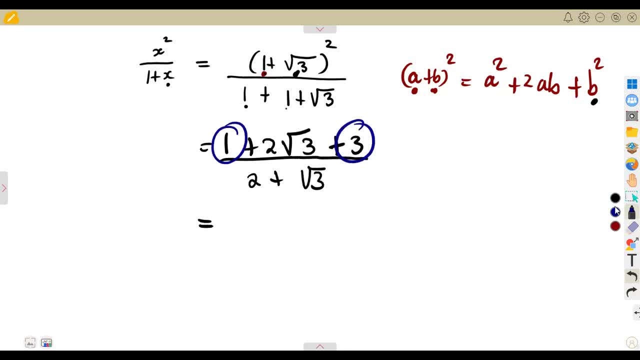 So let's add our numbers 1 plus 3, that is going to give us 4, plus 2, square root of 3.. Everything over 2 plus the square root of 3.. So SEDs, they use rules or laws in their simplification. 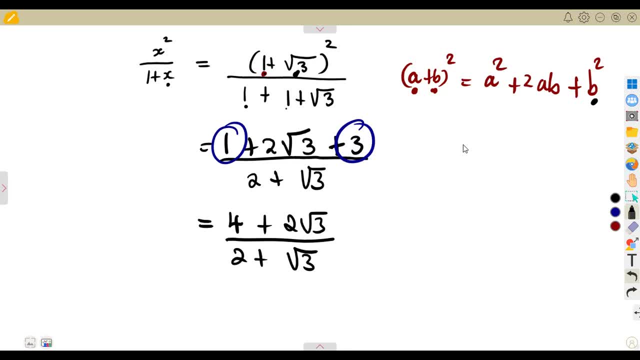 And you are supposed to understand those. So if you are to, If you are given this condition- that is the idea there- If you are given a situation that you have got a division of SEDs, a division like this and you have got two terms that are adding like this: 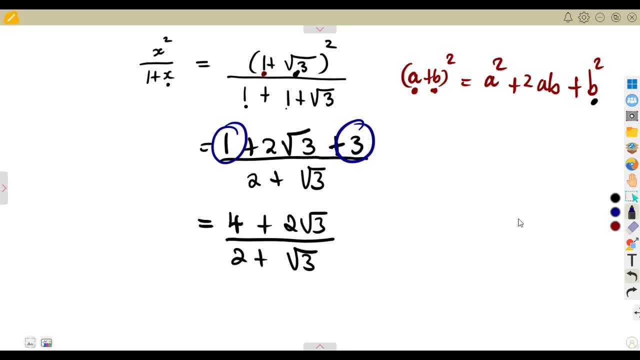 you are supposed to do what is called the rationalizing of the denominator, to make sure that the denominator remains with a rational number, A whole number, Not a square, not a SED. This one is a SED, So how do you do that? 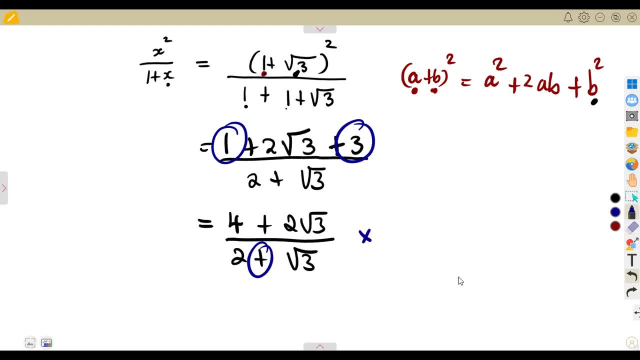 You multiply, You introduce a negative in the denominator where there is a SED, So this will be 2 minus the square root of 3.. You do this also in the denominator. So you multiply both the numerator and the denominator by introducing a negative, this one. 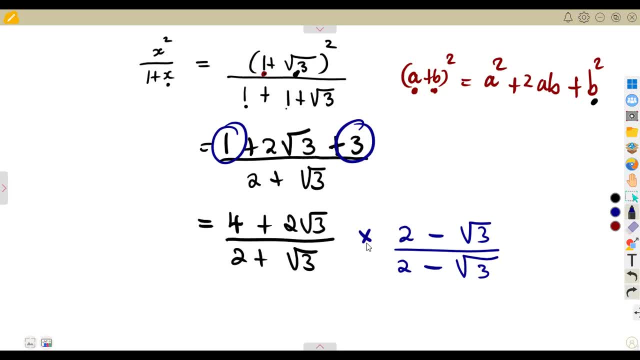 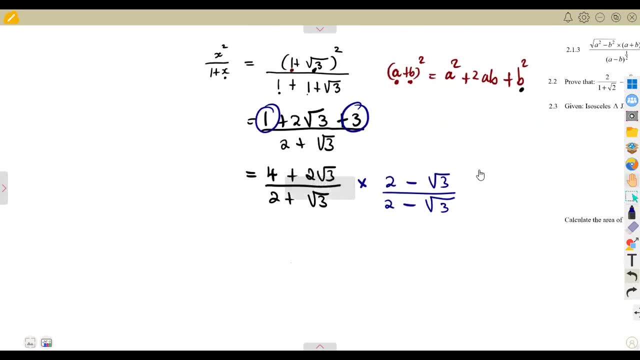 In the denominator, you introduce a negative. By doing that, you are going to see that You will have a rational number. So that part. actually we talked about that on our SEDs, So make sure that you watch those videos also on the SEDs. 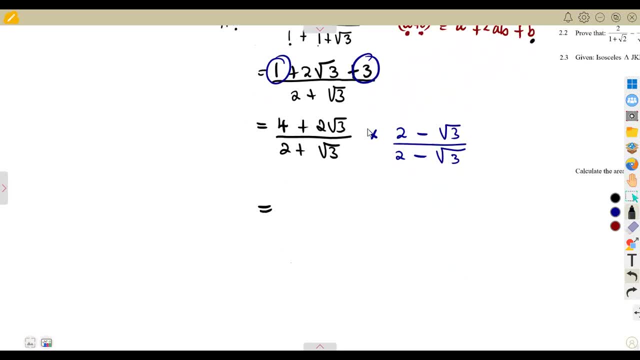 So in the numerator you are simply going to multiply. These are just two brackets to be multiplied. The same thing in the denominator also. So if you do not want to have a condition, you can just rewrite this as 4 plus 2,. 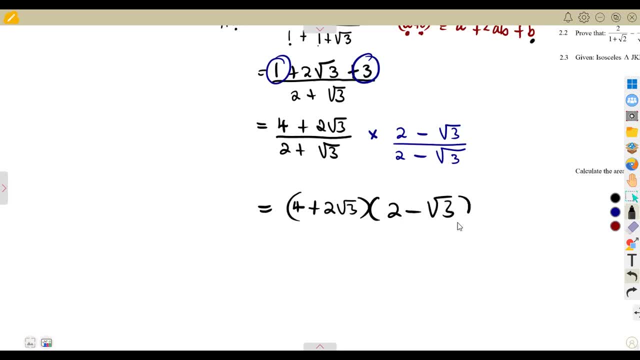 the square root of 3 in a bracket, into these two minus the square root of 3, this other bracket, 2 plus the square root of 3.. In one bracket, another bracket, there's 2 minus square root of 3.. 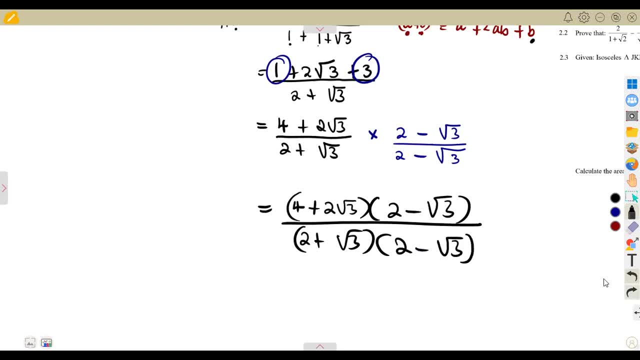 Do not cancel this, because if you cancel, you are neutralizing your question. You are now back to the original question that you had, So never be tempted to do that. Just expand your brackets. 4 multiplies the 2. That is going to be 8.. 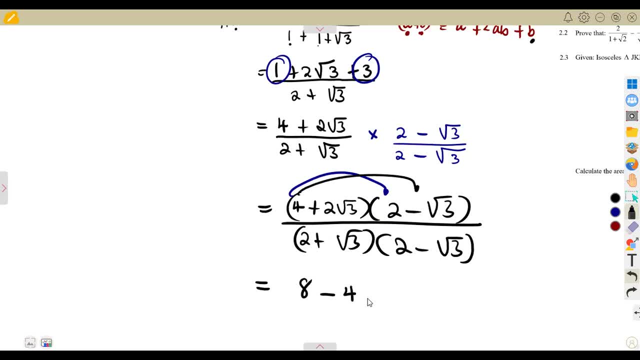 4 multiplies the square root of 3.. That is going to be minus 4 square root of 3.. All right, You are done with 4.. You move on to the plus 2 square root of 3.. It multiplies: 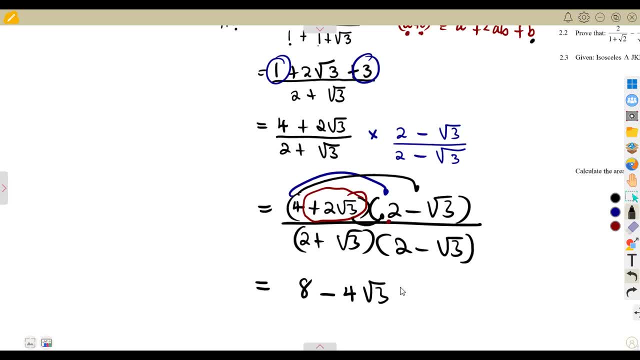 2.. So that's your distribute here 2 times 2.. That is going to be 4 square root of 3.. 2 square root of 3 multiplies minus square root of 3.. So it's like this: 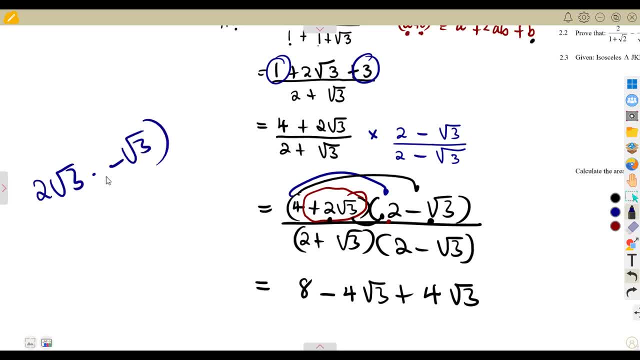 2 square root of 3 times a negative square root of 3 like this. So remember what we got previously: Square root of 3 times square root of 3.. It gives us a 3. So it will be a minus 3.. 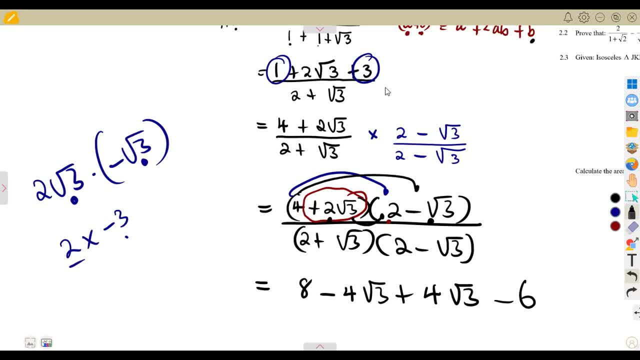 And 2 times minus 3 is going to be a minus 6.. Remember, guys, we talked about this before when we got this 3.. It was from square root of 3.. Square root of 3 times square root of 3.. 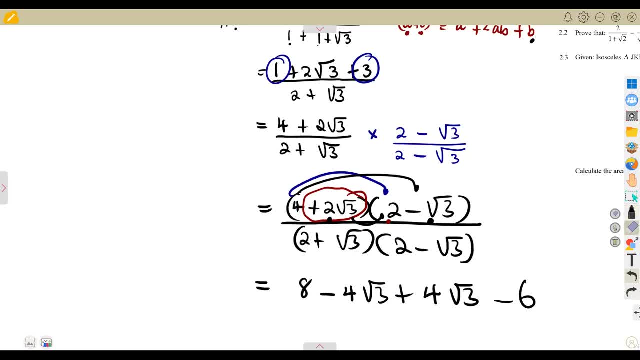 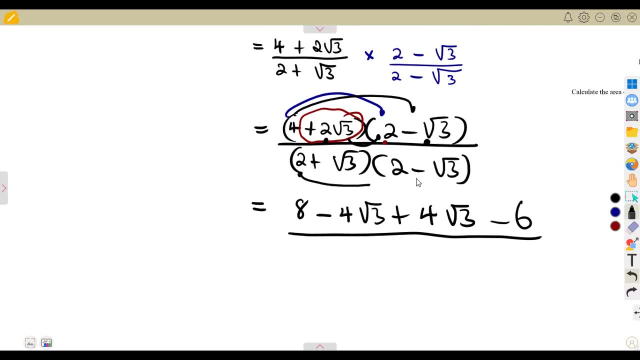 So I'm not going to talk about that again. Consider the previous case. All right, With the same idea, you are going to expand the second bracket. 2 multiplies the second bracket. Everything in the second bracket must be multiplied by these 2.. 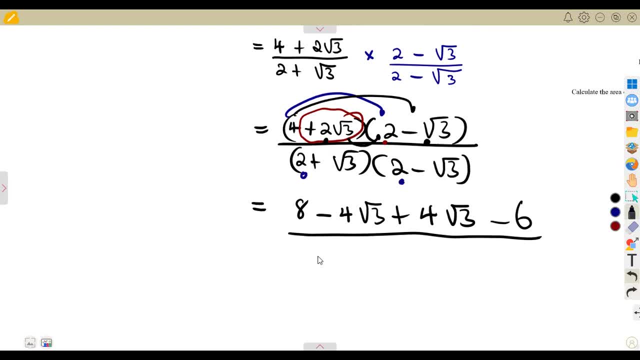 So that means 2 times 2 is going to be 4.. All right, Then you've got 2 and minus square root of 3. So there's a minus 1.. So 2 times minus 1 is going to be minus 2.. 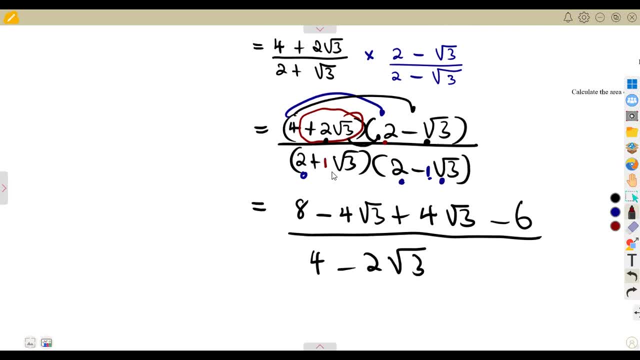 Square root of 3.. You are done With 2,. you move on to 1. Square root of 3.. It multiplies 2.. So it's 1 times 2, which is going to be 2 square root of 3.. 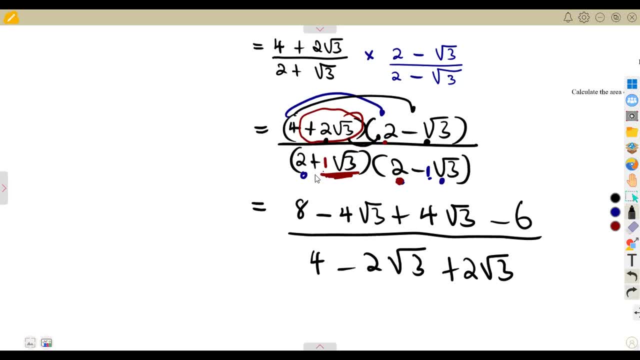 All right, We do the same thing on the square root of 3.. This is square root of 3 times minus square root of 3.. So there is a minus square root of 3 there. So the square root of 3, the square root of 3, we got a 3.. 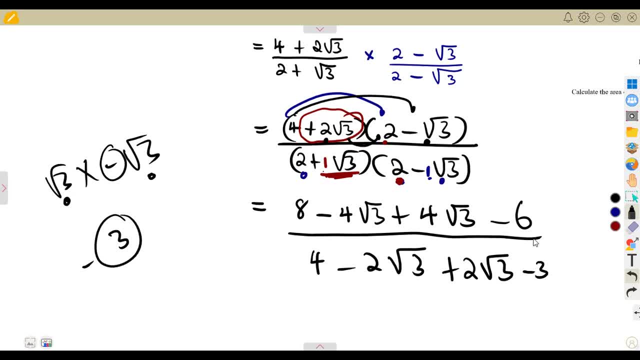 Remember, but this time there is a negative, So it will be a minus 3 at the end. Remember your simplification of the square root of a 3.. All right, With this situation, you are going to see that there is something that is happening. 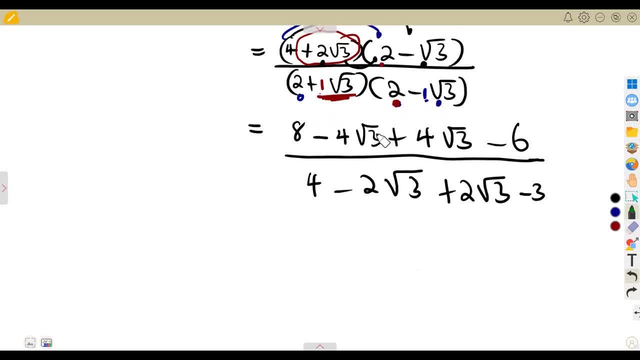 that you need to consider here. These are like terms. All right, The same thing with the whole. numbers also are like terms, So I can simplify this: 8 minus 6.. So 8 minus 6.. If you simplify it this, that is going to be a 2.. 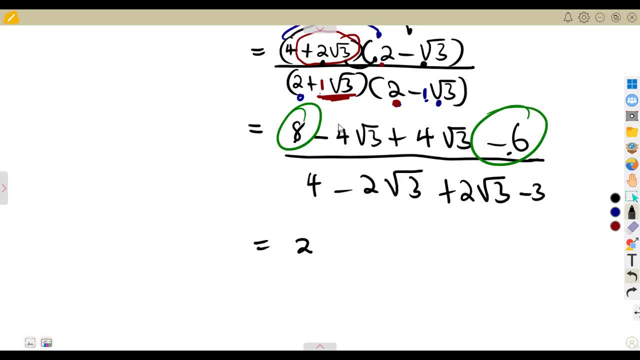 Minus 4 square root of 3, plus 4 square root of 3.. These are the same. So minus 4 plus a 4.. That's a 0.. So 0 square root of 3 is same as a 0.. 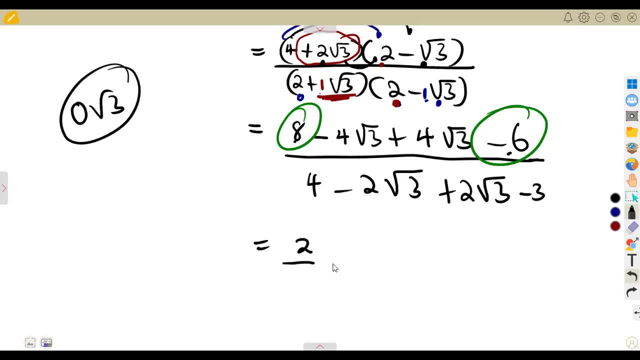 So there's nothing that you're going to have in that part, It's just going to be a 2.. Over you do the same thing: 4 minus 3.. These are all numbers. So 4 minus 3, that is a 1.. 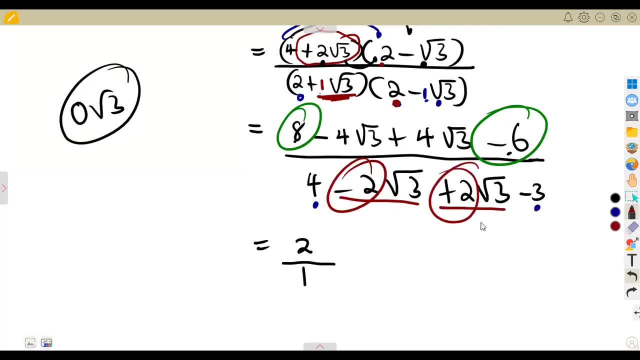 Minus 2, square root of 3 plus 2. square root of 3 minus 2 plus 2.. That's a 0.. So I I talked about this. So 0 square root of 3, that's a 0.. 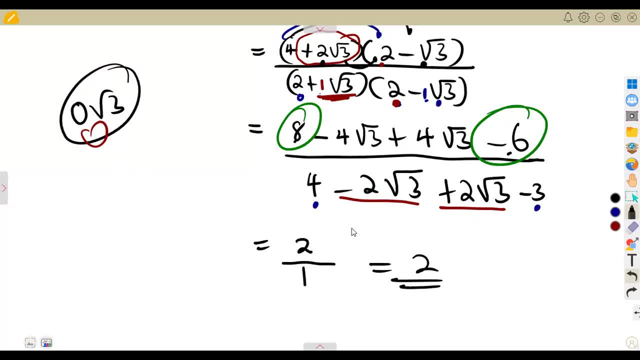 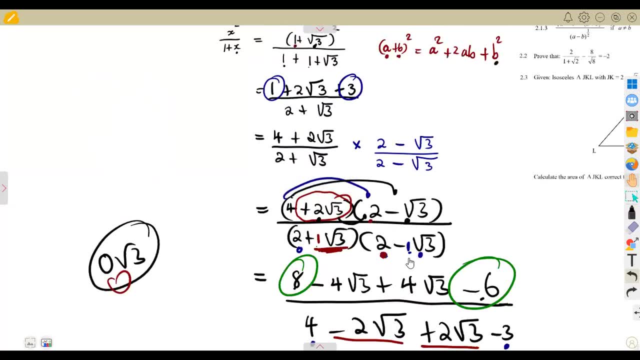 So meaning say you're going to have 2 over 1, which is a 2. That's it. So, as you can see the square root on the square root there, they eliminated each other. So that means you're not going to have them in your simplification. 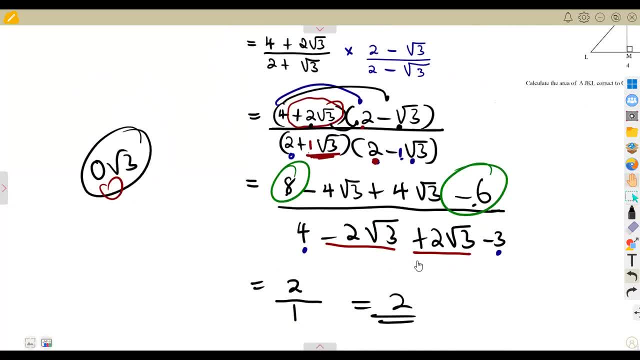 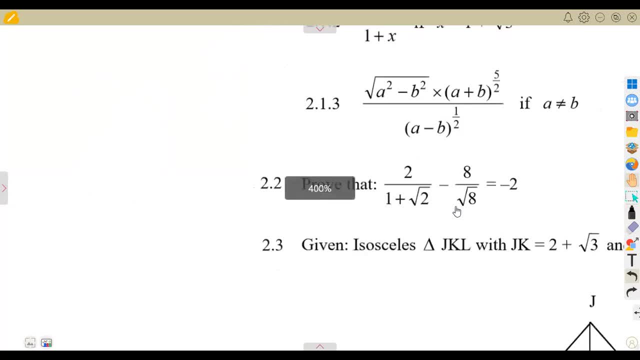 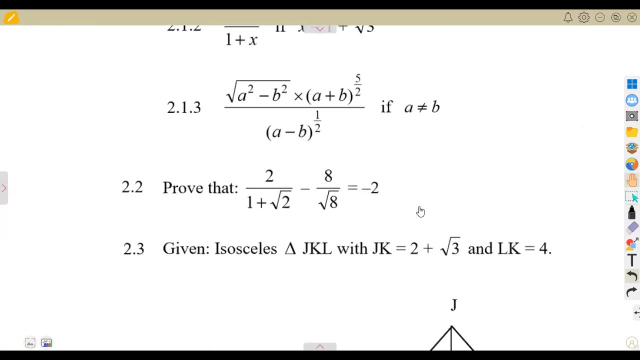 That is how our questions might be given as So this is what it was going to be at the end. All right, Let us consider 2.13.. Again, simplify, And this is 4 marks again, And a is not equal to b. on this expression, 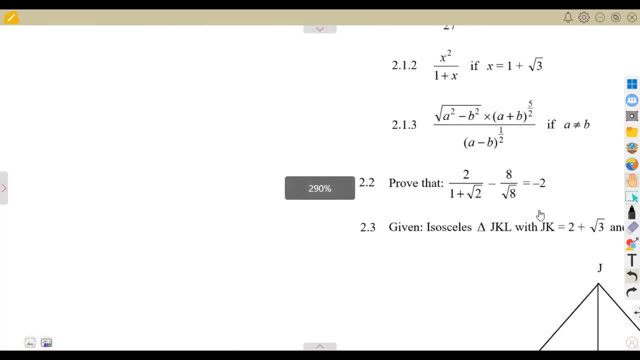 So we are given this part. I'm just going to rewrite this. All right, Let me just rewrite here. So that's 2.13.. We are given, to simplify, the square root of a squared minus b, squared like this, Multiplied to a plus b, to the exponent of 5 over 2.. 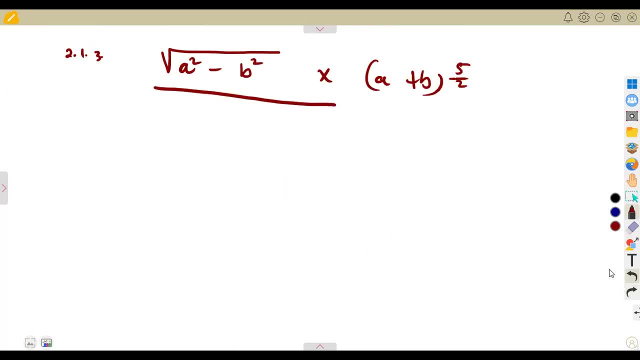 All right, And this whole part here is Divided to: All right. Sorry guys, This is divided to a minus b, to the exponent of 1 over 2, like this, If you were to consider this as maybe square root of x times: 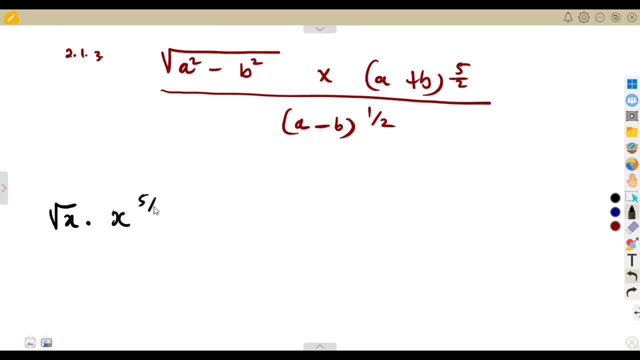 maybe xc to the exponent of 5 over 2 over maybe x. You had something that is about the same basis that you understand much because it is Written as x. You understand that much, Guys, as long you see these exponents there. 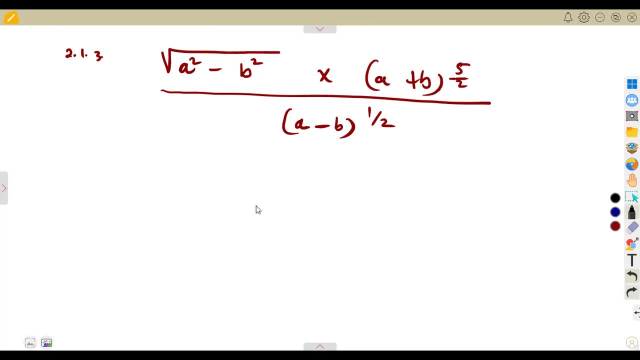 Think of the exponents, Also the laws of your exponents, In the same manner that you understand that if you are multiplying the bases which are the same, you add your exponents. If you are dividing these bases, which are the same, you subtract. 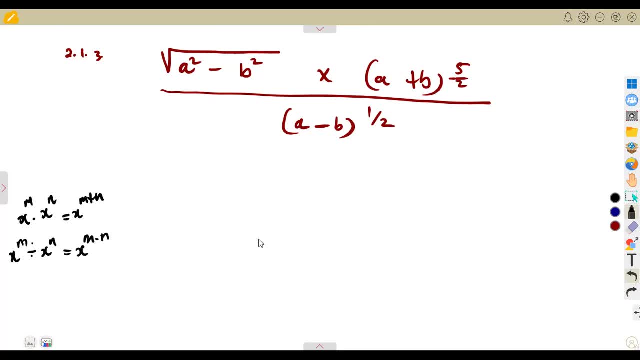 Your exponents in the same manner: a minus b. If it is the same, that is the same base. a plus b: If it is the same, that is the same base. So the question is, can we have another a plus b, or maybe another a minus b, so that we can simplify this from where? 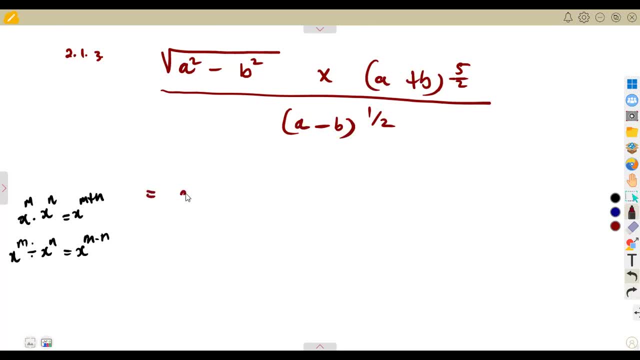 OK, let's consider first. the square root is the same as to the exponent of a half. So This is just a given or can be written as to the exponent of a half. Remember from your laws, of your exponents A plus b to the exponent of 5 over 2.. 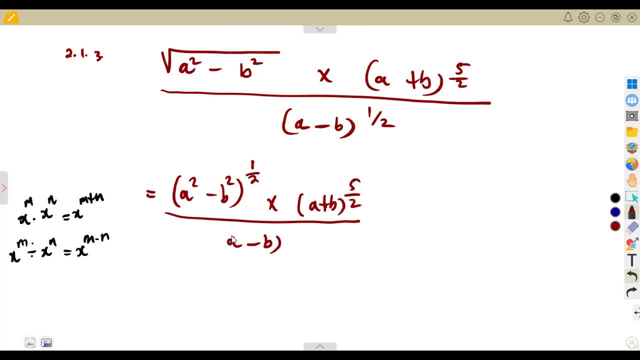 There's nothing that you can do. You will never be tempted to expand that one. You can't expand this one in your syllabus unless you go to another higher level. But for now in your syllabus that one is impossible. You can't expand this type of a fraction. 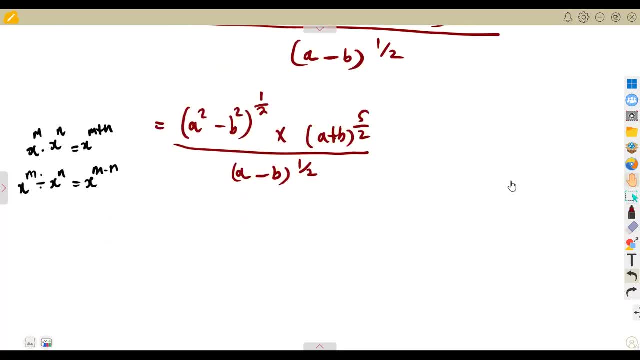 Just leave it like that. But if you are to check, we understand that a squared Minus b squared. This is a difference of two squares Which is going to give us two brackets. In actual sense, we are supposed to have the bracket of a minus b into the bracket of a plus b. 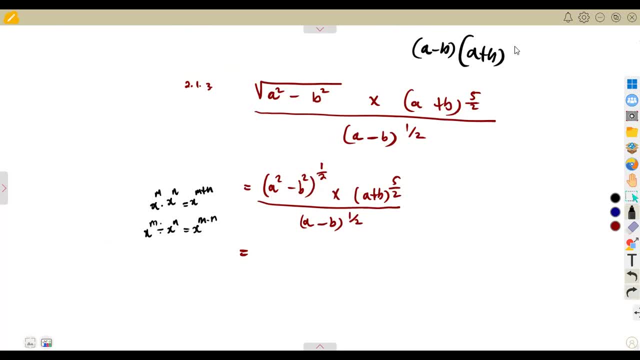 Being affected to the exponent of 1 over 2.. Everything that we are seeing here being affected to the exponent of 1 over 2.. Our difference of two squares, which is the a squared minus b squared, But there is an exponent. 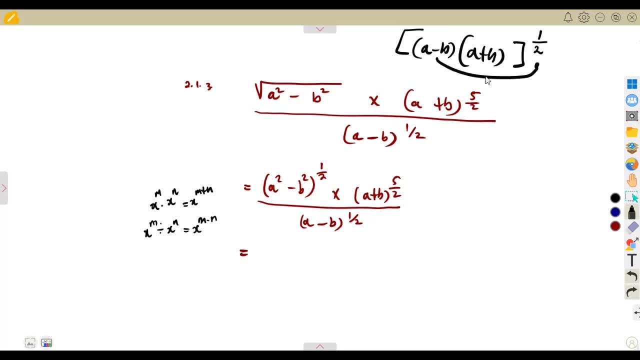 Of a half there. So what does it mean? It means everything in this bracket is going to be raised to the exponent of what? Of 1 over 2.. The bracket of a minus b will be raised to the exponent of 1 over 2.. 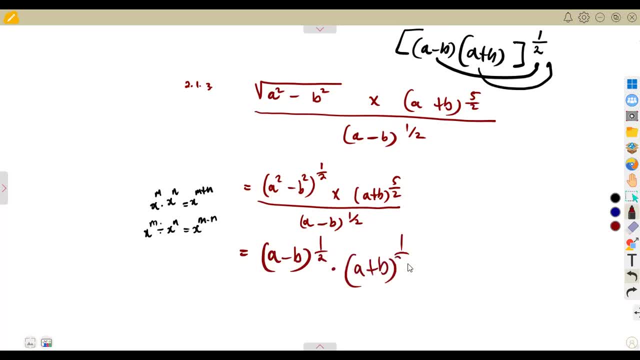 The bracket of a plus b will also be raised to the exponent of 1 over 2.. We have expanded this part. All right, With this, we move on to the other part. We are still multiplying this. There is a bracket there. 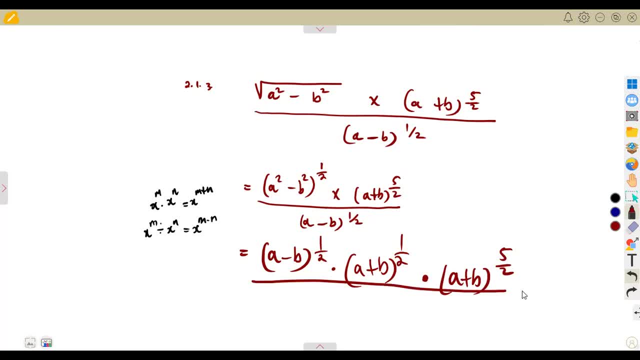 A plus A minus b to the exponent of 5 over 2.. In the denominator, there is a bracket of a minus b to the exponent of 1 over 2.. Which I said, we can't simplify this, But by having now these same brackets, the brackets that are the same. 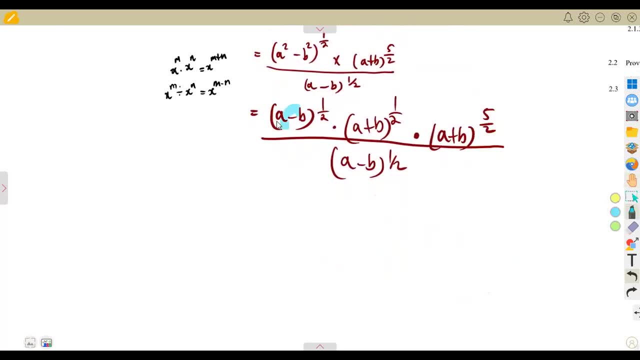 The bracket of a minus b and also the bracket of a minus b. This alone tells us that there is something that we can consider And, besides, that, these two brackets are exactly the same Even without applying our laws of exponents. without this, these two brackets are exactly the same. 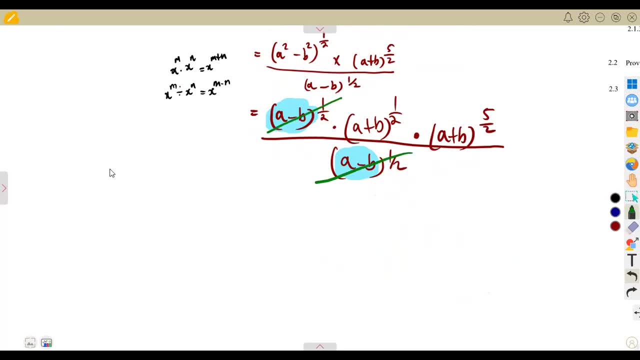 So I can just cancel these two brackets. There is x over x is a 1.. x over x is a 1.. So if you are given that part, if you are given this part, you can cancel, You can even cancel. 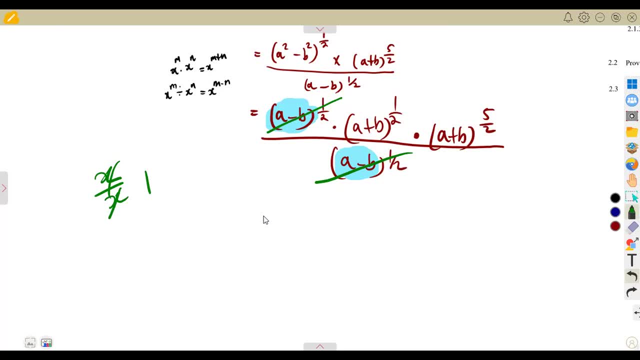 So meaning to say that If you are given a consideration where the same you can cancel- But let's say you did not recognize that, You just recognize these are the same bases- Then you want to subtract your exponents. You are going to subtract half minus half. 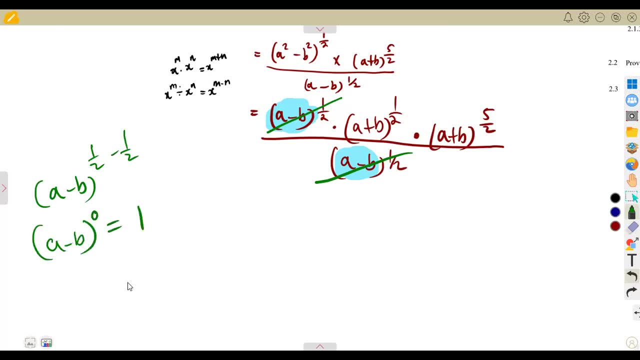 It's going to be a minus b to the exponent of a 0. And this will be a 1.. The whole bracket is being raised to the exponent of a 0 there. So still, you are going to get a 1.. 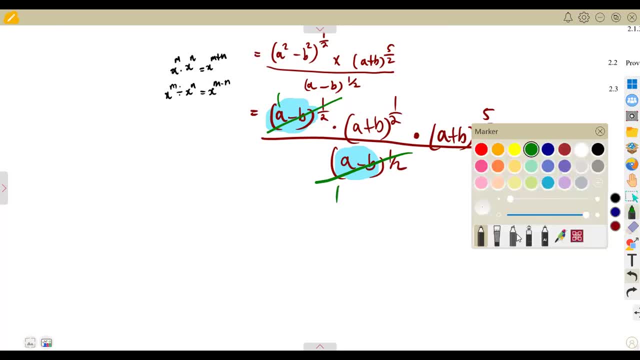 All right, Let's move on to the other part. We have got another Part which is the same, in this case the bracket of a plus b and the bracket of a plus b. These two brackets are also the same, in the same manner. 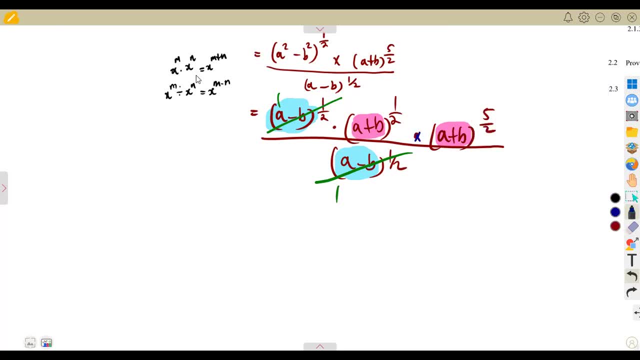 But this time we are multiplying. So on the multiplication, we said: if the bases are the same, what do we do? We add the exponents. So in this case, if you were to add the exponents, it was going to be a plus b. 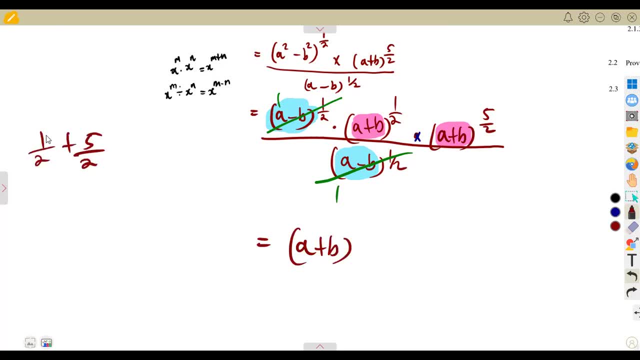 You add This was going to be 1 over 2 plus 5 over 2.. So remember, if we have got this consideration of the Same denominators, just add your numerators 1 plus 5, which is 6 over 6 over 2.. 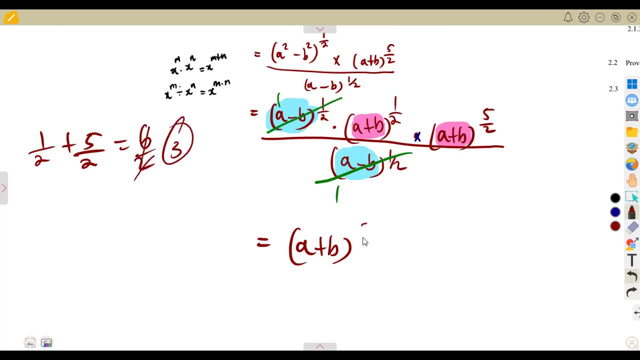 Sorry, 6 over 2.. And this is going to be a, 3.. So that was going to give us a plus b to the exponent of 3, which we can expand. But remember this is also an identity that you're supposed to know. 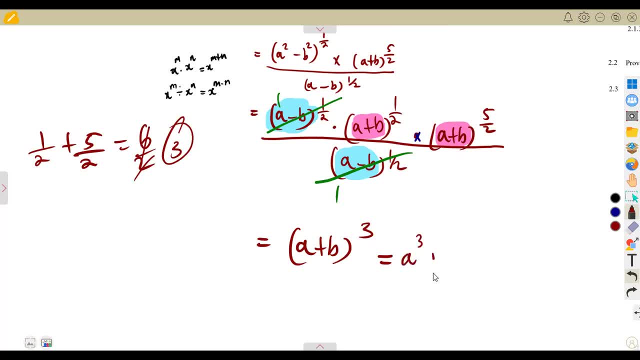 a plus b to the exponent of 3 is same as a cubed plus 3a squared b plus 3ab squared plus b. So take note: a squared b, then it's going to be a, b squared, then a and b are the bodyguards. 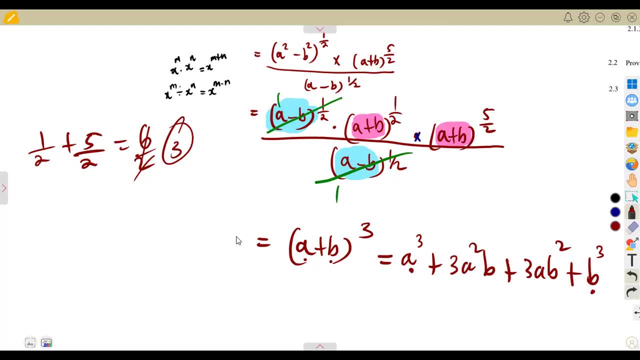 being raised to the exponent of what of 3.. So it's an identity that you are supposed to also understand or that you are supposed to to know. All right, So each and every part that you have, you are supposed to understand And your identities- you can simplify your identities. know your identities when I expand. 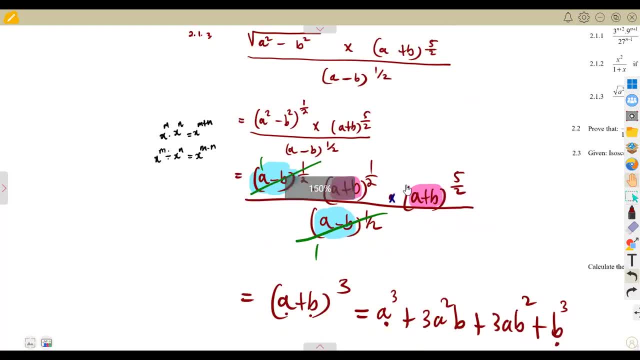 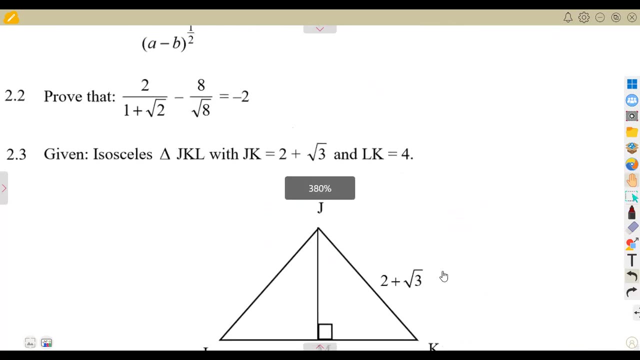 one, one, guys, it's up to you. So this is it, Just like that. So you see, the laws, everything has to be has to be applied properly. Prove that this whole part that we see is equal to minus two four marks. 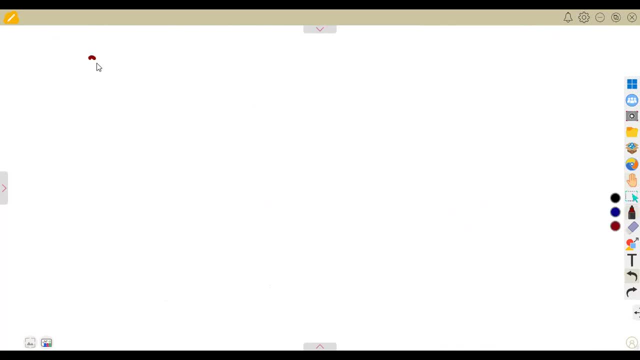 We are supposed to prove This is 2.2. All right, we are given two over one plus the square root of two minus eight over the square root of eight. They are saying: this whole part must give us a negative to prove. to prove it means you. 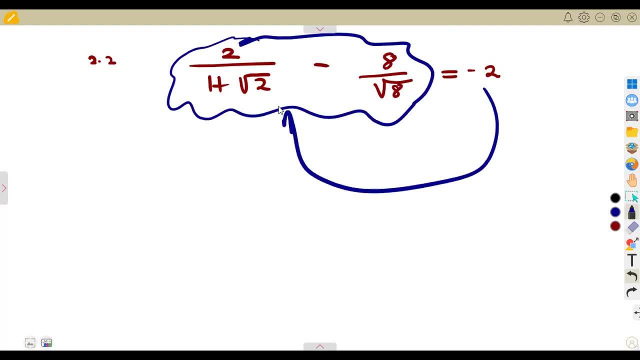 are supposed to take one of the sides. So, guys, it's going to be complicated to start here to. it's going to be very complicated, So it's easier to work from the complicated side to the easier path. All right, So, choosing the left hand side, we are going to see that we have got two over one plus. 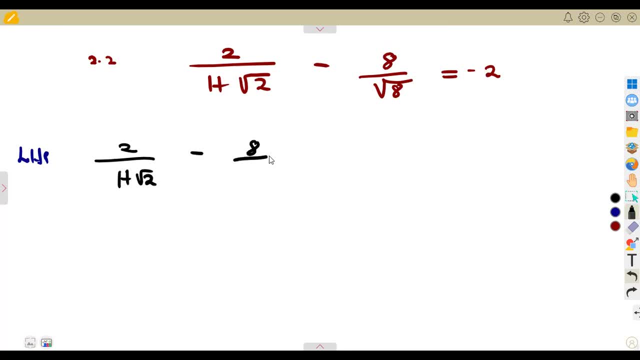 the square root of two minus eight over the square root of eight. This is what we have. I talked about rationalizing of the denominator previously. if you still remember how we calculated this part, That is the same thing as long We have got. 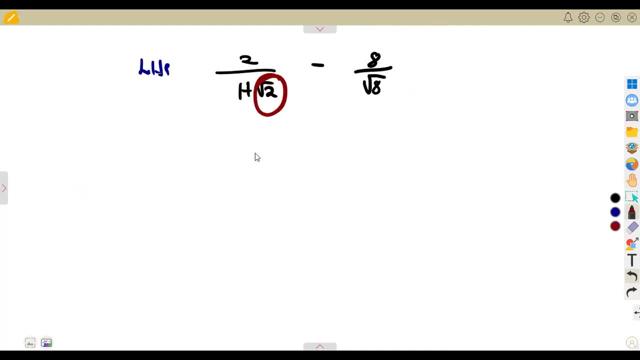 This denominator having a ratio, an irrational term, an irrational number, a number under the square root. But I said, if it is an expression like this, you introduce a negative where there is a said, where there is a square root. So this was going to give us. let us just consider it like this: 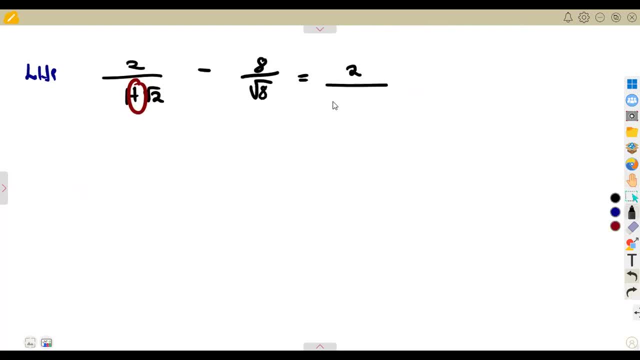 So this was going to give us two over one, plus the square root of two. So, considering the part where the said is, if we introduce a negative, this was going to be plus. you multiply the plus and minus, so it will be minus the square root of two. 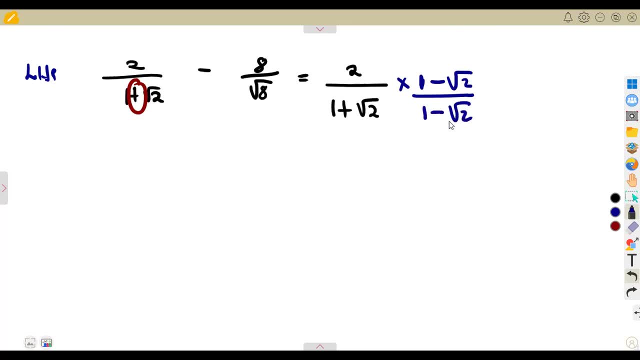 over one minus the square root of two. multiplying by the numerator and integer the same simply means you multiply it by one. So there is no effect on that one. There is no effect at all. There is no effect. This happens When you. 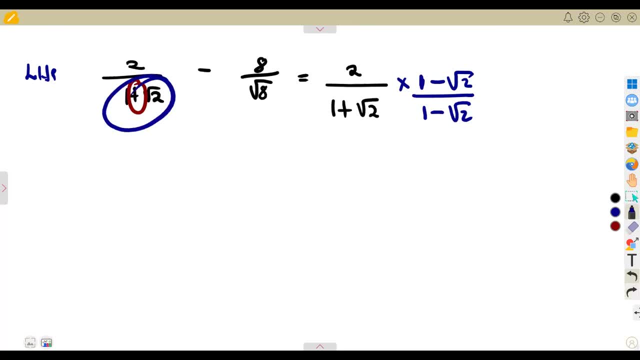 Add a negative. it is when you are given two terms, you are adding or subtracting. But when you are given a single term like this one, a single said, there is nothing added, There is nothing subtracted. You multiply by. that said as it is. 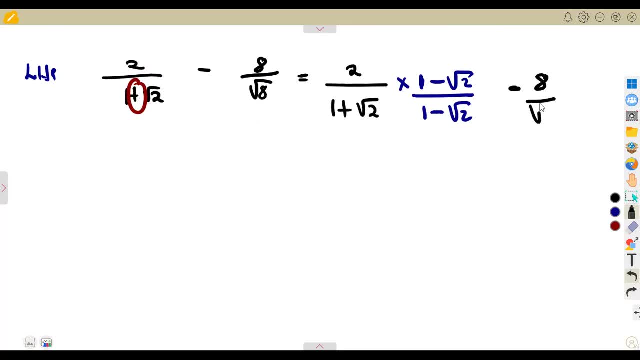 So it's minus eight over the over the square root of eight. So the square root, it's an irrational number. So we want to rationalize this. You multiply by. that said as it is, It's a single term. There's nothing added. 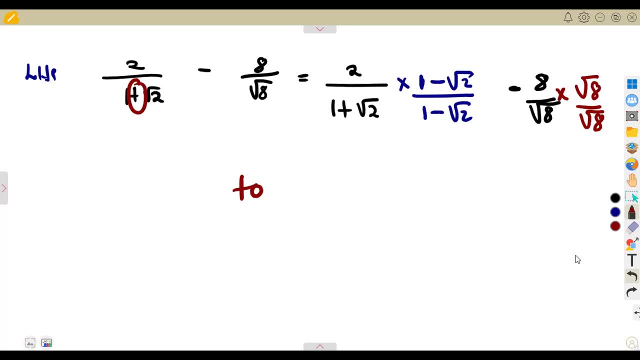 It's like there's a plus zero there, So what are you going to do? It was going to be. there's nothing All right. So when you're given a single set, just like a zero is plus zero, So just use that single set as it is to rationalize. 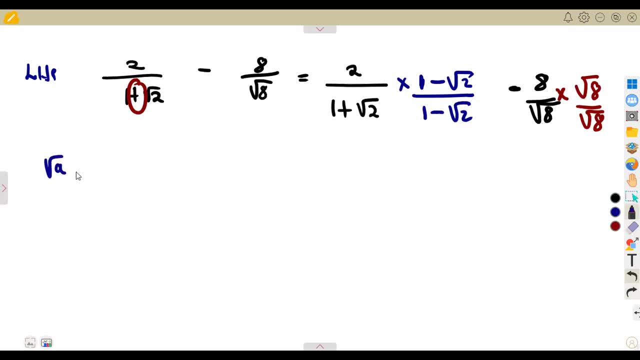 Why, Remember, I say the square root of a number times the square root of that same number. If this is a and this is a, the answer will be a. So if you multiply the square root of eight to the square root of eight, eight and eight, 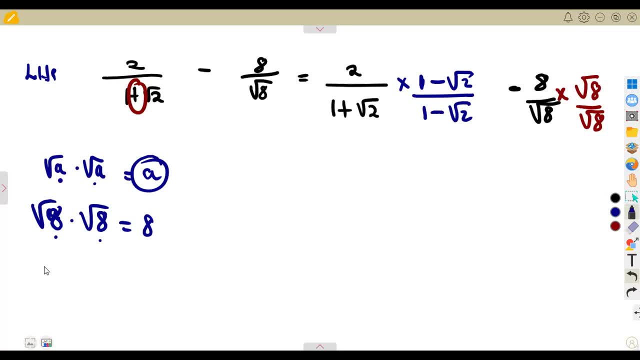 are the same. So the answer is going to be eight. Or you can multiply eight times eight square root of 64, which is eight again on in the same. So by rationalizing we can simplify. the numerator multiplies the numerator on its own. 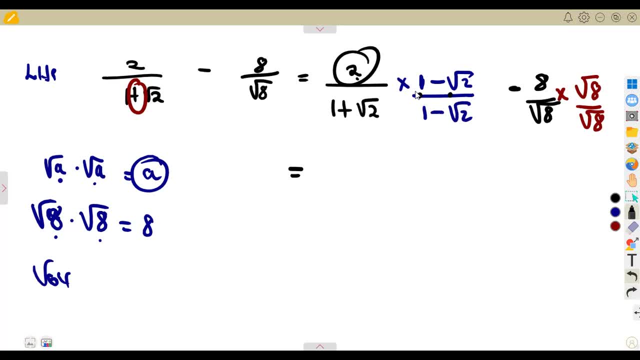 So, guys, as you can see, two is going to multiply everything here Two times one. That is going to be two. Two, Two times minus square root of two, that will be minus two square root of two. There is a one there minus one. 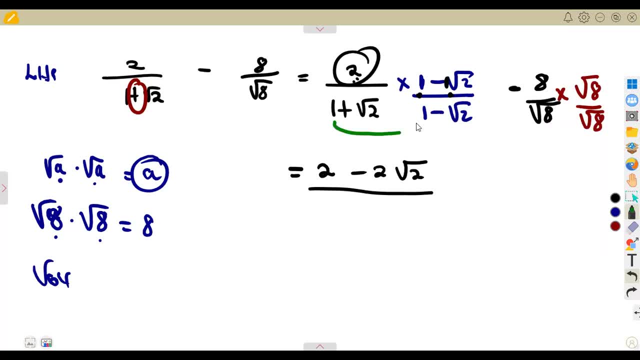 Everything over the denominator. you do the same thing. One is going to multiply with one. that is going to be one. You move on to this: one multiplies minus square root of two. That will be minus the square root of two. So you've got minus the square root of two. 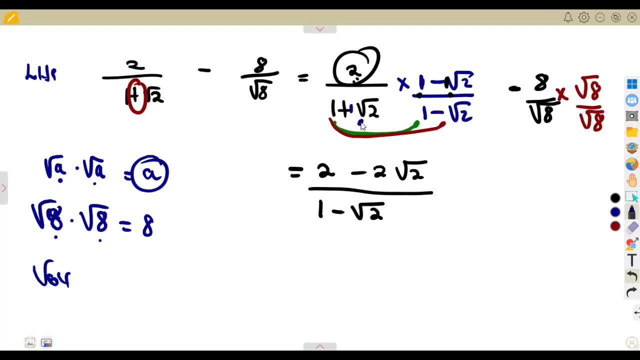 You are done. You move on to the square root of two. It's a plus here, So square root of two, Two times one, That is plus square root of two. You move on the square root of two times minus square root of two. 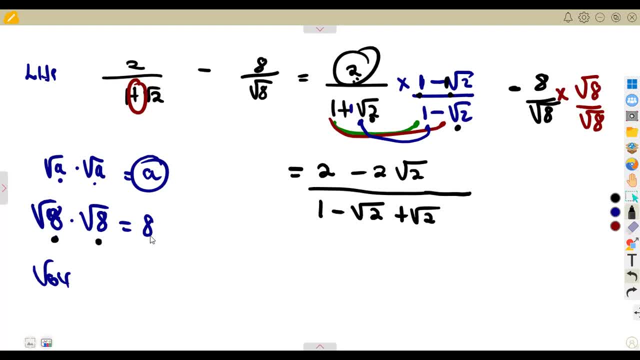 Remember what I said: Square root of a number times the square root of that number is that number. So the square root of two, if it multiplies the square root of two, we are supposed to get a two. But because plus and minus on the multiplication, plus and minus on the multiplication is what 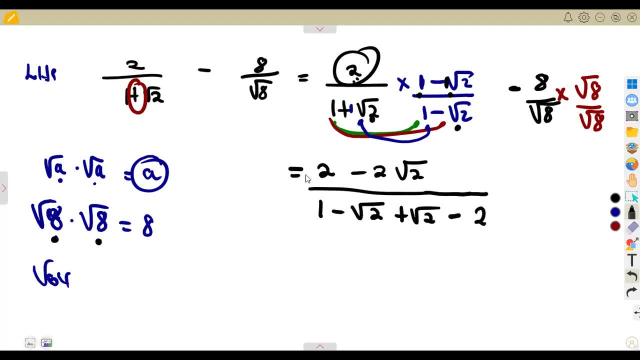 it's a minus, So it will be minus two guys. on the multiplication, Even I just use a calculator. No, I just use a calculator, Just use it. It's the same, Because the answer that you're just getting there is the same as the one that will just. 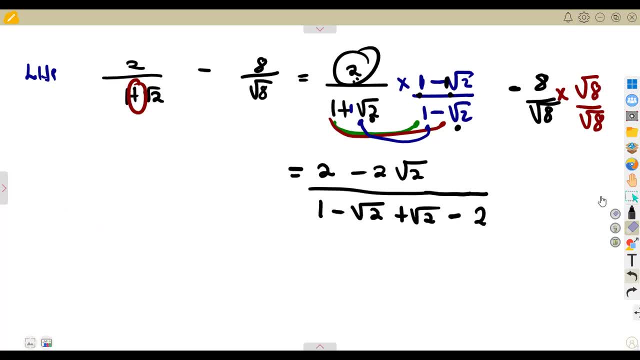 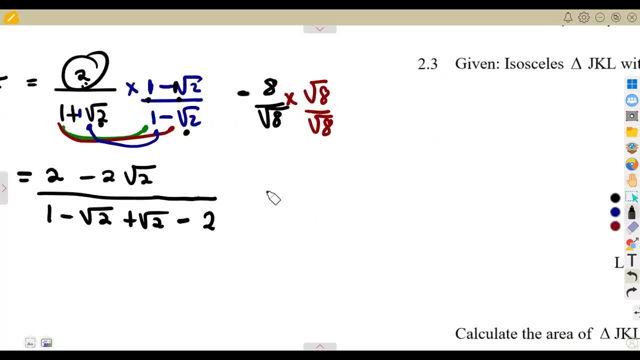 knows this one by head. So if you're having confusion, just use your calculator to multiply square root of two times square root of two. All right, No one is gonna talk about that Minus. we do the same thing on our multiplication. 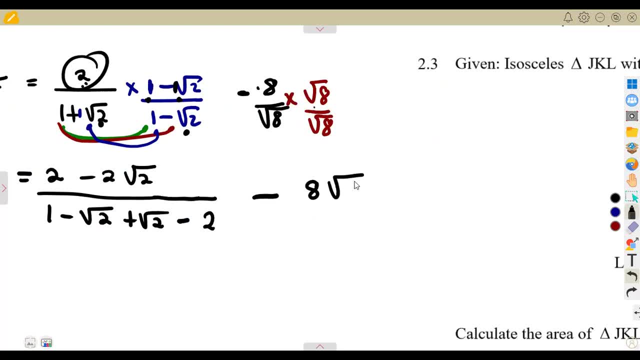 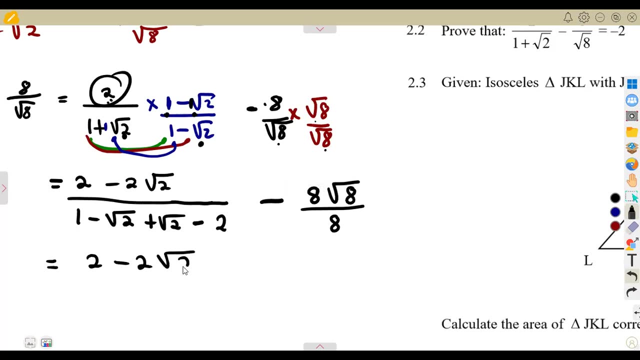 Eight times the square root of eight means we've got eight square root of eight Over the square root of eight times the square root of eight. we are back to that. So remember that we're going to get an eight them. Then we simplify further to minus two square root of two. there's nothing that we can do. 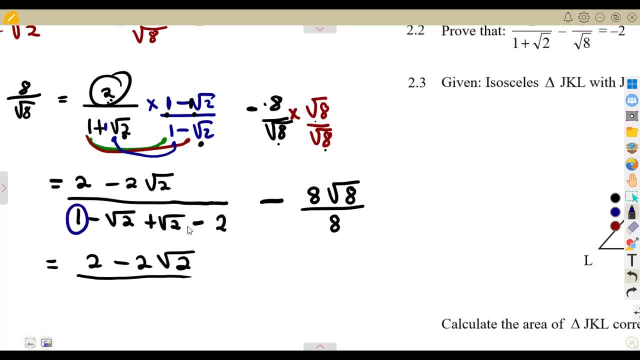 everything over the denominator. there is a one, there's a minus two. these are all numbers. So we can subtract one minus two. that is going to be minus one minus square root of two plus square root of two, square root of two. This is the same as minus one plus one. minus one plus one. that is zero there. 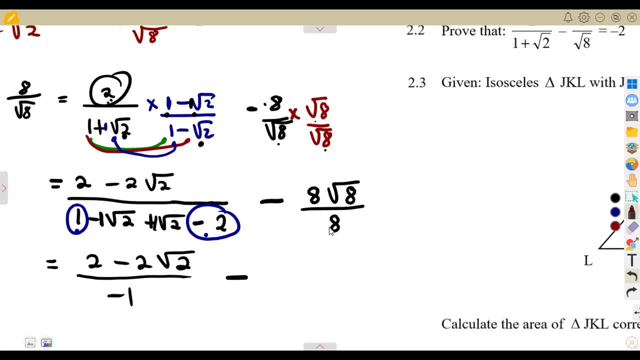 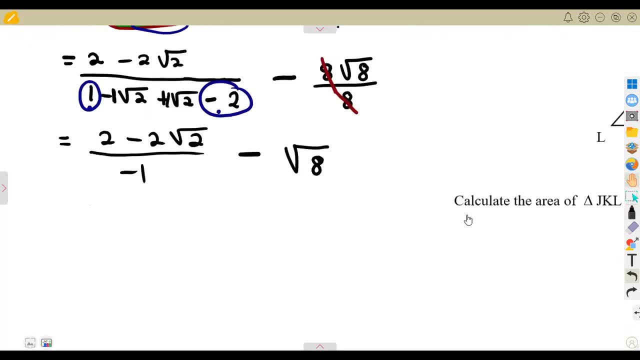 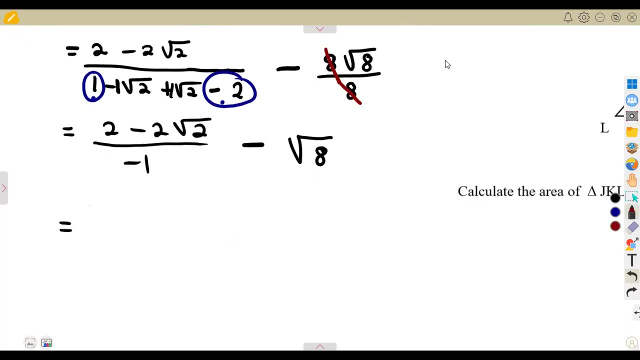 So many say there's nothing there. So this will be minus eight and eight cancels we remain with the square root of eight. So at this stage we are going to simplify dividing by negative one. remember from our grade 10, a plus B over C is the same as A over C over C. like this is same as A over. 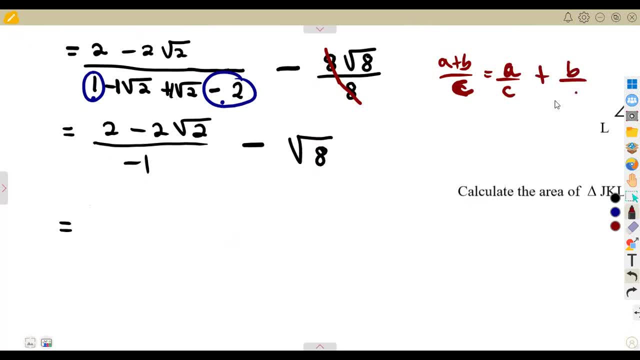 C Plus B over C. So meaning to say this is MS two over minus one, which is going to give us what minus two? the same thing, this one minus two, square root of two over minus one. So if you divide minus two and minus one, minus two and minus one, that's a positive. 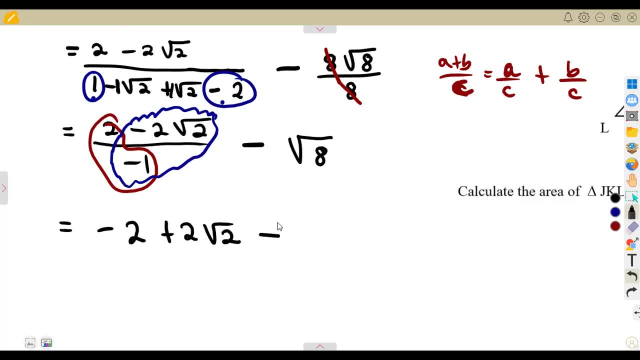 two square root of two. all right, minus the square root of eight is not equal to minus one. So the square root of eight is not in the simplest form, the square root of eight is not in the simplest form, this one. So it must be as simple as to say it's either. you're going to simplify that part, the square. 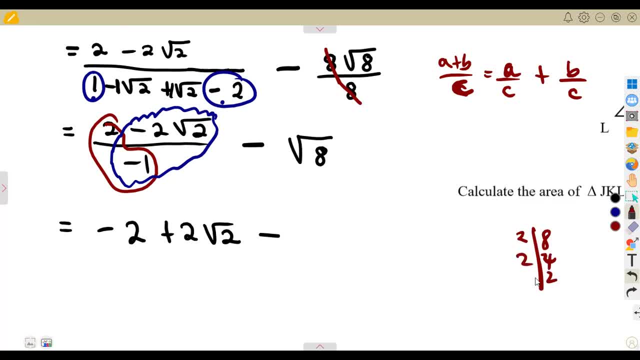 root is a prime numbers, two into eight, which is for two and two. then you've got two and two. that's a pair, So a pair. you write it outside of the square root. where there's no pair, you write it. 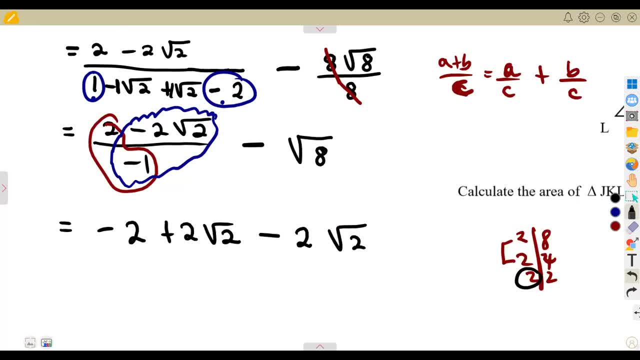 inside of the square. it's up to you. But at this stage I want you to be clear, Because even if you have a square root, you have a negative one. you have a negative one Even someone who knows or understand that square root of eight is same as four times. 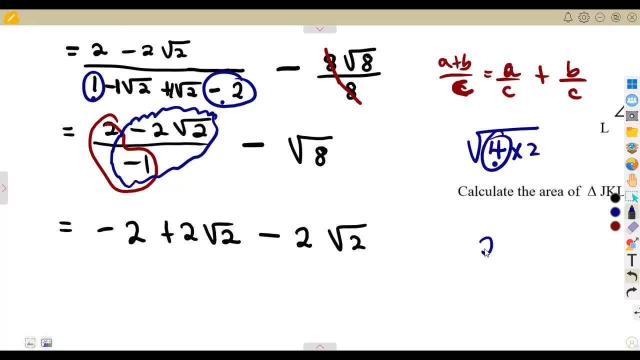 two for a perfect square, and the square root of four is two. square root of four is two, So the square root of two. we do not know. So we still have the same answer, even if you don't show this and use your calculator. 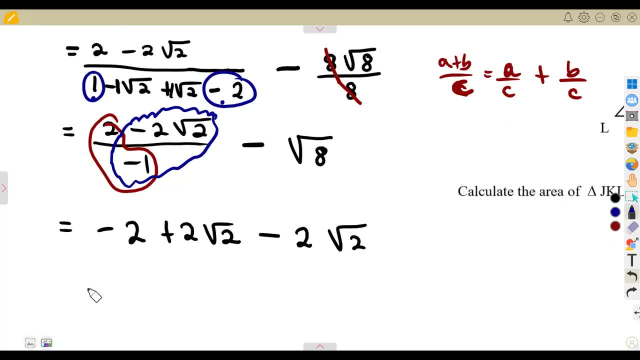 at this stage. do that, do that, do that? All right. So this is two square root of two minus two square root of two, that's a zero. there, This cancels my two minus two, that's a zero. So at the end, you are going to obtain minus two. 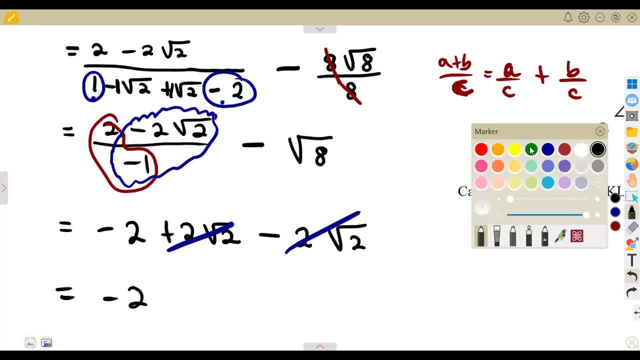 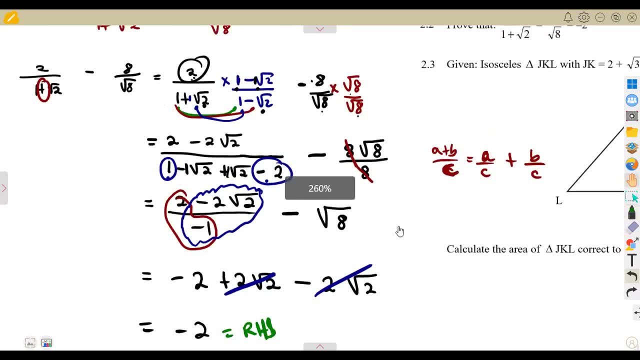 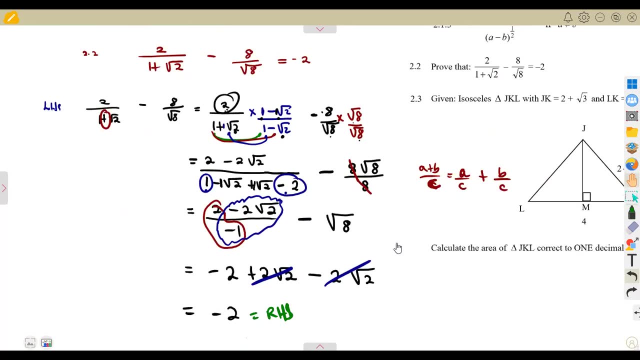 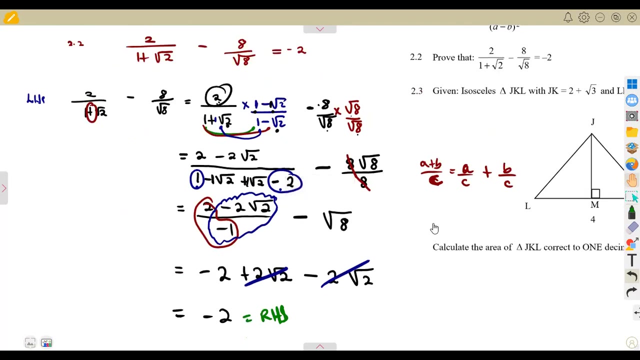 So this is exactly what we are seeing on the right hand side, So this is exactly what is equal to the right hand side of our of our equation. So we take it as an equation. We take it as an equation, All right. We hope we take that one as an equation. 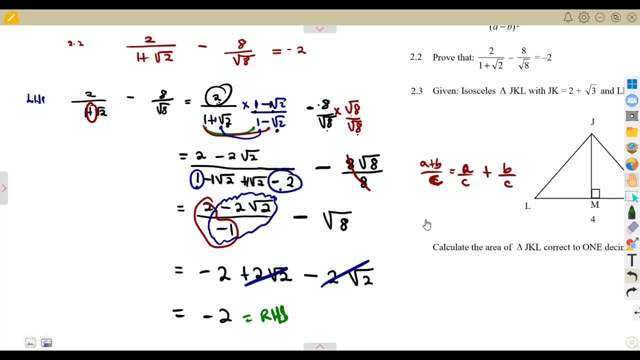 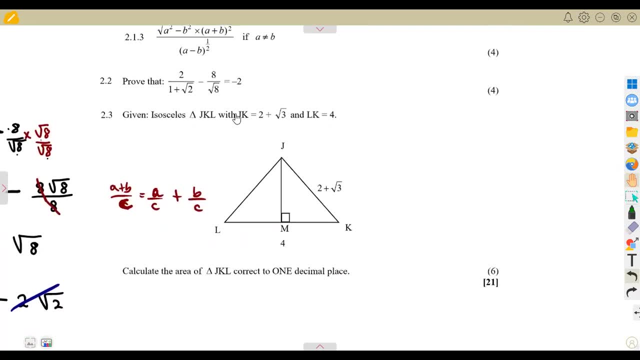 You prove that this is equal to the right hand side, Just like that. So they are saying: let's hope it's not a continuation, or at this one is on its own. Okay, so all right, all right, two plus this. all right, this one is on its own. I just 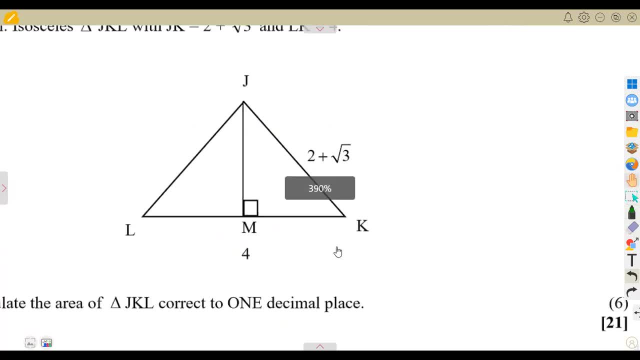 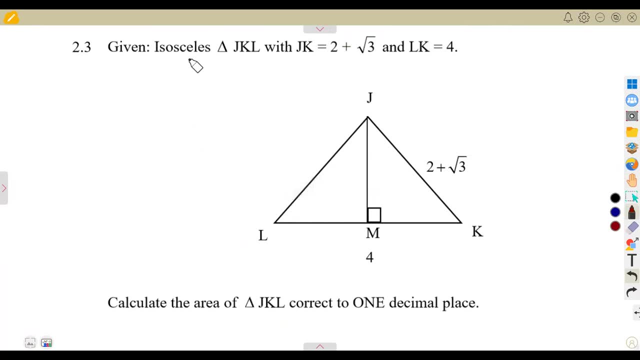 thought maybe it's gonna be a continuous. most times they want you to continue from that, But anyways, this is on its own 2.3,, given that the triangle that we have in this case is an isosceles- isosceles triangle. 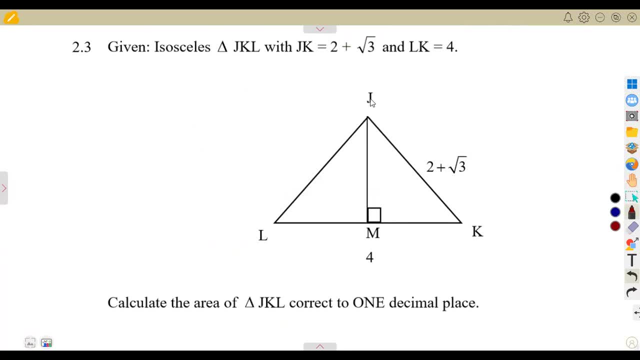 j, e, k, l. if this is an isosceles triangle and we see a line drawn like this, perpendicular to the base, that line, it is not just perpendicular, it is the perpendicular bisector of this base. it is the perpendicular bisector. 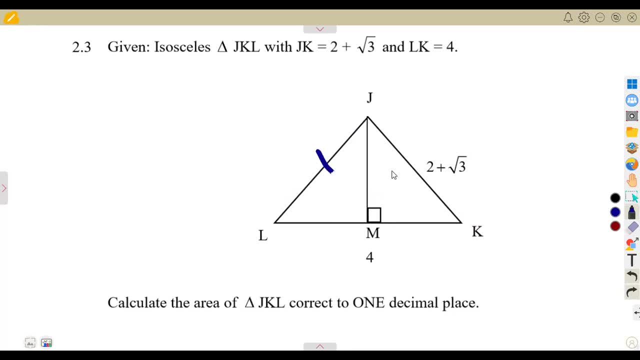 And it shows us that The sides of the isosceles triangle which are equal at these two sides, and this is the perpendicular bisector which bisects this line into two equal parts. So it means from L to M it is the same as from M to K. 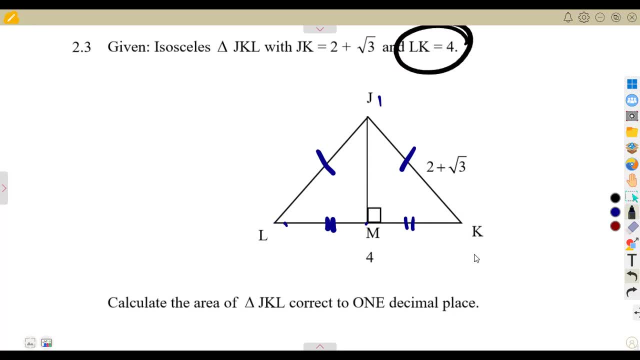 So if we are given the wall of L, K as four units, we divide this by two because the same. so it means I've got two units, two units here. That is what it means. I'm just interpreting our diagram. If this is two, square root of two plus square root of three, it also means this is two plus. 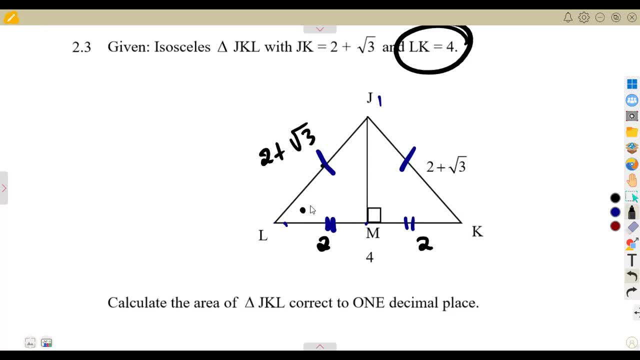 the square root of three. because these sides are the same, These two angles will be also equal. we are not there now into geometry, this and that, our analytical geometry. we are not into that now, All right. The question was: calculate the area of this triangle? 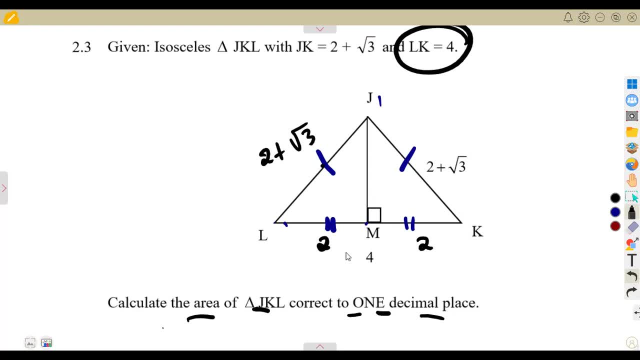 Correct to one decimal place. Now you are given an instruction. That's why they told us before that you are supposed to determine whatever that you have to do this more places, unless stated at the wise That's a condition of an otherwise this one. they stated otherwise here. 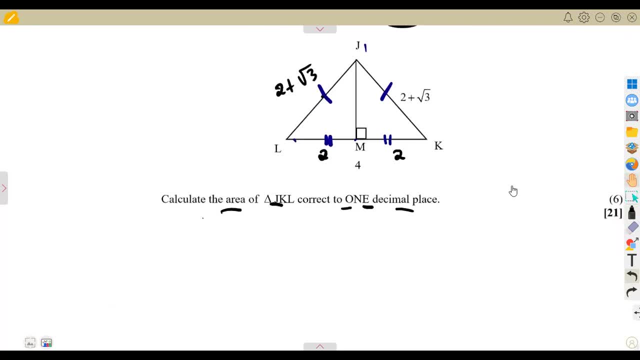 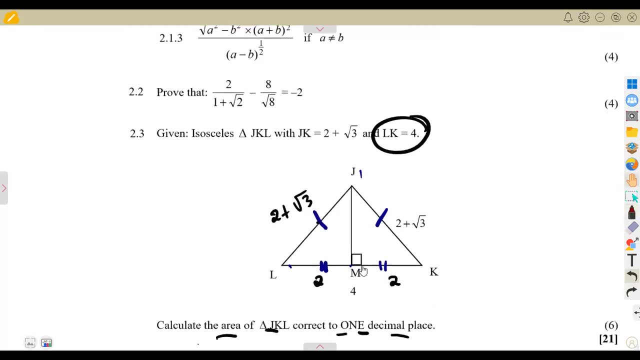 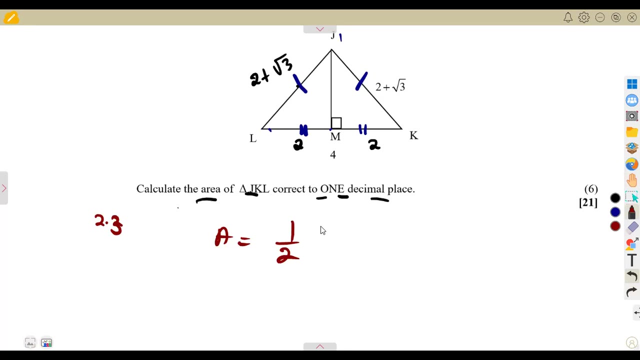 But anyways, even though they stated otherwise, we need to determine the area of this triangle. So how can we determine the area? The area of this right angled triangle, If you were to consider this, is 2.3.. The area of a right angle triangle is given as half times, the best times, the perpendicular. 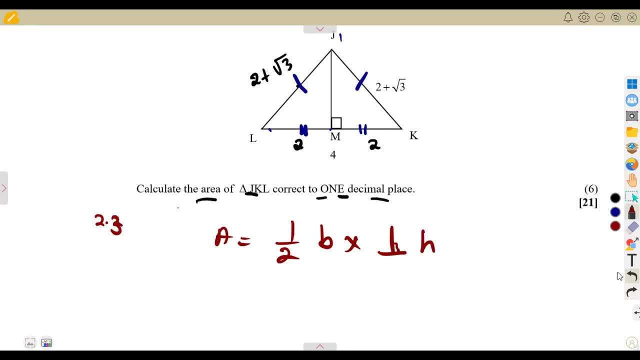 height, which is the perpendicular height. we are referring to this- J, M, And the best of this triangle is going to be L to K. When you're given this triangle, this is the perpendicular, This is the best, So meaning to say, in the calculation of this area, 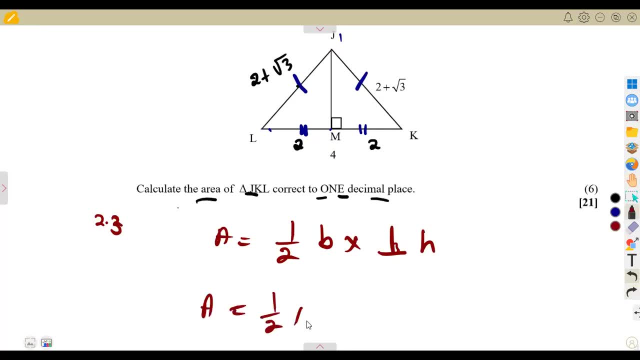 We were going to have something like. this area is equal to half of the best, which is the L K times the perpendicular height, which is from J to M. So you are going to be stuck in this J- M. We have the L to K, which is this one: 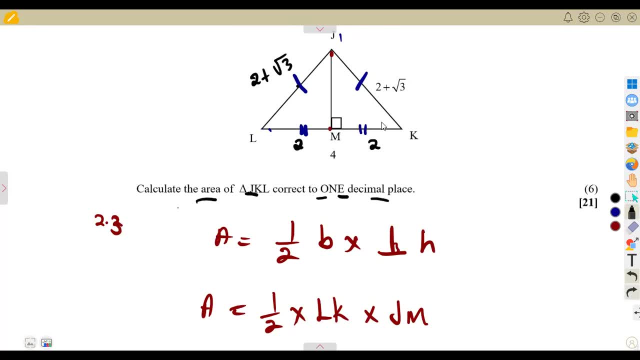 All right. So there was no need for us to even try this as two and two. unless you want to use this triangle on its own, This triangle is on on the calculation. We're going to see that one where it is special, Not now. 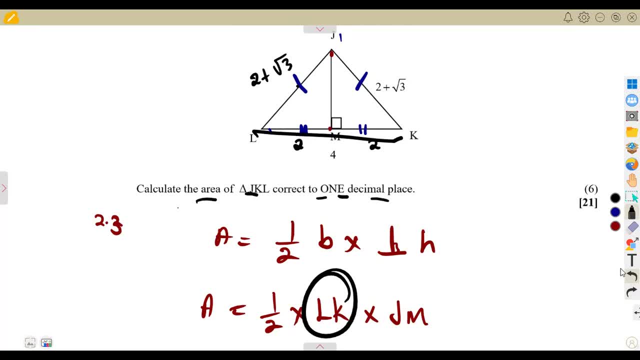 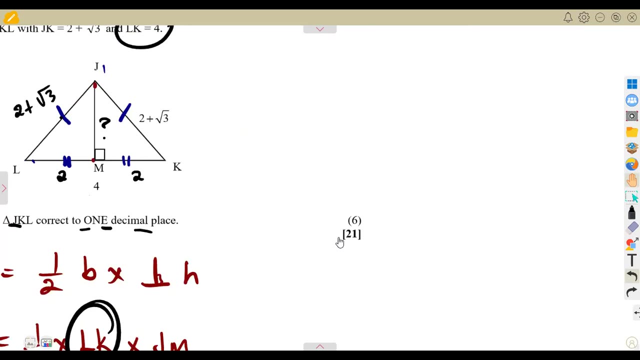 Okay, Okay, We have it as it is. from L to K is four units. What about J? M? We do not have. from point J to M? We do not have. So these, we are stuck, We are stuck. So what are we going to do? 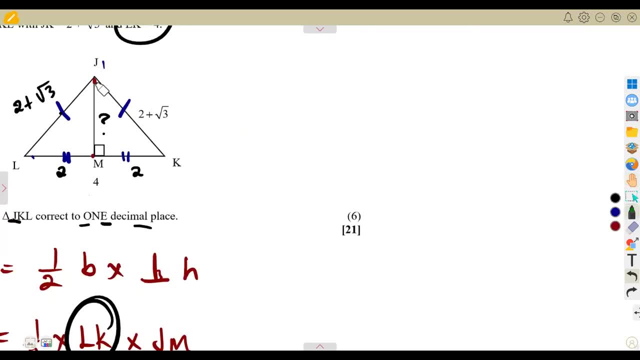 We are going to use the piece of this triangle because it's a right angle triangle, So we can use just the piece of this triangle to solve for the third side. To solve for the third side means to find that that side. This is our J, This is our M And this is our K. from M to K. 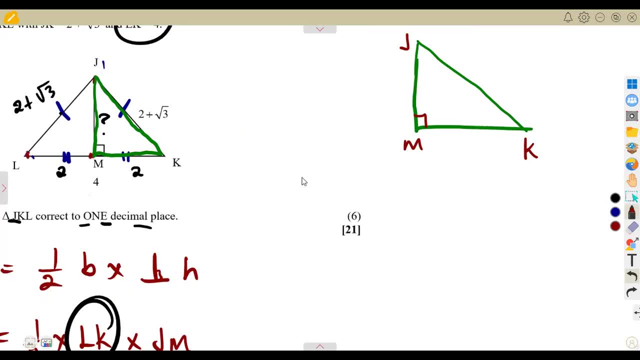 We say this is equal from L to M, which is going to be two units, And we are given two plus the square root of three, And this case is the hypotenuse, the one that is opposite or the one that faces the 90 degrees. 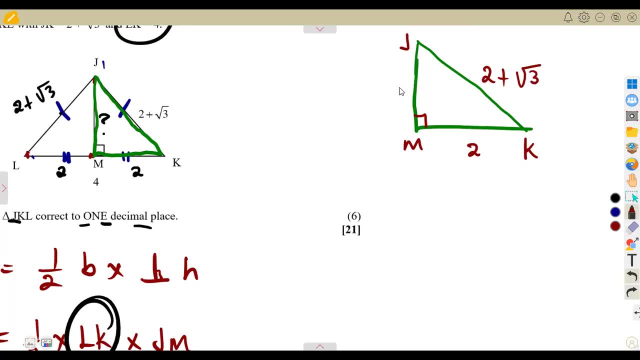 The one that faces the 90 degrees. we are supposed to solve for the third side, which is to calculate jm, how, using our pythagoras theorem, we understand that c squared is equal to a squared plus b squared, where c squared is the hypotenuse. so 2 plus the square root of 3 squared is equal to a. 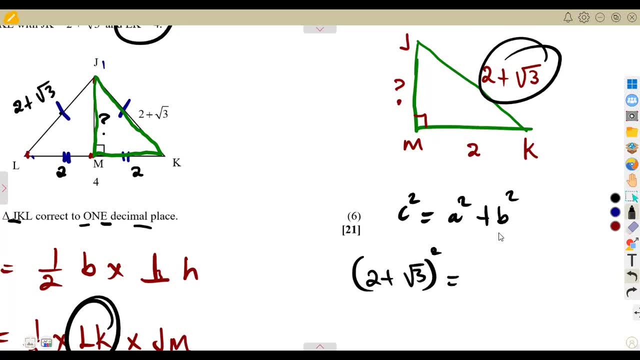 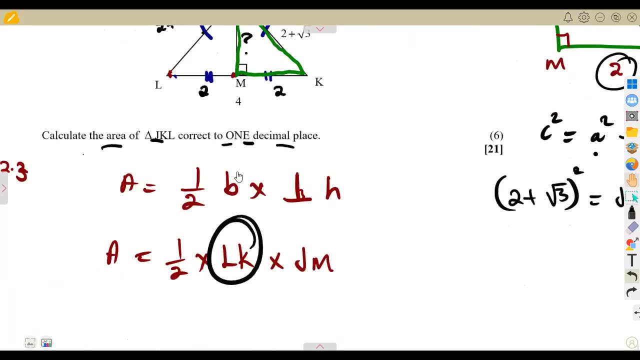 squared plus b squared, which is a and b are the shorter size that you're given. so you can write jm squared plus b squared, which is this side, the other shorter sides, by. just given that this area is supposed to be given to one decimal place, it is a clear indication that we can also work. 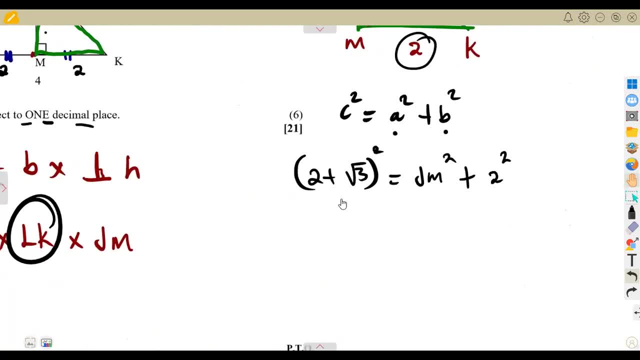 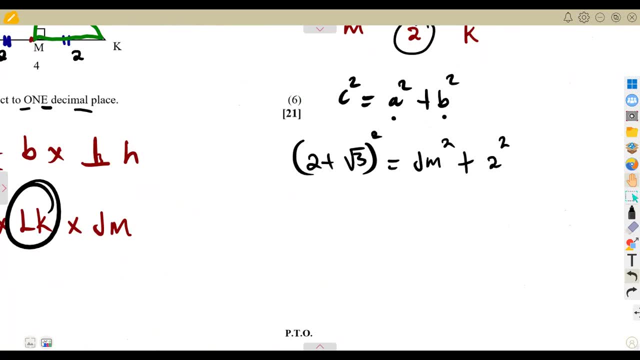 with decimals in our simplification. so if i am stuck in my simplification on this one, i can just use my calculator or i can expand. this is up to you all right. so if i am to use the calculator was most likely to be the best one. so if i am to use the calculator, i can just use the calculator. 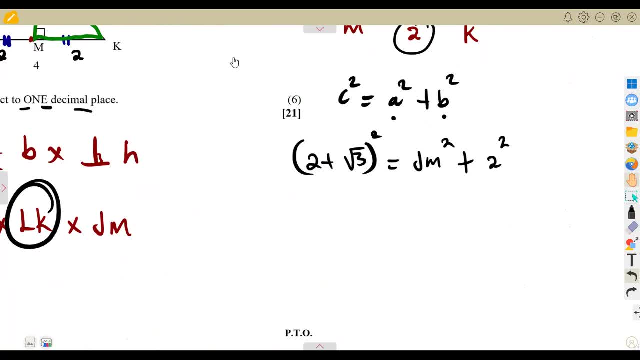 of us. we are used to this uh calculator concept, so let me just uh give this one so that we see how we're going to have on our simplification. so you are supposed to be very, very careful in this uh situation. you can just use your decimals, because already you're told your answer should. 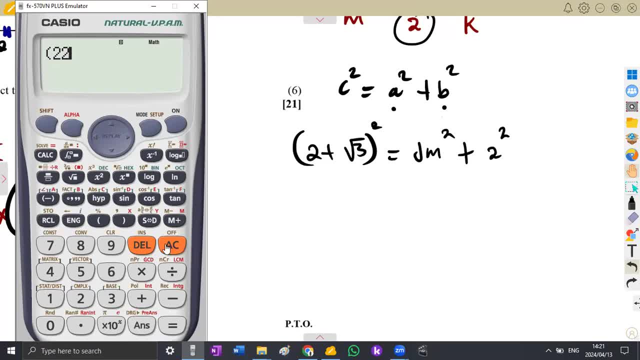 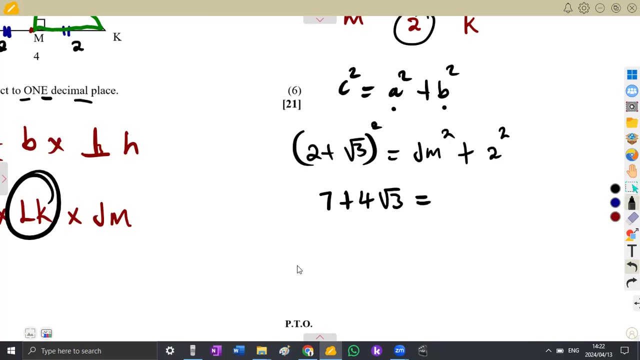 be two decimal place, so you can also use that two plus the square root of three in a bracket. then we square this all right, so this is seven plus four. you can even write it like that: all right, uh, seven plus four, square root of three, which is equal to what? uh, two squared. so two squared, that's a four. so it's going to be j. 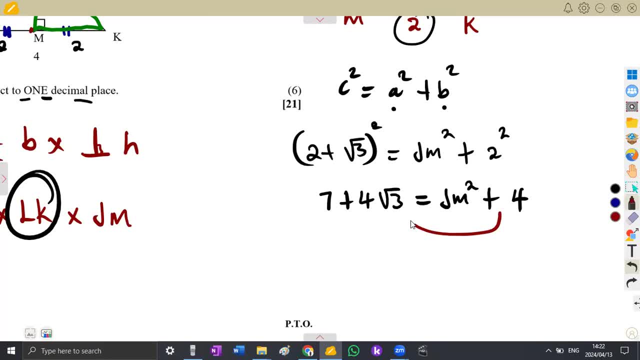 m squared plus a four. so transposing this four to this side, that is going to be a negative, okay, so meaning to say we're going to have seven plus uh four, square root of three minus a four, if we take it this side, which is equal to uh j m squared. so on this one you subtract the numbers, this one. 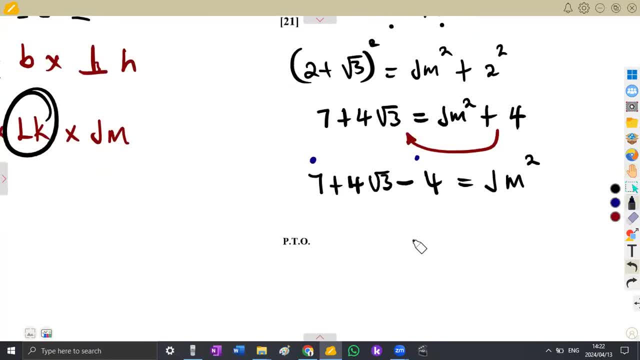 minus this one, which is going to be a three. seven minus four, that's three plus uh, four, square root of three, which is equal to j m squared. how do i remove the square? i have to introduce the square my j m. so j m is the square root of this. so you can even leave it like that as the square root. 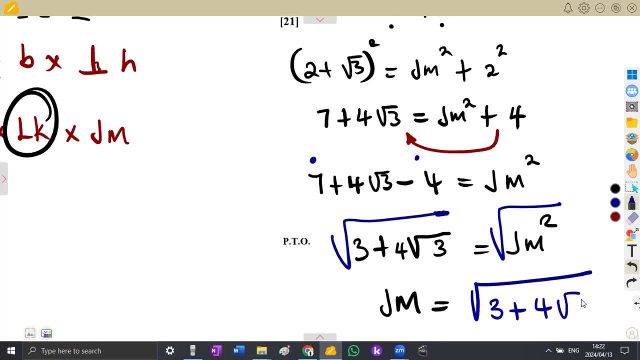 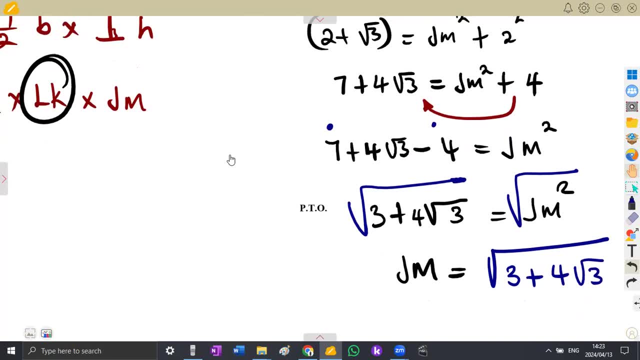 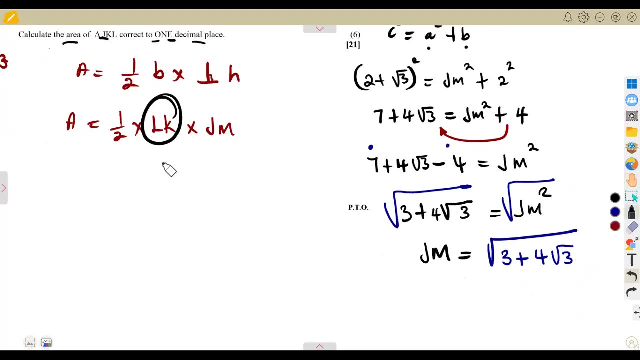 of three plus four, square root of three. uh, we're just gonna leave it like that. there's no, there's no effect at all. there's no effect. yes, you can use your calculator to have a decimal or just ignore, right, just ignore like that, it's fine. so this is our. j m just substitute him. uh, having this. 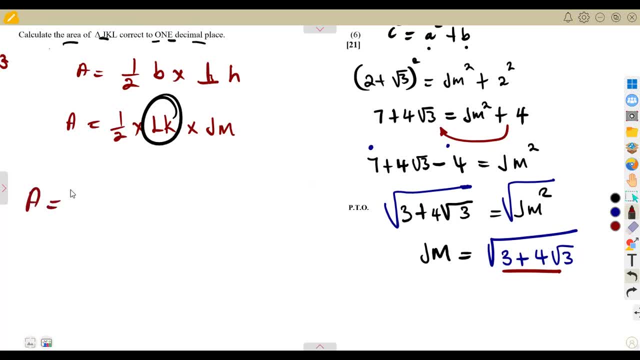 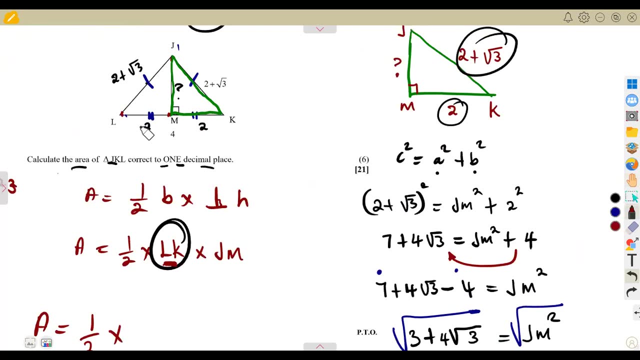 it means we are going to also have a, a better answer, because our answer is going to be executive value, because we never rounded off, so our answer is going to be the exact answer. so this is half of the best, which is l to k, which is the one that we have on our information. from l to k, that is two plus two, which is four units. 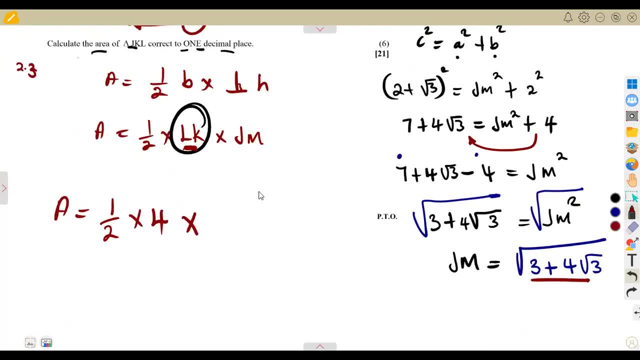 so we are going to have, uh, four units times jm. we calculated our jm from this and we saw that it's going to be the square root of three plus four, the square root of three. so it's just a square root under a square root. but do not worry about that, because the calculator is there as 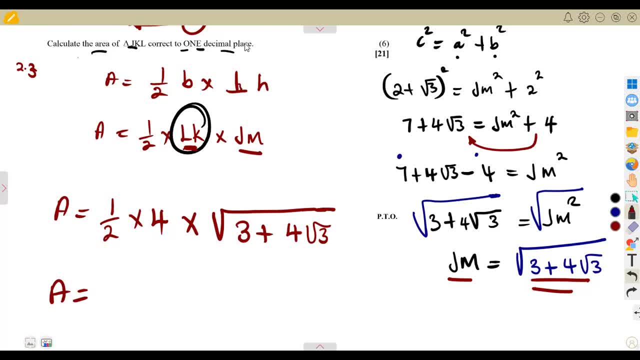 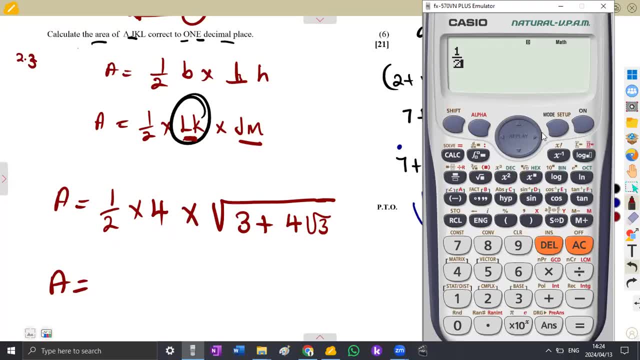 your assistance in this exam. uh, and also you are told to leave your answer to two decimal places. so that's an advantage. so meaning to say we are going to have one over two multiplied to four, multiplied to the square root of three. inside of you same square root, there's plus for the square root of a three. so this was going to give us 6.301. 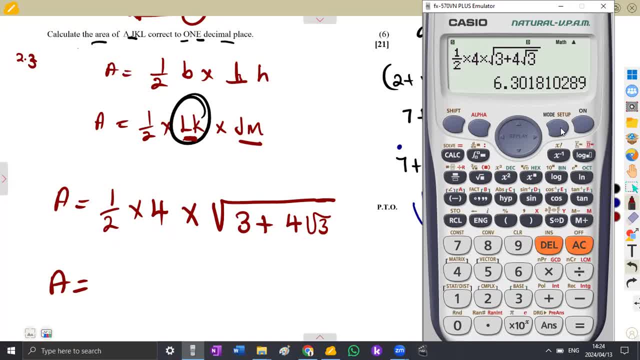 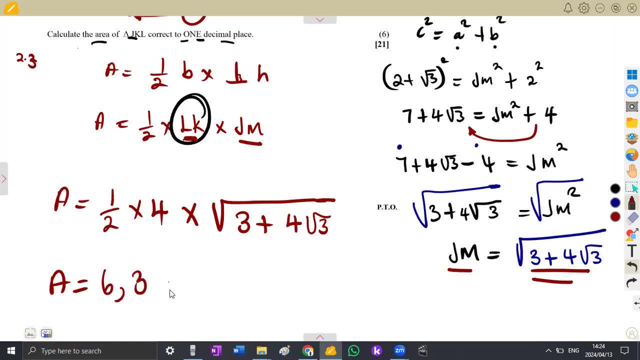 which is 6.3. if you do not know how to run off, just shift. you go to the setup. remember? you fix your calculator to one decimal place, since you're told to one decimal place, so this will be 6.3. so our area was going to be 6.3 square units or units squared, so that is how we could have. 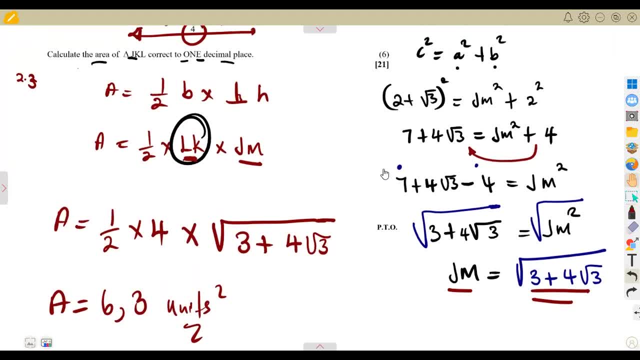 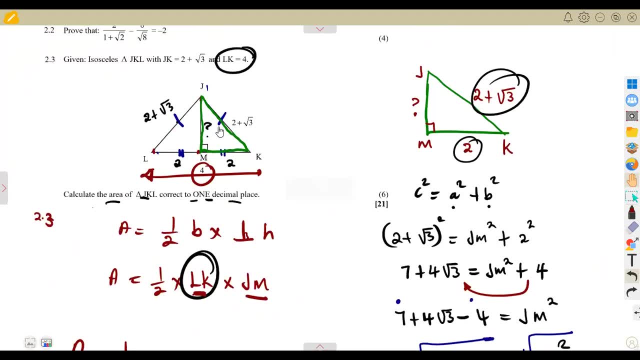 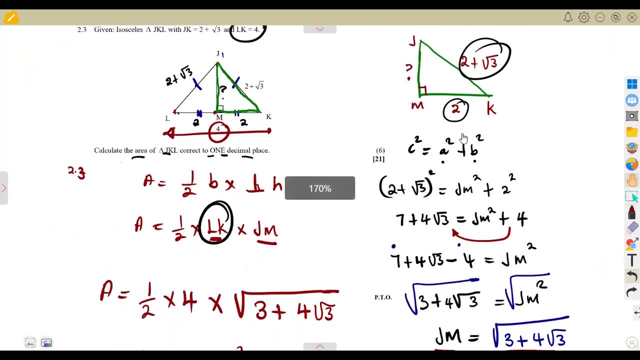 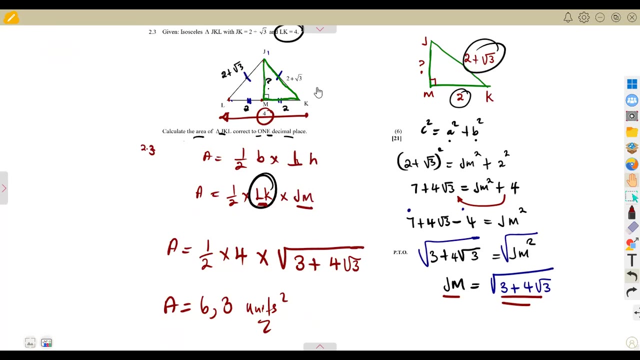 calculated our area. given this situation, you needed one. the idea of a right angled triangle concept, using the idea of a right angle triangle concept. you can use that. you can use that to calculate the area. given this situation, you needed one. the idea of a right to calculate the hypot. I mean to calculate the, the perpendicular height, without the perpendicular. 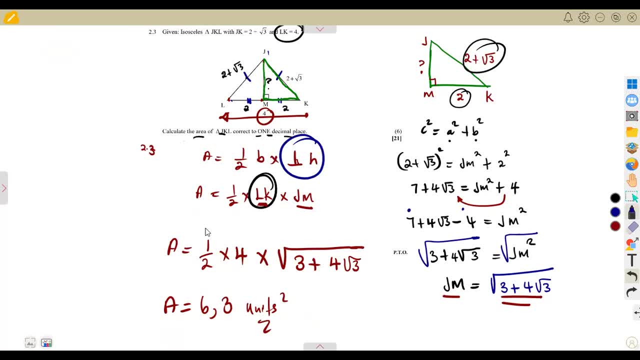 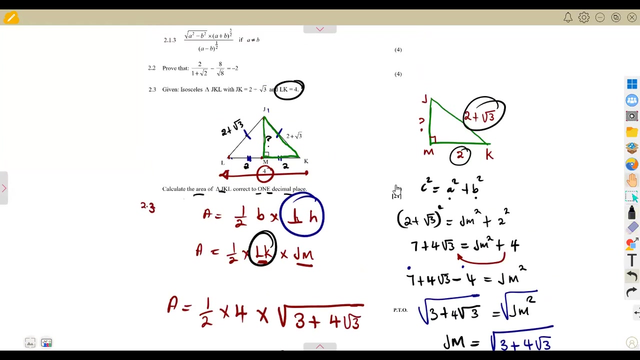 height. it was going to be difficult for us to determine this area, but with your perpendicular height, everything is easy. let's see what we have on the other. these are your typical questions. your exam is going to be like that, so this was actually 21 marks on question. 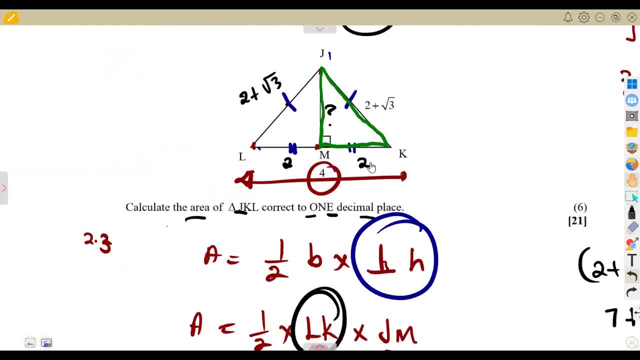 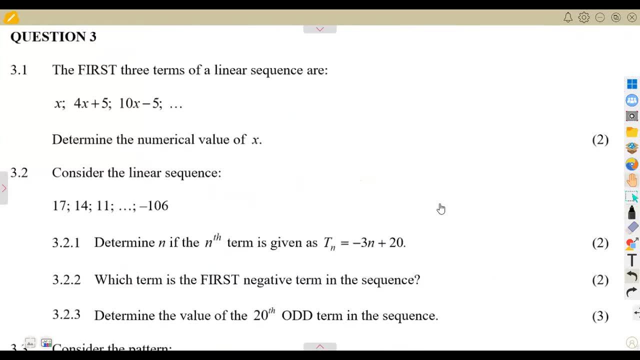 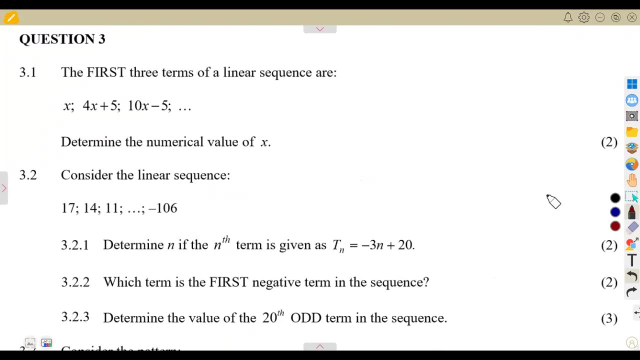 on the wall of our question uh 2, 21 marks. this is a lot in exam. you need to know your simple questions, those uh great 10 questions. revise as much as you can go to your basics. know your basics. question number three: number patterns. we are given a sequence. in that case, the first. 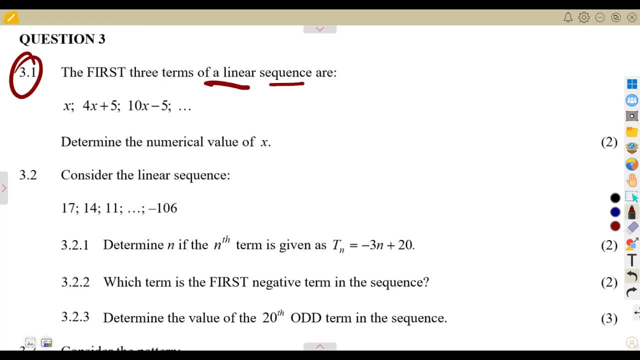 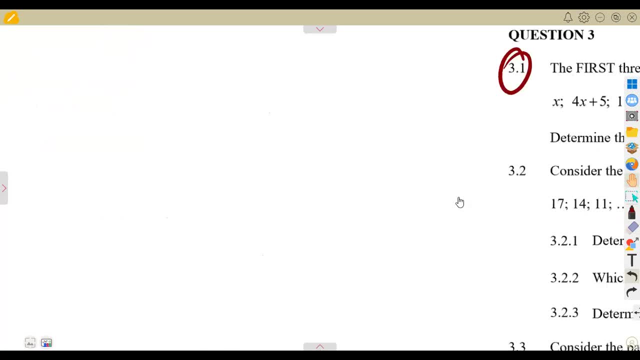 the three terms of a linear sequence are: these are the three terms that we have and we are asked to determine the numerical value of x, 2 marks for that, given these terms that we are given and we are told that it's a linear pattern, given x, uh, given 4x plus 5 and also given 10x minus 5 and 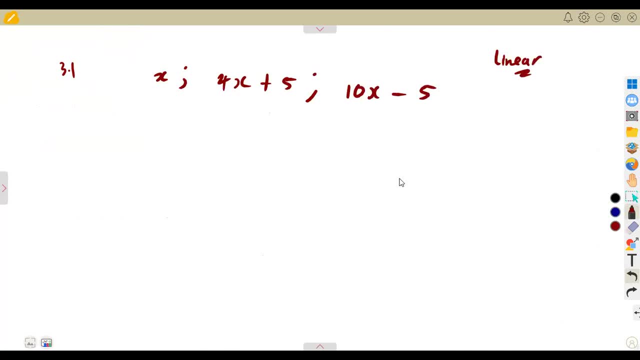 this is a linear sequence, where we know that in a linear sequence there's something that is very, very common, which is the difference. you work with the common difference. we know that this common difference is the same: t2 minus t1, second term minus the first term, third term minus the second term. it is the 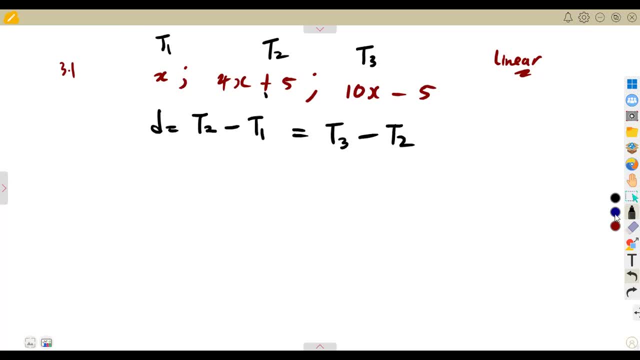 same throughout. so if it is the same throughout, let me find this and equate it to this, so i can formulate it as an equation: t2 minus t1 is so your t2 is what 4x plus 5, which is subtracting t1. t1 is just a term, just a single term. it's x. so, guys, 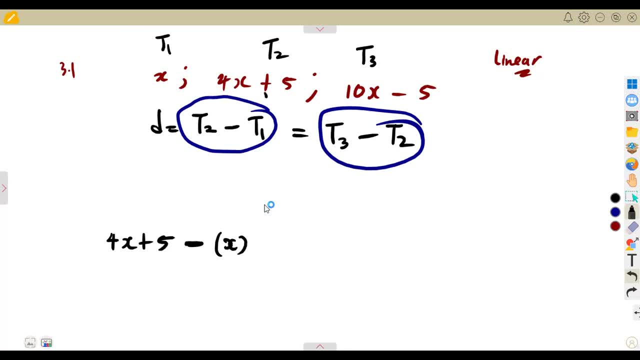 there's no need for a bracket there. but if you want, just do that. this is equal to t3 minus t2. what is our t3? our t3 is 10x minus 5 and it is subtracting t2. and our t2 is what? 4x plus a. 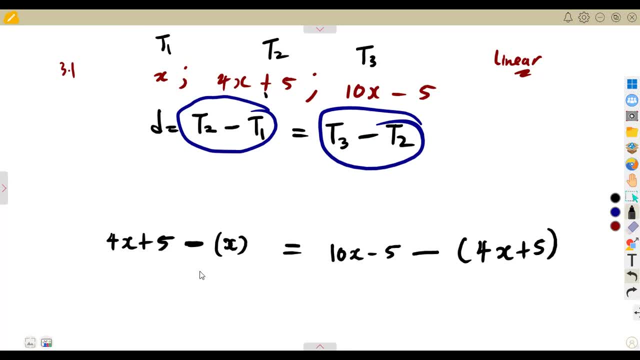 5. heck, not know your formulas. all right, so let's subtract: this is just 1x there. so 4 minus 1, that's going to be 3x plus 5 is equal to 10x minus 5. expand your brackets by negative 1, that is negative. 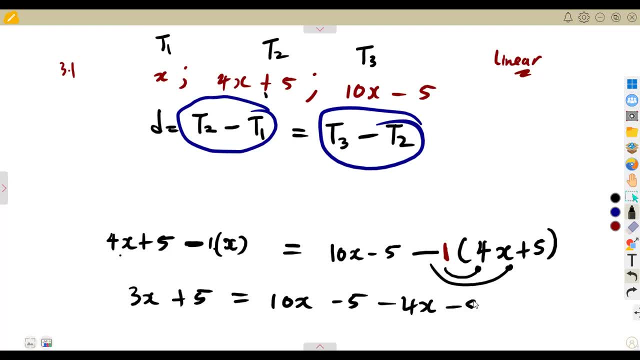 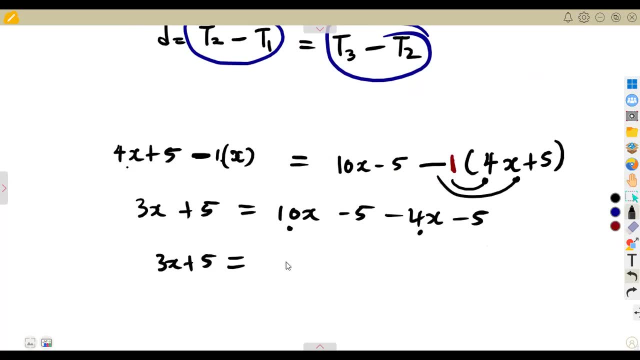 1 times 4x negative 4x times this, that's a negative 5. so if you were to collect your terms, this was going to be: 3x plus 5, is equal to 10 minus 4, which is 6x minus 5. 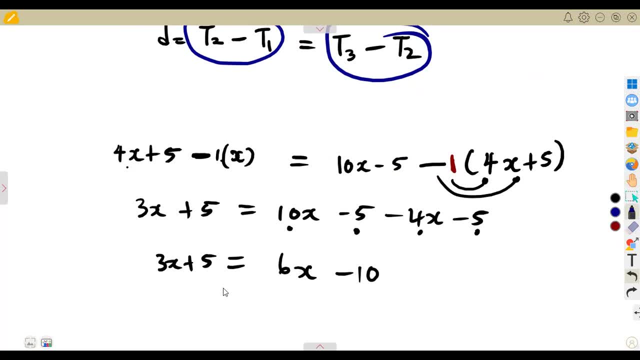 that's a minus 10. so collecting the terms of x to one side of the equation is up to you which side you want to work with. you can move these terms 3 to the other side, then 10 to this side. it means we are going to remain with a positive 5 plus a 10. it was a negative, so it's going to. 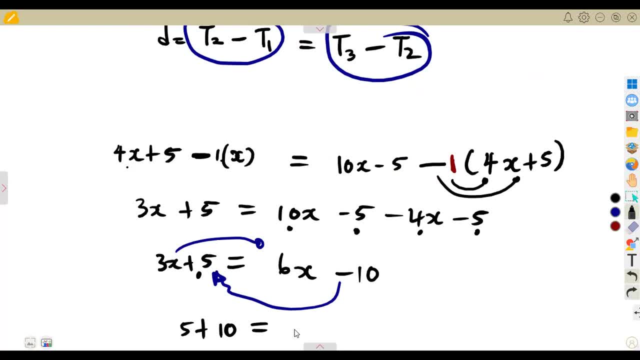 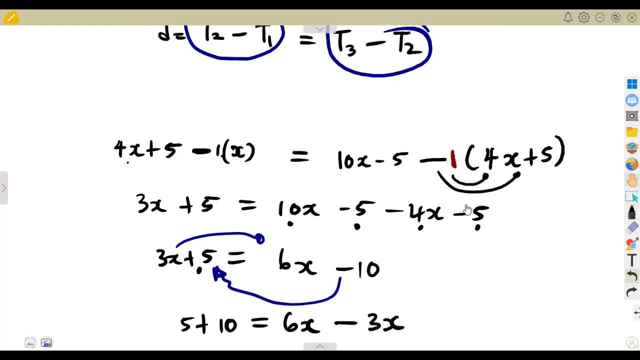 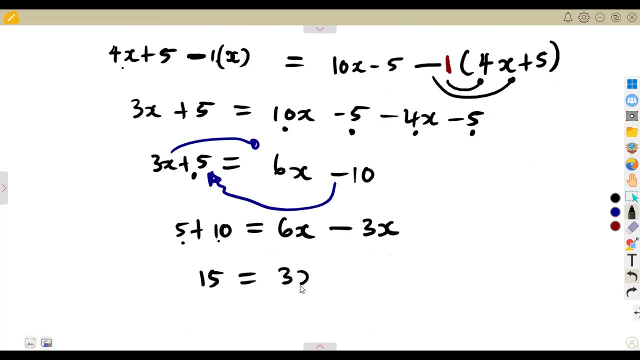 be a positive. 6x is already on the right hand side, so if you transpose the 3x it carries a negative. it was a positive, so on the other hand, it will be a negative. 5 plus 10, that is 15, is equal to 3x. it's a multiplication, so just divide by 3, by 3. 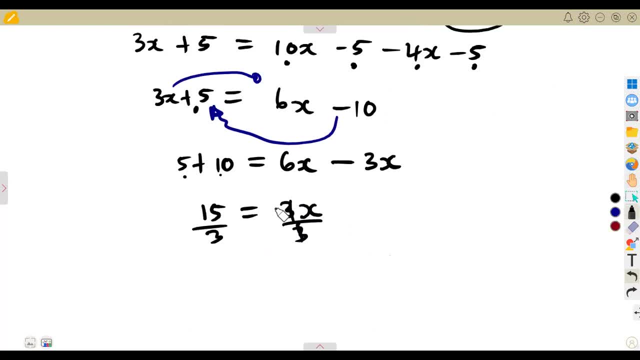 so meaning to say, if we divide by 3, that's a 1. on this case, so x is what 15 divided by 3, which is a 5. so in this situation, you are going to have your x as a 5, which is the numerical value. 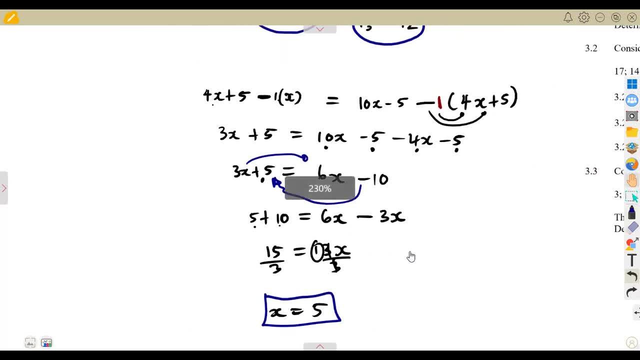 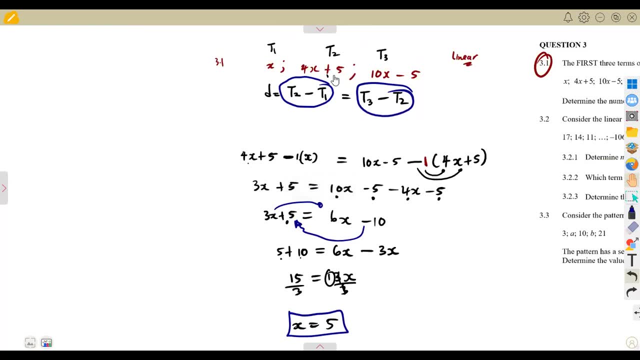 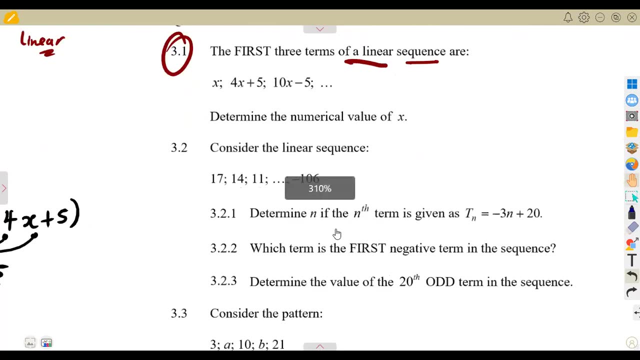 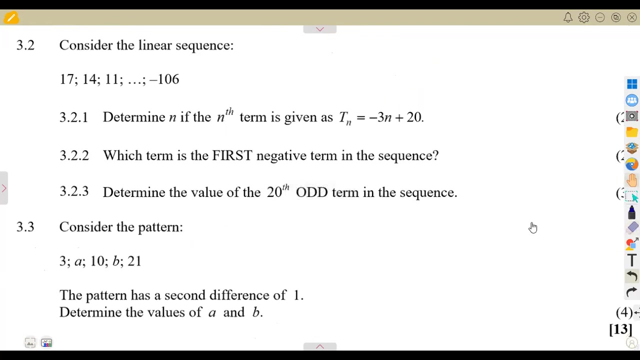 the numerical value. they want to know what is your x, the number, the number that corresponds before. these are expressions that we have all right. so that is, uh, the value of x. just so for x, all right. 3.2. consider the linear sequence is another question on it's on this one. consider this sequence, not another sequence, but this one. 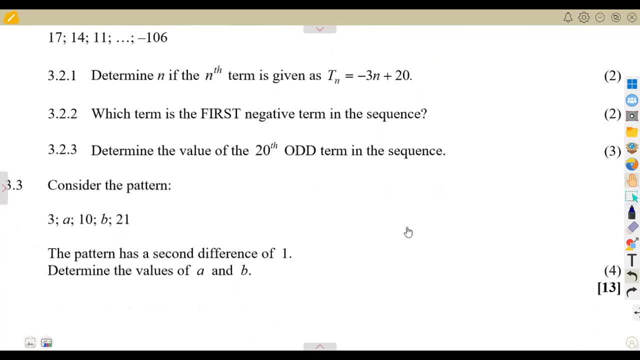 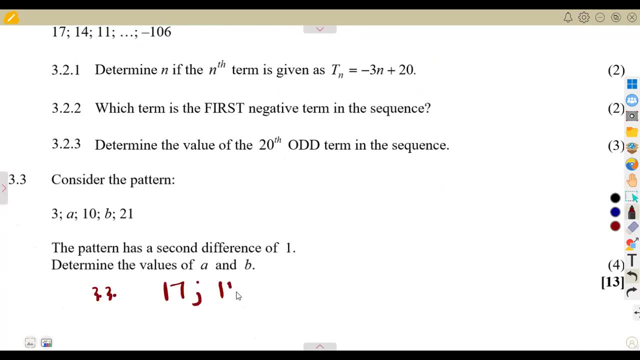 uh, that we are given as 11. it's a linear sequence, take note. all right, so that's our 3.3. we are given 17, uh, 14, 11, and so on and so on. they are saying there are so many values there, not to say there are three values. no, there are so many. and so on, all right up to the last one. 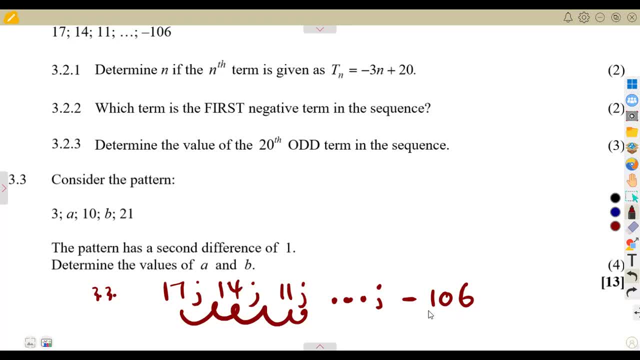 so this is an indication. we are going to continue with this up to a value when we have got minus one. so remember it was going to be up to minus 106. that was going to be the case. so the question is: determine the nth term, if the nth term is given. 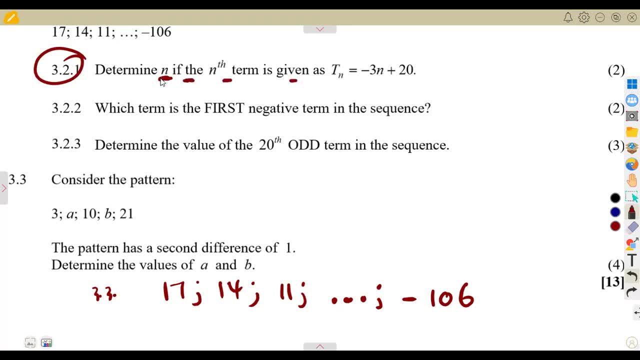 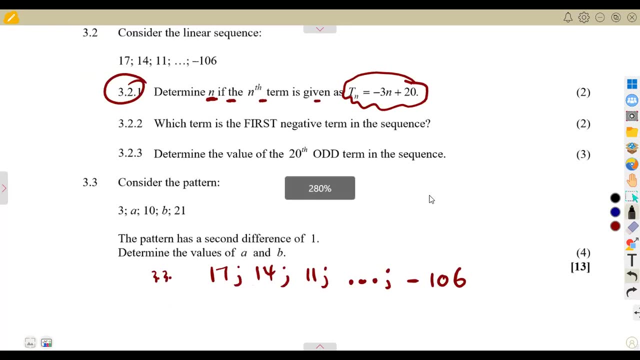 as sorry. determine n. determine n, n if the nth term is given as so we are already given. remember, this is a linear pattern. you're going to use uh, the common difference, this, and that you determine your expression, uh, tn, from the formula. remember, your tn can be written as a plus n, minus one times d, or you can use that uh written concept your tn. 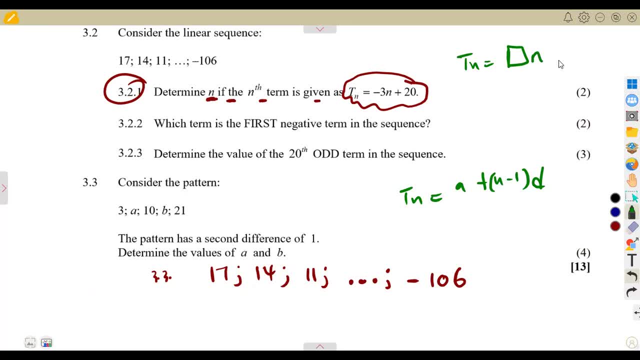 is gonna be: uh, the difference times n plus a certain value, where this one represents what the common difference. and to find this, you use any given point. at the end you're going to have this. so they already calculated that for you, they. they already calculated this for you. 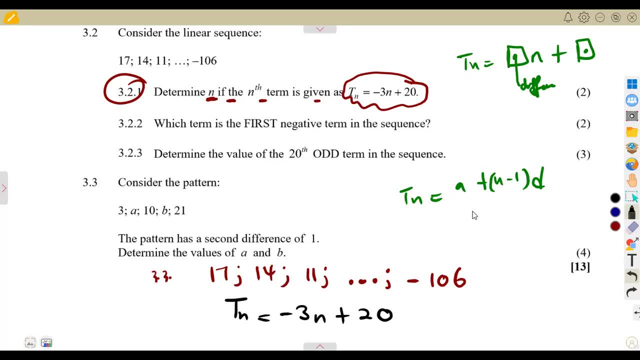 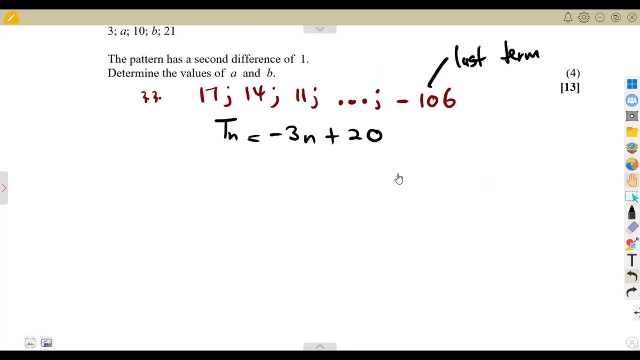 so you are not going to recalculate. no, it's a continuation. determine n. why are they saying so? because this time we are given a special term which is the last term. in most cases they don't even give you this last term, but there they gave you why. it represents that tn is equal to the last. 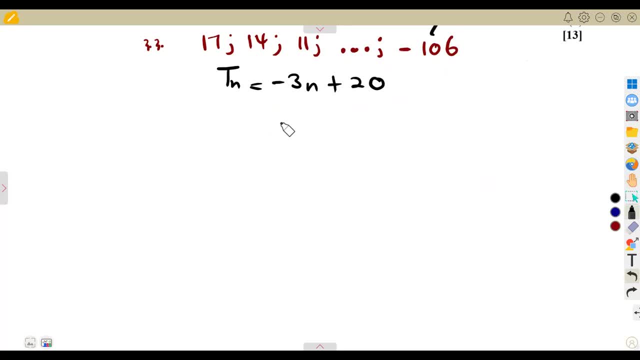 term in the presentation. so if tn is equal to the last term in the presentation, then it is equal to the last term. it means minus 3n plus 20 is equal to minus 106. tn is equal to the last term, so therefore this is equal to this. if it is like that minus 3n is equal to, we transpose this to: 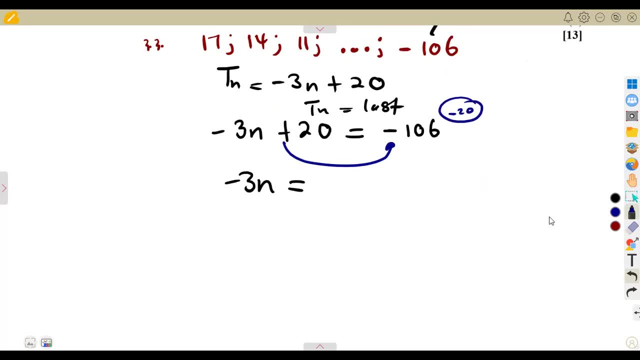 the other hand, it becomes a negative. what a negative. 20. it was a positive there. minus 106. minus 20, it's minus 126. so dividing by negative 3, by negative 3, it means our n at the end was going to be a 42. so this is our n. 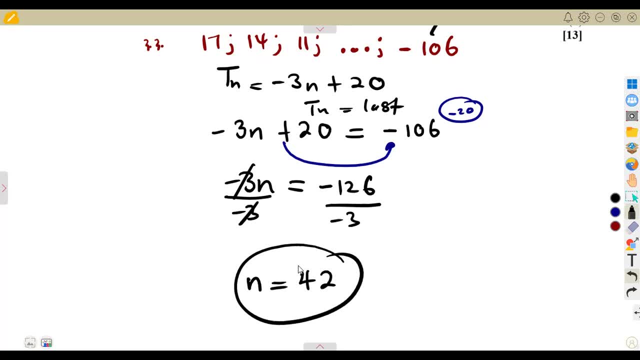 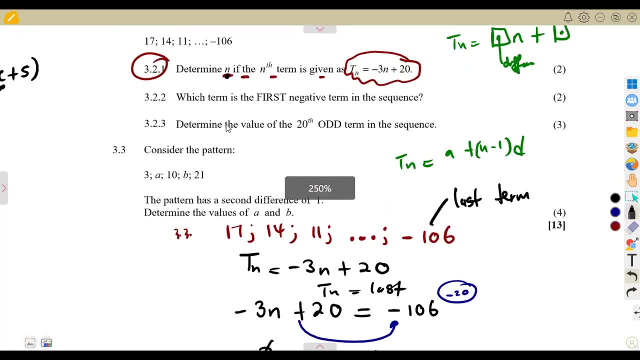 that is what we're given. we have the last, so you use the last term, all right? 3.22. which term is the first negative term in the sequence? which term is the first negative term? so this one, it's- uh, it's up to you. maybe you have got patience. 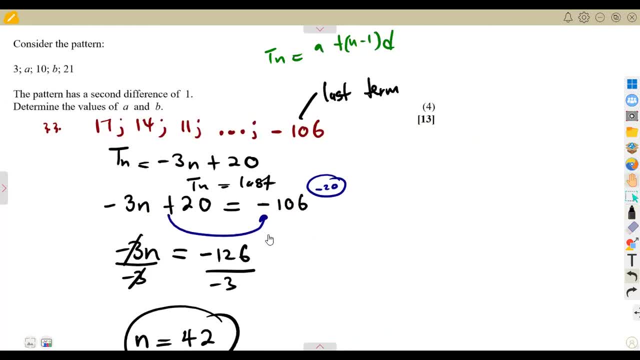 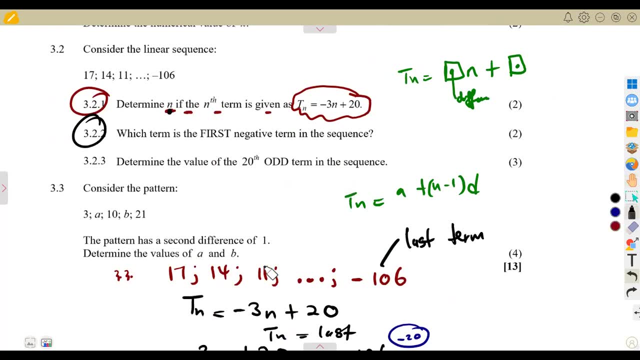 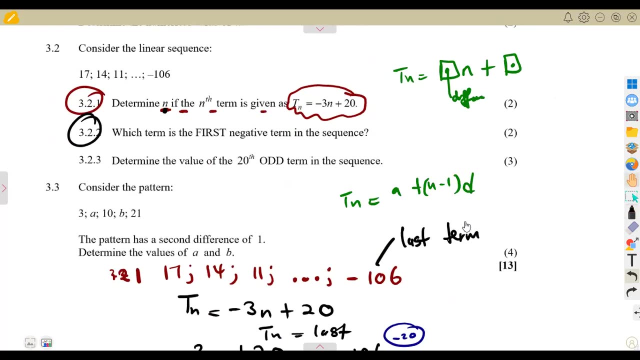 if you have patience in your calculations, this is what you're going to do. i'm going to show you two ways. so this is 3.2. uh, sorry for that, this was 3.21, 3.21. then we move on to 3.22, so 3.22. they are saying that we need something. 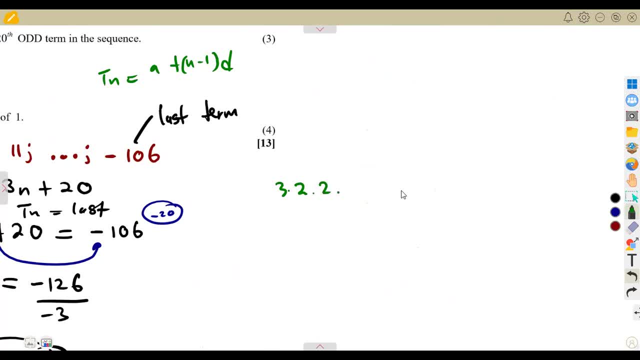 something. so this is 3.22 and we've got a number 3.22. we need n plus dot and this means we have in this long term, in this number 3.22, we need the first negative value, not not the first negative event actually, but 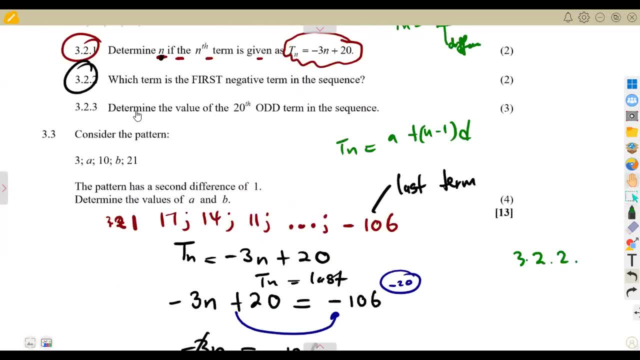 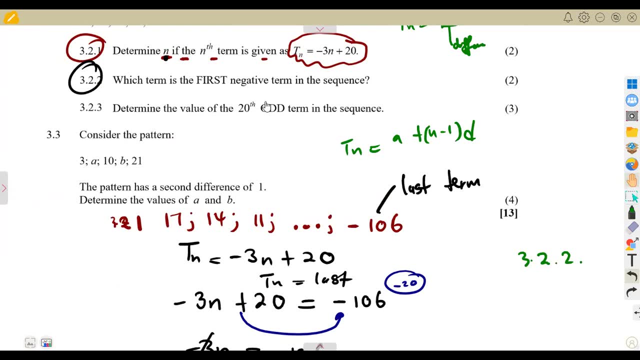 like: on which term are we going to have that first negative one? on which? what is the end? which term is the first negative term in the sick? which term not the first negative, but which time, like if you're counting one, two, three, four and so on. so if you've got patience, you're going to write these numbers, because if you're going to profit, give me a. 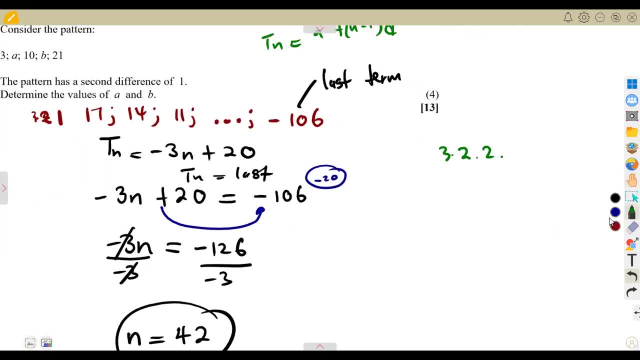 plus in and Tin好像. If we check here, this is 17.. There is a difference throughout. here There is a common difference. Remember how do you calculate your D: T2 minus T1,, which is 14 minus 17.. 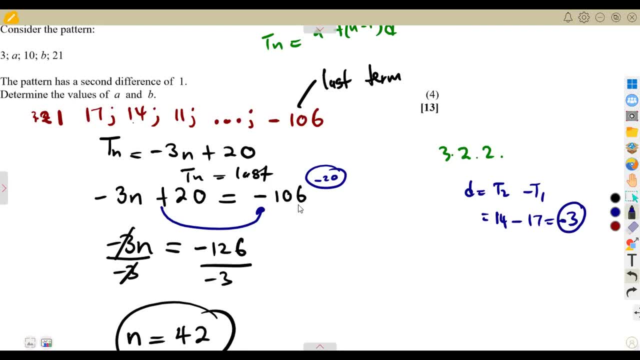 That is going to be a negative 3.. So, meaning to say each part to get the next term, you were adding the difference of minus 3.. On this one, you add minus 3.. On this one, you add minus 3.. 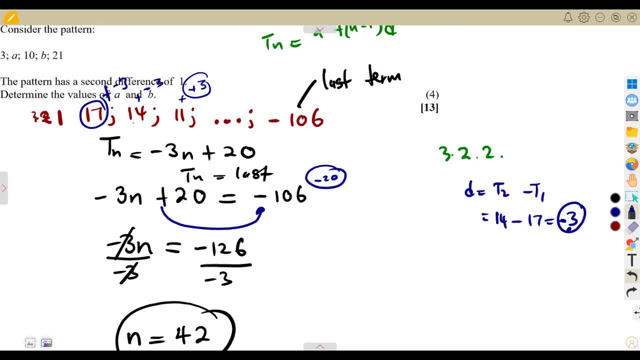 On this one, you add minus 3.. So on 11, if we add minus 3, what are we going to have? Okay, let's go back to our calculator. Let's get back to our calculator here. So this is it. 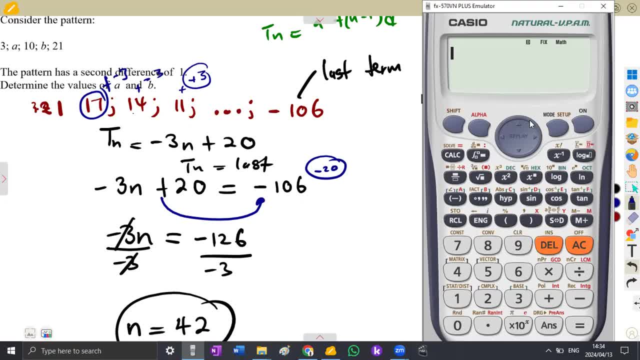 Remember our calculator before we fixed this. So let's just go back to the normal mode. So we need the normal mode 8, then press 2.. So this is what I'm trying to do. This is what I'm trying to say. 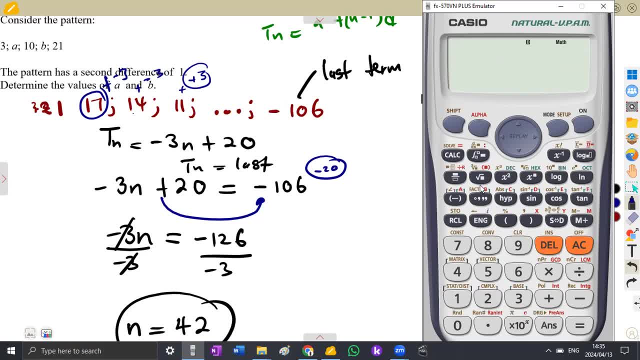 You add this, you're adding a minus 3 there. So it's 11 now plus a minus 3.. This is what we have. You add a minus 3.. This will be 8.. Meaning to say the term that is following here is 8.. 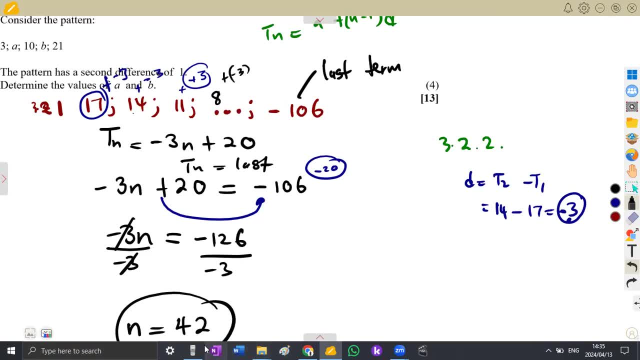 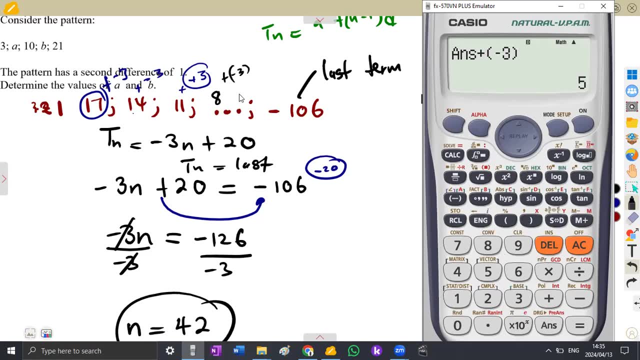 You add again a minus 3 on that 8. So you add a minus 3 on this number until you get the next one, Until you get the next one. So you get what A negative That's a 5. You add a minus 3.. 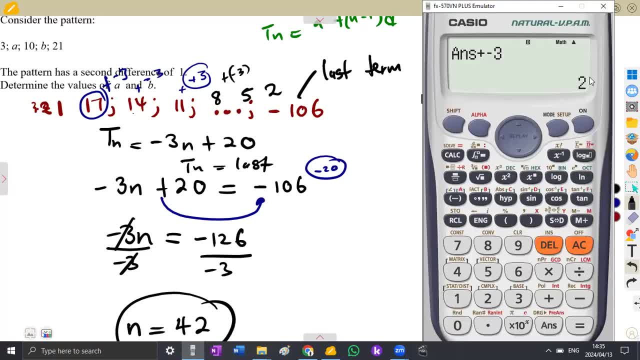 That's a 2.. You add a minus 3.. We are still on positive values. So if we add a minus 3, I want you to see here We get if we add okay. why is it delaying now? 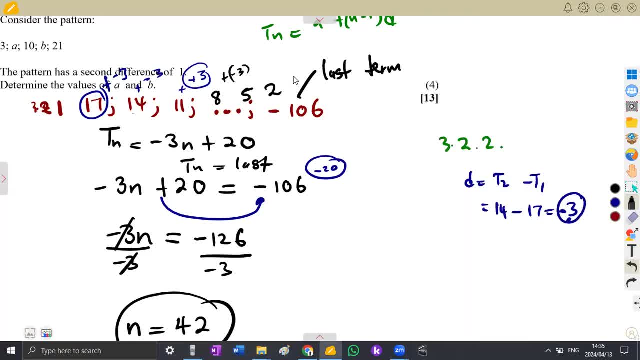 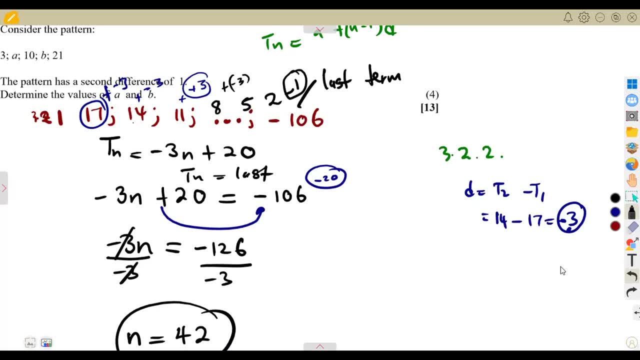 That's a negative 1.. We get a negative 1, and that's a negative. this one We are getting. what A negative That's where. that's our first negative number. this one, The first negative number, is going to be minus 1.. 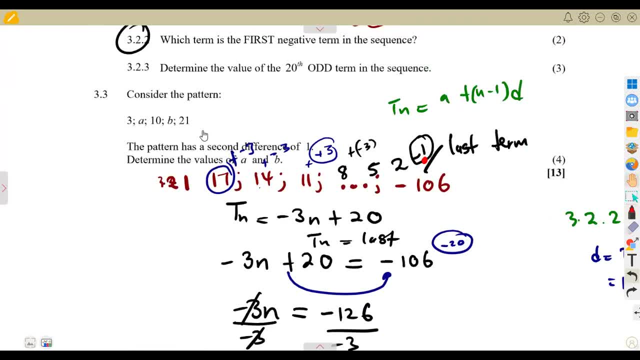 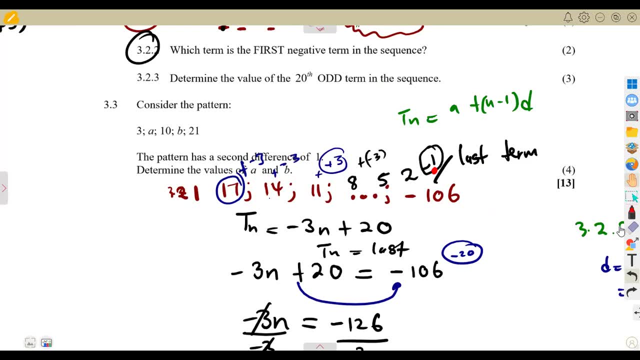 But the question is not asking us about the first negative number, no, Which term is the first negative term? Which term will correspond? So we count now: 1,, 2,, 3,, 4,, 5.. 6, 7.. 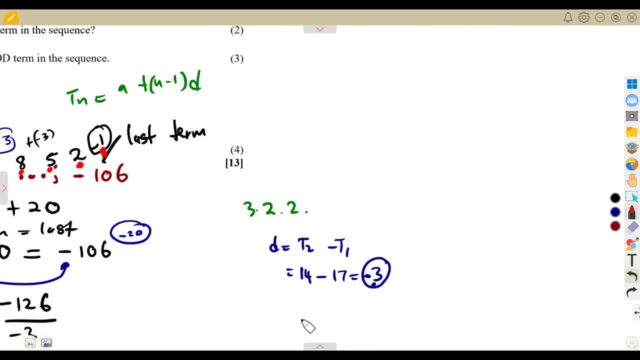 So it is the 7th term. So n is equal to 7.. We are talking about what? The 7th term, The 7th term, What is, or what could be another way, if I do not, maybe there are so many numbers. 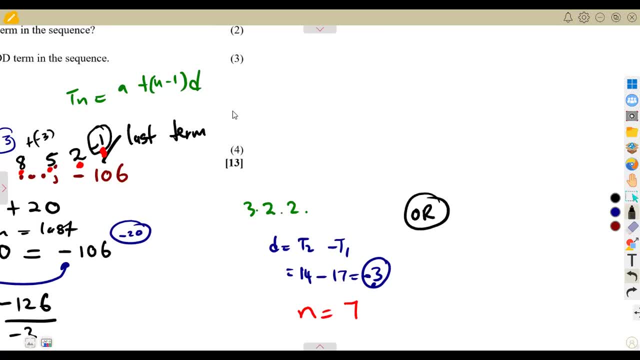 and now I have to just imagine, if you are adding, maybe there are so many values, It was going to be too much. So this is it. They are saying we need a condition when the first term is a negative, So it means that term- remember, Tn is the one that represents the term. 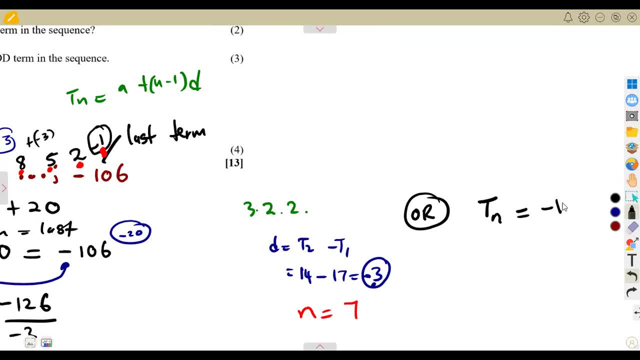 And the term is negative. So it means Tn is supposed to be equal to a negative value. So any negative value means values that are less than 0.. We do not know that value. Is it going to be minus 1?? So we can't say it is equal to minus this. 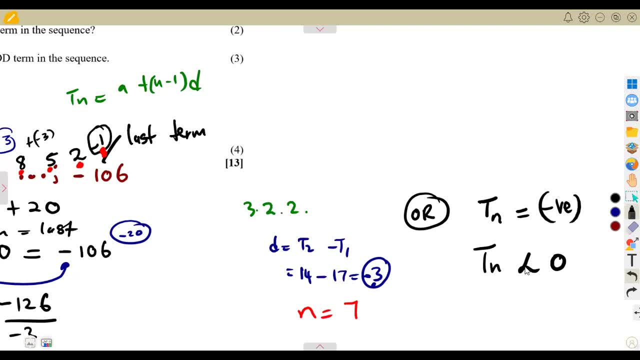 But we know to be negative means the value must be negative. To be negative means it must be less than 0. I mean to be less than 0 means a value is negative. So if Tn is less than a 0, and we have that Tn, we are given an expression. 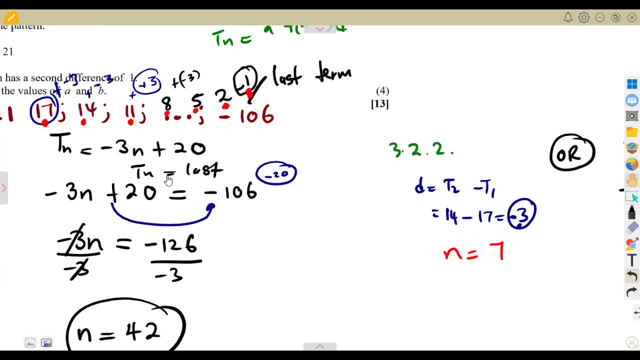 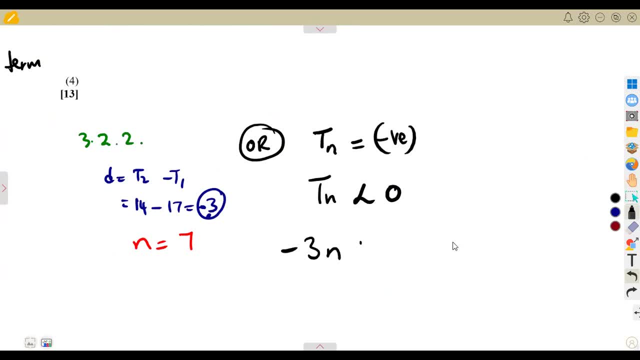 For Tn, remember minus 3n plus 20.. So we take that now, In terms of n minus 3n plus 20 is supposed to be less than a 0.. We solve: Minus 3n is less than remember. this is a linear inequality. 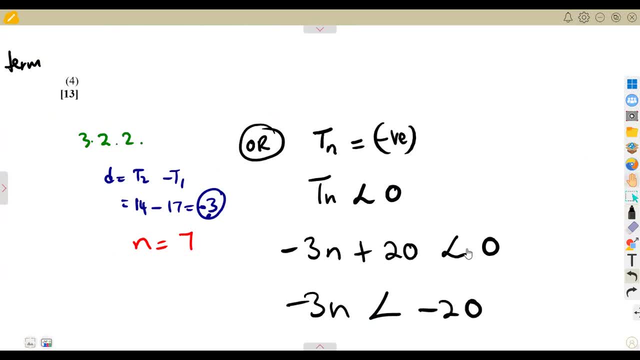 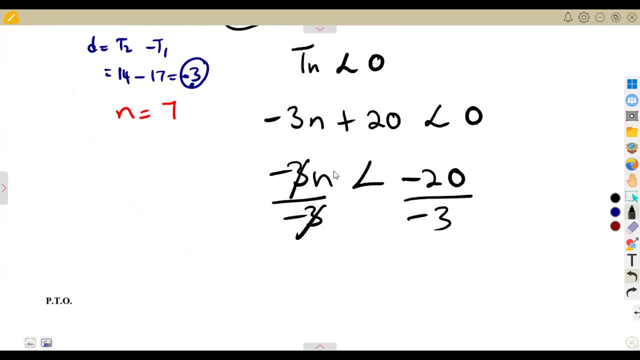 So just transpose this: It becomes a negative 20.. On the other hand, how do you find n? You divide by a negative 3. The moment that you divide by a negative under inequalities, you are going to reverse, to change the inequality. 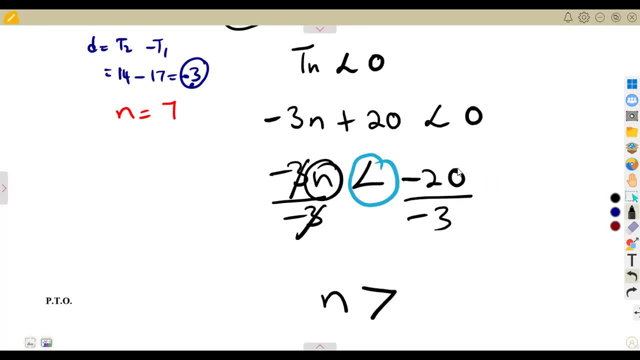 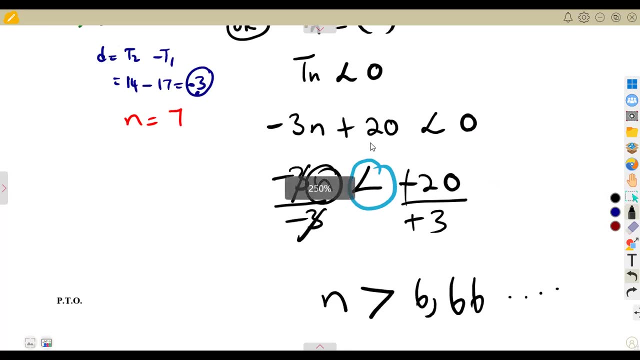 So it means n is now greater than 20 over 3.. And 20 over 3 has a decimal, a 6,666, something like that. So it means our n to have or to give us Tn as a negative number. 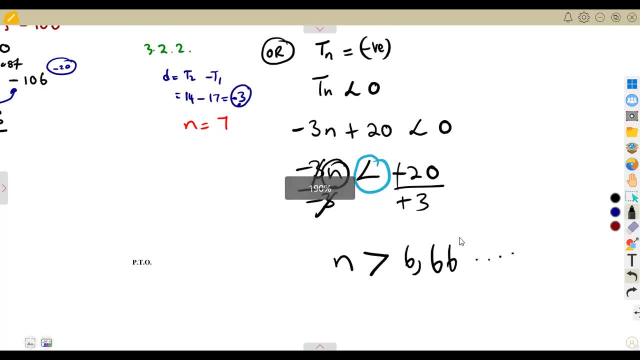 n must be greater than 6,666, and so on. So which whole number? because n is numbers. like which number are you talking about? And it's a whole number. So which whole number do we have just after 6,666 and so on? 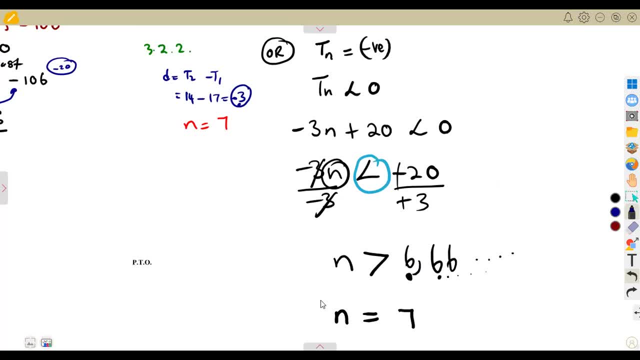 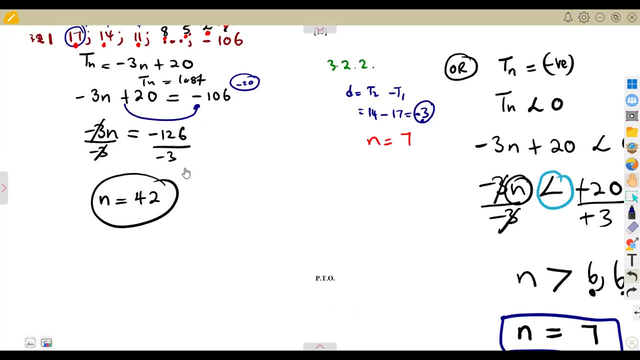 The whole number that follows is 7.. So n must be equal to 7.. So you could have solved this. from where? From this, From this inequality concept? there are so many ways, so many ways to consider, so many ways to consider. 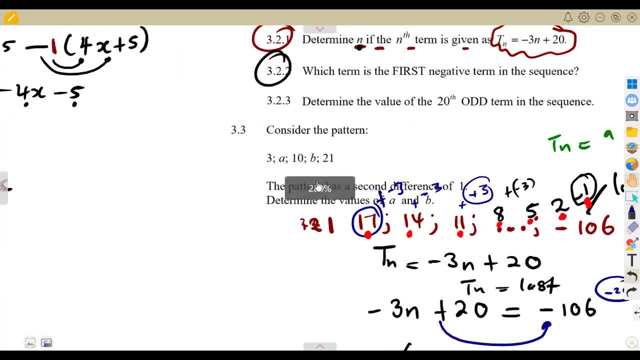 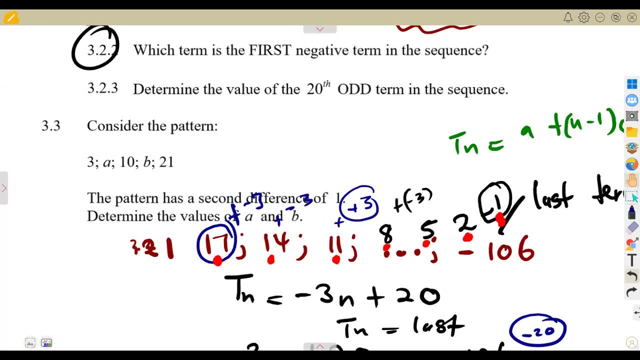 All right, Determine the value of the 20th or determine in the sequence, the 20th. but, guys, let's be, let's, let's, let's understand, Let's be mathematical When answering questions. determine the value of the 20th. 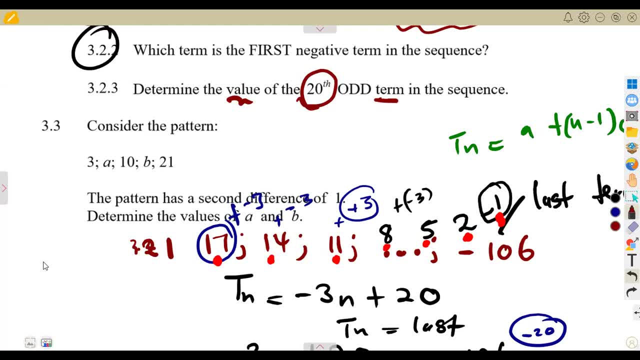 Not just a term. No, no, no. If they wanted a term, they were going to write, but they even wrote this in upper caps. I mean to show you that it's no longer what you have. This one is for odd terms. 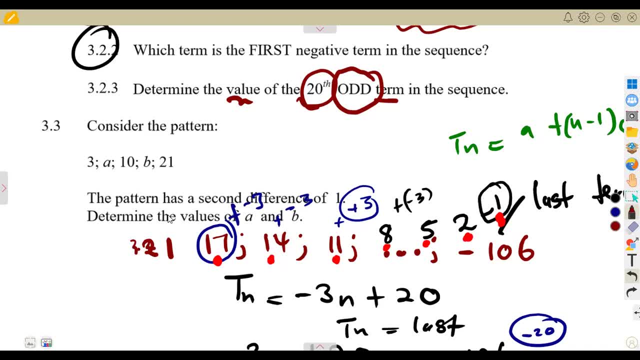 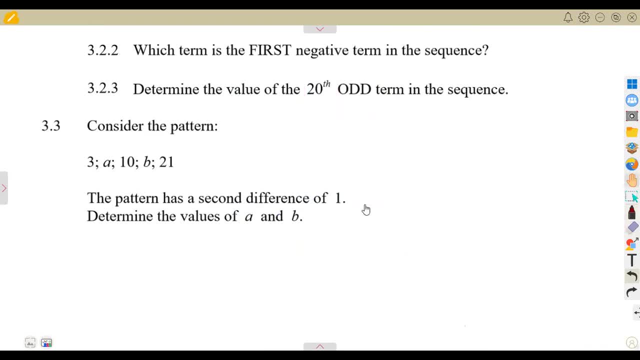 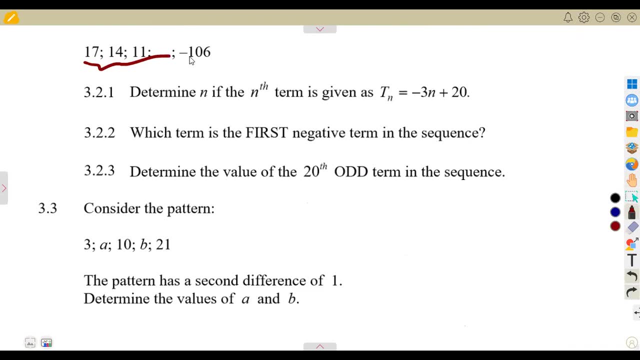 Odd, odd, odd terms, odd terms. So the question is: what is an odd number? So the question is: what is an odd number? So this here it was TN, not for odd numbers, but for everything there: crime numbers, odd numbers. 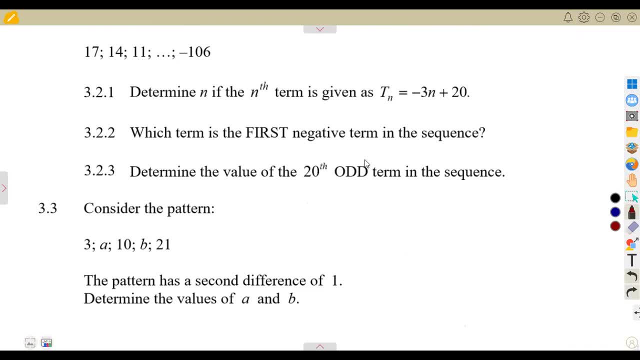 everything is there, But now it must be of odd, odd, Odd numbers. These are numbers. when you divide by two, you're going to have a remainder, always a remainder of one. You divide by two, You have a remainder of one. 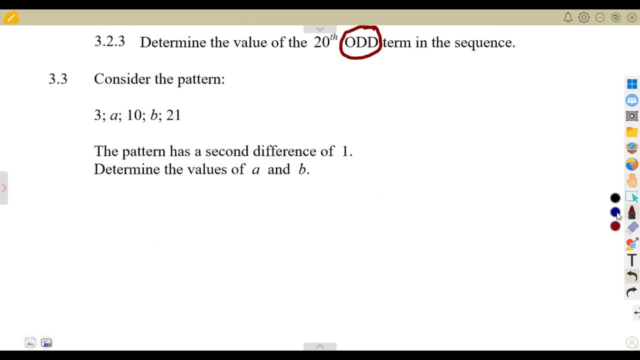 These are your odd numbers. So what are we talking about there? On odd numbers, when you divide by two, you have a remainder of a remainder of one. Let's talk of one, three, five, seven and so on. These are odd numbers. 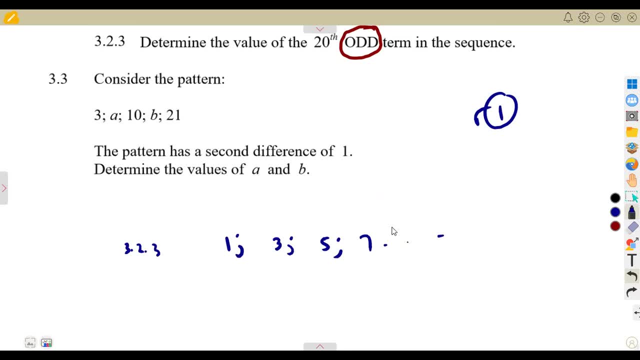 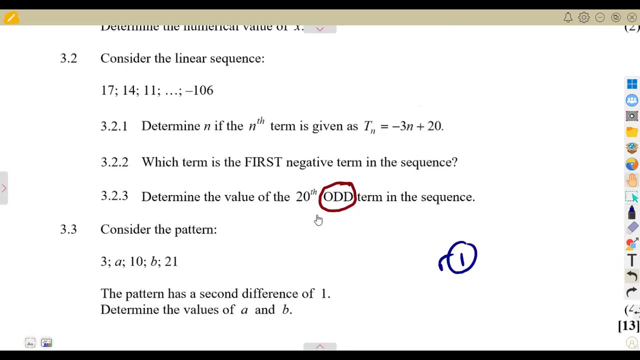 Yes, some prime numbers are odd numbers, Some prime numbers are odd numbers, but as we are focusing on odd numbers, we are focusing on odd numbers. So it means we were supposed to create a sequence of all the numbers, This sequence that we are having- 11,, 14, that we were given before. 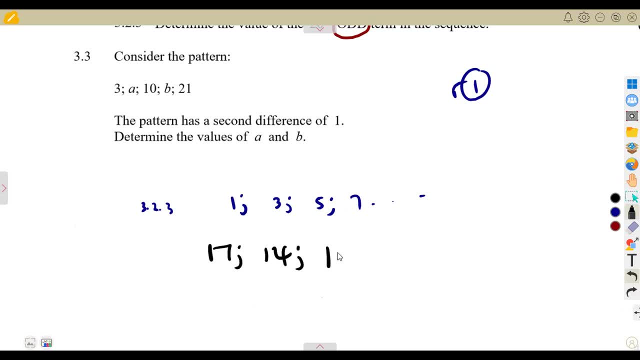 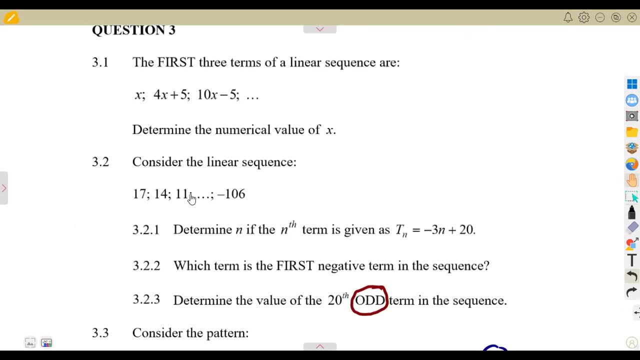 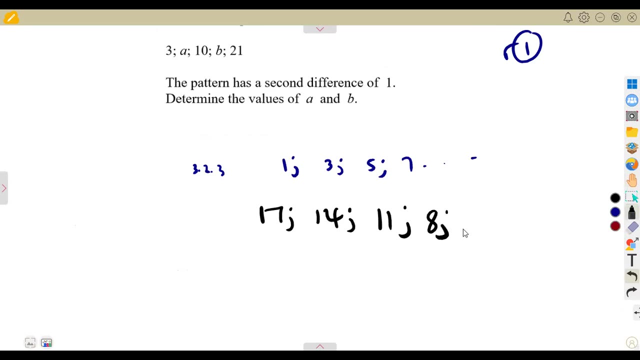 it was 11,, 14, sorry- 17, 14,, 11, 8.. Okay, remember, when we added those numbers, when I added those numbers, we got eight. And when we added, we added minus three, we ended up having five. 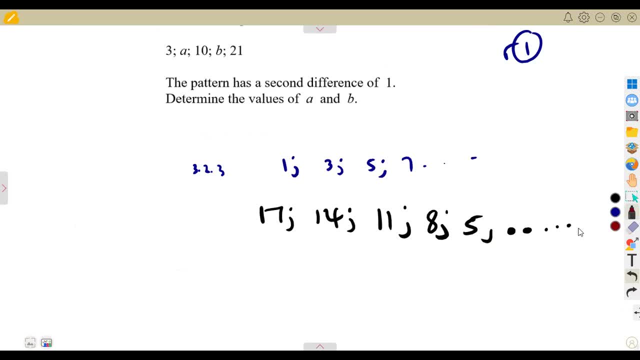 Remember when I was adding those numbers and so on, and so on. This is the sequence, the original sequence. On this sequence that we have, you plug out odd numbers in that manner or order that you are given. You plug out the odd numbers to form a sequence of odd numbers. 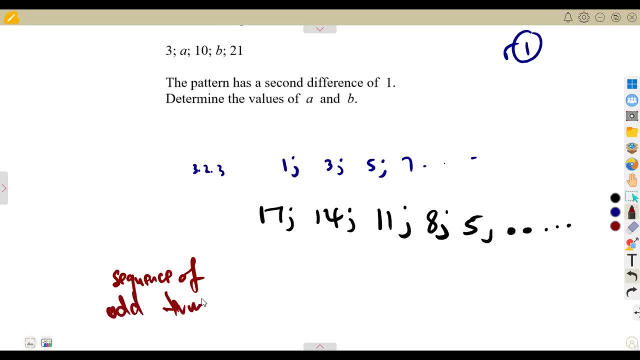 Because it must be of odd terms, odd numbers. so we must have a sequence of what Odd numbers only Only. If they wanted to talk about even numbers, you form that one for even numbers only. So which odd numbers? It's now a new sequence. 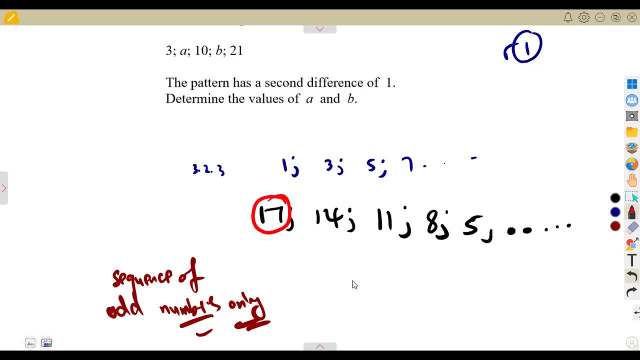 17. is it an odd number? Yes, we divide by two. There's a remainder of one there. So as long you divide by two and it's not exact, That's an odd number. So 17, 14, 14 divided by two, that's a seven. 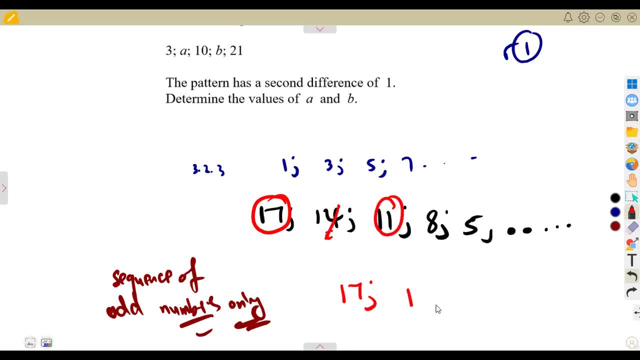 So this is not an odd number- 11. That's an odd number. If you divide by two, you get a remainder. eight divided by two, That's a four. So this is not an odd number. Five is also an odd number. 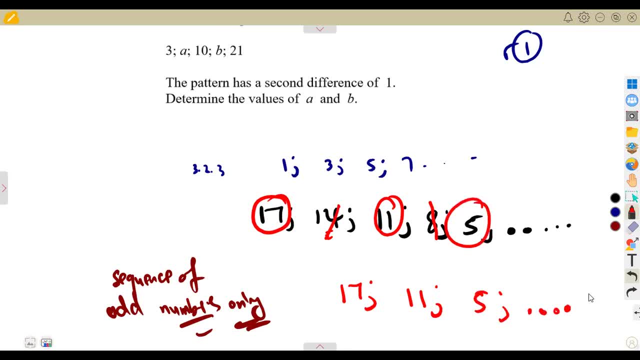 These are odd numbers, So they are going to continue like that and so on, and so on. We don't know where are they going to reach. So this is a new sequence Of what? of odd numbers. So from this sequence, you now answer the question. 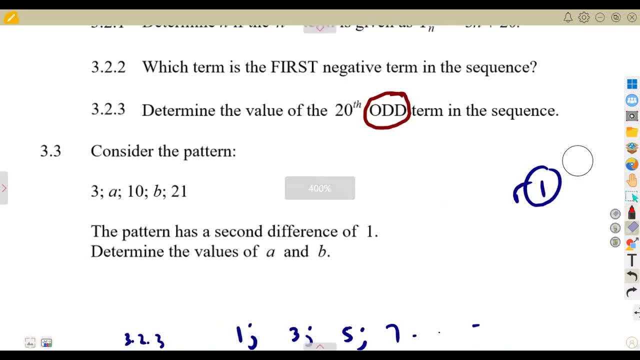 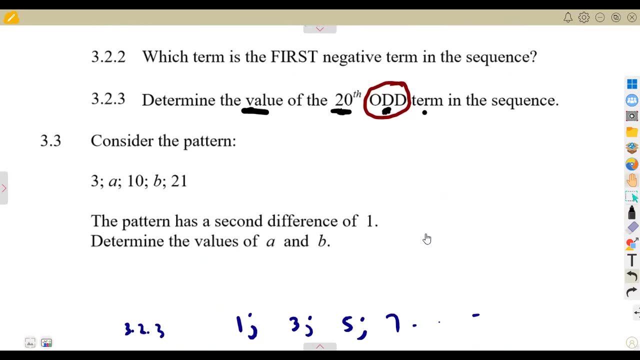 The question is: don't just rush that. we understand it, understand what it is saying. after that, Now determine the value of the 20th term of what these odd numbers. So we need T 20 of odd number. So this one is no longer there. 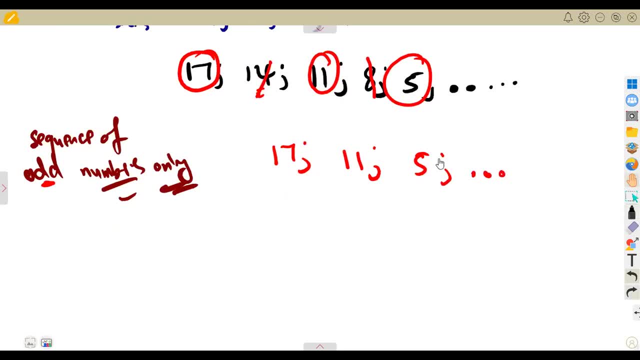 This one is no longer there. That's why we are even not talking about that T, and it's not. it's not that we have to find the TN from these odd numbers and we find what T 20 from there. So is it a linear sequence? 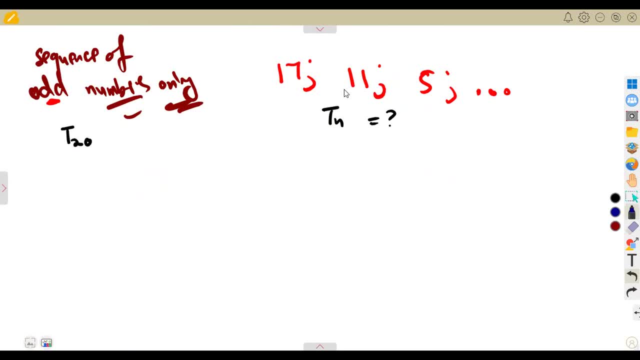 Is it a linear pattern? That is the question. Let's find the differences 11 minus 17.. There is a difference of minus six. Five minus 11 is a difference of minus six, meaning to say there is a common difference. And whenever there is a common difference, it means we are working with a linear pattern. 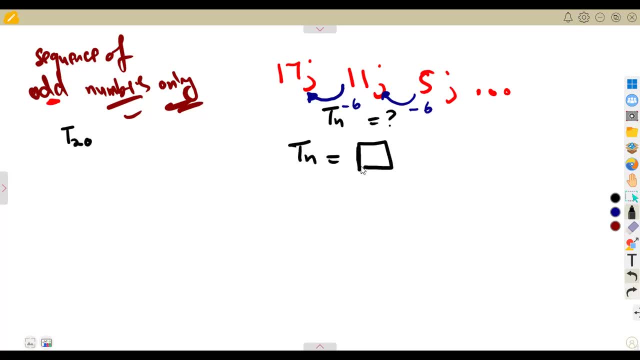 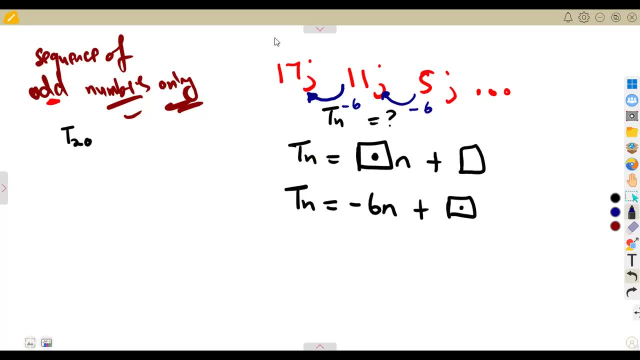 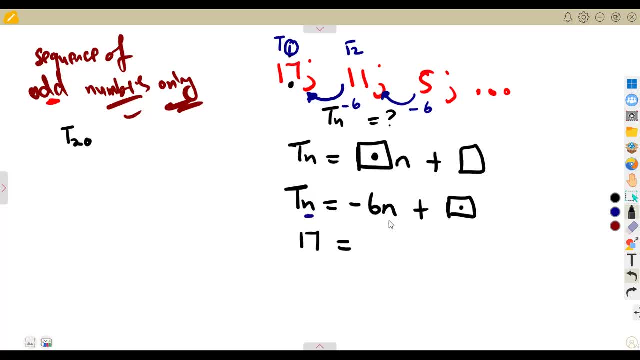 So T one, it's 17. when any is what, when any is one, when this N is one, you have to find this value. So this 6 transpose this side is a plus 6. so 23 will be equal to the value that you do not know. so 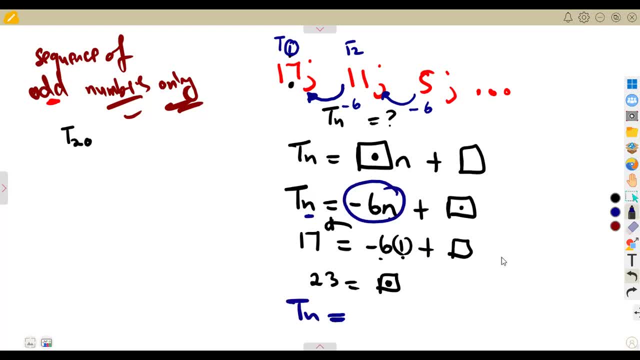 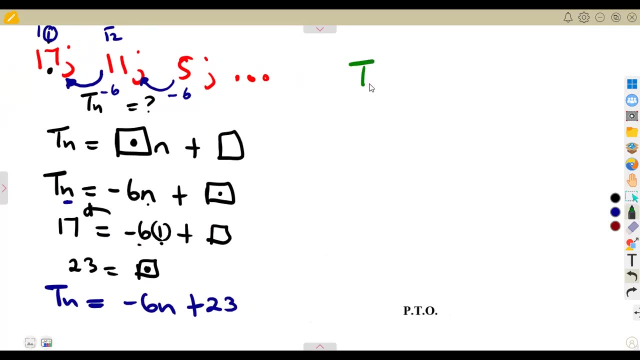 therefore, our tn was going to be given as minus 6n from that difference, plus the answer that we got, which is 23, or you can use this formula in short, which states that in a linear sequence, tn can be determined by this formula: a plus n minus 1 times the common difference. 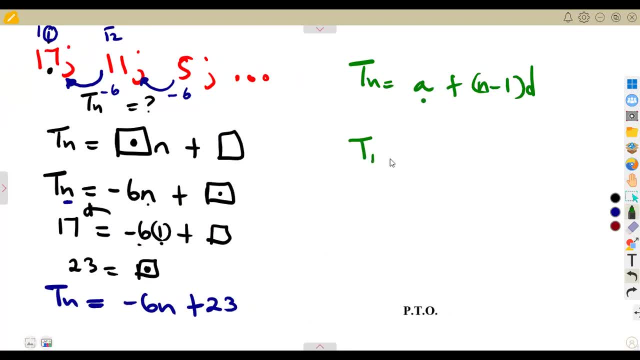 where a is the first term. so tn was going to be a, which is the first term and our first term. according to this sequence of odd numbers, our first term is 17 plus n. we do not know this n so far, but we know d is the common difference. 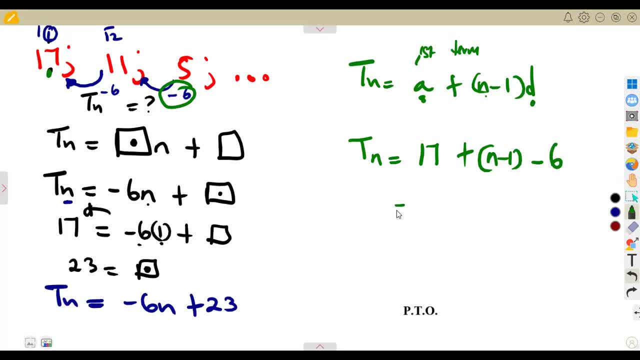 and our common difference is minus 6. so you have to simplify this. expand the brackets minus and the plus remains as a minus. so it's minus 6 times n minus 6, n minus 6 times minus 1 plus 6. add the numbers together. after expanding your brackets, you can have 23 minus 6 n, like this. 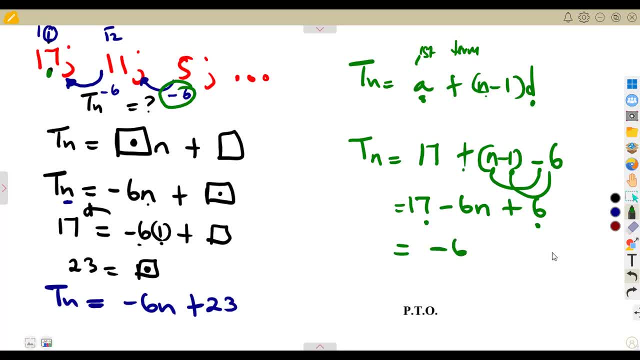 or you can have it as minus 6 n plus 23. you can have it as minus 6- n, like this, or you can have it as minus 6 n plus 23, just like this. it's up to you. this is how you can calculate your tn, so you're going to choose. 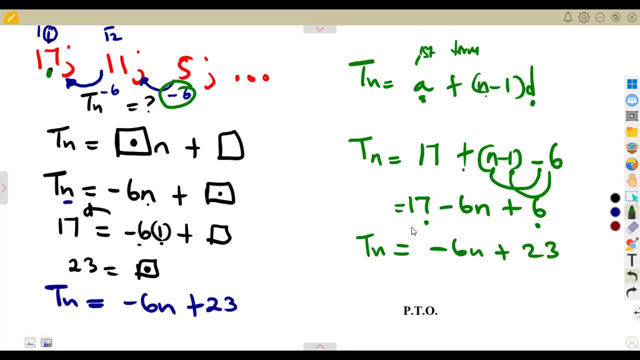 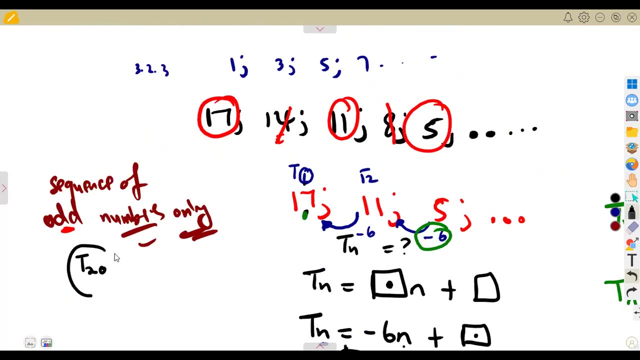 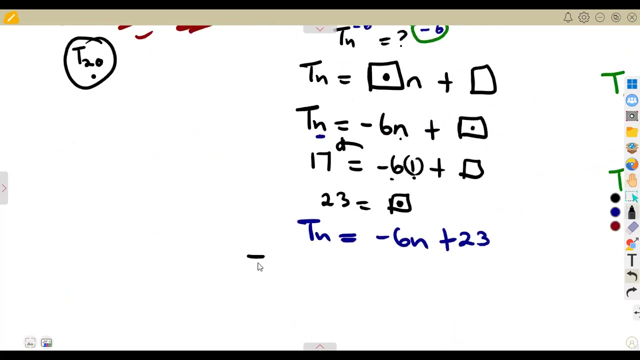 which method is easier to work with. that you understand the method that you do understand. with this tn, we are going to determine the 20th term, because the question was to determine the 20th odd term, the 20th odd term, so the 20th odd term. it means we are to determine t20 of these odd numbers, so that's a. 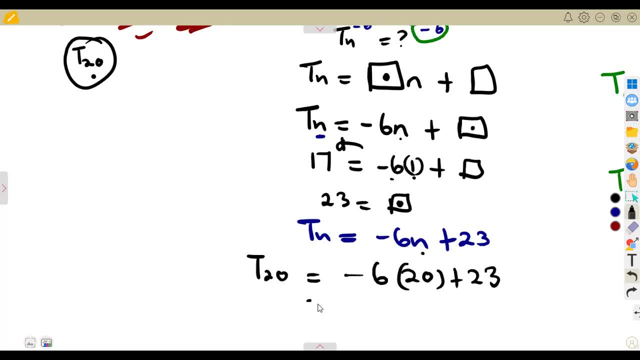 20 there plus uh 23. so at the end of the day, uh, this was going to give us minus 97 and, as you can see, minus 97 is actually an odd number. it is truly an odd number. so it must be of a surprise that you were told that this must be an odd and you get an even number. 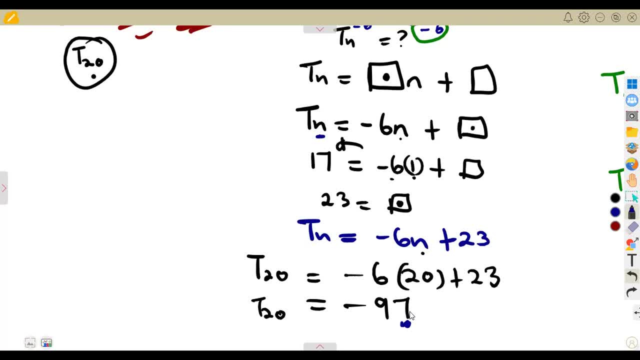 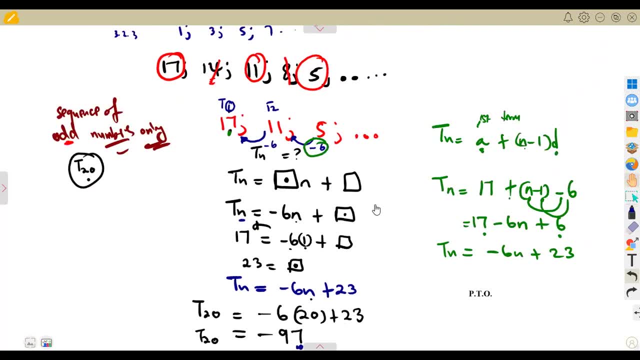 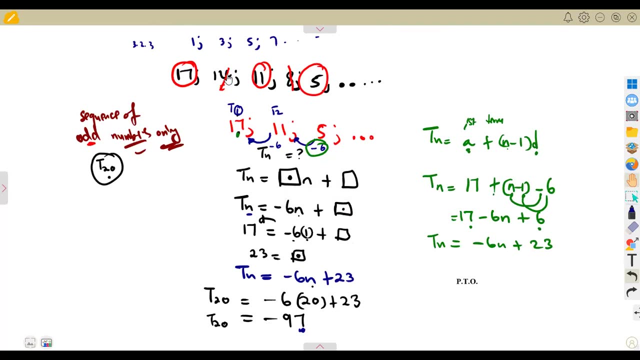 it must be of surprise. so this is how you answer this type of a question. you form the sequence of what you are supposed to determine. is it of odd numbers? is it of even numbers? you extract the even numbers from the original sequence. you plug out what you are given. what are we given? odd numbers? 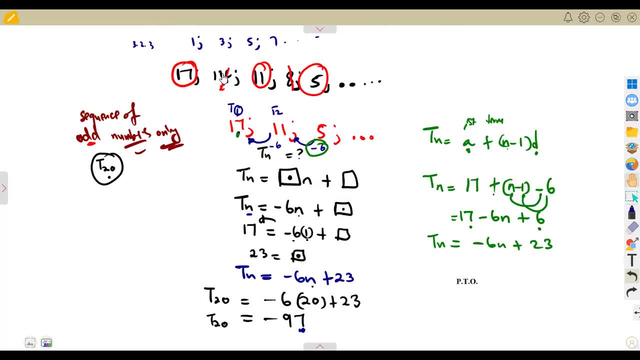 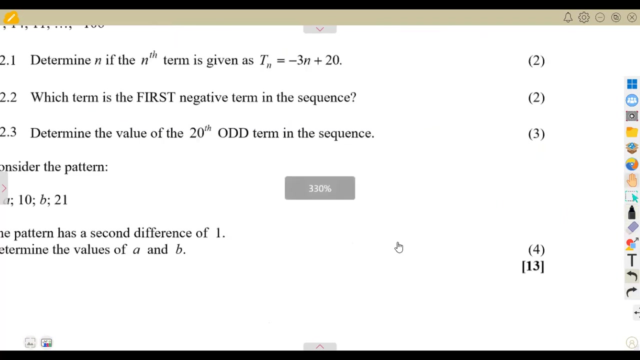 plug out the odd numbers from the sequence, take them out in the same manner, in the same sequence. plug them out as you are plugging them out. you are forming a sequence of odd numbers, just like that, so you just need to work with many persons understand these all right. consider the 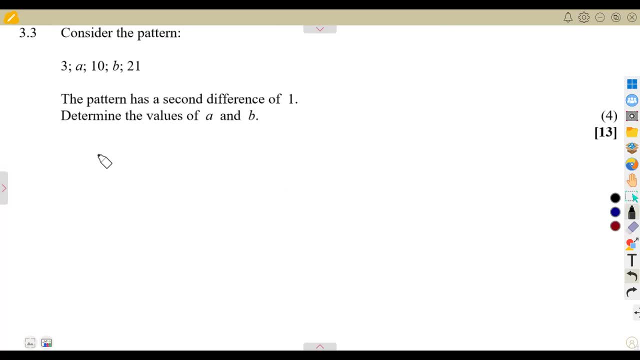 pattern. we are given another pattern on three points. in this pattern we are given this as 3 a, 10, b, 21. this is what we are given and they are saying the pattern yes, a second difference of one. so meaning say there's a first difference, a second. 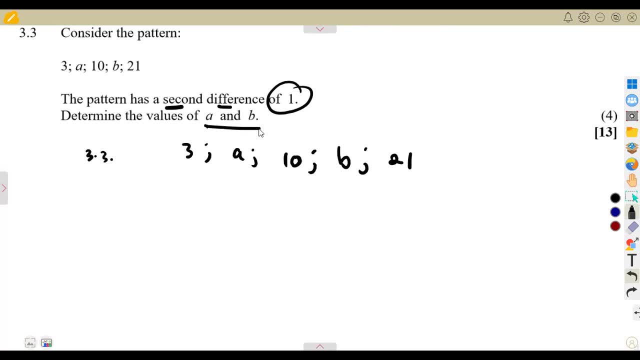 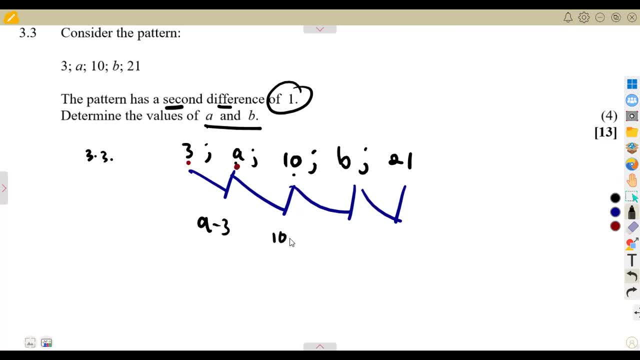 you can't simplify that 10 minus a. 10 minus a is just 10 minus a. no one can simplify that b minus 10 it is just b minus 10. no one can simplify that 21 minus b. no one can simplify that. these are the first differences. we got our differences. then they are saying: 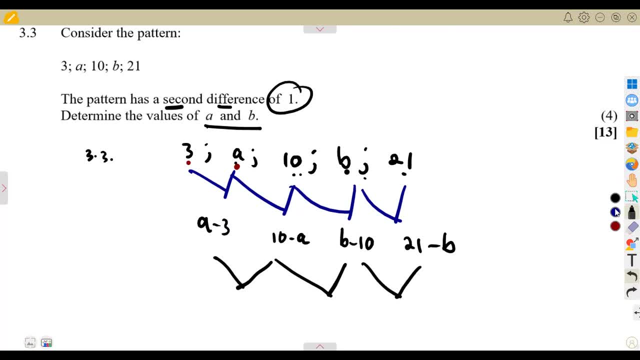 for the second differences. we were supposed to actually subtract this: this one minus this one, this one minus this one, this one minus this one. but instead of doing that, they are telling us that that second difference is one. there is a difference of a one, there meaning to say: 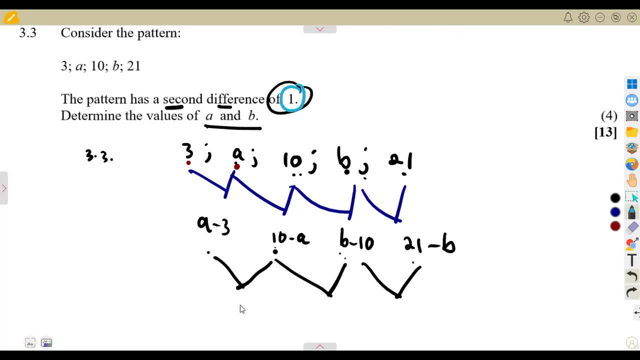 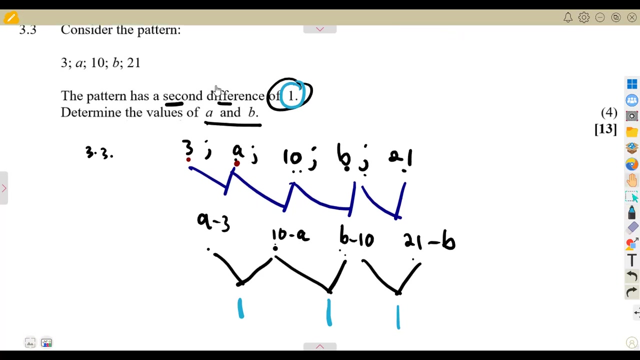 the moment that you subtract these two, you are going to get a one. you subtract these two, you are going to get a one. you subtract these two, you are going to get a one. the second difference is common throughout for a quadratic sequence of a quadratic pattern. so the question is: how can we determine the value of a and b? how we need four marks. 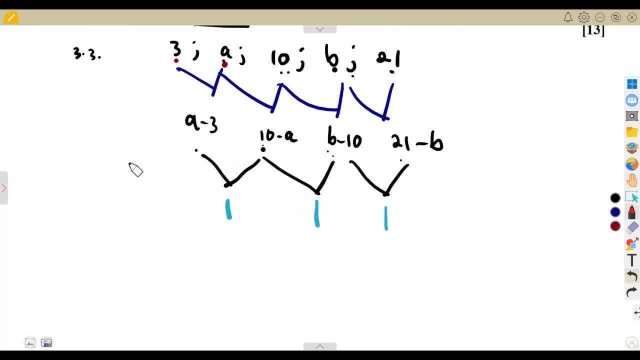 to. we need these four marks. how can we have a and b? okay, if you're see properly here, there's nothing that we can get from this part because of where it is coming from. there's nothing, but now this one that we are seeing here. we know that it is our common difference. 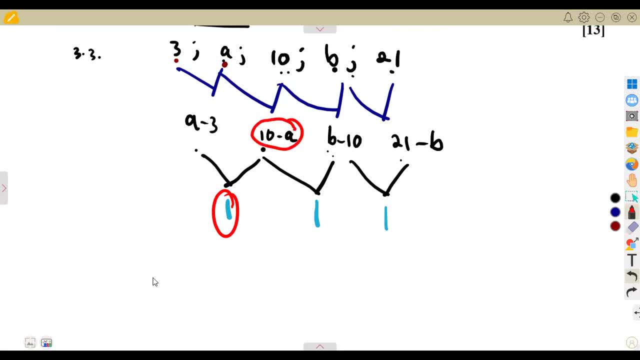 where we are to subtract this term 10 minus a minus, this term of a minus three. that is where we got the difference of a one, because it is the same. so we can form an equation like that and in this equation we can see that it is only a that we have, so we can solve for a. it's not as simultaneous. 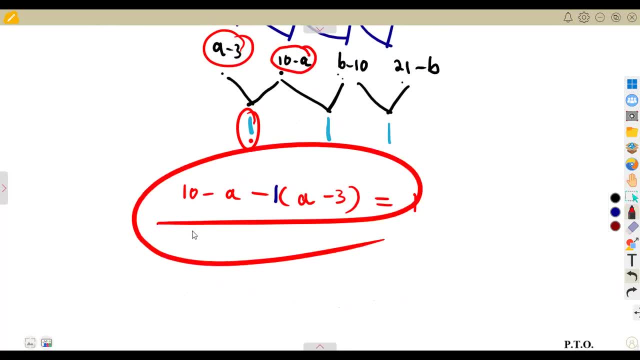 at this moment, because there's just only a in this equation, expand your brackets. 10 minus a minus one times a, that's minus a minus one times this, that's a plus three, is equal to one. uh, 10 plus three, that's 13 minus a plus eight means minus one plus minus one minus one. so minus one minus one is going to. 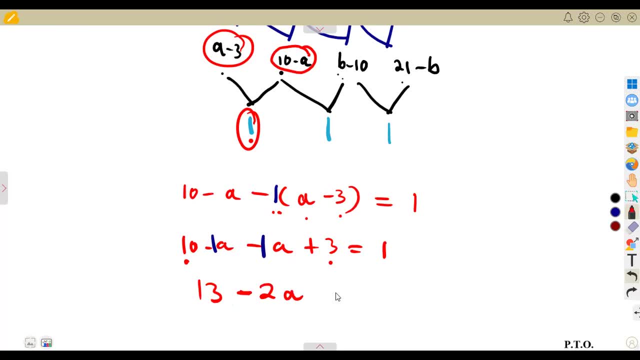 be minus two a, so that's minus two. a is equal to one. so if we're to solve for a, we're going to transpose uh, this 13 to the other hand. it becomes a minus 13. one minus 13 is minus 12. divide by negative two. 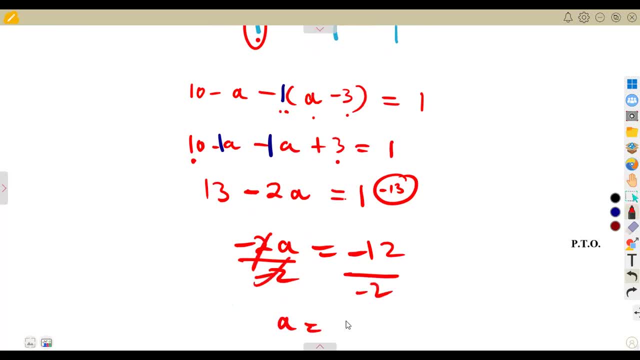 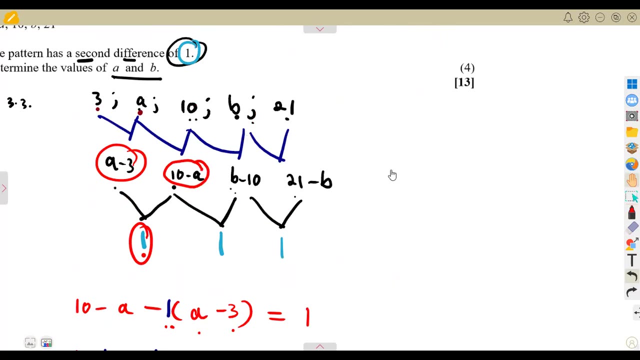 uh, both sides. so a was going to be. what a positive six. we just use a calculator, so meaning to say we're going to have a as a positive six. so how can we find b? we also do the same thing. we go where there's a- b. we know that, so we can just take any part where there's a- b. 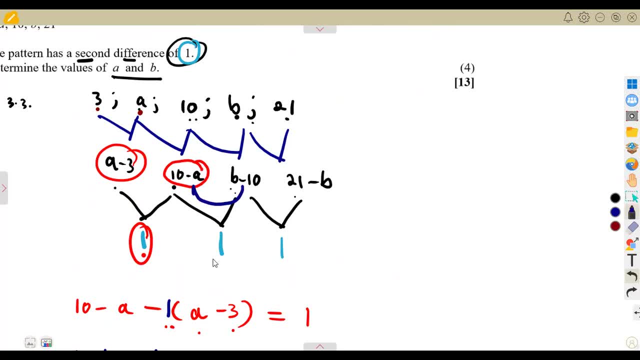 all right, you can take this part. this one minus this one must give you a one, which is fine. you can also take this one. there's a, there's some, there's something that i want you to see here which is an equation. all right, uh, this one is going to affect. 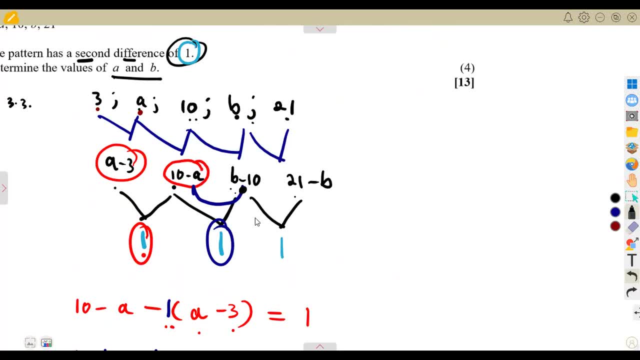 because we do not have a. so okay, let's just use this one, no problem. remember our a: we got this as six. so let's just put in our a here, 10 minus a. remember this was 10 minus a, so 10 minus a. and our a we got it at six. 10 minus six, that's a four. so mean you say there's a four there. so if 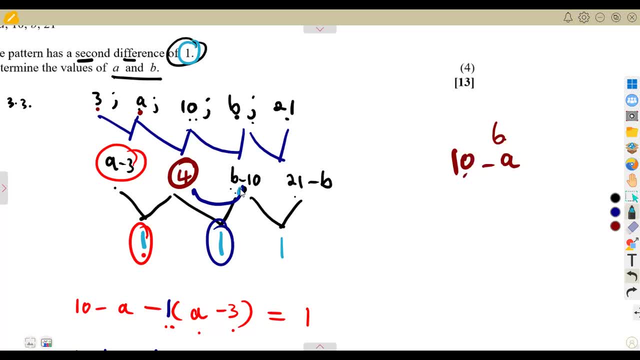 you're to do the same thing. where a, b is, you are going to have the difference of these two. to get what? the same one, because that is our second difference and our second difference on your quadratic pet is the same. remember that whenever they talk about the second difference is the. 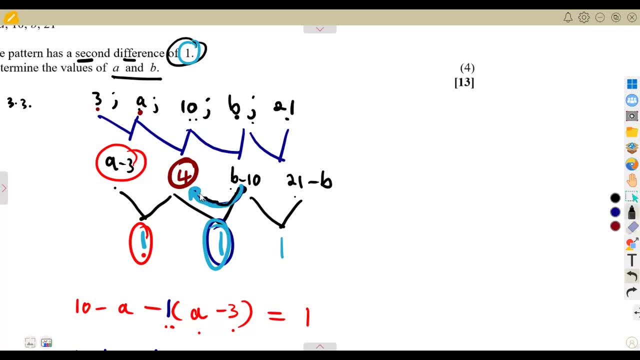 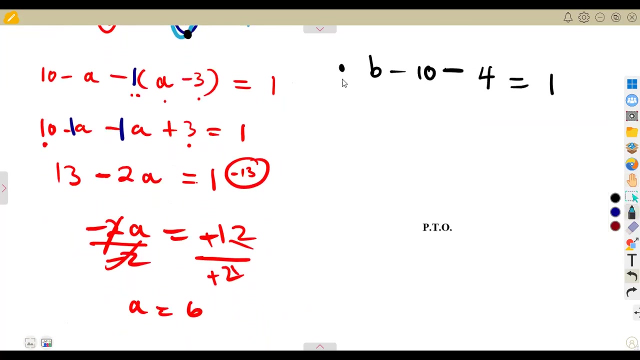 common difference. so it means b minus 10 minus four. it's an equation. so you form an equation: b minus 10. we subtract what from there? we subtract a four. we must have the same common difference of a one. so in this equation, as you can see, it's only b that we have. so we can solve for b on this. 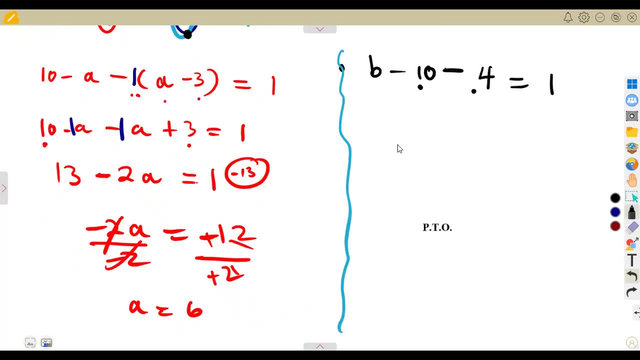 equation now: all right, minus 10, minus uh four, that is, minus 14- is equal to one. so b was going to be. transpose this: that's a plus 14, which is going to be a 15. so in this case, our b was going to be a 15, our a as a six. 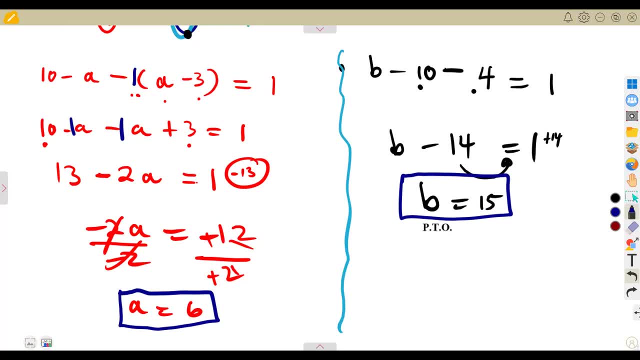 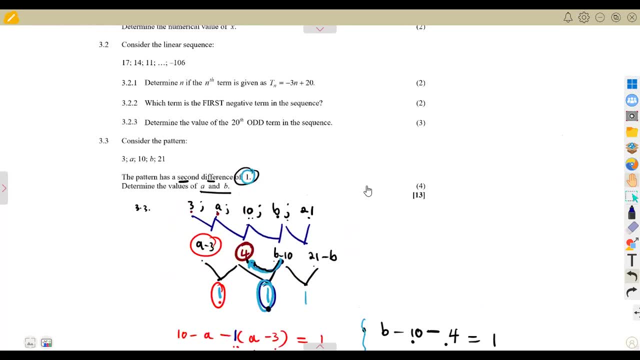 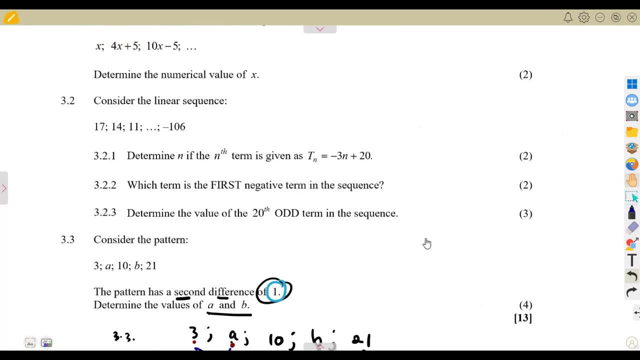 just like that, so you see how these questions can be. like they can play around. four marks for that. so that was our question number three: 18 marks on everything that we are seeing on this question, 18 months, so actually under exam. this is what you're going to. you just have to be able to do it. 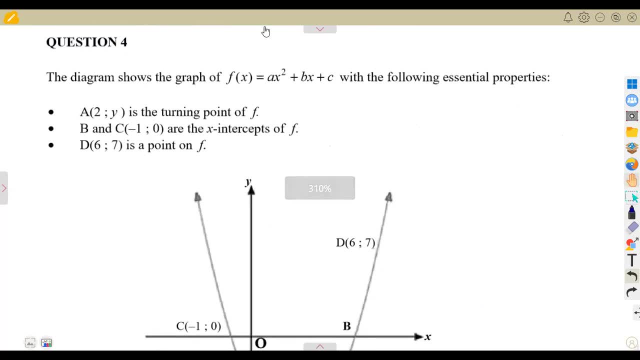 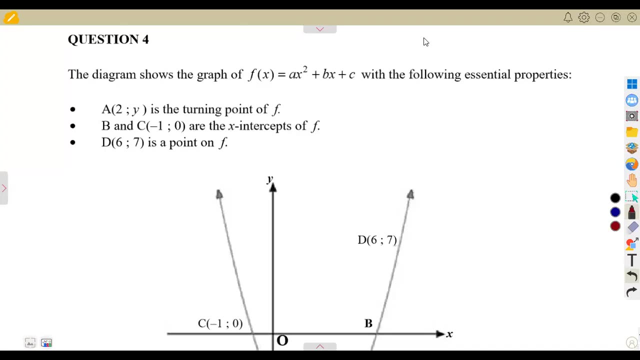 be very, very careful in how you simplify, uh and so on. just just try to be uh careful in in presentation. presentation first. the presentation on its own must be perfect. so let's consider this part. question four: what are we given? actually, there is a function. okay, the diagram shows the graph of f, of x, a, x squared, plus b, x plus c. 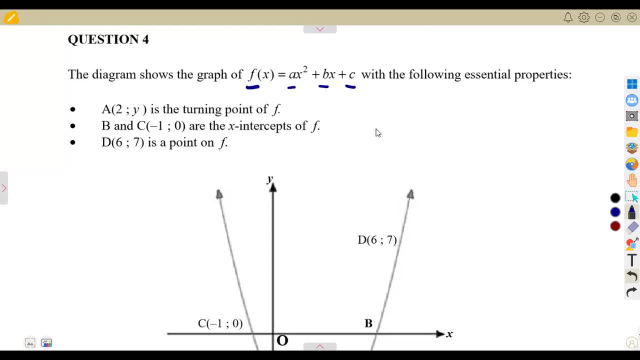 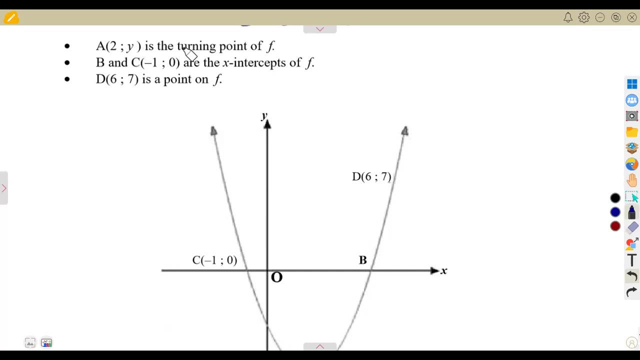 that is the format of a parabola, which is a quadratic function with the following essential properties, very important properties that you're given there. they gave us a, which is two versus y. two s to y is the turning point of f. so if we check on the diagram, we've got the point a. 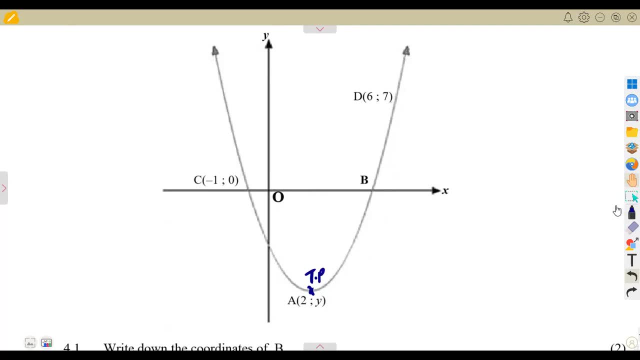 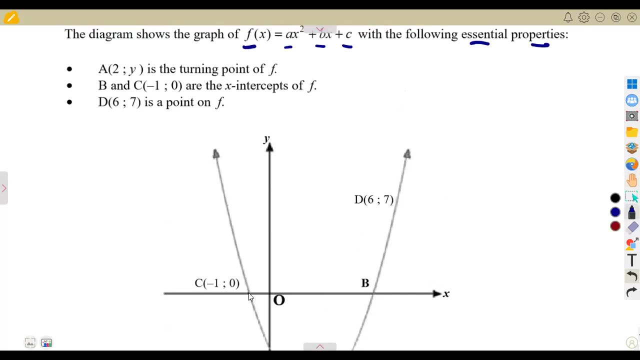 here. so that's our turning point. okay, we're given the x value at the turning point b and c, which is minus one zero. so the point c is minus one zero and the point b. here these are the x intercepts. d is the point six, seven is a point on f. so d is just a point situated or located. 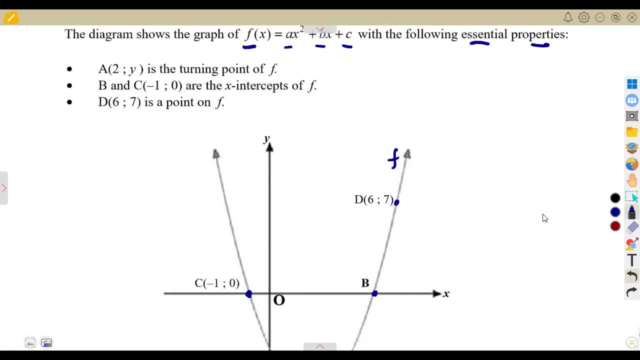 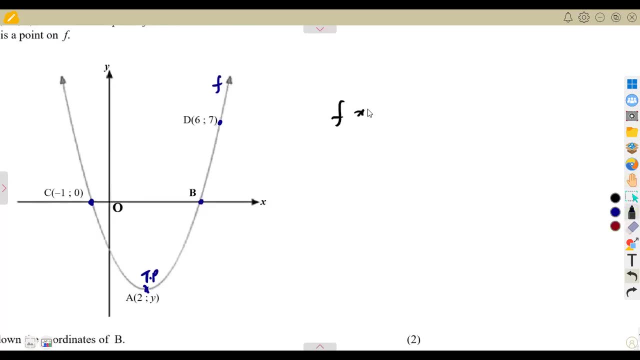 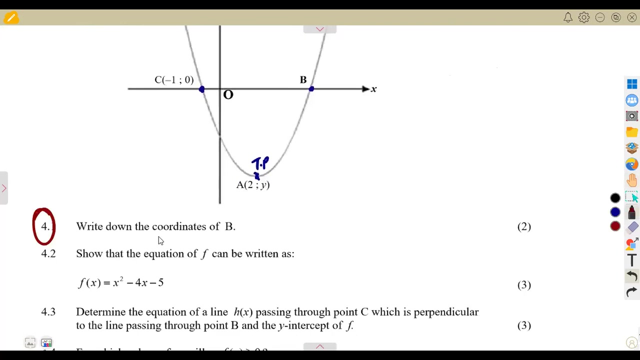 on our function f. that is what we have, and this function is a quadratic function which we are given the format f of x is equal to a x squared plus b, x plus c. all right, let's see 4.1, write down the x coordinate, that is the x coordinate supposed to be the x coordinate of b. 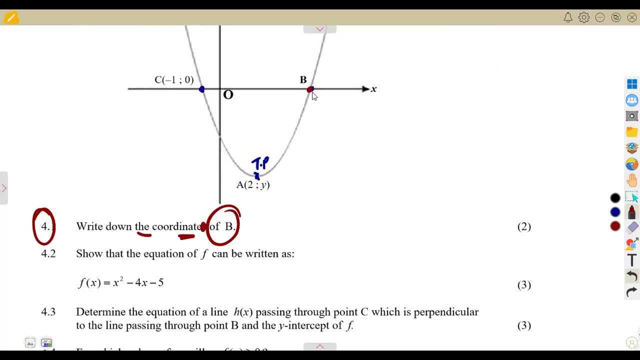 all right. so the x coordinate of b, that is, the x value at point b, the x value at point b, all right, if we were given our- let's say this is quadratic function, x squared plus five x. let's say we are given this you were going to consider all right in the 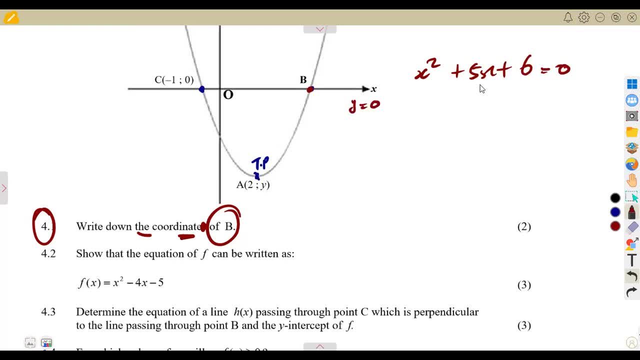 x, axis y is equal to zero. so this is equal to zero. you solve your equation, but there we are not given the equation, we are just given the format only. so what can we use? why are we given the turning point, the x value at the turning point? why they know that you are supposed to use this concept of the? 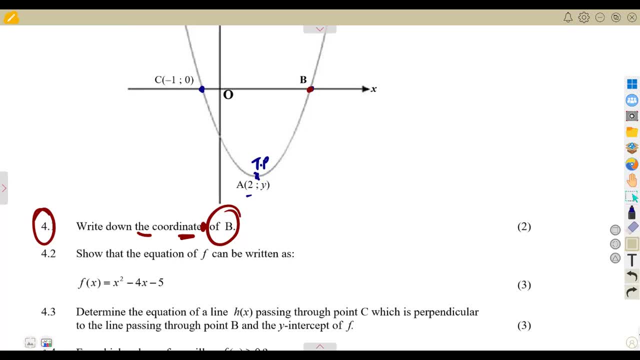 turning point. so i'm gonna explain this. let's hope you will understand me on this one, this one. i just hope you will understand me. all right. so this is the situation at the turning point tm. if we are to draw a vertical line straight to the x value at the turning point, y is equal to zero. so this is the 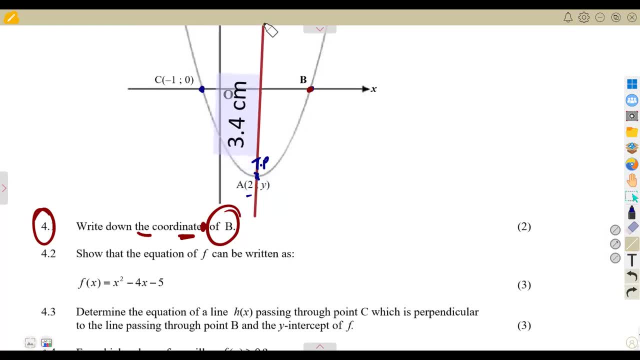 straight passing through the turning point, like this, straight, all right, so this one, okay, just a little bit like this: straight passing through the turning point, like that, going up as this line goes up straight at this point, the x that you are seeing at this point, there, this x, here this x y. 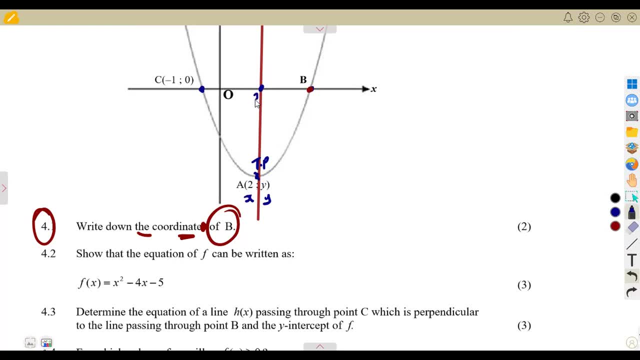 as a point is the same, because this line that you're seeing is parallel to the y axis. so throughout this line, which is called the axis of symmetry, throughout this line, x will be equal to two, throughout the line, throughout. so that can be an advantage. why we can take that? because at point b we know that 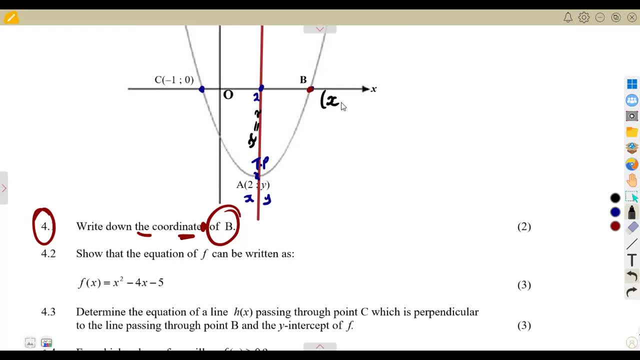 we were going to have the value of x and we were going to have the value of y, and we were going to have the value of x versus the value of y, where we know that along this line, y is equal to zero and this point is supposed to be x versus we. we just need to know the value of x. we already know that. 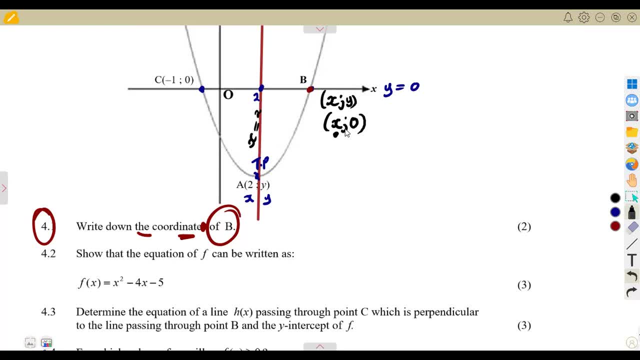 y will be a zero then. so don't focus about that, even here, to this point, at this point, it is two, it's two versus y is zero. throughout this line, y will be a zero, so don't focus that. just consider the x. so, using the midpoint concept at the turning point, because this is the axis of 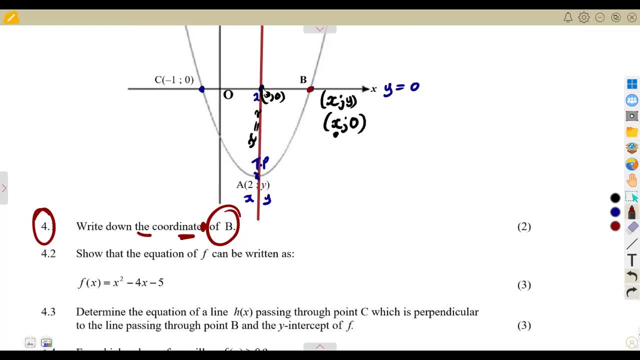 symmetry, the axis of symmetry. it means it, it divides your graph into two equal parts. so this is the midpoint, using the x? uh intercepts, which are the solutions. it follows that from the solutions minus one, uh, this will be the idea. so, four point one, using, so you're going to use uh, the mid point concept. 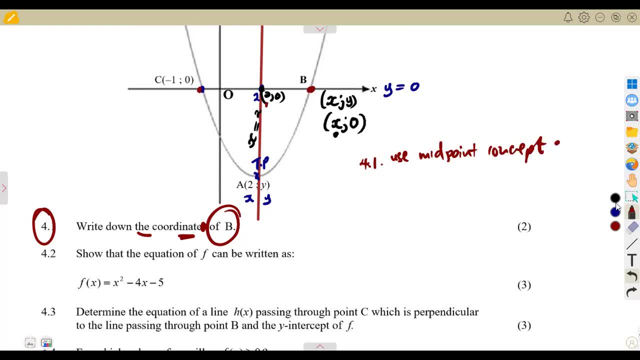 so using the midpoint concept, but just focus with x. we know that the x value, of this point to the x value, is supposed to have x one. this was supposed to be a formula, guys. you know your midpoint. but in this case, what i'm simply saying already, we know the part of y. don't focus with. 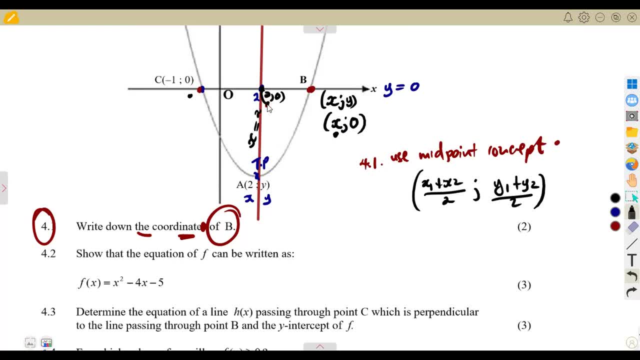 just focus with the midpoint. you already know the x at the midpoint is true. how did you get this? you had to add the x value, the x value, this one, which is minus one, plus the x value at the at the, at the point b, which we do not know, divide this by two. you are. 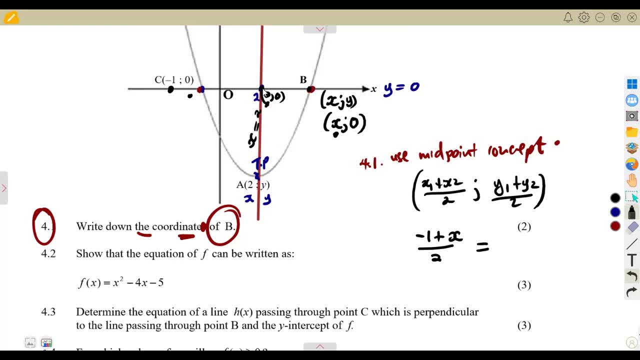 going to obtain the x value at the midpoint. and what is the x value at the midpoint? the x value is true. so that's an equation for you. solve that for x. so this is same as over one. so you can cross, multiply uh one times, uh, this. i'm just going to change one times this. 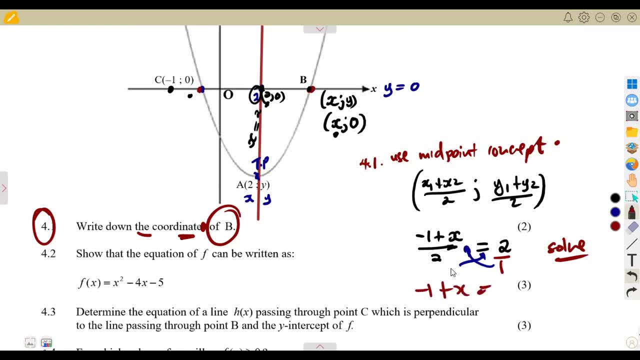 is going to remain as it is. minus one plus x is equal to two times two, which is a four. all right, transpose the minus one to this side, it will be a plus one. so x is going to be four plus one, which is five. so meaning to say that at the point b, x. uh, write down the coordinates, guys. you see the way. 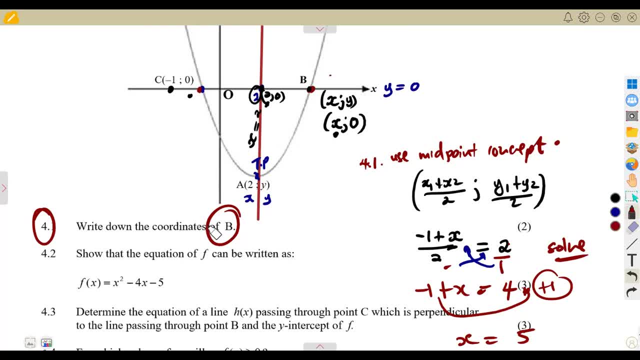 i don't know- now i think i'm tired guys- the coordinates of b. i don't know where did i see the x there? all right, so the question was: the coordinates of what of b? so at point b, we now calculated our, our value of x, which is what? which is five? so meaning to say, therefore, the point b is: 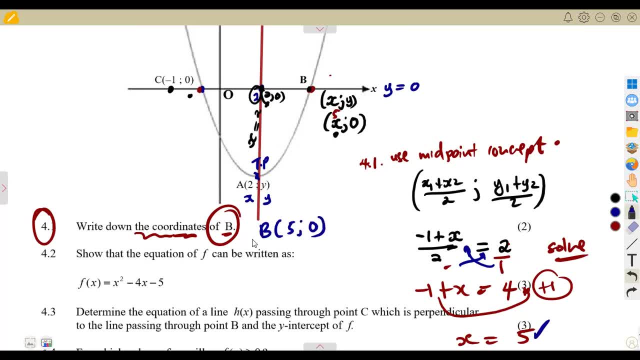 going to be five zero. these are the coordinates of what of b. all right, so pardon me, guys, for the way that i i i had to read the way that i read that one. i said x coordinate is just the coordinates of what of b. there four. point two show that the equation of f can be written as: 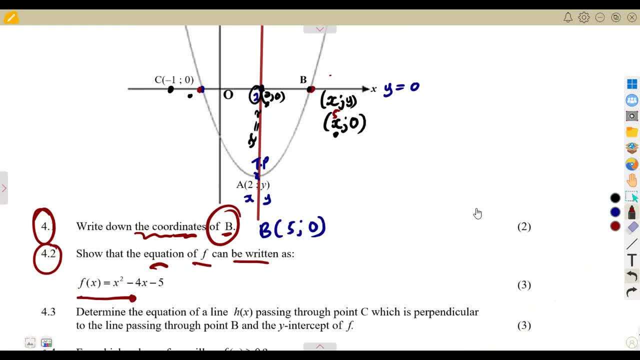 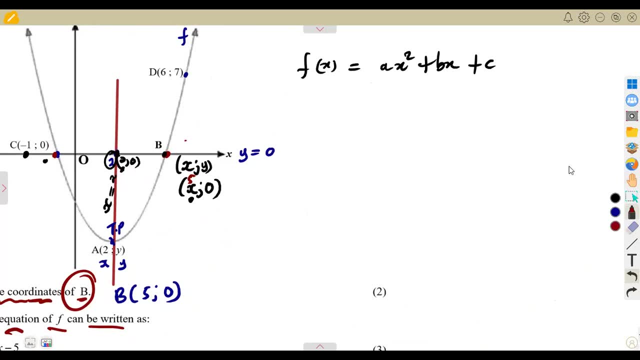 our equation of f can be written as: so what they are simply saying is that form an equation. you just have to form an equation. so how do you form an equation? uh, given this format, say hi, it's a, it's a parabola. so how do you form the equation? all right, it follows that when given the intercept, 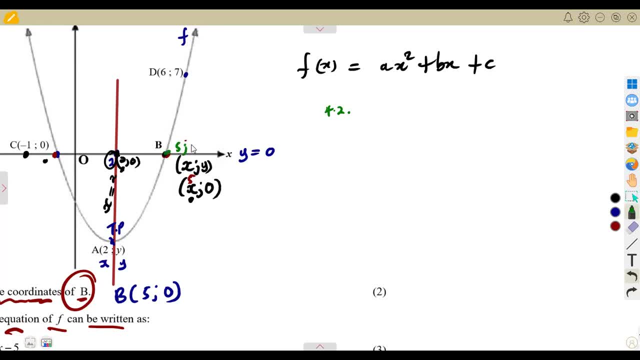 the x intercept, which are the solutions? because the x value is five. remember this is five zero. when given the intercepts like this: okay, because the turning point you do not have. you do not know the y value there, you just know the x value. so you do not have the turning point in full. if you are given 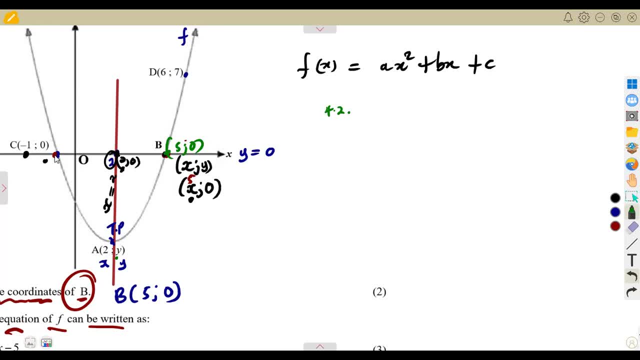 the turning point. there's a method for that, but if you are given the x intercept, which are the solutions f of x or y is equal to a into x minus the first solution, into x minus the second solution. this is your format: x minus x1 in x minus x2. so it follows. 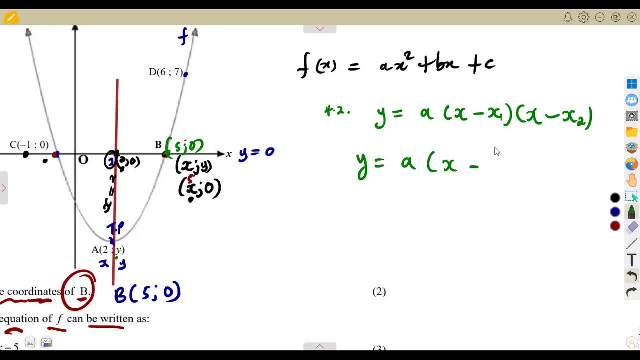 that y is equal to a into x minus x1, our x1. and the solution at the end, in the, in the y, in the xx, is there. what is the x value at this point? it's minus one. so it was gonna be a minus one into x. 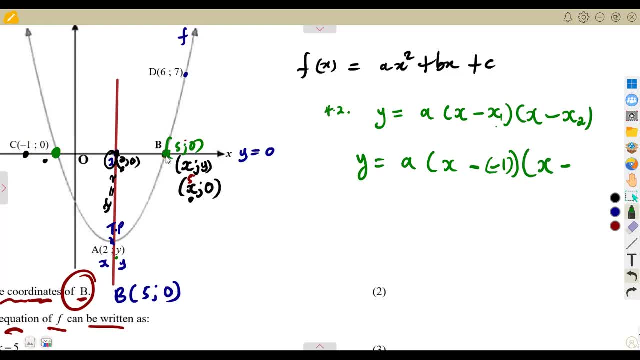 minus x2. our x2 is the x value, also at the intercept, which is a 5. so this is same, as we have got minus and minus there, that's a plus 1 into x minus 5. all right, so it's: either you're going to expand this or just leave it as it is, so that you determine the value of a. so to determine: 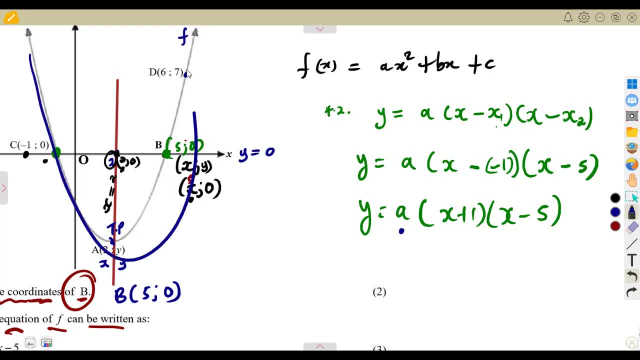 the value of a. you take any point which lies on this function, a complete point where there is x and also the value of y. so we can't use this point because we just have x. we do not have y value. so we are going to opt for the point d, which also lies on f. remember we are told that d lies on. 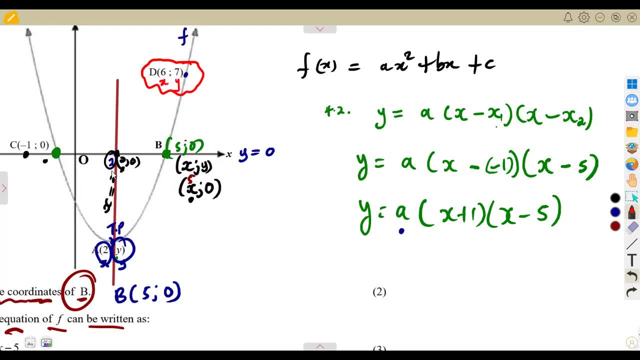 on our f, where we are given this as 6, 7, with the value of x, which is 6, and the value of y, which is 7. we can substitute: y is equal to 7 at a point where x is equal to what to 6. so this is 6. 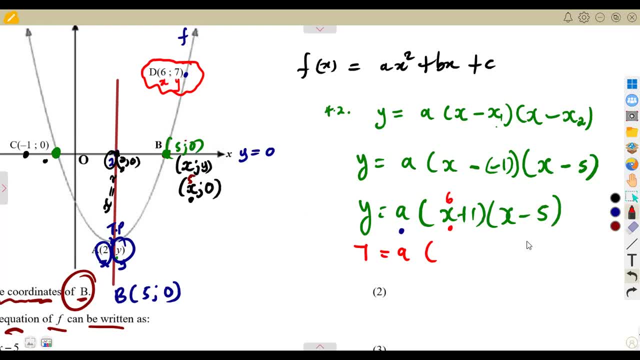 in place of x. here you're going to subtract a 6, 6 plus 1, that's a 7, into x is a 6, 6 minus 5, that's a 1, so that 7 is equal to 7 times 1, the 7a divided by 7, by 7 guys going to divide, so a is a 1, so 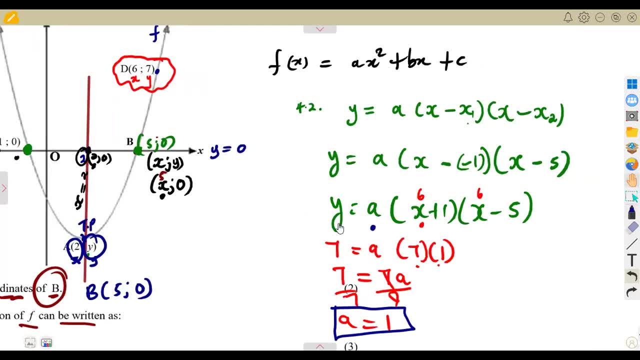 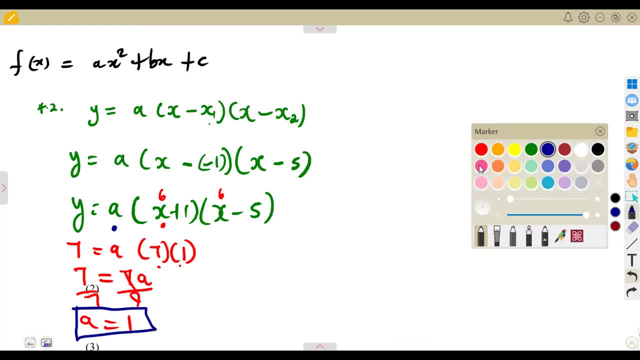 meaning to say you have got the value of a by substituting any point that you are given which lies on the function. that's why you are given that point which lies on the function, that's why on function. so, going back to this stage, because we have calculated the value of a, it follows that 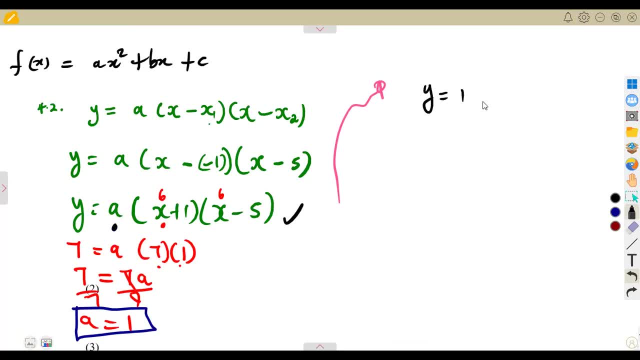 y is equal to 1, which is our a, into the bracket of x plus 1. into the bracket of x minus 5, 1 times. anything just remains as it is, so just like there's nothing there. so if you are to check, the format is just an expanded format. remember from your grade 10, you expand two brackets where there's 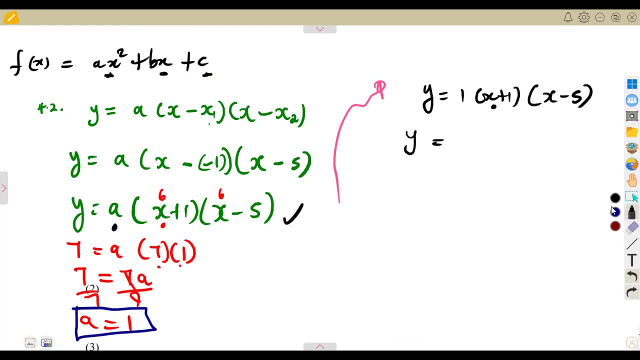 x and x, you're going to have x squared, so just expand your brackets. so in this case you have to expand brackets or remove the brackets, all right, so how? so? multiply by x, this is 1 times x, so it's just going to be x plus 1 as it is. so you distribute by x. x multiplies x, that will be x. 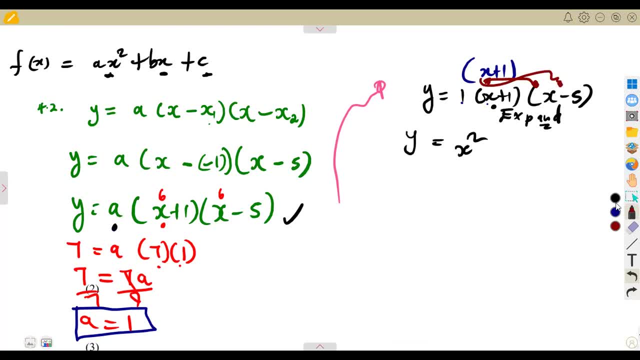 squared. x multiplies minus 5, this will be minus 5x. but then you move on to 1, x and x. you're going to have x squared, so just expand your brackets. so in this case, you have x squared, so you're going to have x squared. so you're going to have x squared, so you're going to. 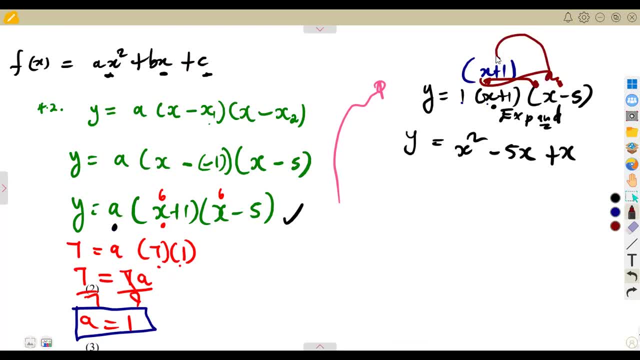 multiply x, that will be a positive x, 1. multiply the minus 5, that will be a negative 5. so meaning to say y is equal to uh. collect the like terms, that is x. squared here there's x and x, so these are the like terms in terms of same exponent. so minus 5 plus 1, that is minus 4, so that will be. 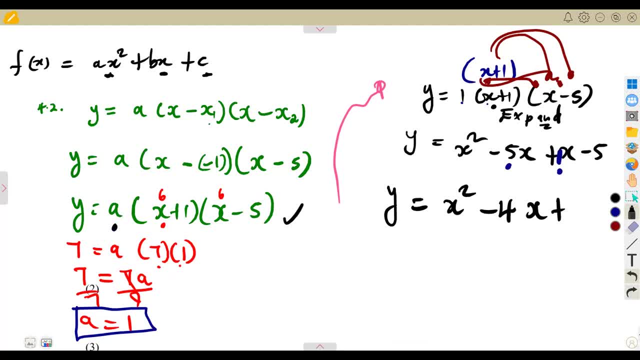 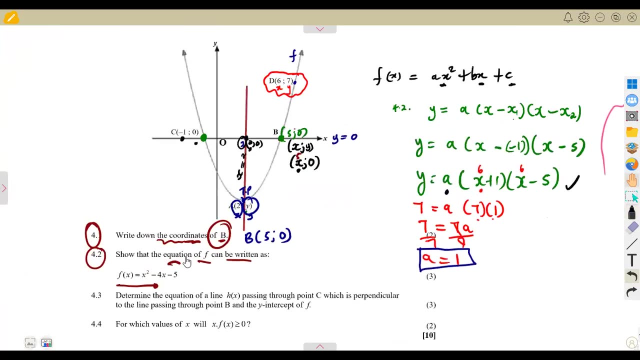 minus 4, x plus um, plus minus 5, which is minus 5. there, it's just minus 5 on this one. this is it exactly the way that we are given there. this is: f of x is equal to x squared minus 4x minus 5. exactly what we are given. so that is. 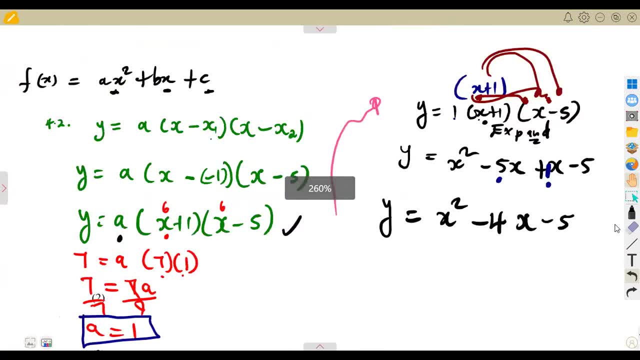 what you're being asked to show. okay, so you can just write as f of x, no problem, for that x. f of x is equal to x squared minus 4x minus 5. so that is uh. in this case, they just wanted you to formulate the function, the, the, the, the, the, the, the equation of that function that you're given. 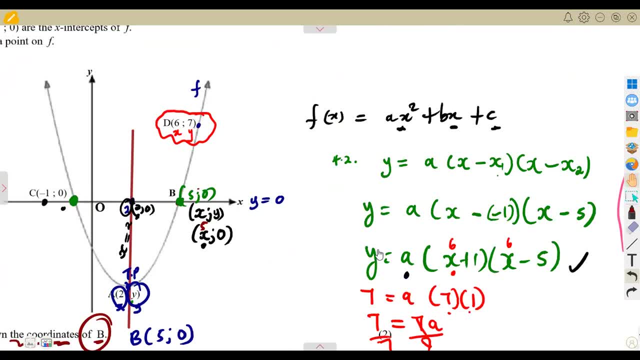 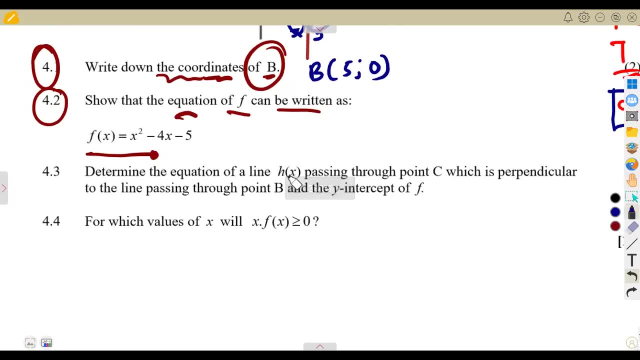 they just wanted you to formulate that, but anyways, let's see, determine the equation of the line hx. this they are saying: there's a line hx passing through the point c which is perpendicular to the line passing through point b. okay, okay, and the y intercept of f? okay, the first thing is we need to determine the equation of hx. 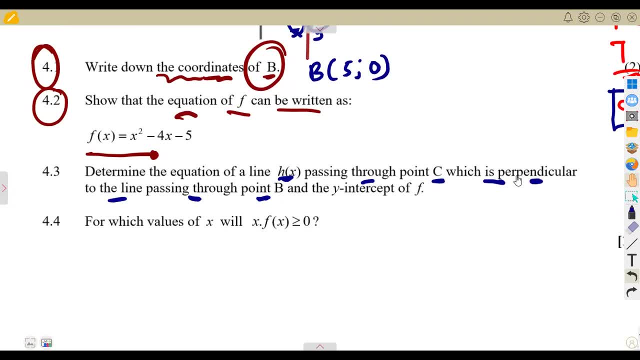 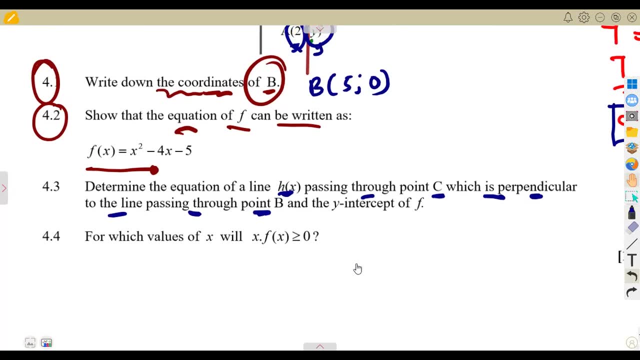 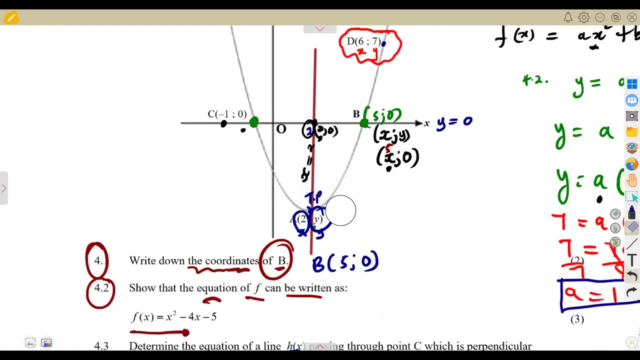 but this hx. it passes through c, which is perpendicular. it's perpendicular to where? to the line which passes through b. there is a line which passes through b here. okay, this is it. so be careful how this question was given. they are saying: let's, let us put this way. i'm just gonna remove this part. there is a line which passes through b and the y. 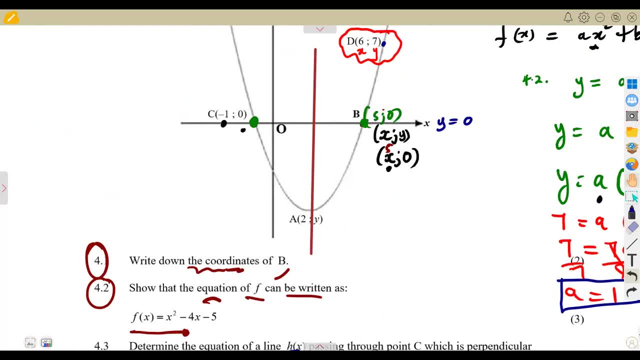 intercept, it passes through b and the y intercept. like this, it must pass through b and y. like this, the line is like this. so the question is: we are supposed to find the equation of the line from the point c, from the point c, from the point c. the line as it is drawn, it is like this: 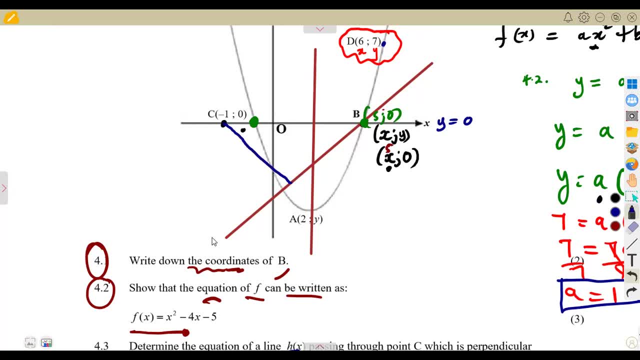 to this line which passes through b, and what the y intercept here? so this is the line that we want to find its equation, which is perpendicular to this line which passes through b and the y intercept. uh, they're saying, okay, let's go back, let's go back. 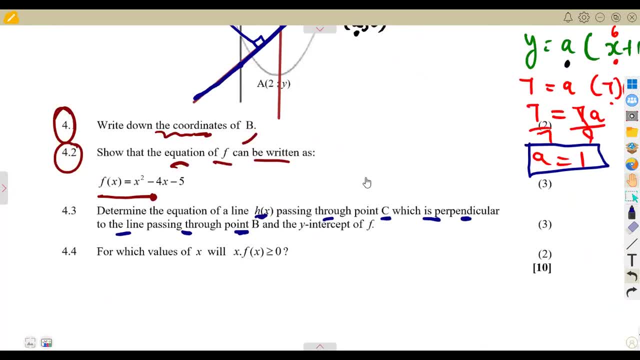 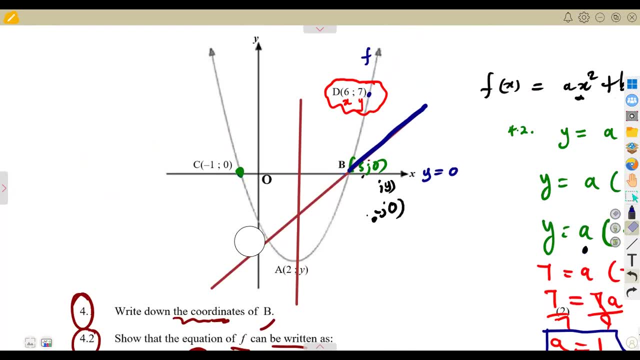 let's go back the y intercept, the y intercept of f, the y intercept of f. so it must pass through the y intercept of f. so if we take this, guys, my sketch is not gonna be fine if we take this way. uh, let's just hope i'm gonna be able to remove. 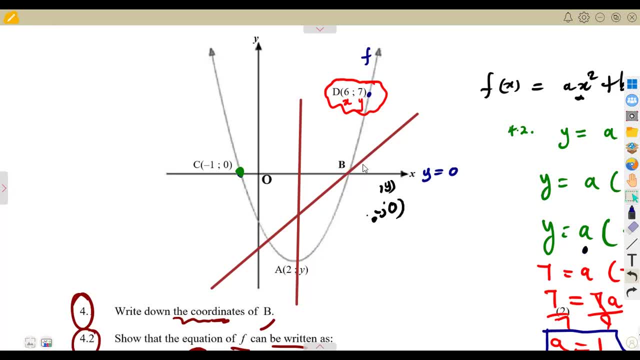 this: it must be through the y intercept of what of f. okay, let's just hope we're gonna win, guys. very sorry, very okay. so let's do it this way. the y intercept of f is: the is here, so it must be like this. the y intercept through b like this: all right, so the line must pass through the y. 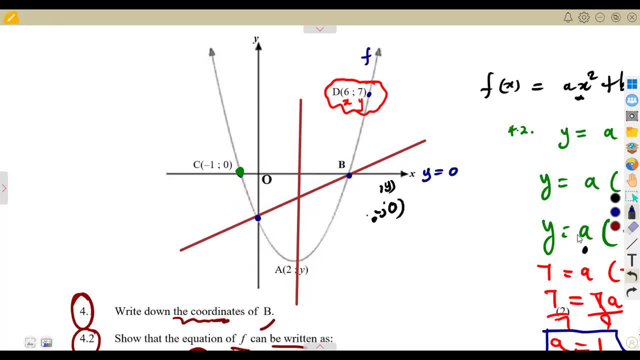 intercept of f and also pass through b. so we want the equation of the line perpendicular from c. so from c it must reach this line. at what? at 90 degrees, this line which passes through the y intercept of what, the y intercept of f, and also through b. 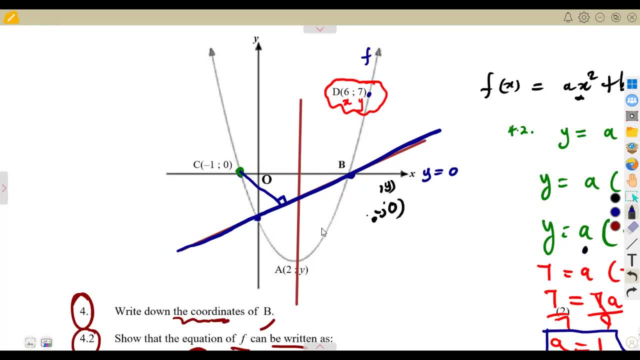 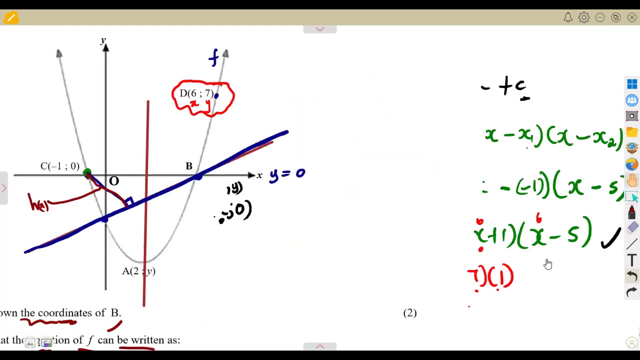 so the question is: we need the equation of this line, i mean the equation of this perpendicular line, this one, this is the perpendicular line, this one, this is our hx, this line. so we need to determine this equation. how can we determine this equation? okay, let's focus on the concept that we are given that they are perpendicular. okay, so if they are, 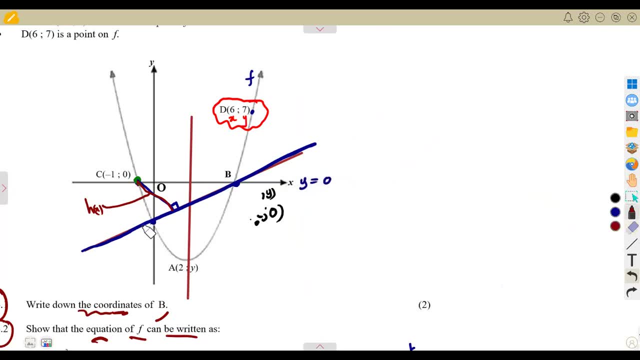 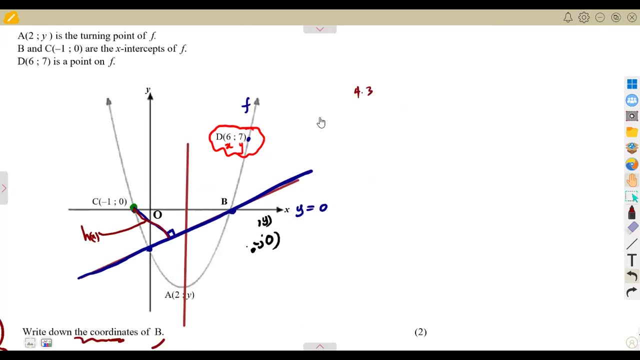 perpendicular. we understand that the gradients of these lines areATs. that's why they are perpendicular. two lines must be a negative one. so this is our four. four point three. i'm not mistaken there. let's check. that's four point three. all right, so if two lines are perpendicular, the products of the 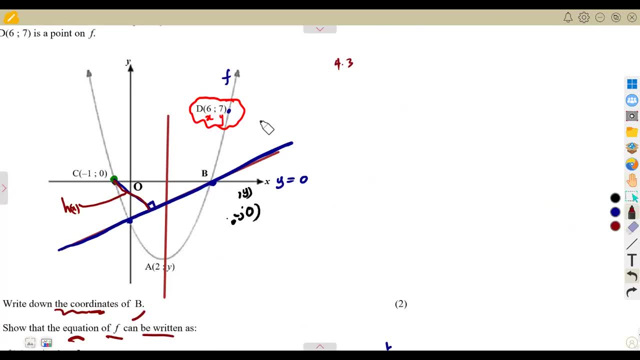 gradients must be a negative one. so the question is: are we having the gradient of this line or can we have the gradient of this line direct? we can't have the gradient of this line direct because we do not know where this line, it is going to pass, this line uh from b, but we know that. 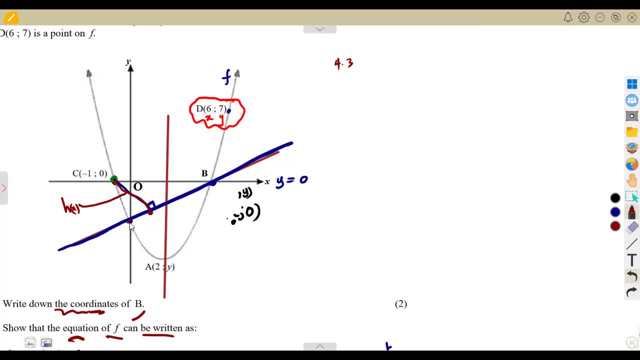 the line from b passes through the y-intercept of what of f. so if it passes through the y-intercept of f, we can determine the point here at the y-intercept of what of f. so what is the y-intercept of what of f? because we are told that it passes. also the line from: 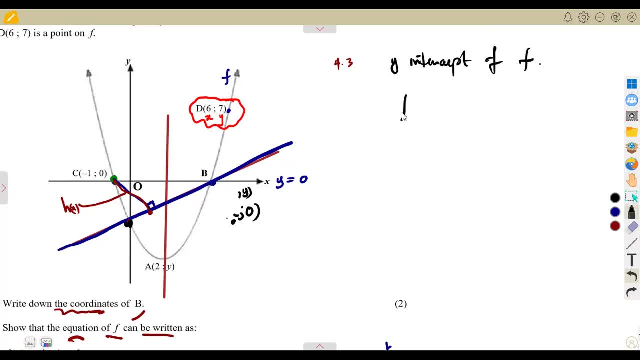 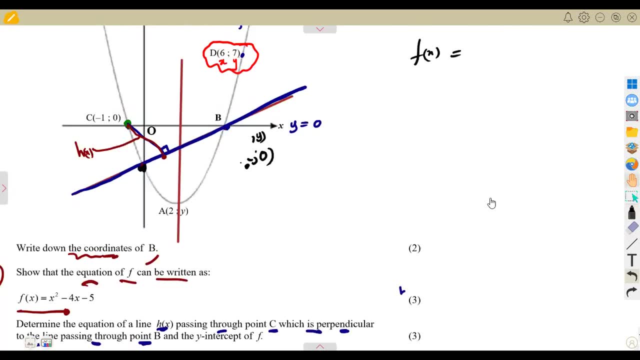 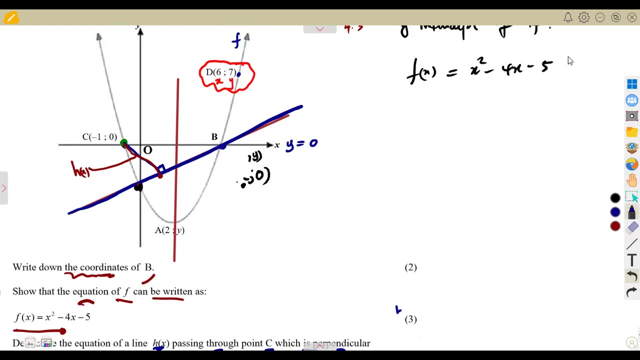 b passes through the y-intercept of f and remember our f of x, the one that we calculated before. uh, we got this as x squared minus four, x minus five. remember from our calculation this was x squared minus four, x minus five, and the y-intercept. we know that x must be equal to what x must be. 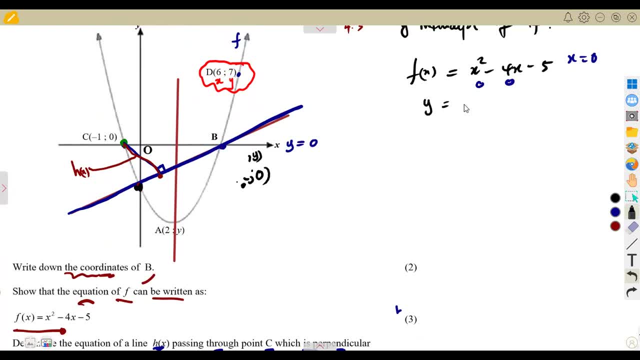 equal to to zero. so if x is equal to zero, it follows that y is equal to minus five. so this point here is minus five, that's zero minus five. y-intercept: x is zero there. so we can take advantage of this point b because we know the point. 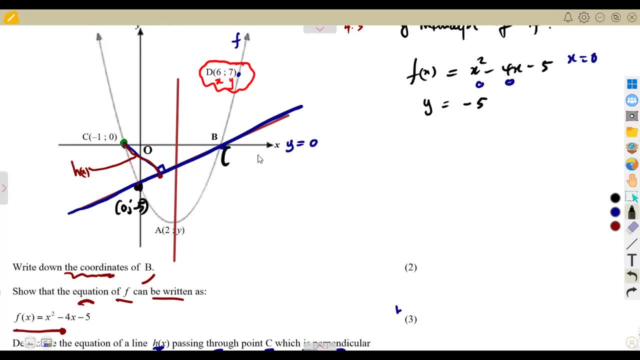 b before the point b, remember, is the first point that we calculated, which was five zero. so we can calculate the gradient of this line from b to c. our gradient, remember from our formula y2 minus y1 over x2 minus x1, it follows this gradient. the y value of this line is: 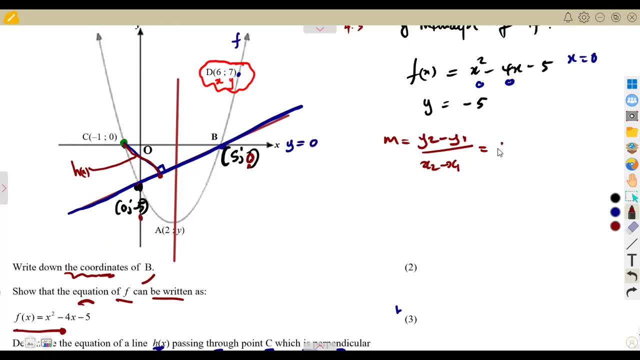 zero minus the y value, which is minus five. so it's zero minus minus five over x2. the x value here is five minus the x value at this point, which is a zero. so this will be positive. five over five, which is one. so that's five over five, that's a one. so the gradient of this line is one and we are 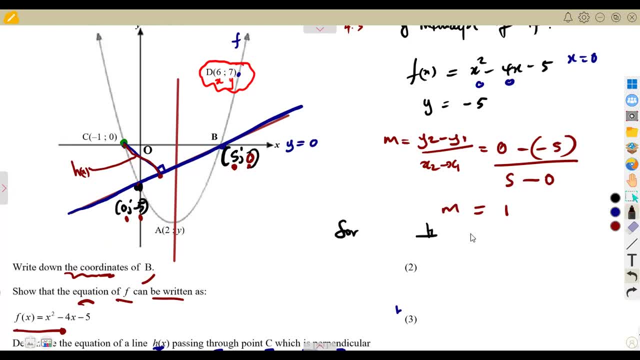 saying, for perpendicular lines, the gradient of the first line times the gradient of the second line must be equal to negative one. so from this line that we are given b, which passes through the y-intercept, its gradient is one. what about the gradient of the second line, which is the one that it is perpendicular to the one for hx? what is its? 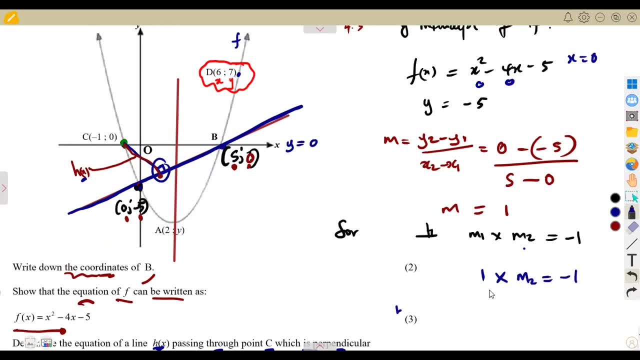 gradient? we do not know, but we know that their product must be a negative one. so if we divide by one, by one, it means the gradient of the second line is minus one, and the second line i'm referring to, hx. so let's say this is our first line and hx. 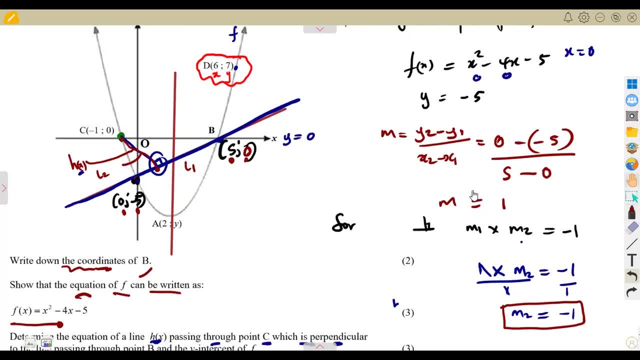 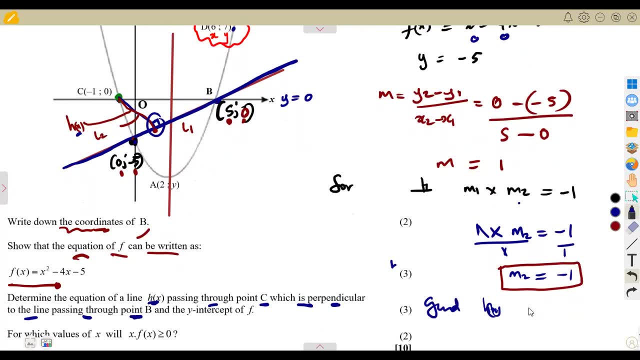 is our second line. so we have now the gradient of the second line, which is the gradient of what? the gradient of hx. we have it as minus one and hx passes through c. so if hx passes through the point c, given as minus one, we have the gradient of the second line, which is the gradient of the. 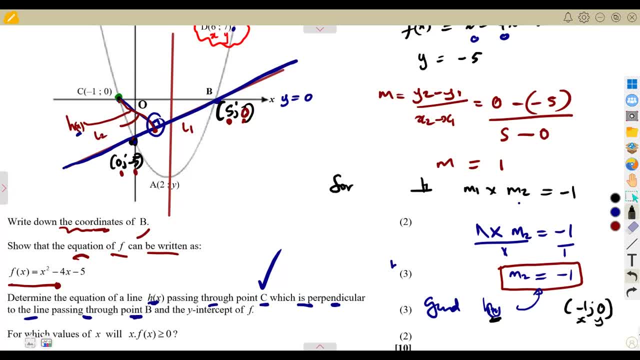 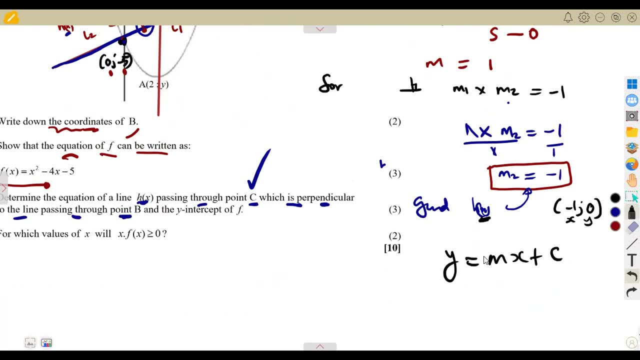 second line, which is zero, we can determine the equation of the line y. remember the equation of the line is given in the form of y is equal to mx plus c. that is the gradient intercept format, where m is the gradient and we calculated the gradient minus one, x plus c, where you can calculate. 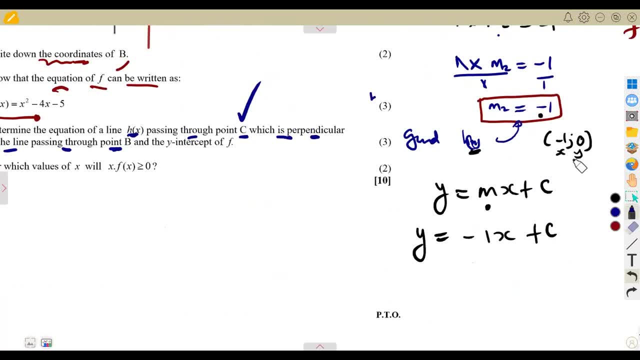 c from the point that you're given which lies on that line, y is equal to zero and x is minus one. that's minus one and hx is equal to c. so we have the gradient of the second line, which is minus 1 times x, which is minus 1 plus c. that's a positive 1 here. so that's a positive 1. so transpose. 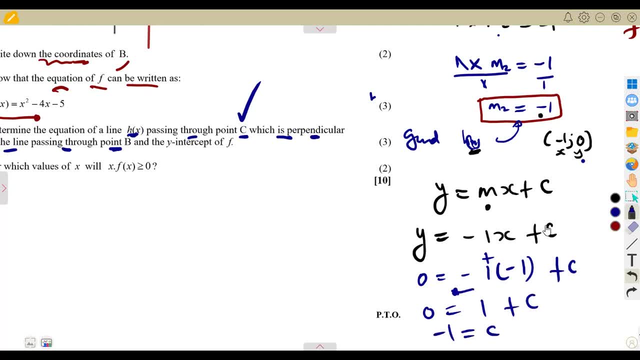 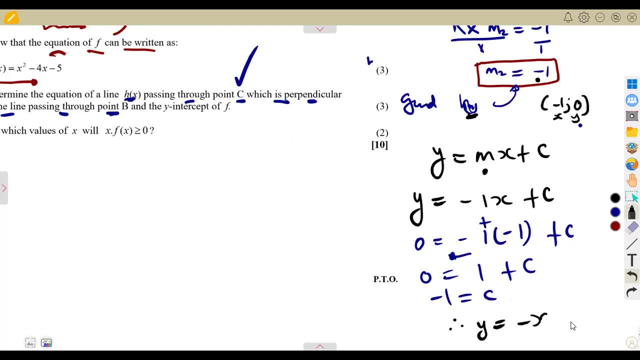 this, it will be a negative. 1 is equal to c, so if c is negative 1, therefore, our equation is going to be: what minus 1 x plus c, which is simply minus x plus c, which is minus 1 plus minus 1, is a negative. 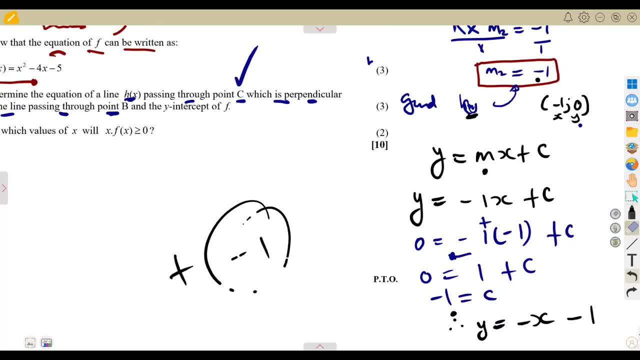 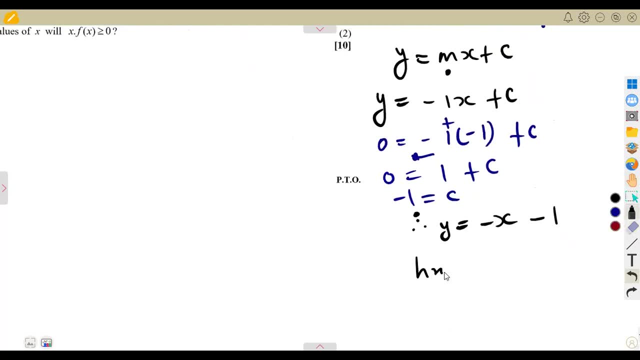 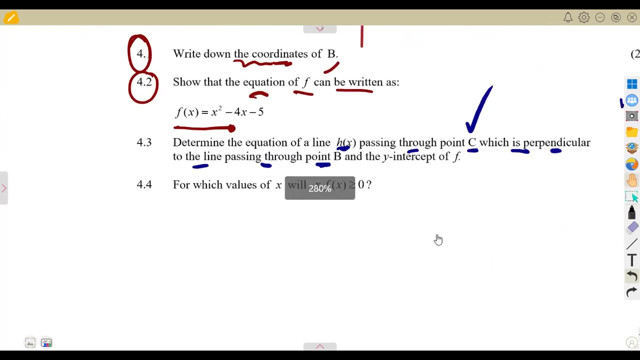 1. so we have got the equation of this line: hx. so that is y is equal to mx plus c, which is minus x minus 1. that was, that was the consideration, just like that. just like that. you just have to understand your functions, for which values of x is going to give us a value greater than or equal. 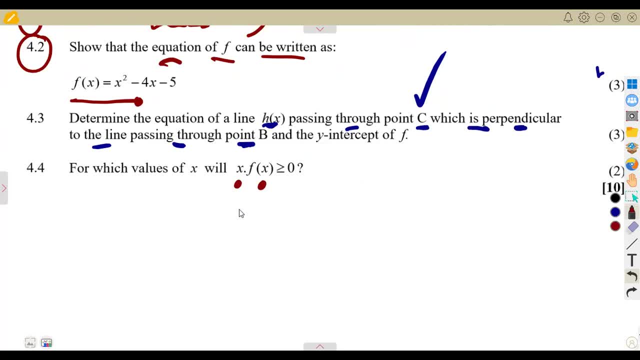 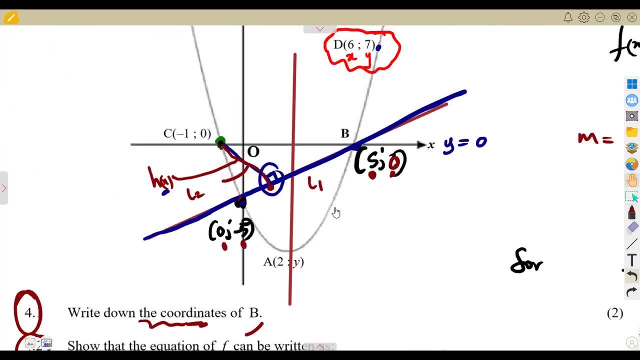 to zero the positive one. so we have got the equation of this line, hx, so that is y, is equal product of x to f of x. okay, the product of x to f of x or f of x is, uh, the function that we have here. so if you're to multiply this, it is simply a consideration like this. remember, we have got 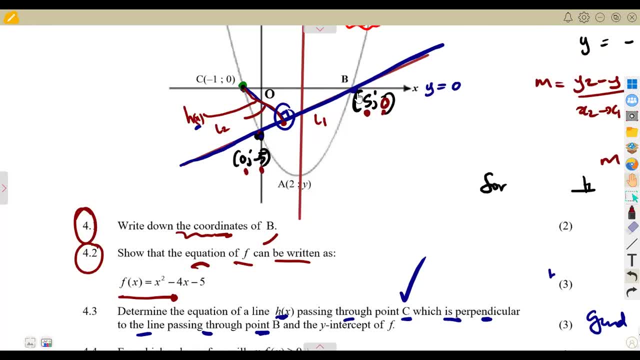 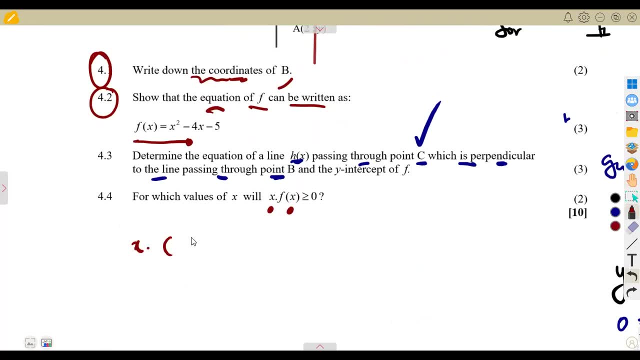 the solutions where x is what minus one and a five, so this one you can go back to your inequalities: the product of x times f of x, our f of x. don't worry about it, but we know that the product of these two that we are talking about, x and f of x, when you were to solve for an inequality, 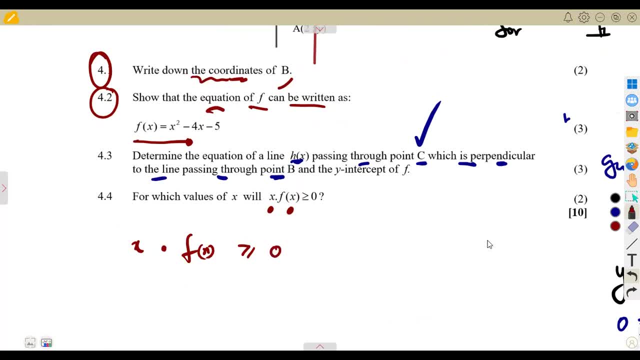 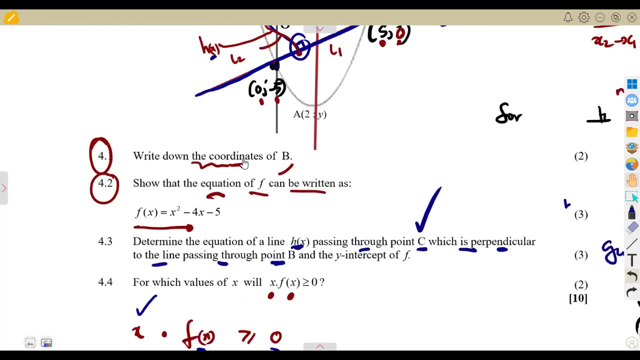 you were going to look for the critical values, which are a conditions where this is equal to you solve. so x at that moment was gonna be zero, or f of x must be equal to zero, and when f of x is equal to zero, that is where we have these solutions on our graph. 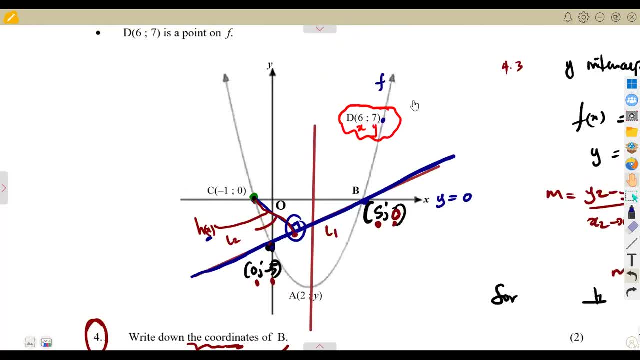 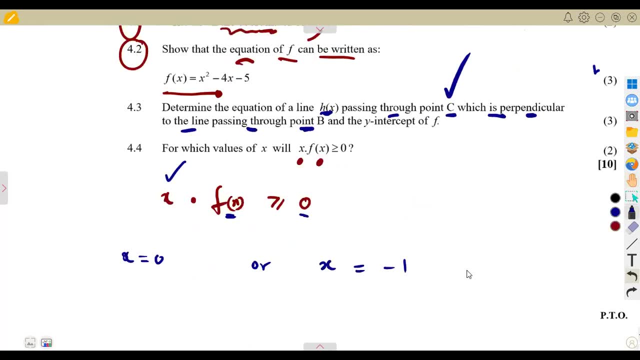 minus one and what, and a positive five. this is where we have our solutions at minus one and what, minus one and positive five. so we also have x, which is minus one, or x which is what, a positive five. so, at which point that you are going to take the x value and you multiply it to the y, uh, to the f. 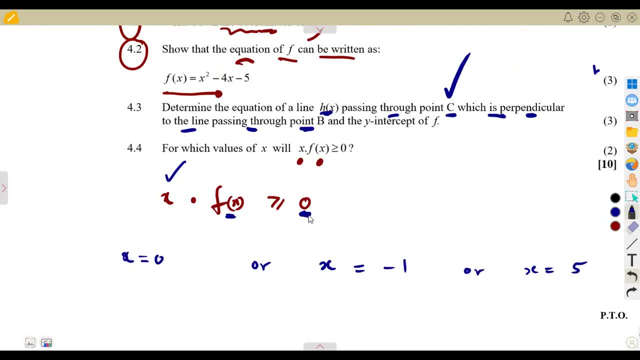 of x, so that your values will be what greater than greater than so. it's actually a trial and error that you're going to take between your values. all right, it's a trial error that you're going to take between your values, but you're going to see that in within these values of minus one. 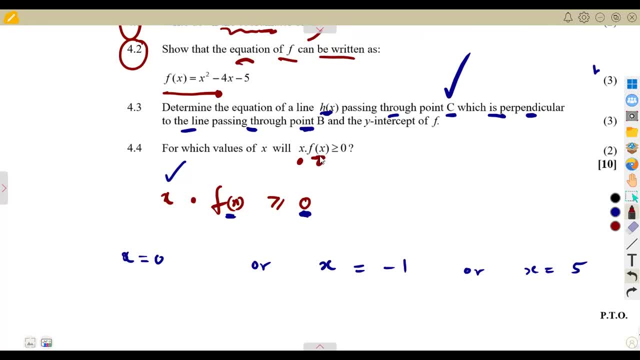 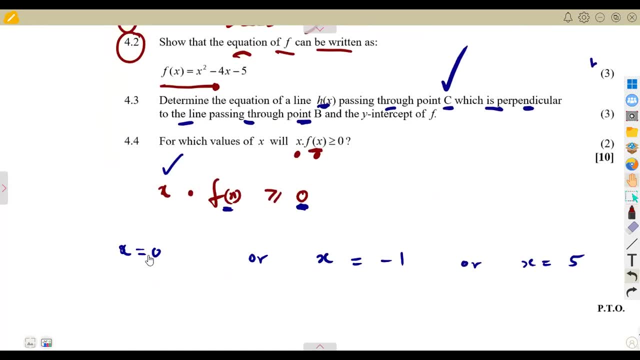 because you were given this. i want you to check your f of x. this is your f of x here. i want you to check: x is a certain value. let's take a consideration to say, uh, these are boundaries. let's hope you understand me, guys. this is minus one, this is a zero, this is a five. there are values which are less than one, which 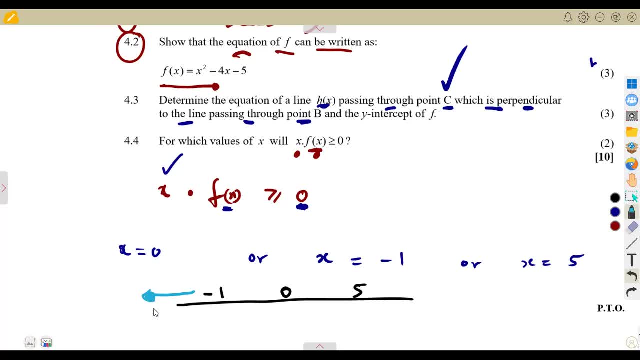 are this side. these values are less than one. think of a value which is there. let's say minus two. all right, i'm just taking a consideration. let's say minus two. okay, if we take values which are less than minus one on our graph here, values which are less than 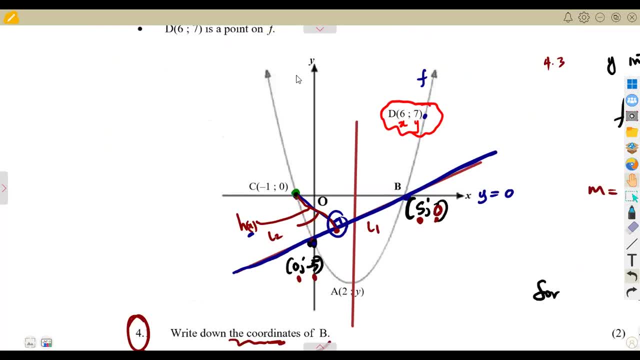 minus one. this is where we have minus one on our graph. here it's a critical value. that's why it's there on our on our graph, values which are less than minus one. these are the values here, these ones x values minus two, minus three. what is the function? how is the function presented? 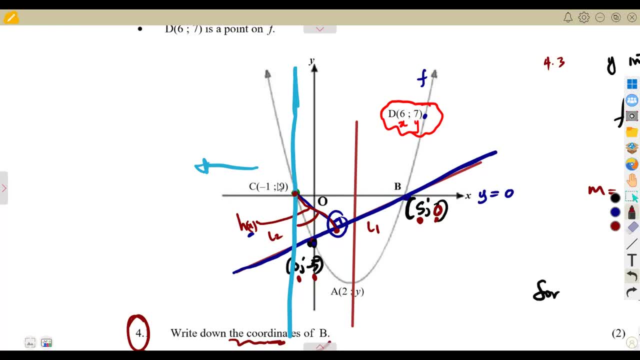 these values between. from these values minus one man, are we seeing that the function is above the x-axis, it's on top of the x-axis. so when this function is on top of the x-axis, it means our f of x is what is positive. our f of x is positive from minus one. going this side, your f of x is going to be minus one. 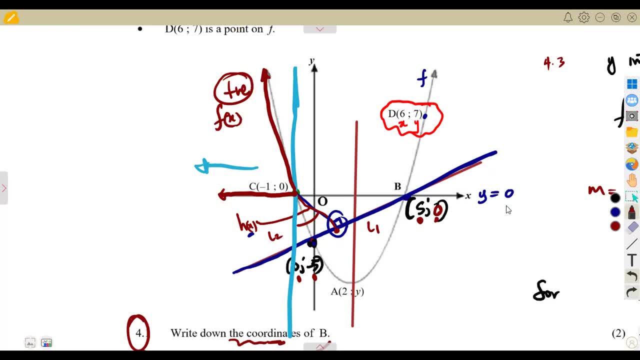 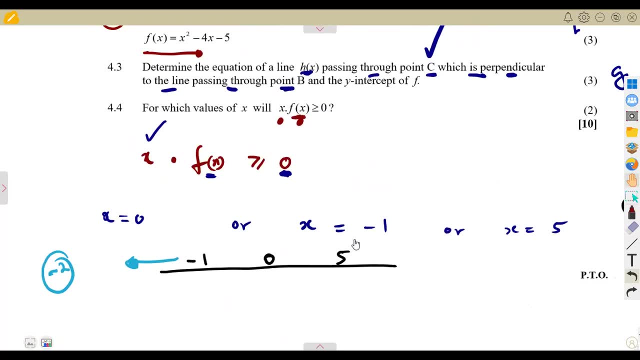 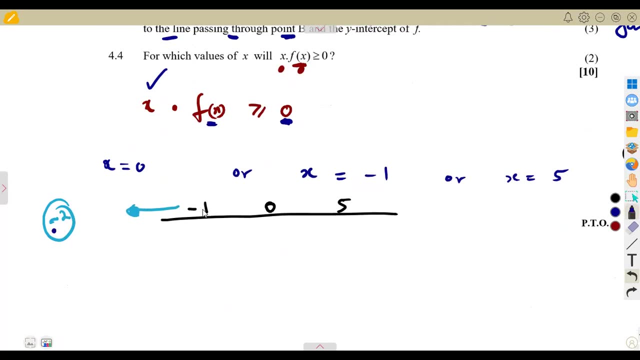 it is going to be positive on top. like that it is going to be positive. so let's go back now and conclude: does it satisfy this condition? because we are saying when x is minus two, these are values which are less than minus one. f of x at that condition is a positive value. this is your f of. 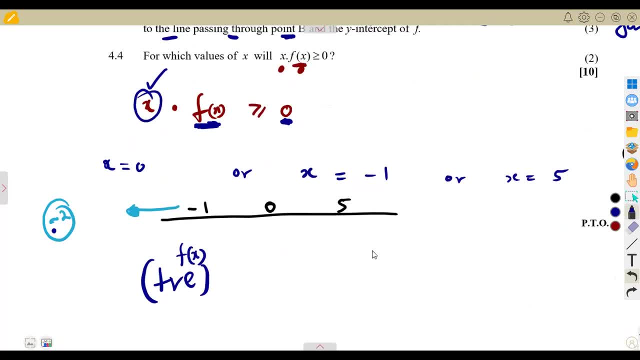 x, this one. but take note, there is an x which is multiplying your f of x and your x. now, because our x is less than minus one. so we can take any value, maybe minus two. so if you take a minor, it's a minus- this one. so your x is a negative value. 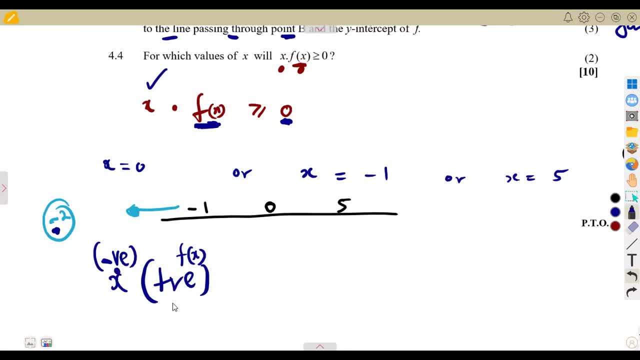 so a minus times a positive because your f of x. remember when we interpreted from the diagram, our f of x was what positive? so negative times positive. what do you have when a negative? we don't need to know the value, we just need to know: is it going to be positive or 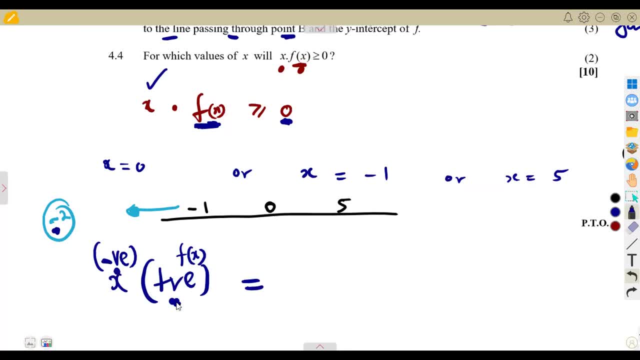 not so negative times. positive is a negative, so what does it mean a negative? these are values which are less than zero. but here they are saying: if you take that x that you are thinking of in that interval and you multiply it to the output which is your f of x, 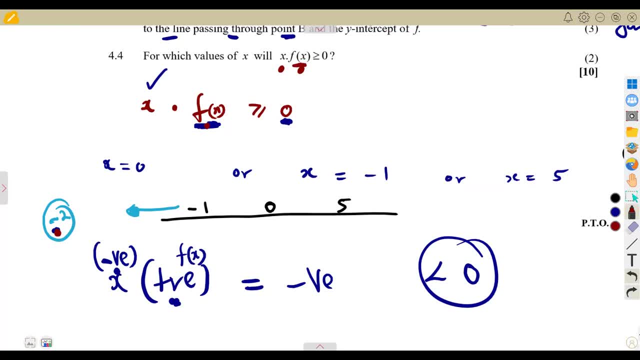 your values must be greater than zero, and to be greater than zero means these values are positive, but this one it is giving us a vice versa, it's a negative. so meaning to say: for all values which are less than minus one, for all values less than minus one, there is no solution there, there is nothing to take. there is nothing to take. 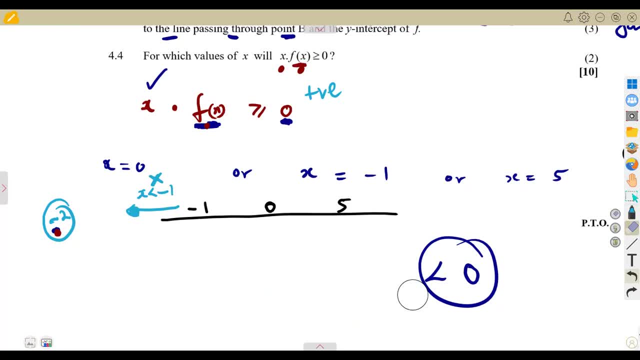 so there is no answer to that. so we can take a negative value and we can take a negative value. there is no answer there. there is no answer, there is nothing, there is no solution. so you move on again our x and f of x, so we interpret from minus one, going this side, these: 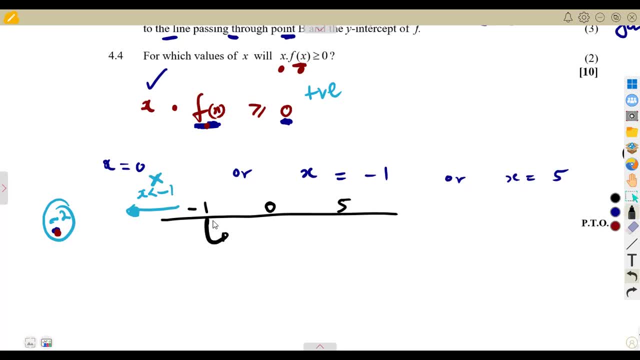 values. they are greater than what. they are, greater than minus one. so the question is: are we going to take from minus one to zero? are we going to take from minus one up to five straight? we have to interpret with what we are given from the diagram. okay, so let's interpret: from minus one to zero what is happening? from zero to five, what is? 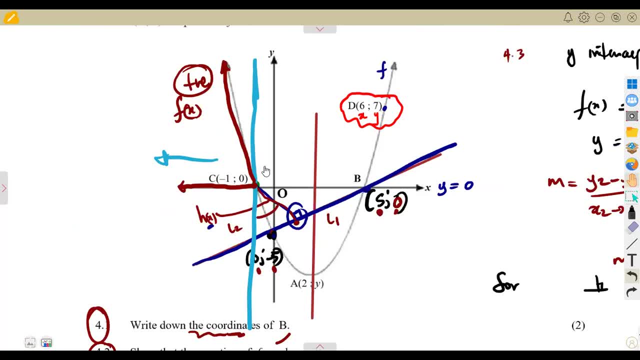 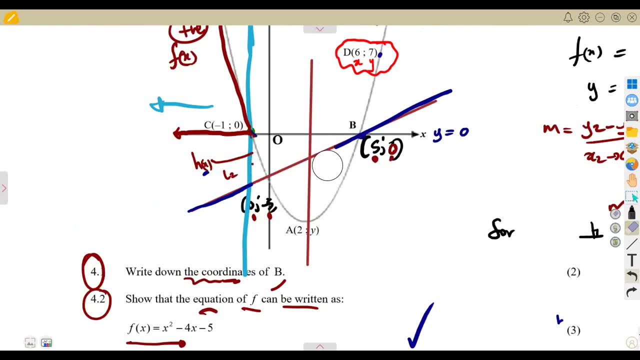 happening, so that we know: is it the whole function that we are taking? uh, that we are taking or not? all right, i'm just gonna erase this part here. i'm just gonna erase this part here, all right. so this is where minus one is and this is where a zero is, all right. 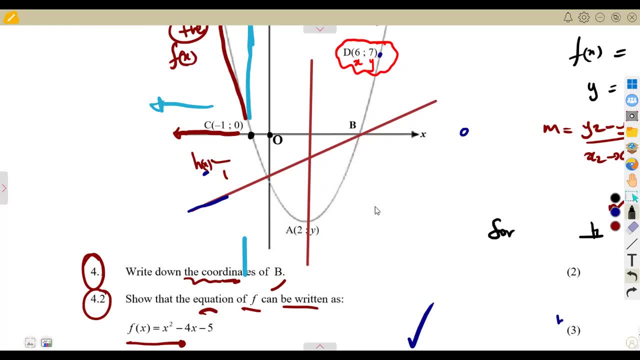 from minus one to zero. we can't use that to say we know that it was supposed to be values in between here. how do you write them? x is greater than or equal to minus one, less than or equal to what less than? or equal to zero? these values, they are in within minus one and zero. but as we check now, 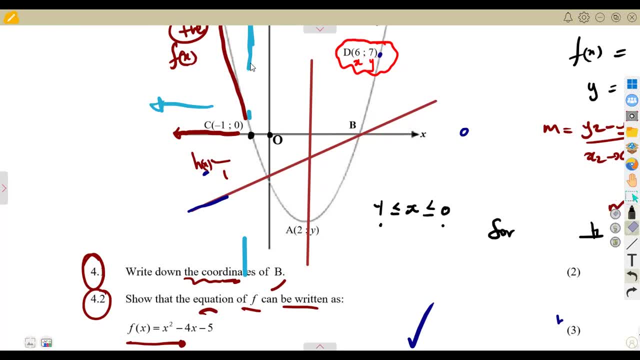 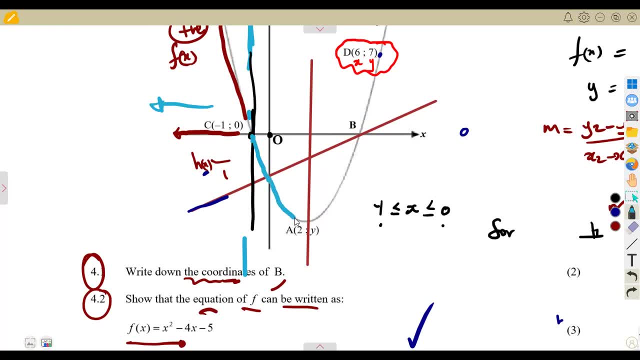 also below. it is also it, it is here, also here, guys, everywhere, f up to here, up to b, this function that we are seeing, our f of x from minus one up to five. remember, at b, here at b, it's five from minus one up to five, including even the zero there, including it. 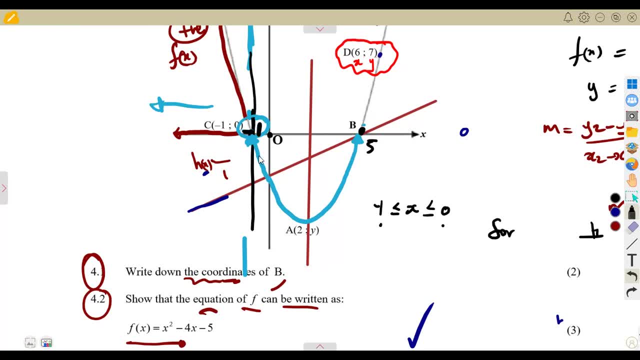 including even the zero. our function is what is a negative, but because a zero is a critical value, so we can also separate that. so it's: either we are going to separate or we take it from minus one to five. there's no problem, all right, but we have to consider: 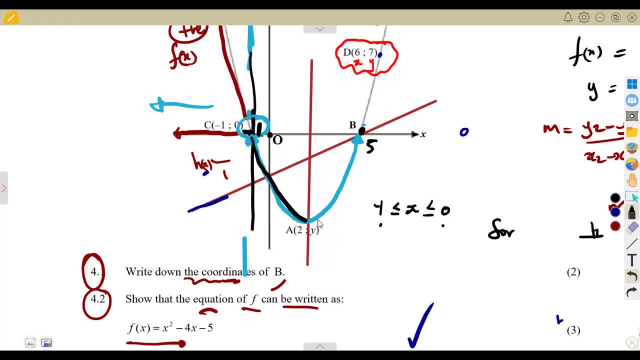 that we are going to separate from minus one to five, there's no problem, all right, but we have to consider that as a critical view. the function is still operating in the negative guy. this is what i'm saying from minus one up to five. so this is what we have. our f of x is in the negative. 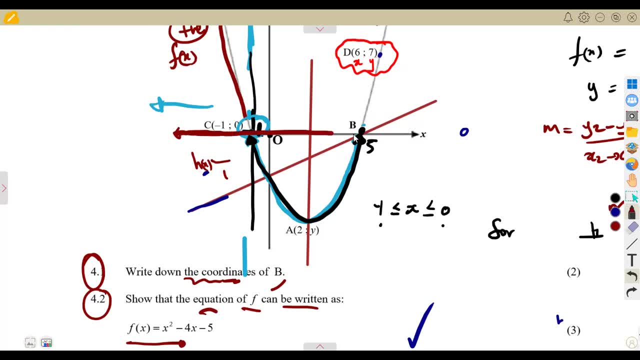 take note: it is below the x-axis. this or x-axis here, it's below the x-axis. so whatever that is below the x-axis, it means it's a negative. if you substitute anything within the this region, your answer will be negative only f of x. okay, this is what i'm trying to say, guys. 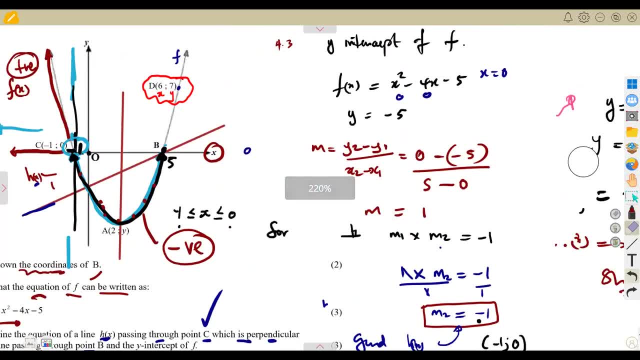 don't confuse, let's take our f of x. where is it this one? you understand me. you definitely understand me. this is our f of x. i want you to test any value. your f of x, which is y, is equal to x squared minus four. x minus five. just take any value from minus one to five. we can't. 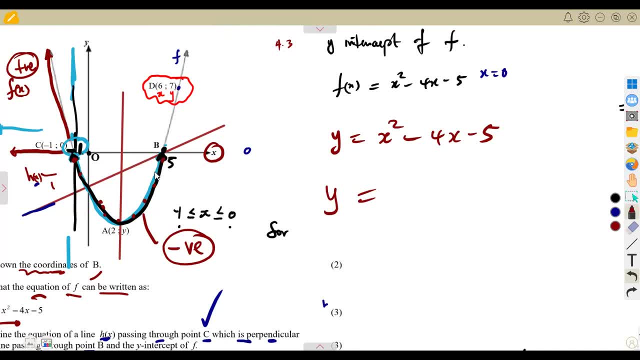 take minus one and five, because these are critical values. you are going to get a zero there, so use any value. you can choose one, you can choose zero. you can choose one, two, three, anything. okay, let's take one. substitute one here, substitute one here. this is going to be one minus four, minus five. 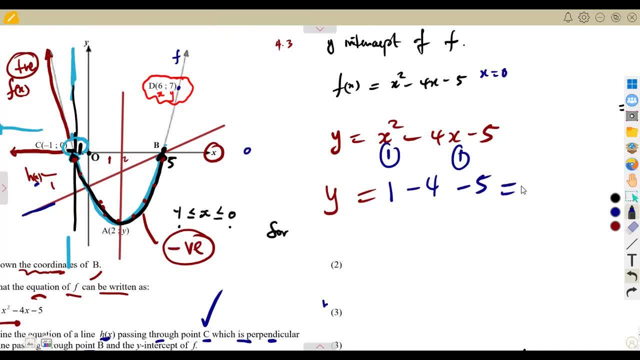 and you are going to get something like one minus four minus five, which is minus eight. why there is a negative? take anything, move on to two. when y is 2, you substitute 2 squared minus 4 times 2 minus 5, anything that you want. there you are going. 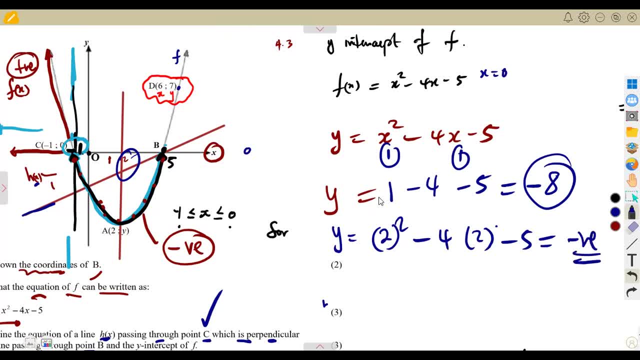 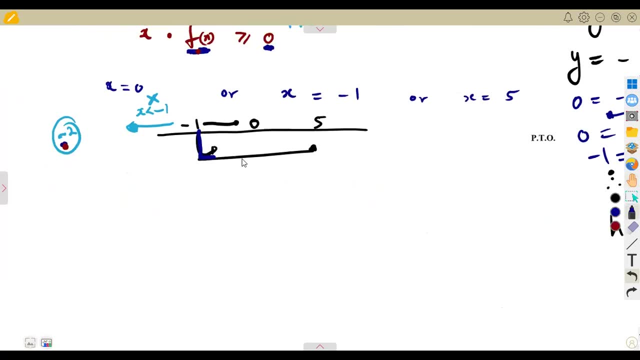 to get a negative answer. there. you will get a negative. so it means these values they are negative. f of x is negative. so let's, let's interpret now. so we say we are going to take from minus 1 to 5 and this interval, so between minus 1 to 5. how do you write this solution? you can write it this way: 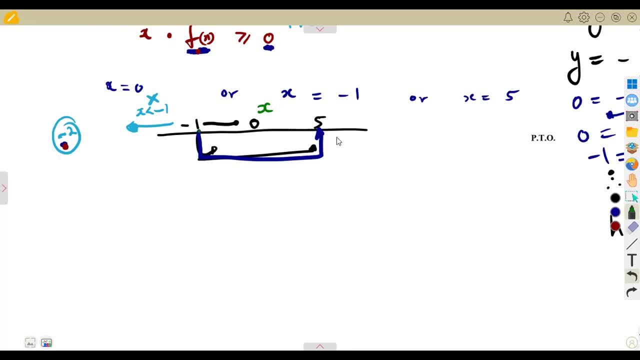 this is how you can write it: x between minus 1 to 5. also, 0 is there? so these values, they are greater than or equal to minus 1, because it's a boundary now, all right, great, uh, this is greater than or equal to minus 1, but less than or equal to 1 to 5. all right, why are we not taking greater? 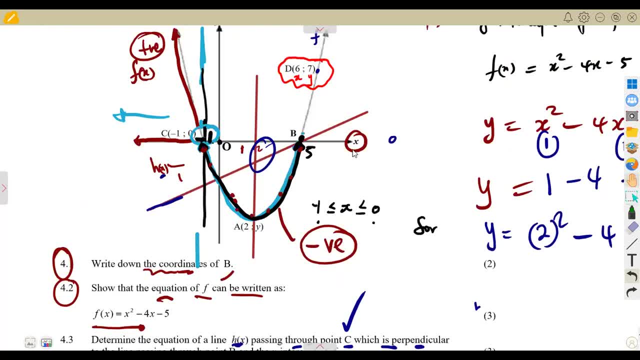 than this, this other side, because from 5, if you check from 5, our function is now above the x-axis. it's another region, so you have to work it on its own, just like what we did this side. it was on its own, so you work with region by region, region by region. so this is your f of x here, this one. 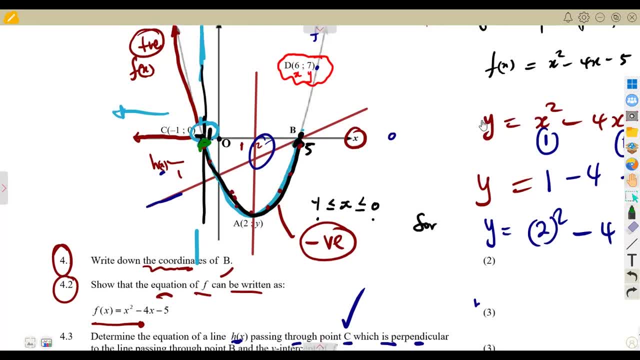 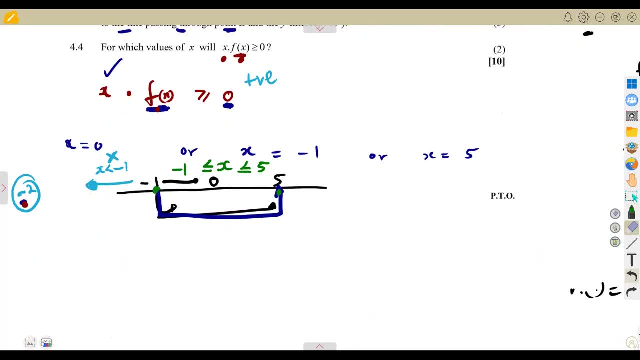 it's a negative, it's in the negative region. okay, so let's interpret: our f of x is in the negative region from 0 to 5. so here we see that our function is now above the x-axis to five. all right, our f of x, remember? the question is supposed to be what we are interpreting here. 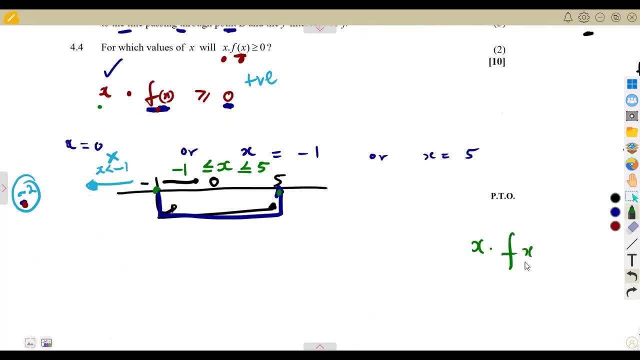 the product of x times f of x is supposed to be greater than or equal to zero. all right, our f of x in that region it was a negative. okay, this is our f of x. we saw that it was going to be negative. then we are taking any value that we have from here. we are going to take any value from: 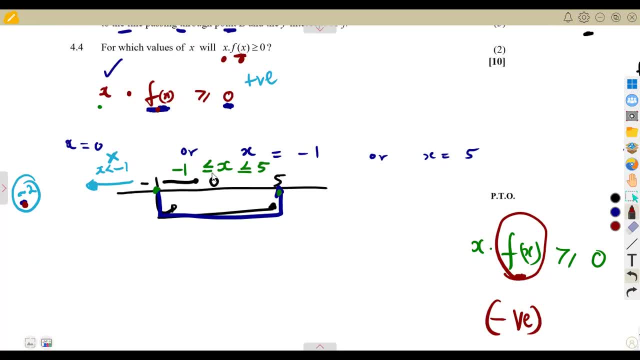 here, all right. so let's take a consideration of a minus one. if you take a minus one, a minus one, you are going to take a minus one there, a minus one as a critical value. you are going to see negative, negative, negative, negative. that's a positive. we are at zero there. 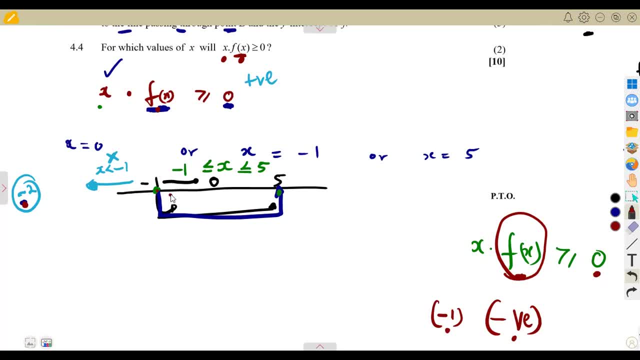 from minus one. you're going to see that minus one, minus are up to zero. these are negative. so in every negative is going to give you a positive meaning. to say a positive is something that is greater than or equal to zero. but now, as we move on to from zero, now, 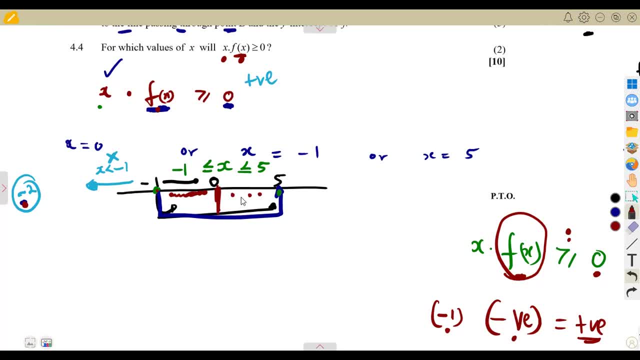 let's take when it is a positive: this one, our x now is a positive. let's take when it is a positive, this one, our x now is a positive. Let's take any value from 0 to 5.. From 0 to 5, we can take when x is 1.. 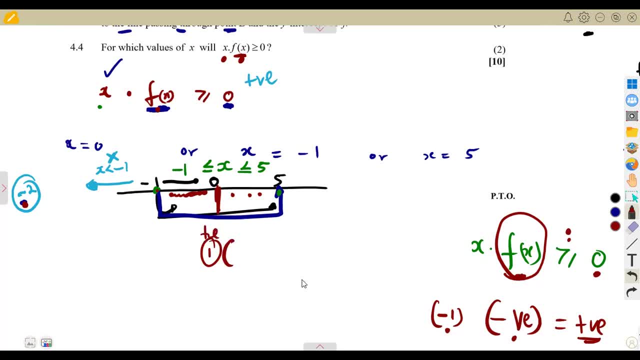 So when x is 1, you multiply: It's a positive, this one You multiply to f of x. Remember the f of x is still in the negative. Remember I combined everything. f of x is still in the negative. 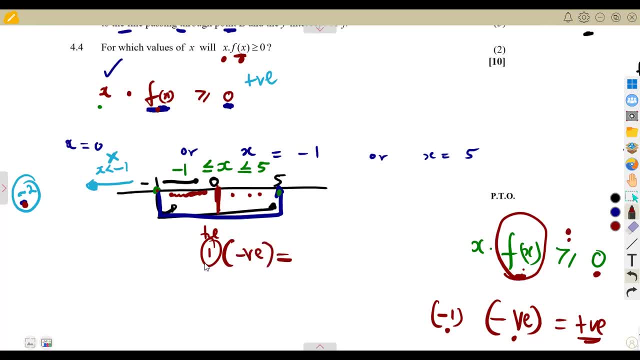 So it's negative there. Let's see what I get here. Positive times negative gives us what A negative It is no longer a positive. So meaning to say from 0, from values that are greater than 0 up to 5,. 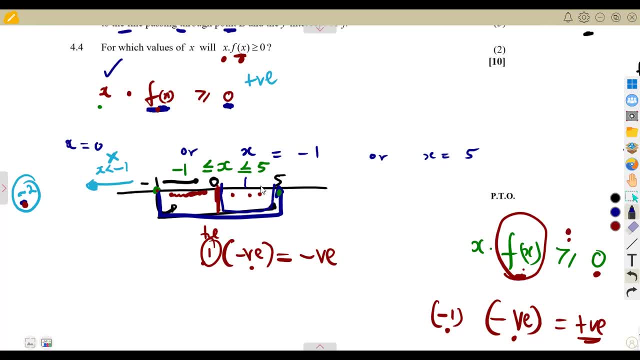 because 5 is a 1,, 2,, 3,, all these values of x. they are positive Because what controls at the end, guys, is that we are supposed to multiply by x. So we also have to interpret with x also. 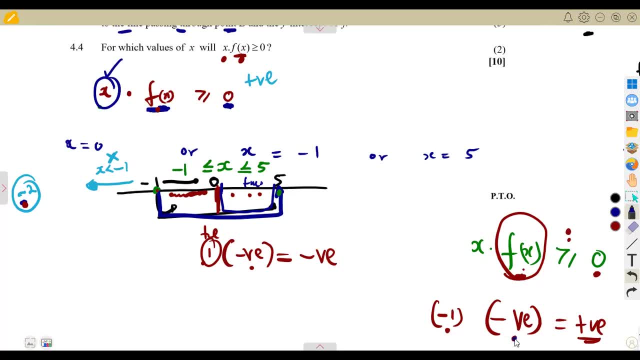 So x times f of x, which is a negative, Negative times negative is a positive. A positive is a number that is greater than 0. So meaning to say, from minus 1 to 1, if you take any x value there it is a negative. 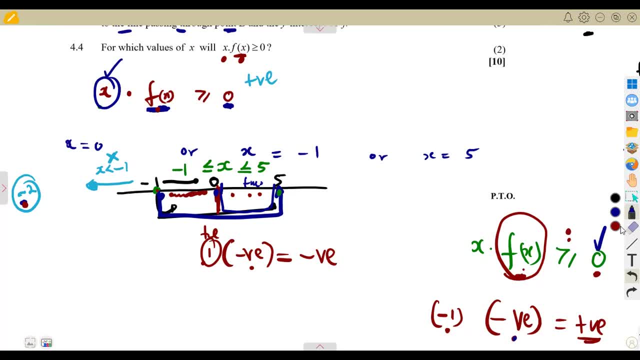 So negative times negative, you get what A positive. So we are going to take everything- this one, it's part of our solution- from minus 1 to 0.. x must be greater than or equal to minus 1,. less than or equal to 0,. 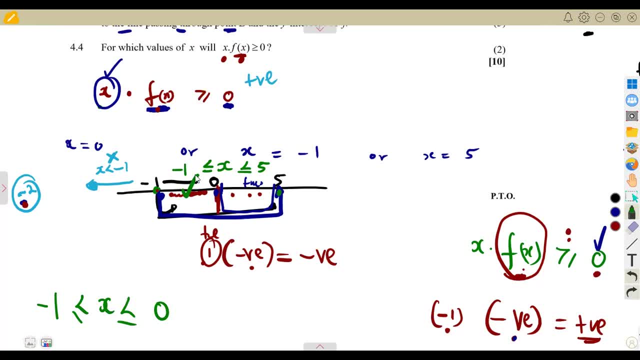 because there's an equal sign there. That is why we have to put this. But if we check along the same interval minus 1 up to 5, where we are considering our f of x, But the moment we move from 0, now it is not going to work. 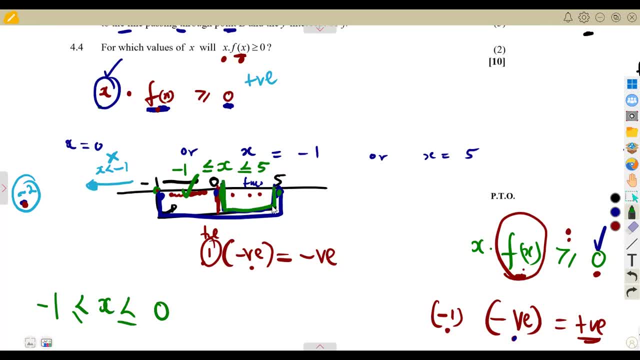 because these numbers they are for x. So if you take any x there it will be a positive, Positive 1, positive 2.. So positive times, negative gives you a negative. Remember before I said: this region failed because the resultant was a negative. 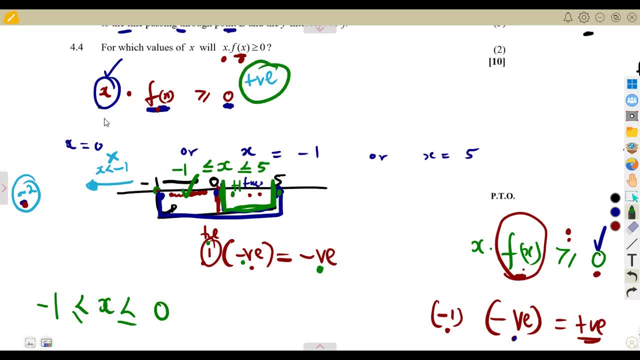 We are supposed to get a positive. We are supposed to get a positive if you multiply both x and f of x. So that's how you interpret. So from 0 to 5, there's no solution there, There's nothing. So this is our first solution. 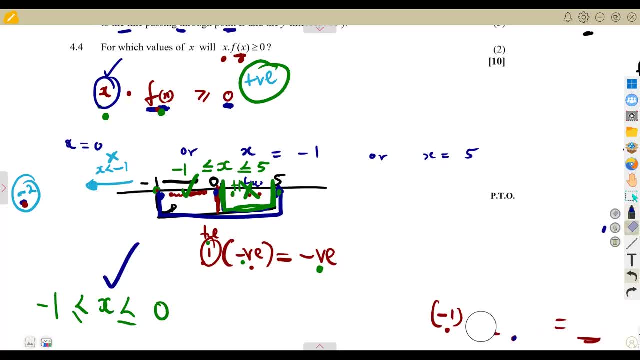 We move on. That's our first solution, this one. We move on to the other one. Which other part is left now? from 5 going onwards? These are values which are greater than or equal to 5.. So let's interpret what is happening on our diagram. 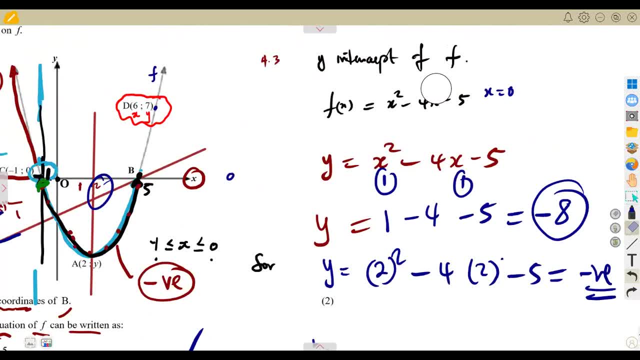 These are values which are greater than or equal to 5 on our diagram. All right, Let's just remove this. Let's not be confused with a lot of information there. Let's hope guys will be able to finish up because you know these softwares: they tend to misbehave when you record a lot of things. 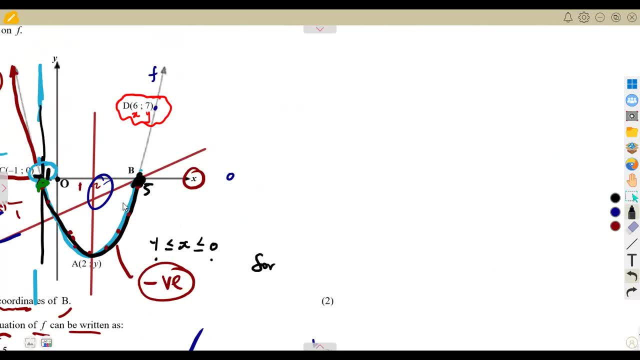 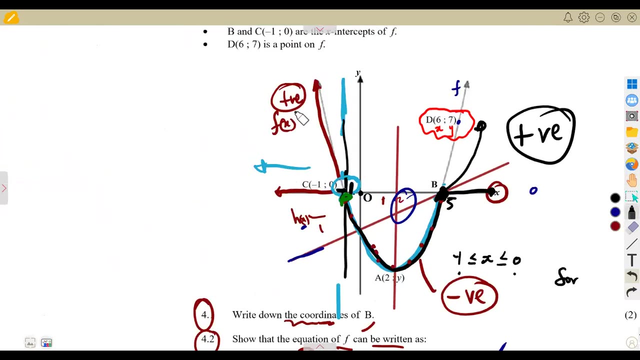 All right, Like I said, let's interpret from 5.. From 5, our function is above The x-axis, meaning to say our function is now positive, just like what it was before. here Our function was positive, But what made us not to take this? 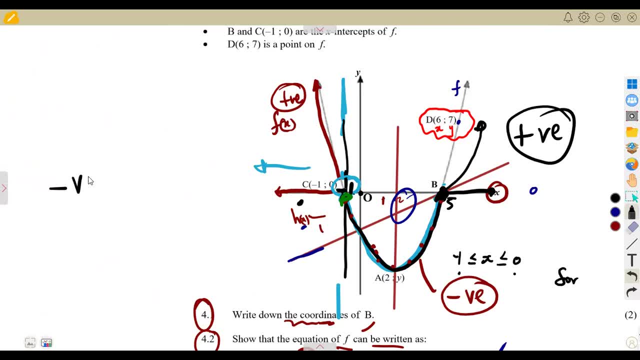 It is because of the x value. The x was negative, Even though our function was positive. we are going to get a negative answer, which is wrong, because we want a positive answer. So this time let's interpret Our f of x is positive, just like what we had this side. 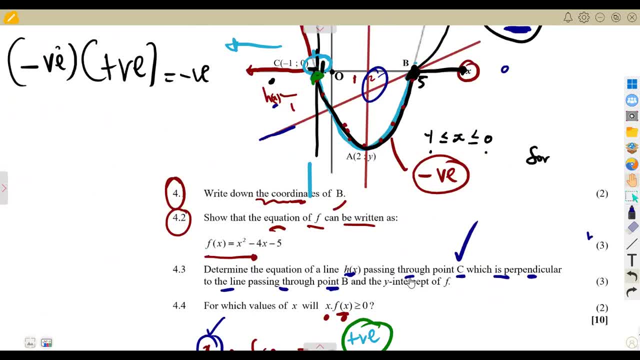 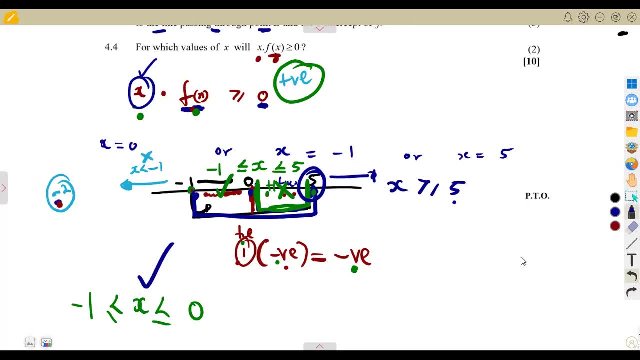 It's above the x-axis. All right, So this is it From that interpretation of values which are greater than 5, x times f of x, Our f of x. we said it is what It is positive. Okay, What about x? 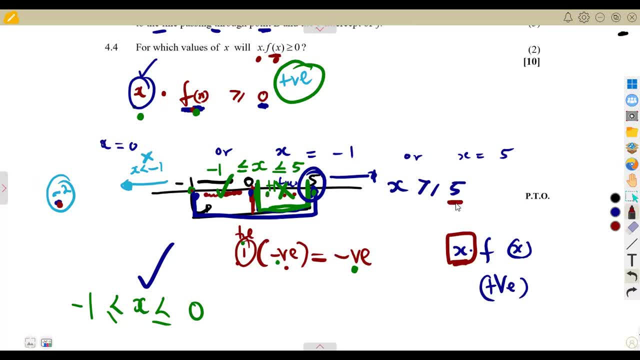 If we are talking about values which are greater than or equal to 5, are these values positive or negative? They are positive: 5., 6., 7., 8., 9. We can't have a negative there. These values will be positive. 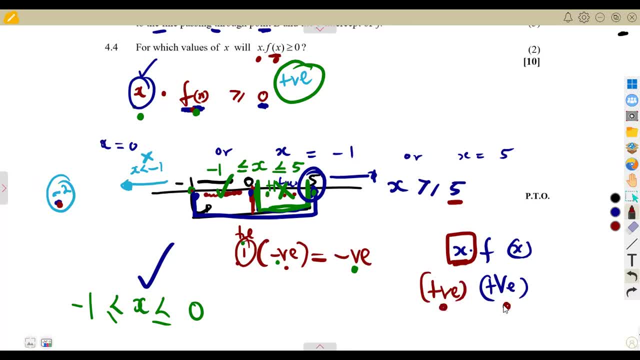 So this time there is positive times, positive. What do we get? A positive. When it multiplies a positive, you get what A positive. That's how we interpret So meaning to say: this is correct: we want it because we want something greater than or equal to 0. 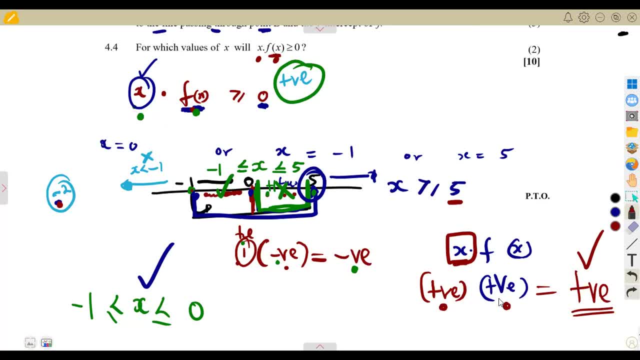 after multiplying these two. After multiplying these two, we must get a positive, And this is exactly what we are having. So, meaning to say, values greater than or equal to 5 are also part of our solution. So also our x was going to be what? 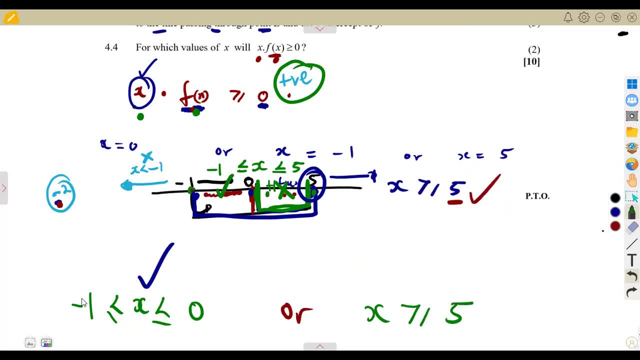 Greater than or equal to 5.. Can you interpret that? So if you are now, if you are now used to these functions, you won't even like, do like this. You just say, okay, just look on your diagram, Okay, this is happening. 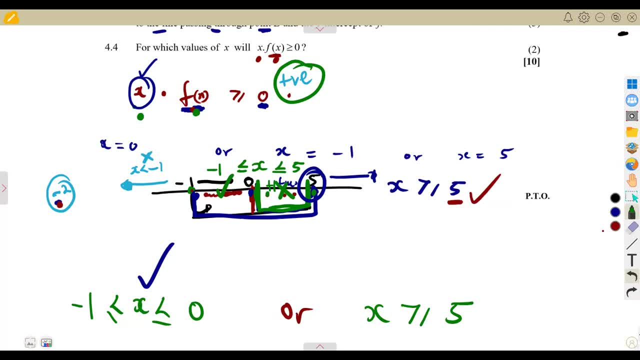 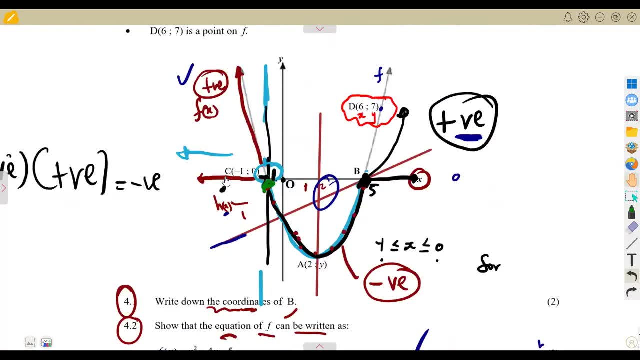 You just look on your diagram, But I'm explaining this so that we all understand. So that is it. You can just interpret on your diagram, Is it? What is it that is happening from year to year? If I multiply by negative, okay, it's negative. 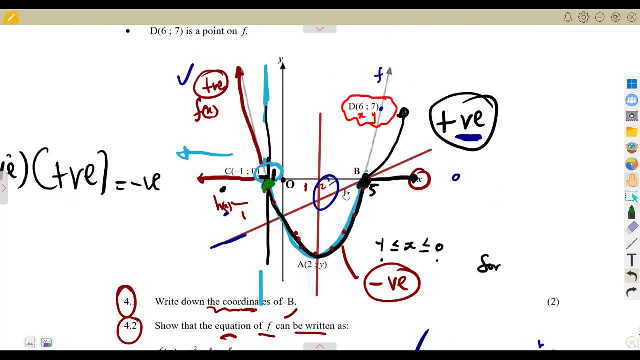 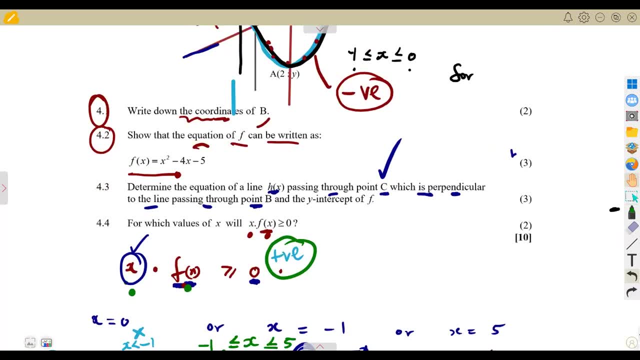 I leave it. I move on from minus 1 to 0.. I move on from 0 to 5.. I move on from 5 going onwards Straight from your diagram. you can do that. So that was it: 10 marks on everything on this question. 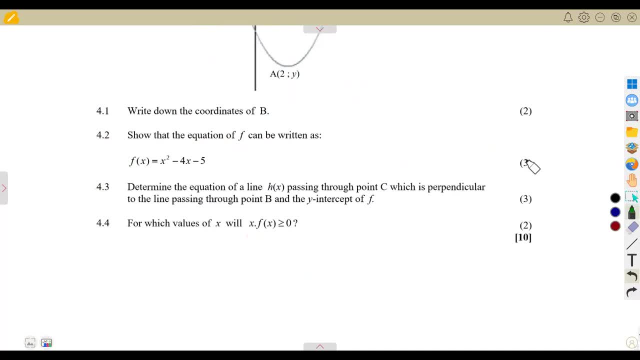 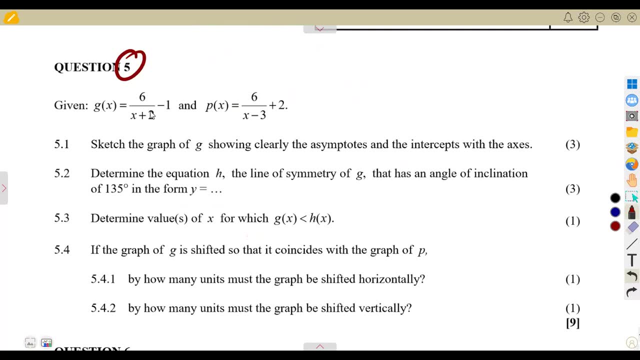 That is how they can ask these questions. Just have to be careful from there. Question number six. Question number five: I mean, given gx, which is 6 over x minus x plus 2 minus 1 and px, Scratch these graphs. 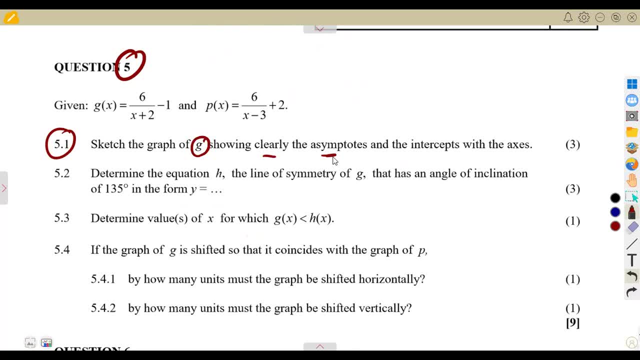 So clearly. they are simple tools. We need the graph of g, All right. We need to show clearly the simple tools and the intercept. So the x is 3 marks for that, All right. So this is our gx, the first one, 5.1.. 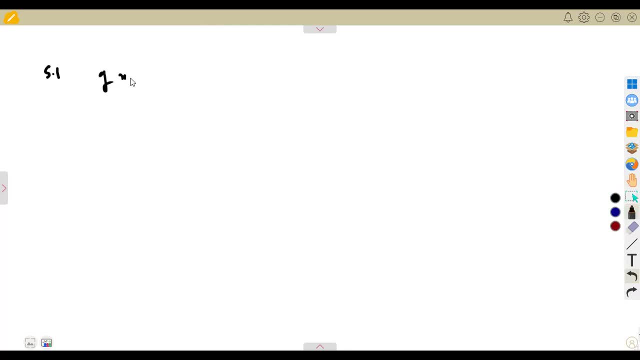 All right. So we need to sketch this graph of gx And gx is given as 6 over x plus 2.. This is a hyperbola. Remember on our hyperbola, if we are given f of x is equal to a into x plus p plus q. 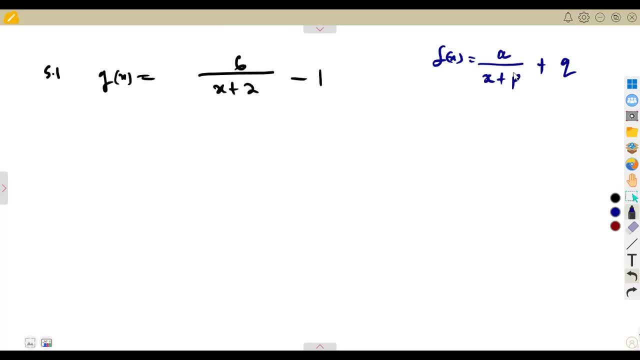 Let's say you wrote this way: It means that you're going to take this x equal to 0. It means it will be minus p versus q, like that. So this minus p versus q is the point, which is at the simple thoughts. 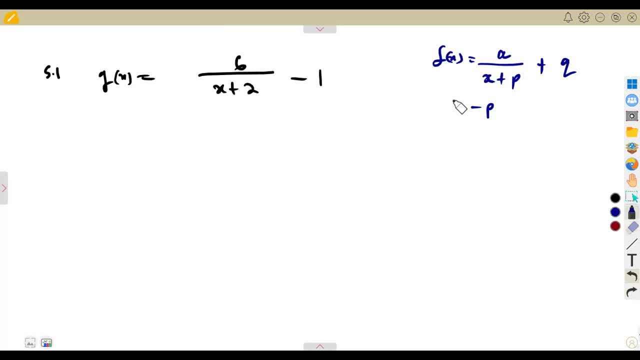 meaning to say: x is equal to minus p at the simple thoughts And y is equal to q at the simple. That is something that you just need to know. So meaning to say: for the equations of the simple thoughts, you just equate this to 0.. 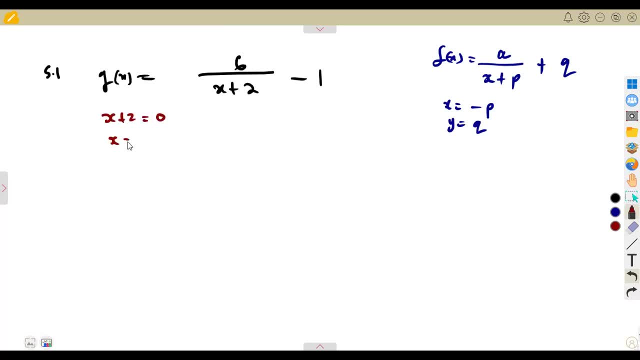 x plus 2 is equal to 0. So, So x is equal to minus 2.. The y value, as you can see, y remains as it is. Y is equal to q. It remains as it is. meaning to say: y remains as it is from your equation. 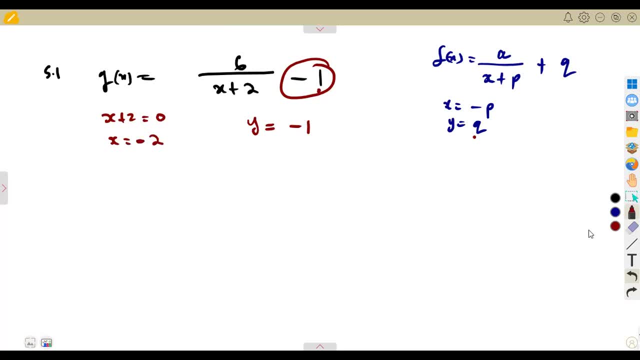 So we have the simple thoughts: This is where the graph is not going to pass, So we are going to need the x intercept. All right, The x intercept on a condition that we know that it must be. y is equal to 0.. 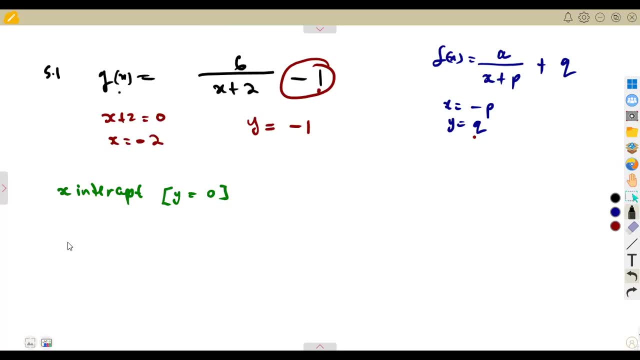 So if y is equal to 0, what are we going to have? That's, 0 is equal to 6 over x plus 2 minus 1.. So this transpose the minus 1.. This side has a positive which is equal to 6 over x plus 1.. 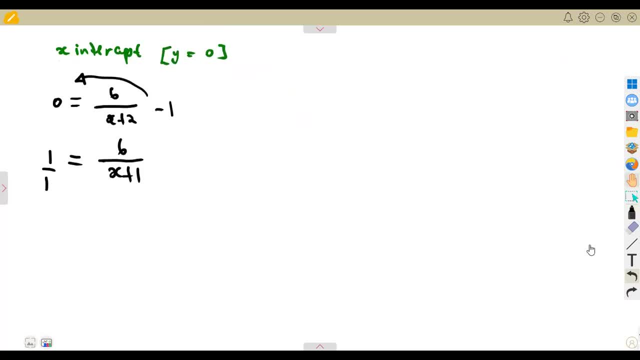 1 as a fraction is same as 1 over 1.. So how can I calculate for x? I can just cross multiply 1 times x plus 1.. It remains as it is. x plus 1 is equal to 1 times 6, which is 6.. 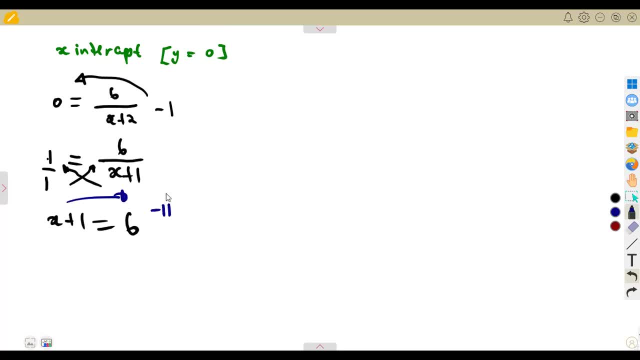 So if we are to transpose the 1 to the other side, that will be a minus 1 on the other hand. So that means x is going to be 6 minus 1, which is 5.. So this is what we are going to have at the end. 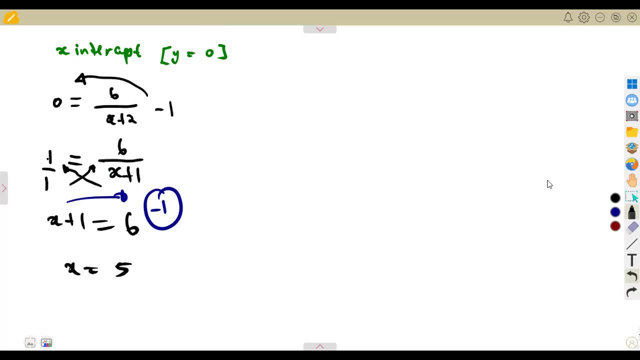 This was x plus 2,, guys. You see now the way that I'm saying this. now. your teacher is now tired. This is x plus 2 here, So that's x plus 2 here. So it will be 6 minus 2.. 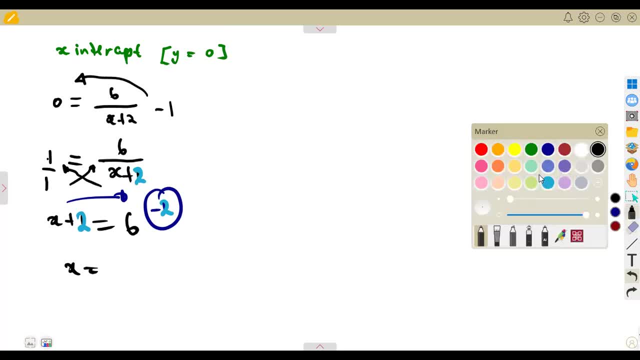 And 6 minus 2.. Let's correct this one. That will be a 4.. Okay, So that is. x is equal to 4.. So that will be our x intercept: 4 versus 0.. The y intercept with the same consideration. 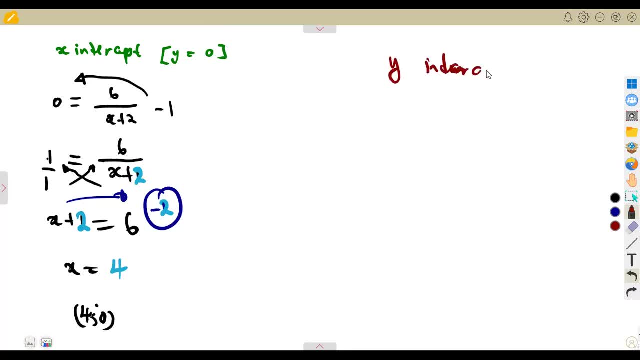 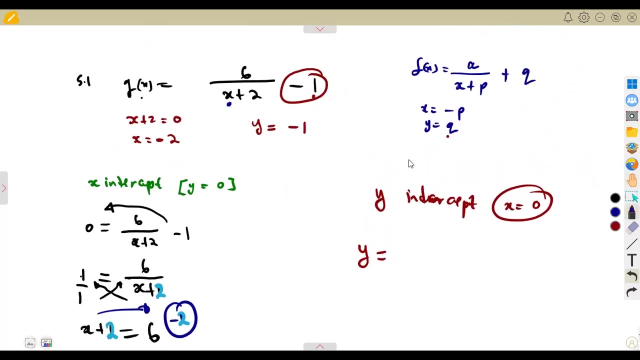 We are going to see that for the y intercept, the condition is x must be a 0. So y is equal to. in place of x, You are going to substitute what? as 0? in wherever there is x, You are going to substitute as 0.. 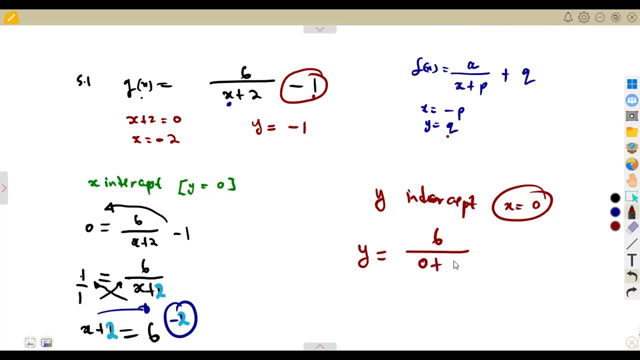 So that means y is equal to 6 over 0 plus 2 minus 1.. So on this one, there is no transposing, There is no this and that. Just use your calculator as it is. It's going to be something like a 2 there. 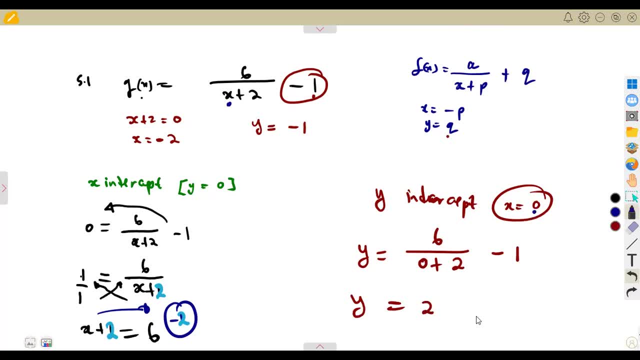 So that will be 0, 2.. All right, Remember the x value, That's a: 0.. And the y: 0.. 0.. 0. 0.. So you can just write the coordinates, Then you can sketch your graph. 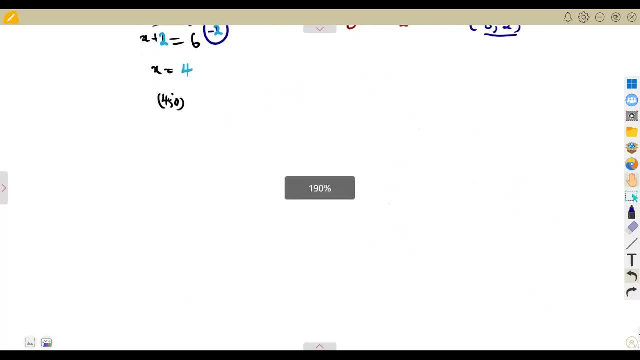 Remember, this is a hyperbola with the idea of a graph that you are to sketch. You can sketch any function that you're asked, as long you have the knowledge or the idea of that function. So we understand that a hyperbola is going to be something of this with our x and y axis. 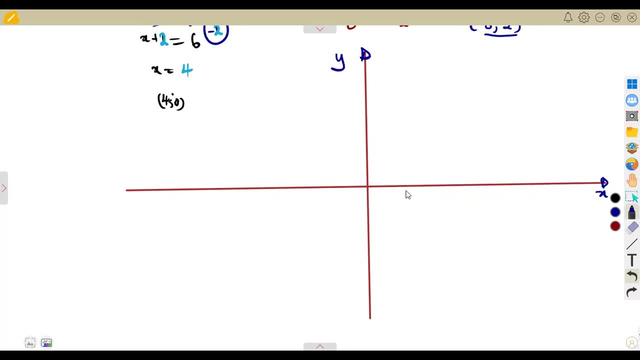 We are going to need first the asymptotes. So let's just say That's 0 here. 1, 2, 3, 4, 5, negative 1, negative 2, negative 3, negative 4, negative 5, and so on. 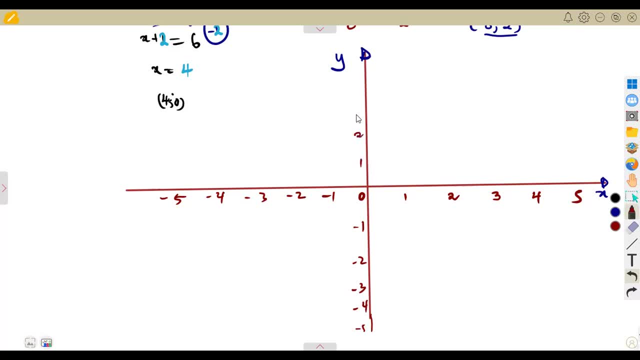 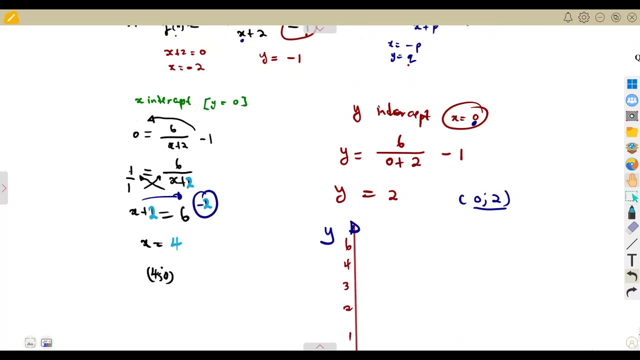 All right, So what you're just going to do is to mark your points and so on, and so on, and so on. All right, So first thing are the asymptotes, because that is where our function, where the function does not operate. The function does not operate when x is equal to 2 and when y is equal to minus 1.. 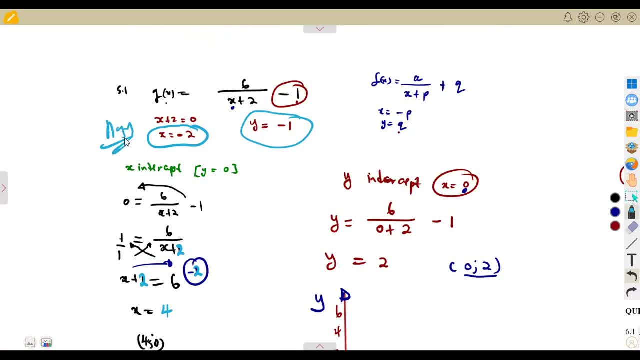 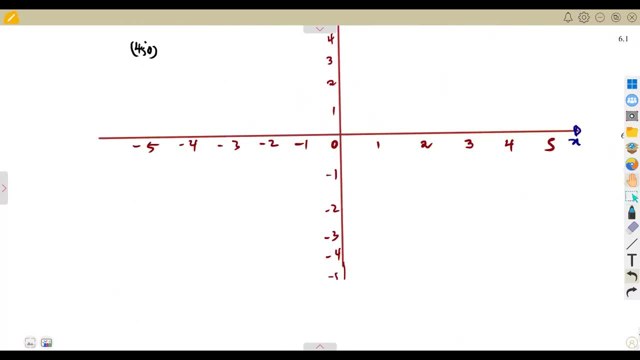 Remember, you're asymptotes. So x is minus 1, y minus 1.. So this is x which is minus 1 at this point. So where x is minus 1.. And what you're just going to do is to indicate a vertical line, guys. 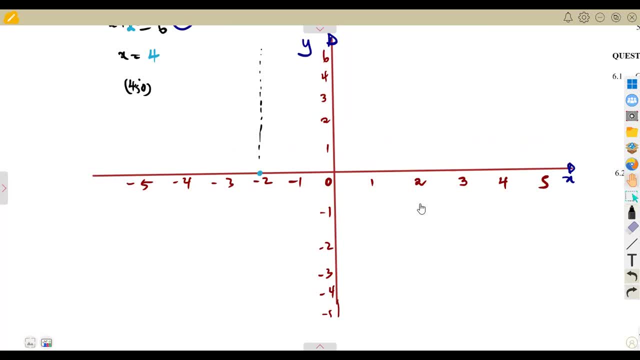 You see where I am. I'm right. I'm. I'm reading exactly minus 2, but I'm saying minus 1, guys, Sorry for that. So this is x, which is equal to what, Minus 2.. So we've got x, which is minus 2, y, which is minus 1, y is minus 1 here. 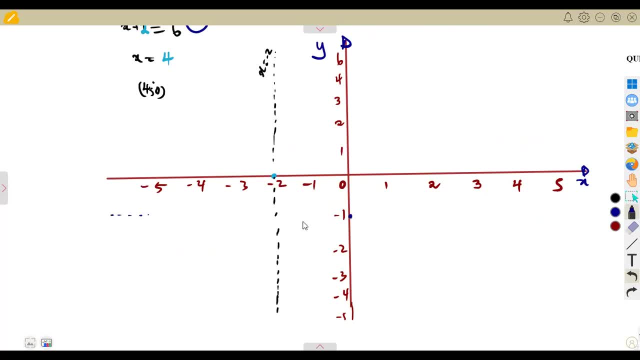 So you draw, Draw a horizontal line straight to pass through the minus 1.. So it's an asymptote. You can even use even your continuous lines. I'm not saying you're supposed to use a broken line. So this is: y is equal to minus 1.. 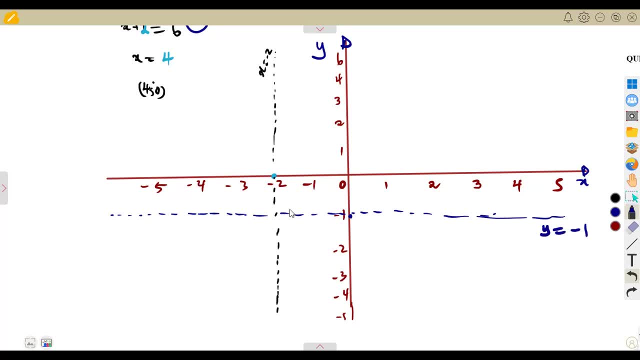 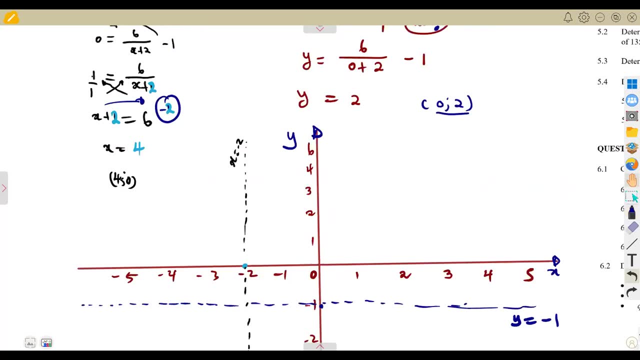 I just want you to properly see. So these are the asymptotes. So with this you are going to mark Our intercepts according to this: we've got the x intercept at 4 versus 04 versus 0, in the x axis at 402 for the y, which is 02 here. 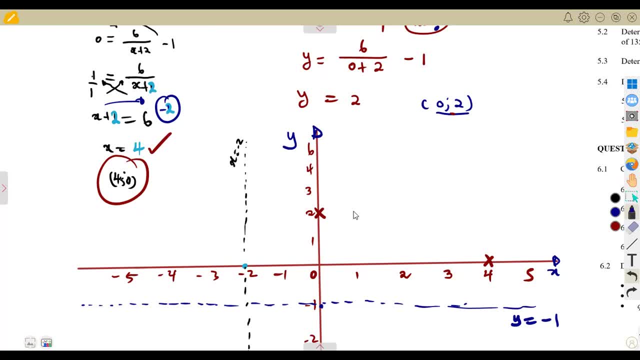 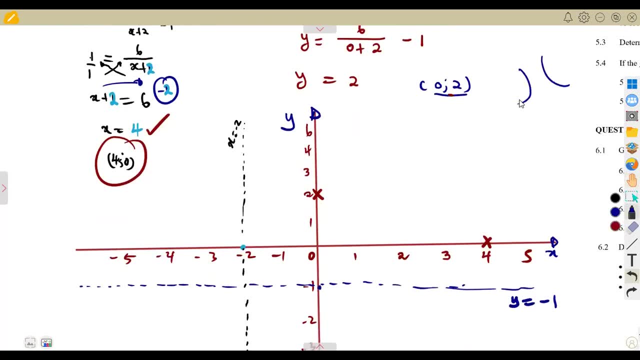 So they are just two points that we're given and they are just on the same side. So, with the value of a that we are given, it's a positive. We know that we are supposed to have a shape this side and this side, but they were just. 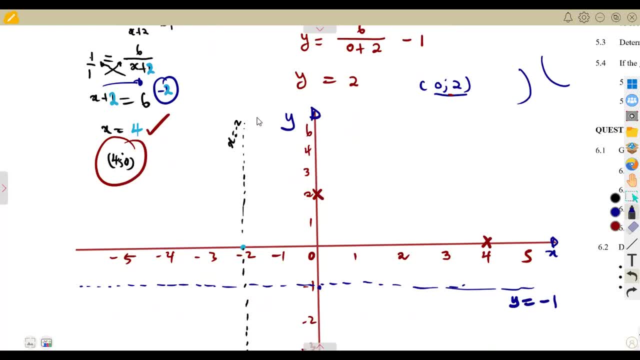 given two points, the y intercept and the x intercept, and they are both on the on one side of what of the function. So if you were to join your function like that, guys, okay, so it's gonna just stretch a little bit, just something like this: all right, going like that, tending to approach, 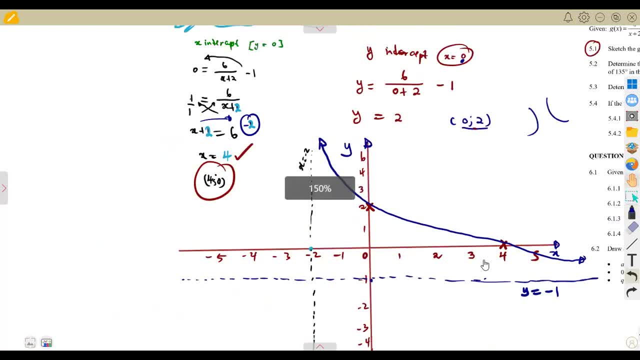 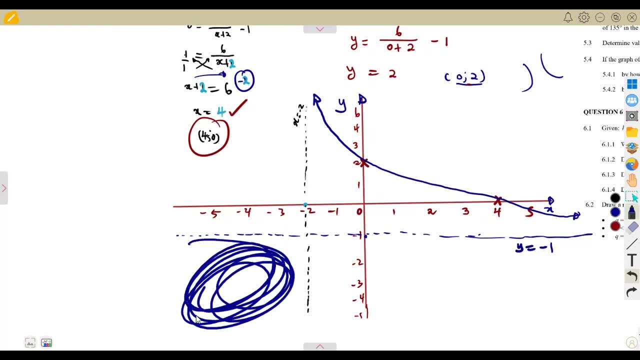 to y is equal to what minus one. we know that we are supposed to have two pieces, So the other piece is supposed to be in this region, this one. it cannot cross these asymptotes, So that is why we do not have the x intercept. 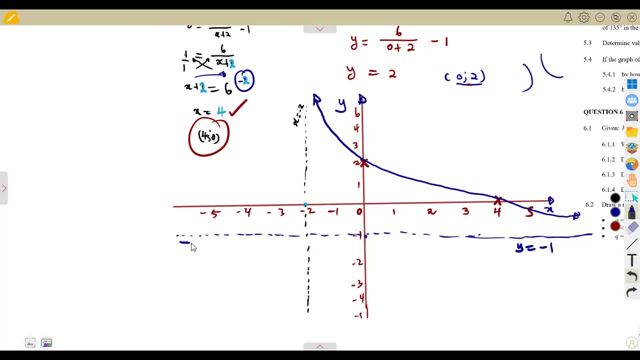 That is why we do not have, Okay, The y intercept, So our function is just going to be in within this region. you have to integrate it, indicate that, because you know the hyperbola, they are supposed to be two strips, one this side. 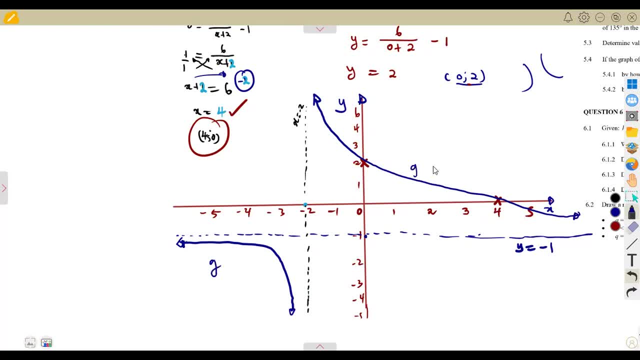 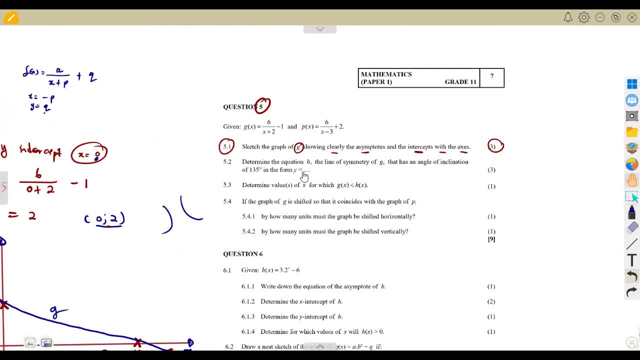 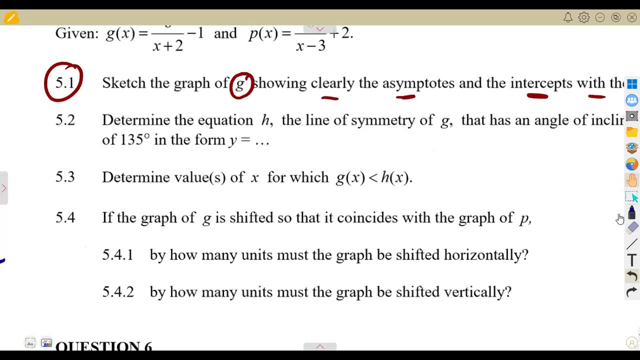 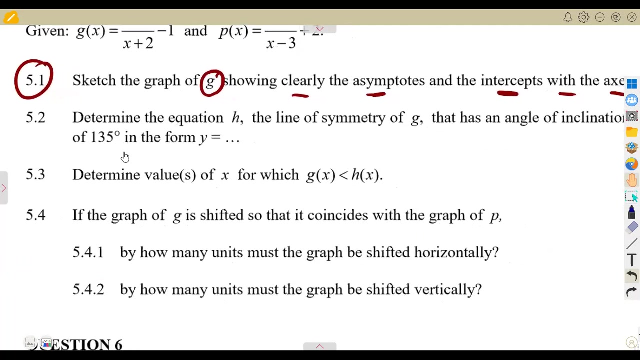 and the other one on this side. So this is our gym, Just like that. All right, You are done. Determine the equation of H. All right, determine the equation of what of H, ego, g, that is, an angle of inclination of what of 135 in the form of Y, is equal to that. 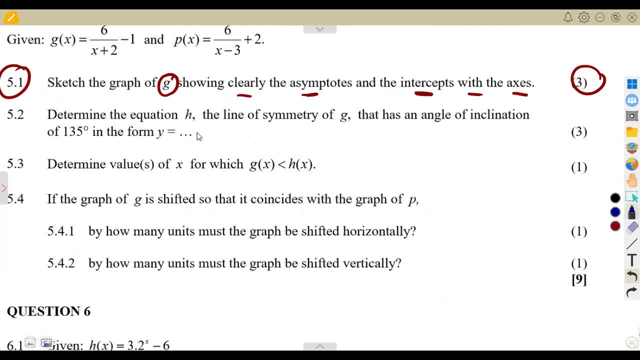 is equal to m, x plus c format. So they are saying we are supposed to determine the equation of H. the line of cemetery of g- remember that whenever you're dealing old, you're working with the hyperbola. the line of c matrix of G. remember that whenever you're dealing all, you're working with the hyperbola. 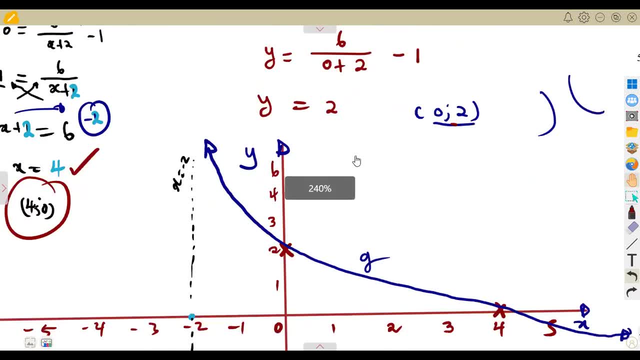 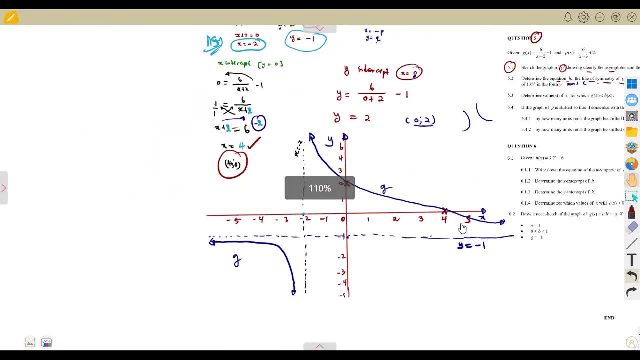 the line of symmetry of G in the measurement of x. you're going to tell the linear curso in both To the line of symmetry is found at, or is drawn or is actually found from where? From the asymptotes At the intersection of the asymptotes. all right, 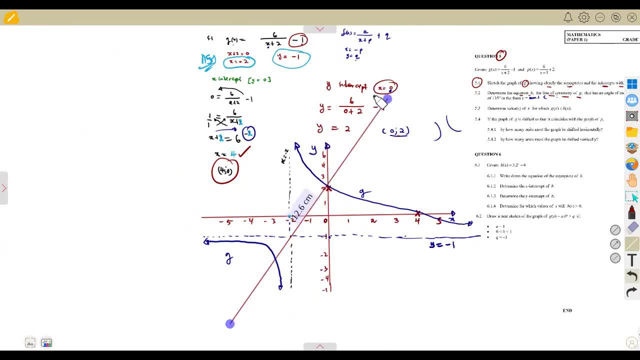 We do not know is it going to pass through which point, but here's just a sketch like this: These were supposed to be our lines, But in this case we are not going to work with both lines, because we are told this one. 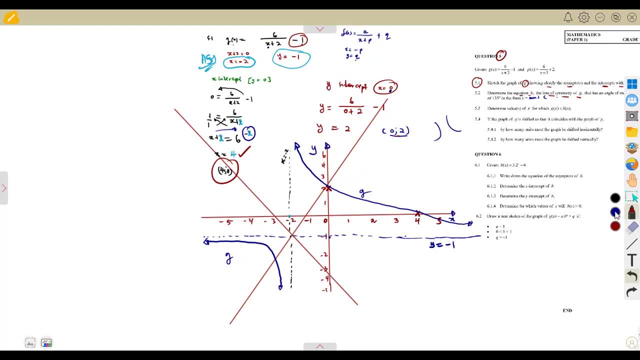 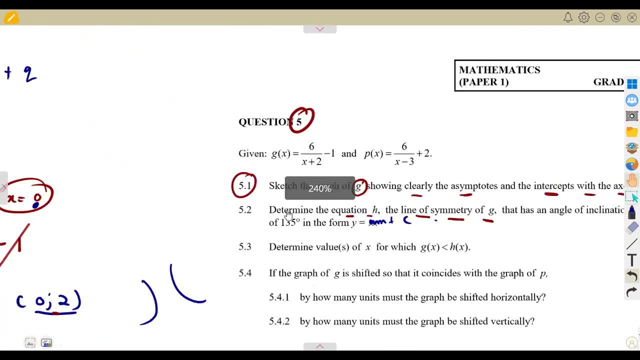 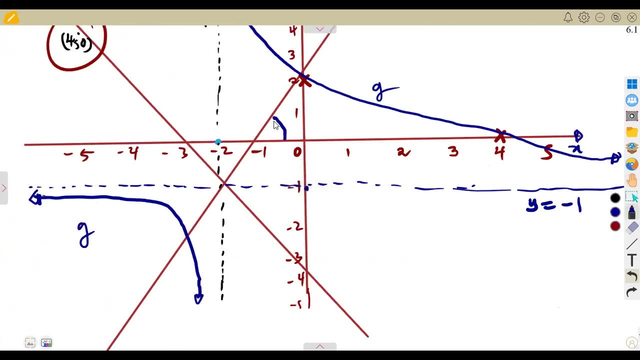 it has an angle of inclination of 135 degrees. It has the angle of inclination of 135 degrees. So we can't say this line has got an angle of inclination of 135.. Guys, this is an acute angle, this one. So this is not. 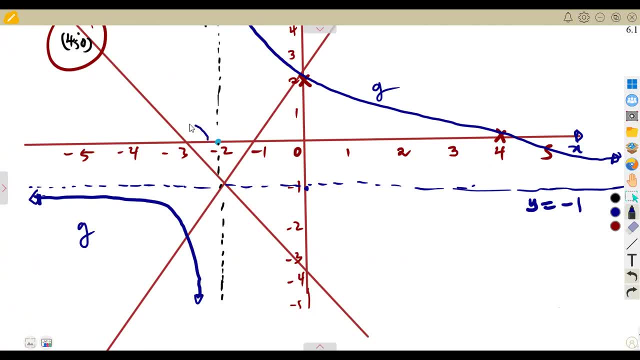 The one that we are talking about is this one with an obtuse angle, the angle of inclination between the line and the positive side of the horizontal axis. So this is the one that we are talking about. So let's say: this is our theta. 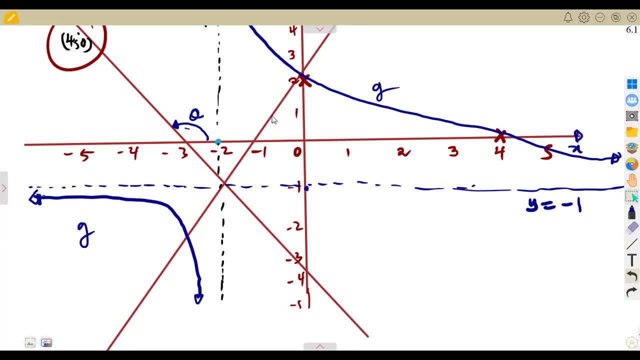 So meaning to say: if this is the one that we are talking about, we need its equation now. So this one is not there. I'm going to remove this. So we are going to need its equation. So the question: how are we going to determine the equation? 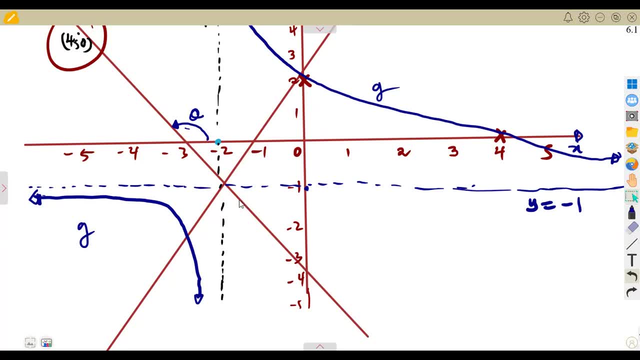 For the equations of these lines, the axis of symmetry of a hyperbola. they are just two things that you need to take into consideration. All right, I want to remove this, guys. Let's just hope you win, All right. 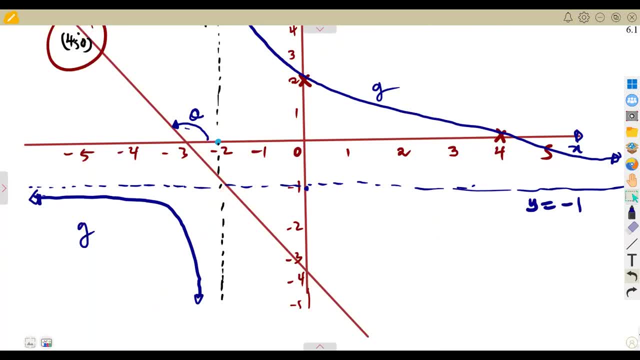 Okay, Okay, Sorry for that. So this is it Okay. So this is it For the equation of this. these two lines, remember with this one that we remove with their positive gradient, they are just two formats for the equations of your axis of symmetry. 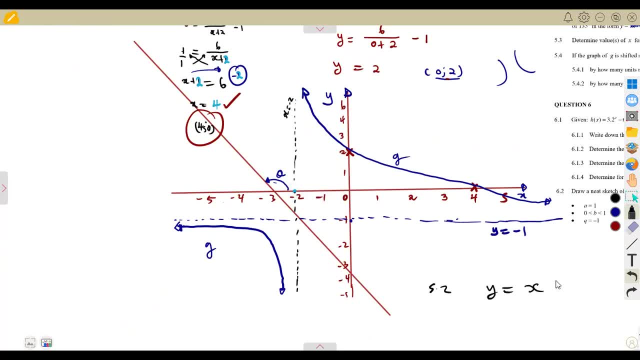 Which formats It's. either it is of y is equal to x plus c, or y is equal to minus x plus c. So that is for that. So the 135, they're just telling you is the one with the negative gradient, Even if you're to use a calculator. 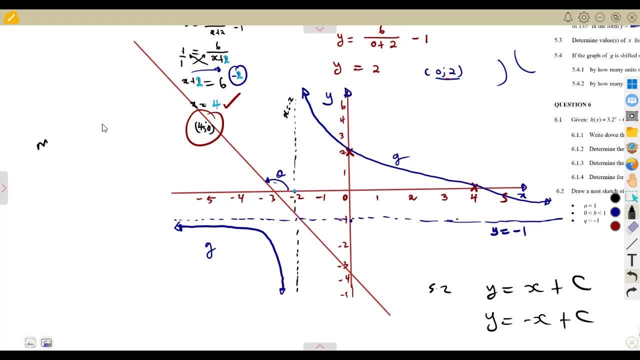 turn 135,. remember gradient is equal to turn. the angle of inclination gives Theta, So you can use that: turn 135 degrees. You are going to see that you're going to get a negative one, but that is not even important here. Yeah, that is the important. 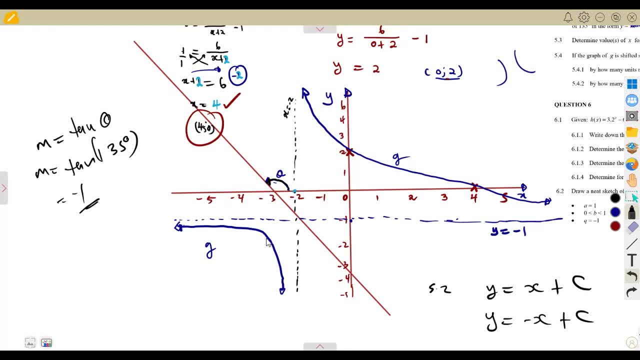 So this was just to tell you that. which one are you using? The one with the positive gradient or with the one with the negative gradient? So this one. it is the way that it is slanted. Remember all lines like this: they have got what? 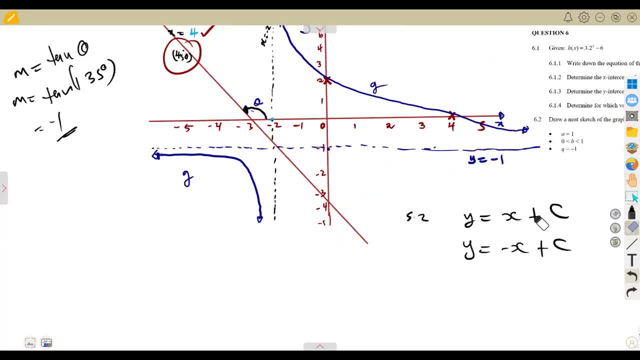 A negative gradient. So meaning to say the one that we're going to use is the one with a negative gradient. Y is equal to minus x, plus c, But I said these two lines. they do pass, whether it is a positive gradient or not. 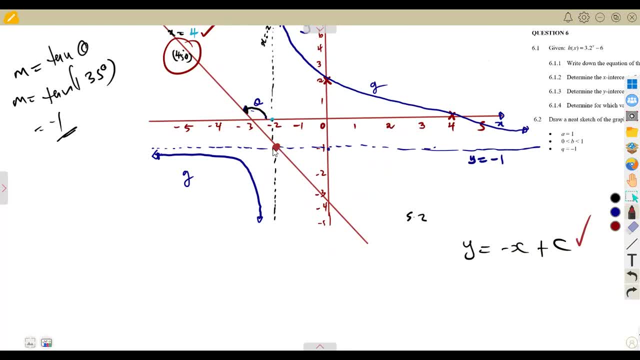 They do pass at the point of intersection of those as simple totes Where x was minus two. remember it as simple totes: X was minus two and y there was minus one. So you use that to determine your equation Why there is minus one when x is given as what. 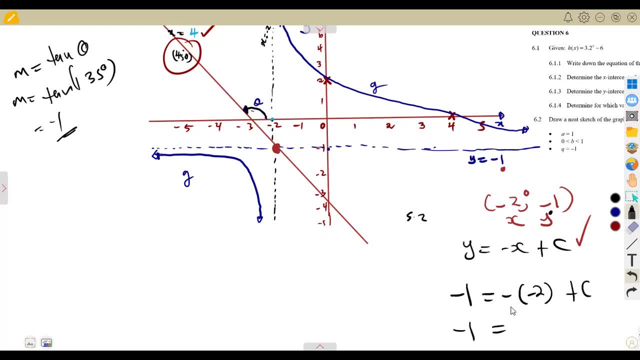 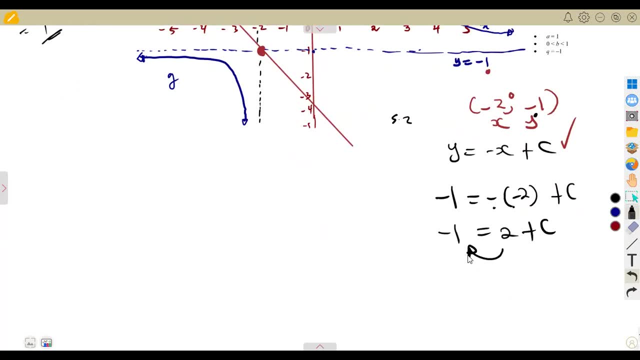 As minus two plus c, So that's minus one is equal to a two plus c. transpose This: that is going to be a positive and negative two minus one. minus two, That is minus three, So c is negative three. So therefore our equation was going to be: y is equal to. 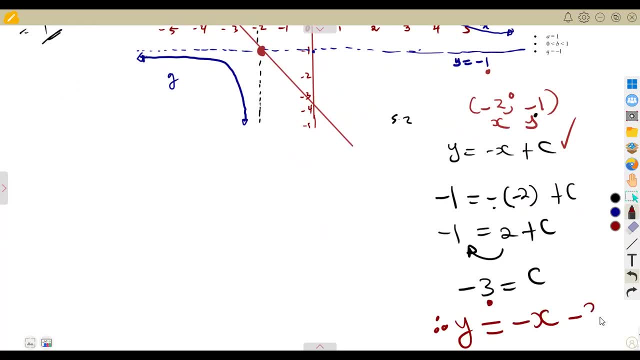 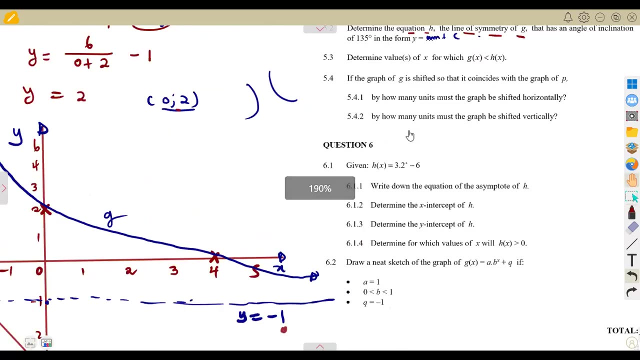 Minus x plus minus three, That will be a minus three, just like that. So this is our hx. Remember? he told us that this is going to be given or it's going to be written as what? as h. So we have got the equation of hx. 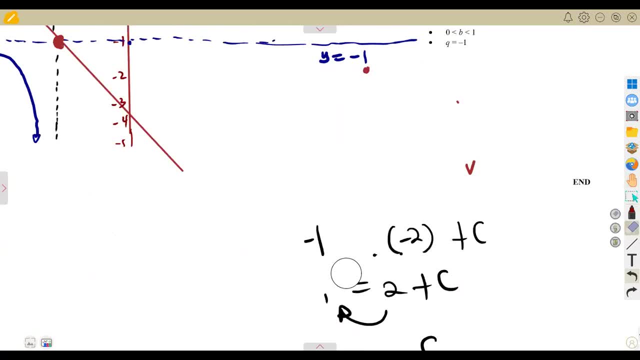 Let's just remove guys. There are not a lot of things. I don't trust these boards. They just tend to misbehave if there are a lot of things on them, So Let's see so that we do not miss anything up to the end. 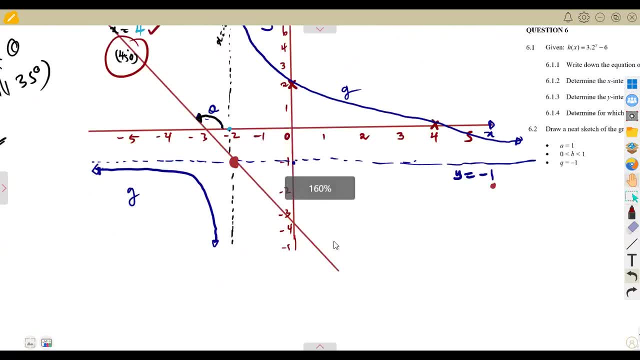 All right, In this case we calculated this. So this is our hx, which is the axis of? what axis of symmetry with a negative gradient? So our hx was negative x minus three, So it means it passes through the y intercepted, negative three. Okay, 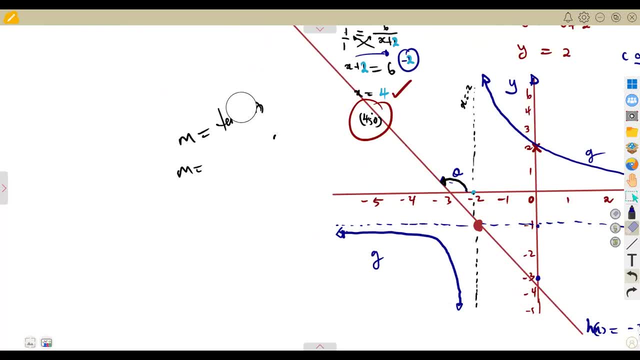 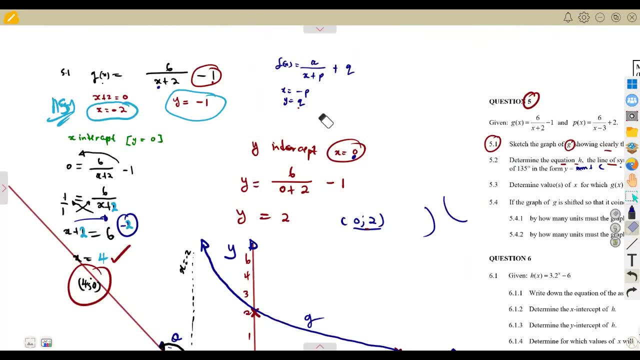 It's another thing to consider, All right. So let us check what we have. What we have, We conclude our quest. and, very sorry for that, I'm just going to remove this one or two things here, just to minimize, All right. 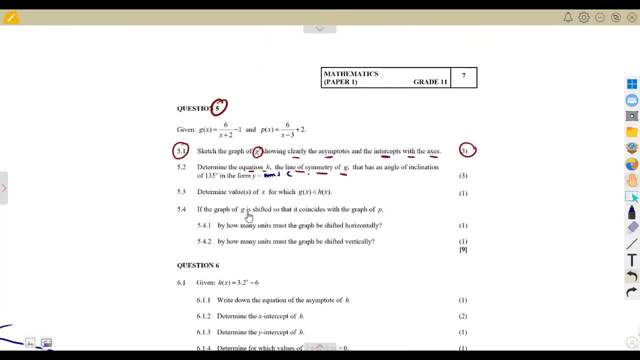 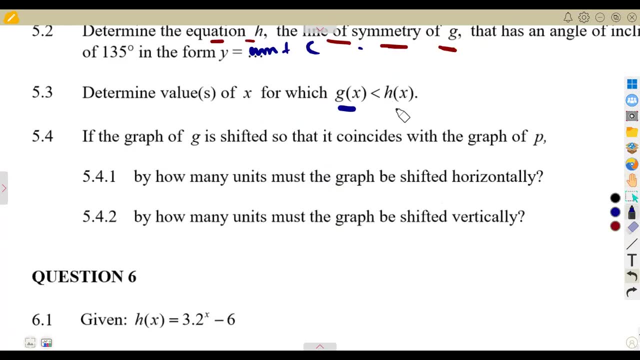 So this is it five. point three determine the values of x for which gx is less than hx. So this one- you can interpret it from the diagram- Where gx is less than x, It's a condition where gx, because it's less than it, is below hx when it is a greater than. 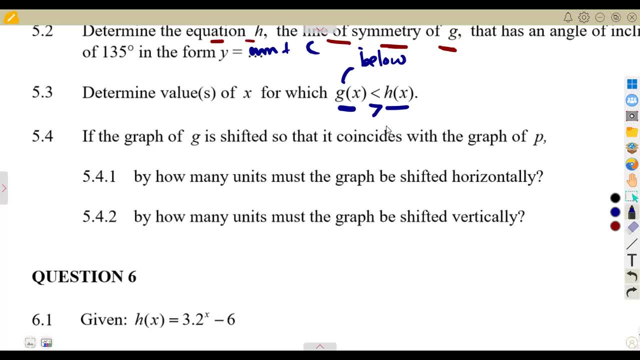 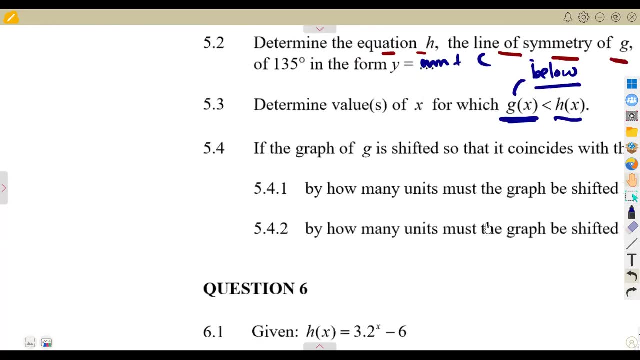 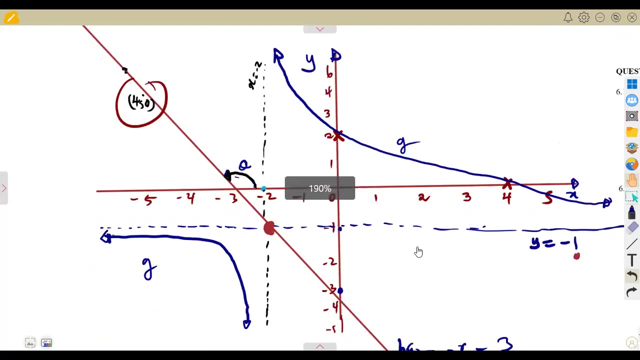 you take when it is above all right, when you take it when it is above hx. but this one, because it is less than we want. every part where gx is found below hx on our graph, where is it? That's five point three: Where is it? so gx is less than what hx. this is it, gx. that's five points. 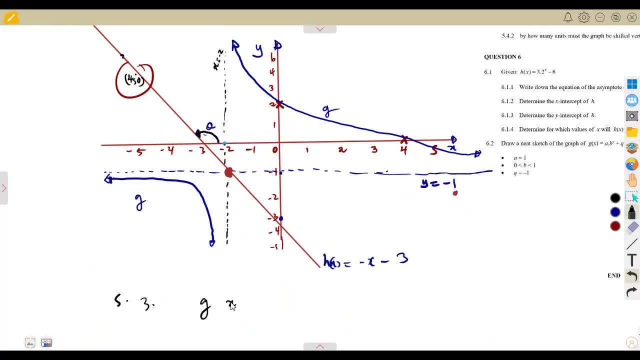 So this will be 5.3. we want a condition where gx is less than what hx. so, like I said, this one is less than this, so it must be below, below hx. so where this is our g, the hyperbola. So if you check along this region, this one, along this region, our g is below this graph. 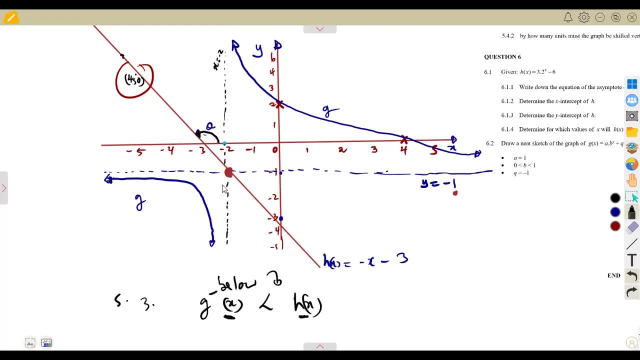 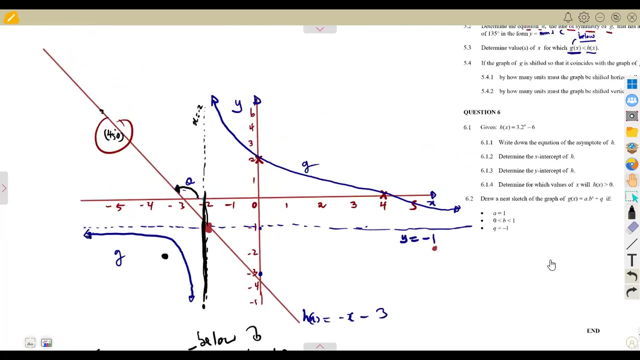 it is below, it is the one that is below Along, these values where x is limited at minus two, where x is less than minus two, minus three, minus four, minus five, all these values where x is what less than minus two. our gx is below, It is below hx, but if you move from that region of minus two, now this side minus two. 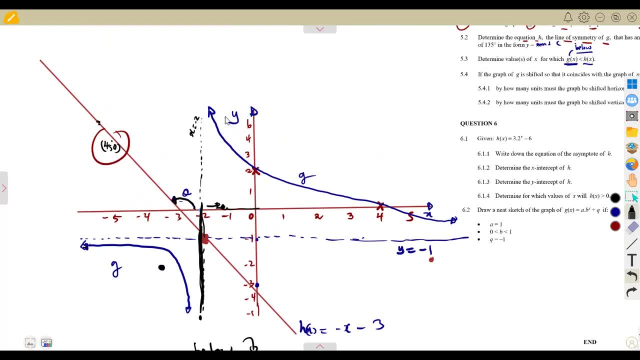 above, minus two, minus one and so on. you will see that your hx is the one that is on top of what on top of hx? our g is on top. so we can't take this region. so that was the only solution. x must be less than minus two. x cannot be equal to minus two at their simple dot. 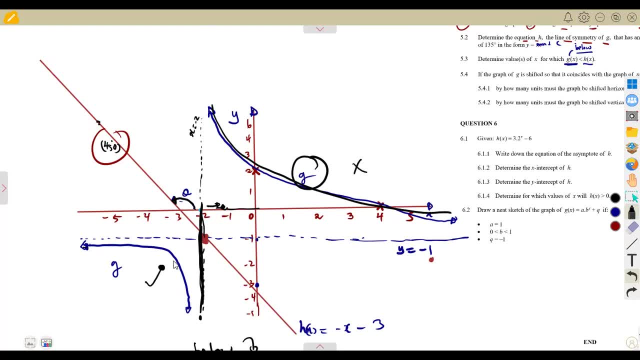 so x is less than minus two. so it was going to be a vice versa. if they said gx is greater than hx, meaning to say our values were going to be what x is greater than two, but in this case our x is less than this. okay, so be careful. be careful how you're going to attempt this. 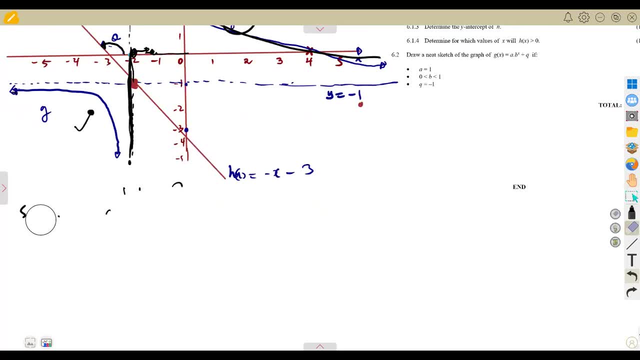 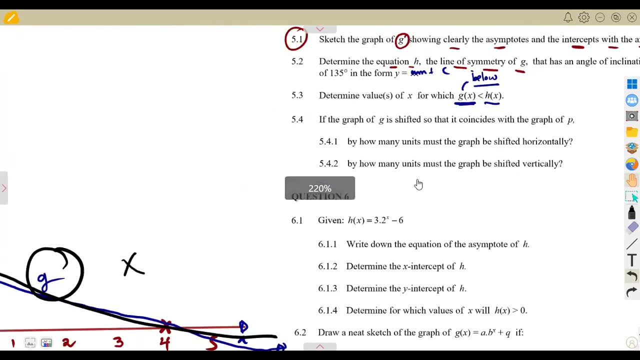 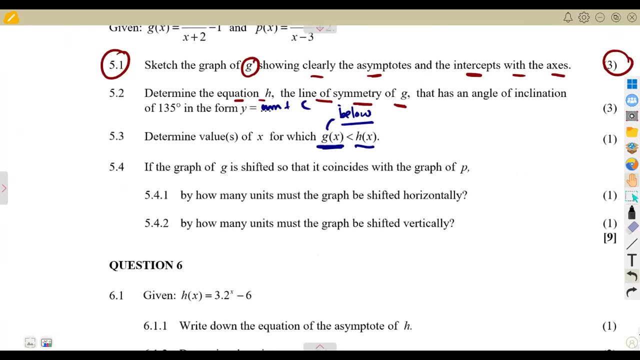 one, and this x is going to be an element of all real numbers that we're going to talk about. so that's it. then, if the graph of gx is shifted so that it coincides with the graph of p, by how many units must this graph shifted horizontally? so this is it, our graph. 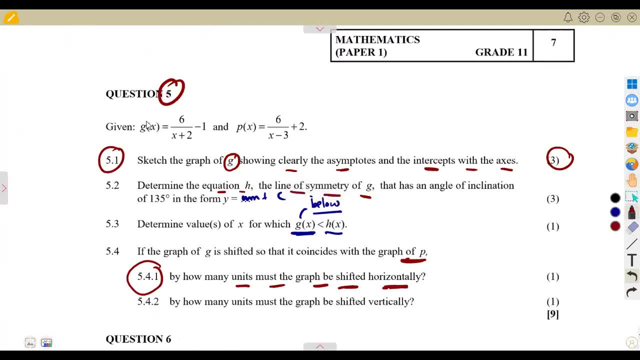 of hx is here. they are saying: we are going to shift until it looks like this one. so how many units are we going to move until it looks like this graph of what? px horizontally? horizontally, these are the x values. so what happens is that when you are dealing with the x values, which is uh, which is horizontal, before at px, we have 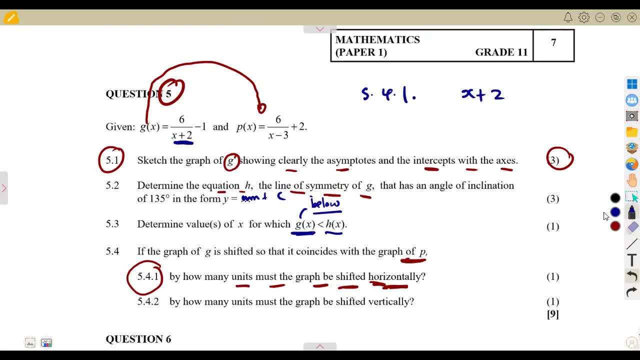 to transform. it was x plus two. so you must ask you yourself: how many units are we going to move so that this will be what? a minus three, so that it will be a minus three? how many units are we going to move so that this will be? 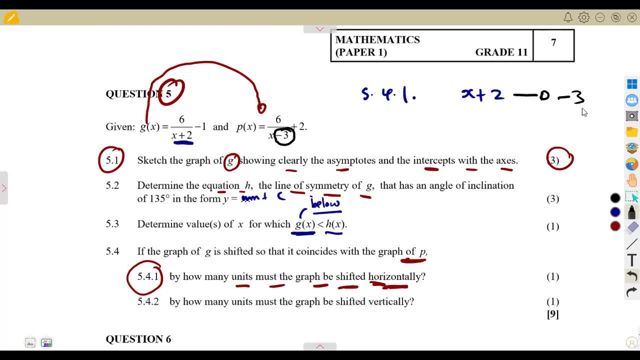 a minus three because it's a minus three. how many units are we going to move so that it will be a minus three? so this is it. if we are to consider this, we are going to move how many units to get a minus three? it means this was a minus five x plus two. we subtract a five like this, so two minus five is. 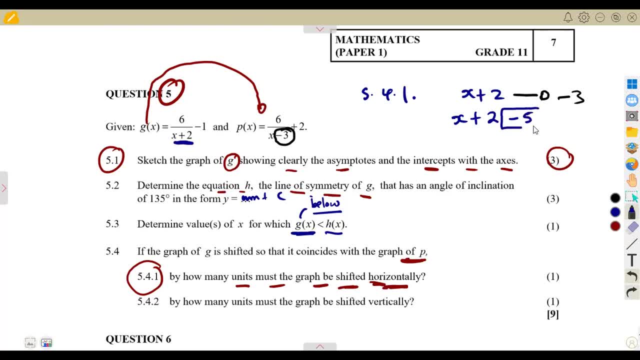 what minus three. so it means we moved how many units if there is a minus five. so take note a horizontal shift. it affects this way, just like how you calculate their simple thoughts. when it is x plus two, you say x is equal to what minus two y, and when it is y, you use it as y is. 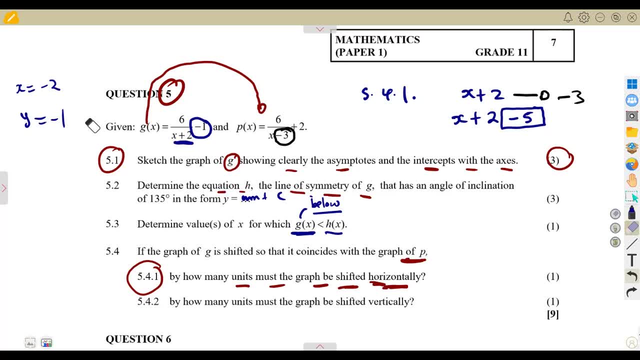 equal to minus one. there is something about x: it opposes the way it is given there. so if you are saying x there, it's a minus five on the presentation. there is a minus five on the presentation. there is a minus five on the presentation. this is not your x. no, this is not your x, the x that we are talking about. 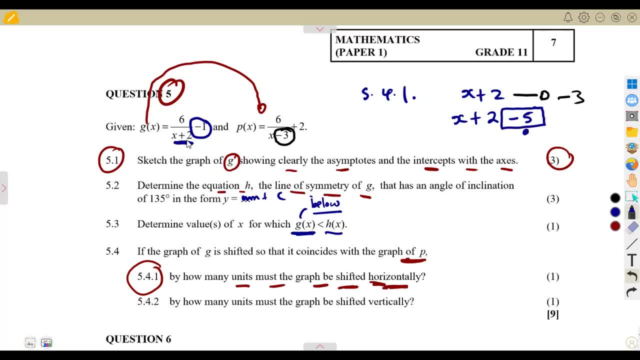 is when you solve, just like when you have x plus two, you find x is equal to two minus two. so it means if x is minus five it's gonna be equal to zero, so x is equal to five, so we move to five units. so meaning whenever you see a negative, you write the opposite way. it means 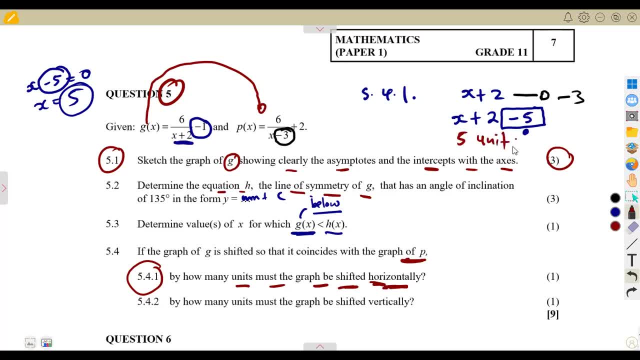 these are five units to the right, to the. to the right because we saw at the end, x is going to be a positive five, so meaning to say is to the right. so when you see an expression like this- x minus five, it's five units to the right- don't consider this negative. but if x is equal to five, it's already telling you where x is going. there you. 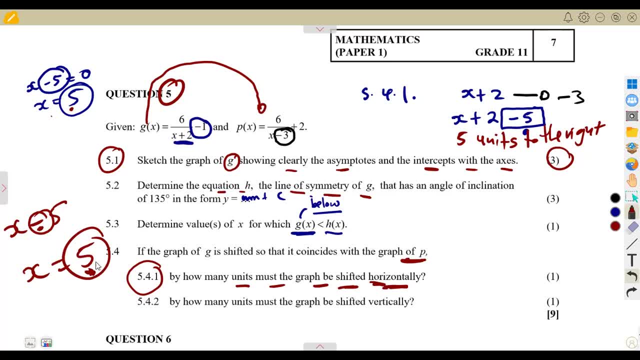 don't change anything. x is five. you're going to the right straight. it's not an expression that one all right. so be careful. what about vertically? vertically, we consider the y values. now it was at minus one, now it's at two. so how many units did we move from minus one until we get to two? 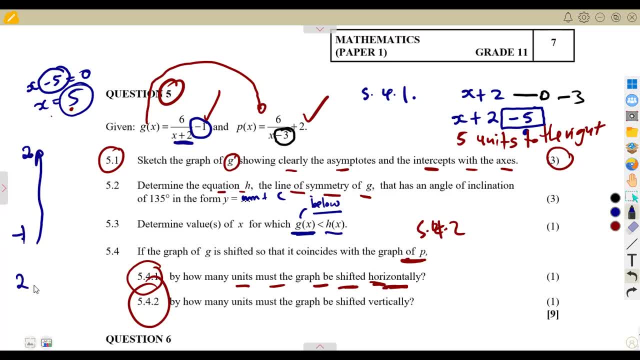 so it's simply two. so it's simply two minus minus one. we moved our menu is three units going up, so these ones are three units up. y is three units up. that is vertically. vertically. you consider how are you moving in the y axis, horizontally in the x, but you have to be careful on the horizontal. as you can see, there are a lot. 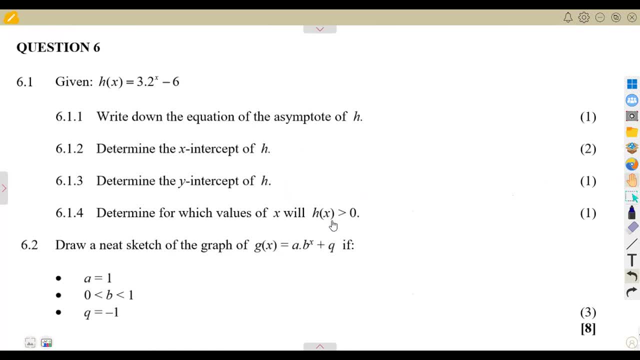 of things there to consider on the horizontal. there are a lot of things there. okay, question six: given hx, is uh two, three into two to the exponent of x minus one. this is our exponential function. so we are given this uh hx. write down the equation of the asymptotes of h. 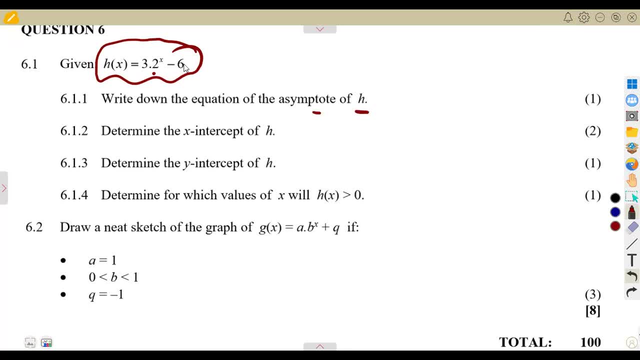 remember, when i give an exponential function, the asymptote is the y value. so our asymptote it's y is equal to minus six. then the x intercept of h, the x intercept it's on a condition where y is equal to zero. so zero is equal to three times two to the exponent of x minus six. 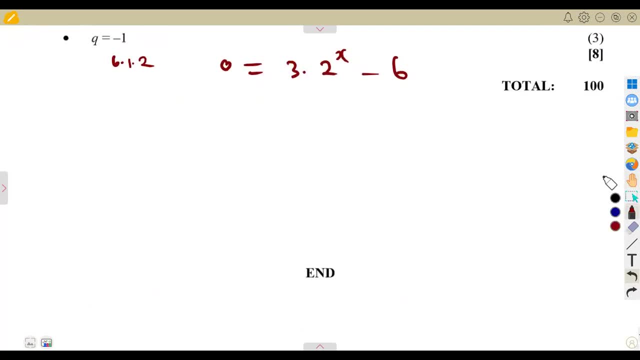 you solve for what? for x, that's your x intercept, y is equal to zero. so if y is equal to zero, you can solve this. transpose minus six, it becomes a positive six. three times two to the x exponent of x you can divide by three, since this is a multiplication. so it follows that two to the 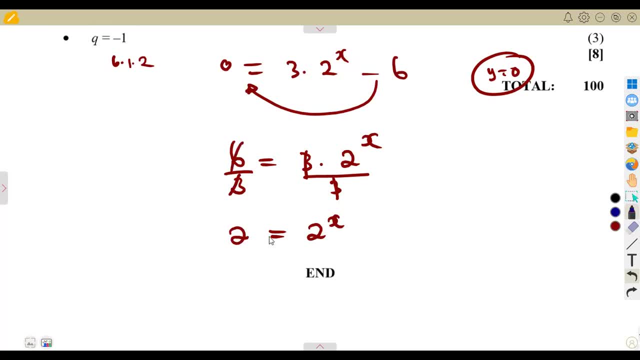 exponent of x is equal to what to two? since this is invisible, the exponent, it means there is a one, and we know that if the bases are the same, like this, we equate the exponents. as long the bases are the same, the exponents are the same. so it follows that x is equal to what x must be equal. 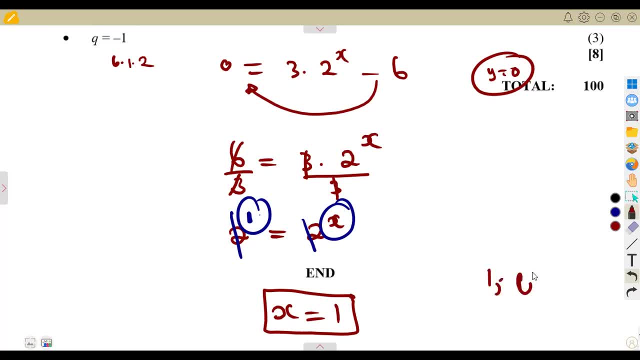 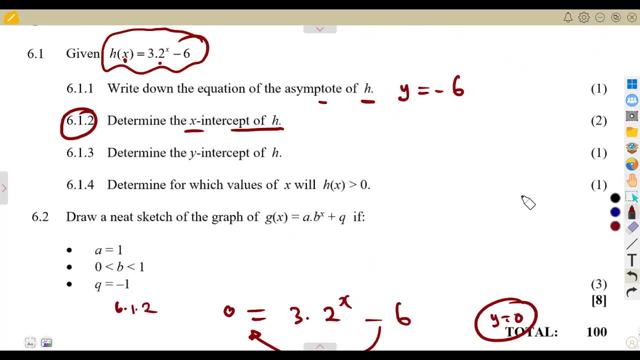 to one. so that's the explanation for the exponential function of h and the exponential function of h, that's our x intercept. that's one versus what? one versus? remember, y is zero there. okay, from there, they are saying: uh, determine y intercept. okay, so the y intercept, it's on a. 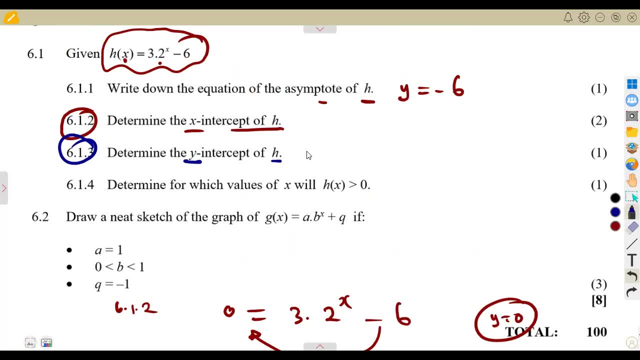 condition where x is equal to zero, so that one you can just substitute into your equation straight: y is equal to x, it's a zero there. so it's three times two to the exponent of zero minus what six? so simplify this on your calculator. uh, that was. 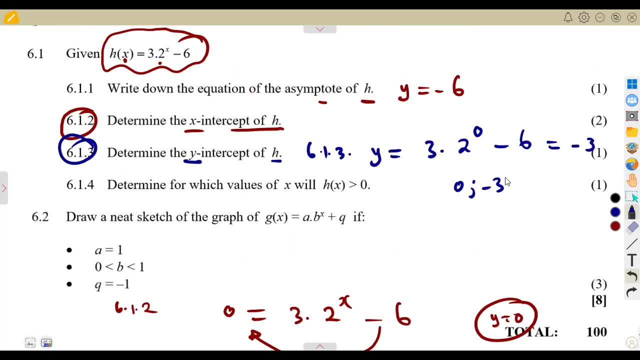 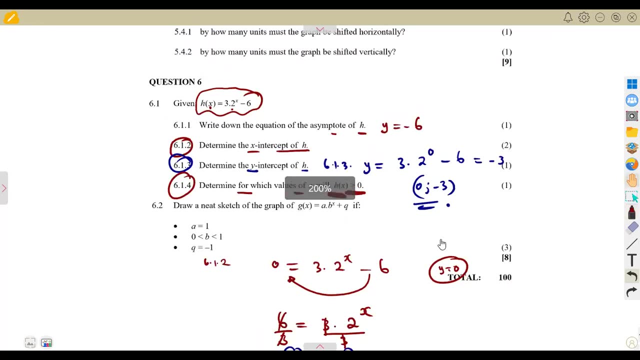 going to be minus three. so that's zero versus minus three. that's your y intercept. determine for which values of x is hx greater than zero. so this one is an inequality. so already on the inequality, we do not know, or we haven't drawn this function, whether you're going to draw. 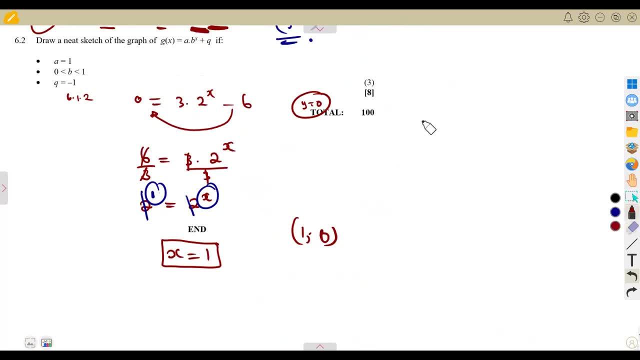 your function. it's up to you, but we need a condition where this function- uh, which is our f, of x, uh, which is our hx, i mean uh, the one that we are given there, where it is greater than zero. where is it greater than zero? it means three times two to x, minus is supposed to be greater. 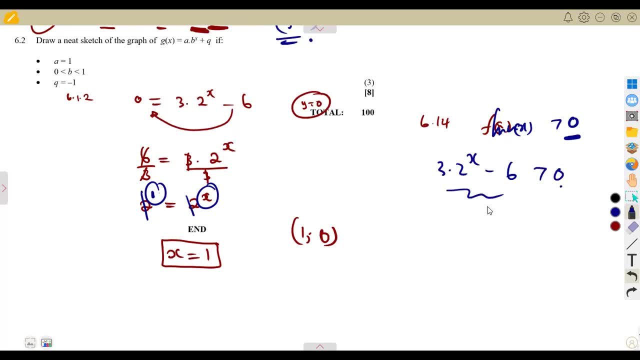 than zero. as we know, each and every inequality, you solve for the critical values and the critical values are the solutions when our f of x, or whatever function that you are given, at that moment, when it is equal to zero and when hx is greater than zero, it means that the function 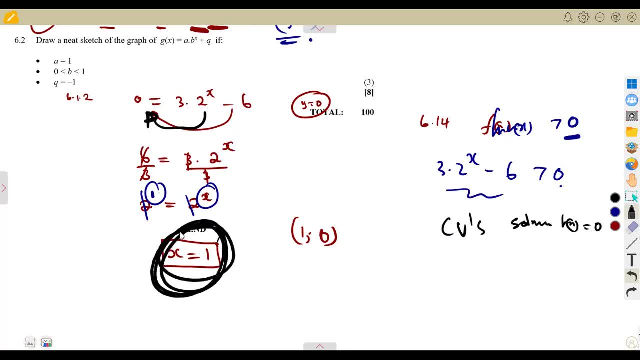 x was equal to zero. we solved this before, so you're not going to solve again. you solved and you got that x is equal to one. so at x is equal to one. that's a critical value. that's a critical value meaning to say: at x is equal. if you substitute a one here, you get a zero. 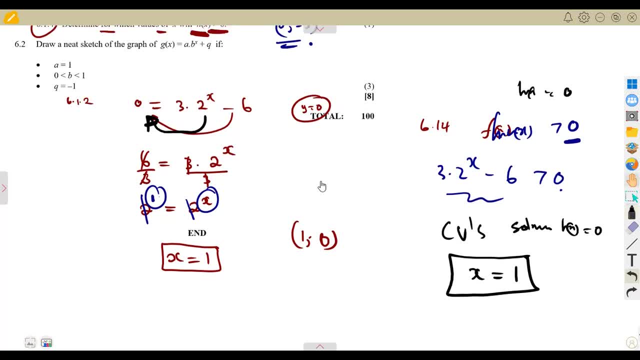 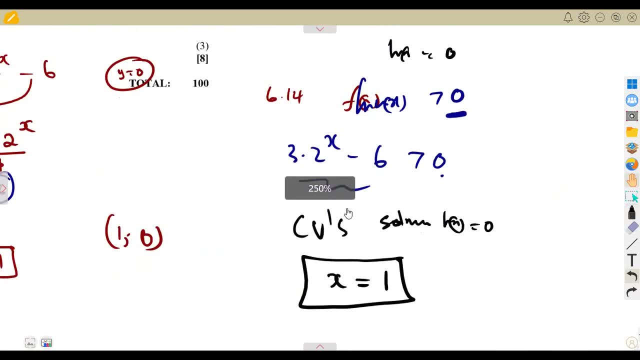 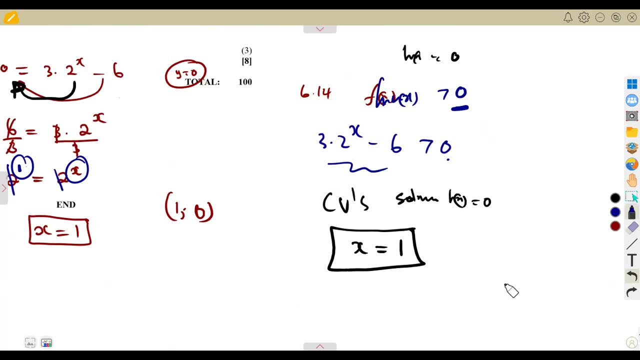 your f, your hx is equal to zero. when x is one, it's a critical, but we want a condition where hx is greater than so. since you have a critical value, you can use that to balance now your solutions, to check how are they going to be related. there is only one solution. there is only one critical value. 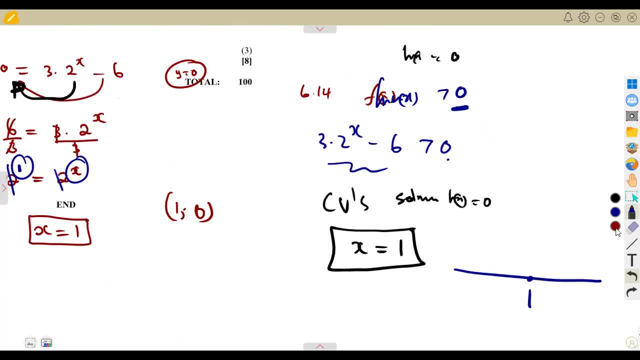 so meaning to say there are just two answers that we expect, which answers values that are less than one and the values that are greater than one. because x cannot be one, because where x is equal to one, that's a critical value. we cannot take that one. so we need a solution where it is less than one, where it is greater than one, so it is like it's. 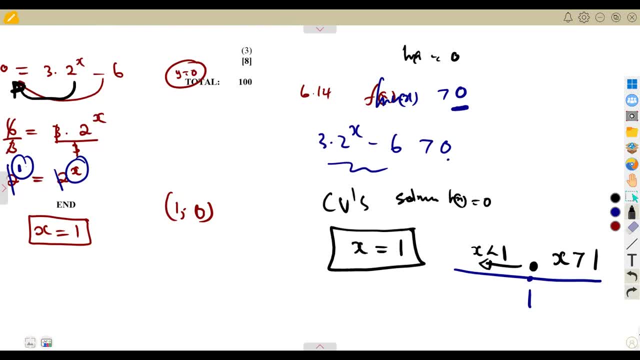 it's in your hands. when it is like that, a question like this, it's in your hands, you can use it. you can just use your, your simplification. substitute any value that is less than one, think or think of any value less than one. let's say, uh, we put a zero there, any, any. 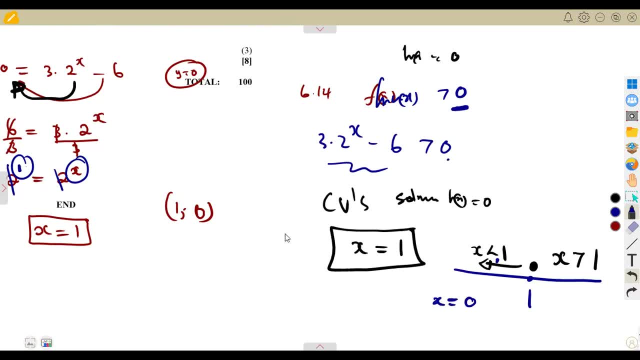 any less than one. put a zero, any value less than one. so if you were to substitute a zero there, you are going to get a negative value, a negative value. is it greater than zero? okay, this is what i'm trying to serve, this to say: substitute any value of your choice that is less than one. so, like i said, i'm gonna. 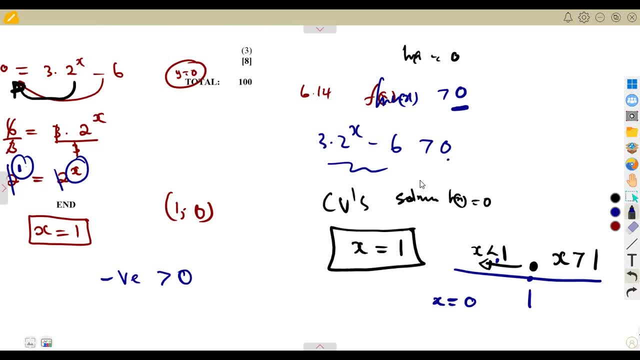 substitute a zero there. zero is not a critical value. a critical value is one, not zero, from our solutions. zero is not a critical value. so, guys, just because of these softwares- now it's difficult for me to even show you what i want you to see because of this time- you see these softwares, guys, they 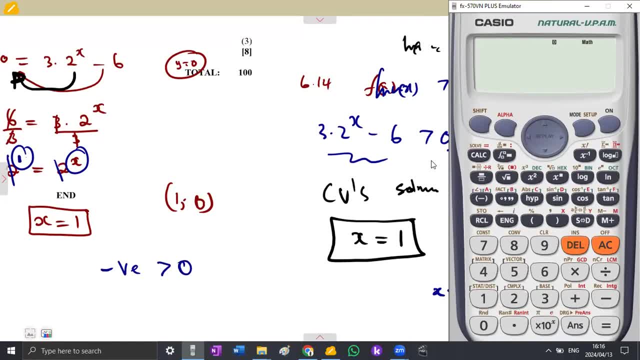 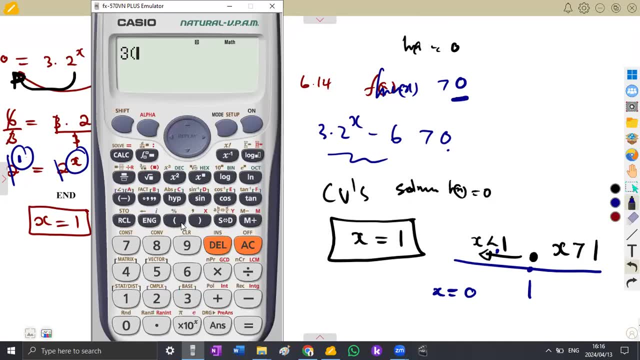 they want you to work for a certain time. okay, but this is what i'm trying to say. i'm gonna substitute here: this is three into our. okay, let's just do it like this: three times two to the exponent of x. just gonna choose any value of our choice there. so we said: if x is a zero there, 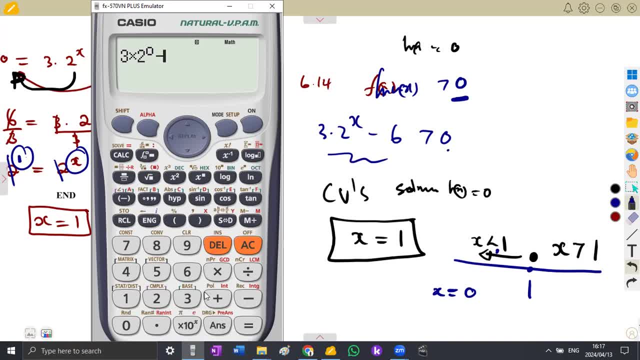 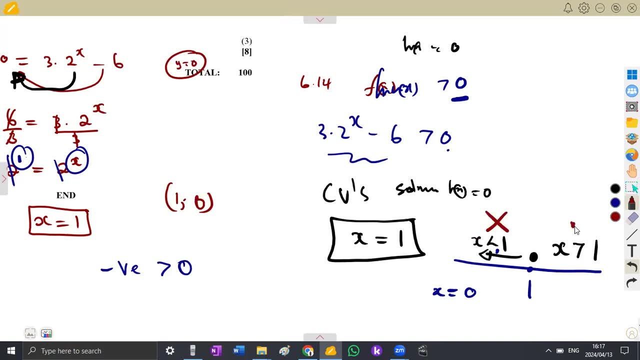 okay, minus six. so we we check, it's a negative three. so is negative three greater than zero? no, it's not. so this is not a solution. we move on to this one. when x is greater than one, any value greater than one you can choose. when x is two, it's greater than one. let's substitute and see where there was x. yeah, this. 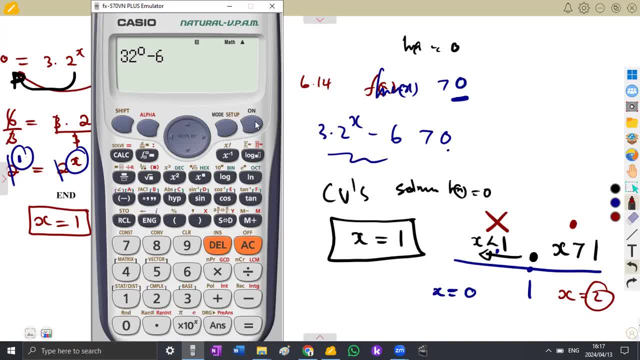 is where our x is. okay, sorry for that. no problem, let me just rewrite it again. uh, remember that's three times two to the exponent of. we are saying our x must be what a two, two minus six. so for any value that you're going to take there, you are going to get positive values. 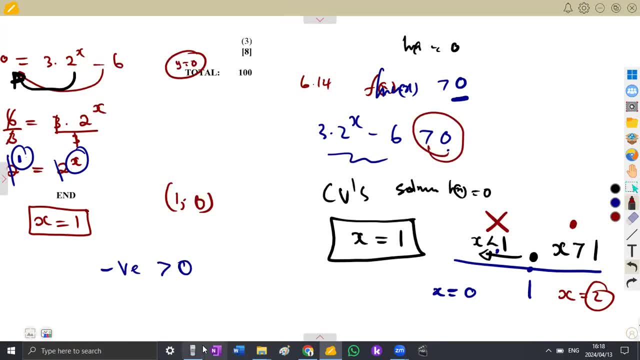 six is greater than what, six is greater than zero. so meaning to say: this solution is true. so, therefore, our x must be greater than, must be greater than zero, must be greater than one. i mean where x is what a, where x is greater than one, our f of x, i mean our hx, is going to be: 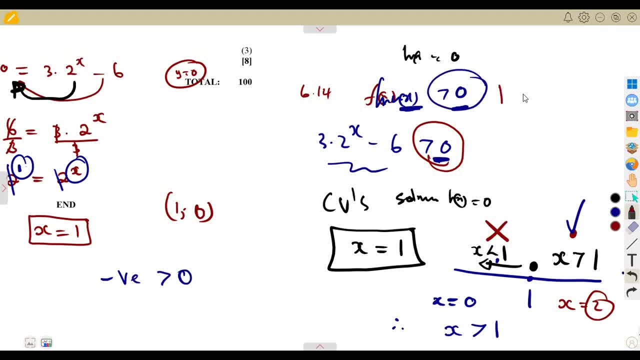 greater than zero. meaning to say, our hx is going to give us a positive answer for all values of x. think of any value of x greater than one. think of any. put it here and see are you going to get a positive or not. also, think of any value that is greater than one and put it here and see are you. 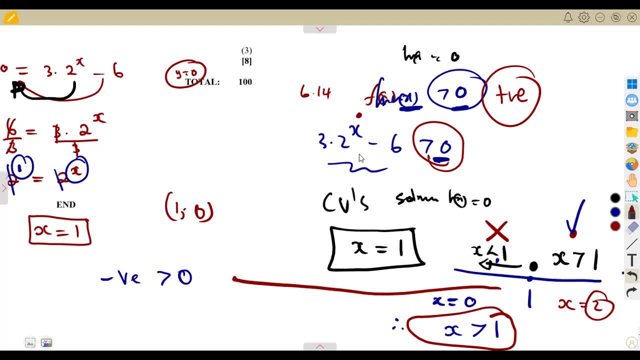 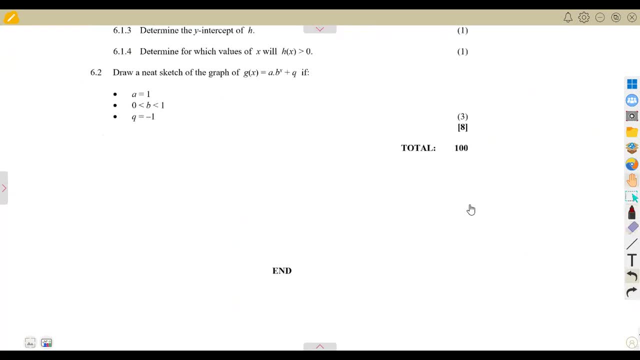 less than what? less than one? substitute it here and see: are you going to get a value greater than a zero? if not, then it means it's wrong. there's no solution there? all right, there's no solution, then we are given on 6.2. draw a neat sketch of the graph of uh. again, it's a exponential function, this one, but we are given. 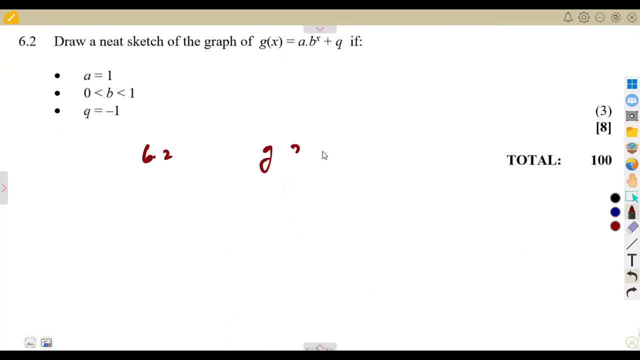 this as g x this time. so they are saying gx is given as a times b to the exponent of x plus q, where a is equal to one. so this is: gx is equal to a, is one times b is a number that is greater than zero but less than one. so meaning to say b is any decimal that you can think of. between it can be. 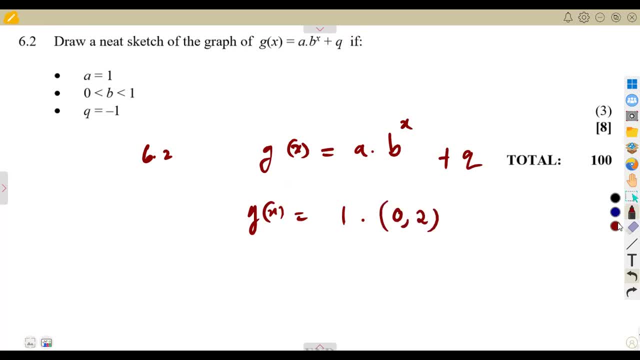 zero, comma two, whatever value that you want. so this one, it's your choice, just any value of your choice, just to consider how the function. but we know this is our b, we just want to see what's going to happen and x is we do not know. remember x, we do not know this one. and 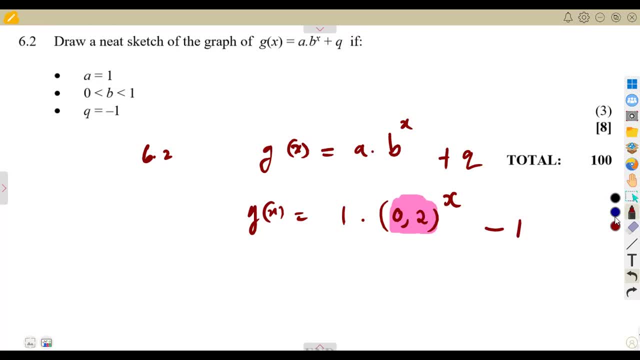 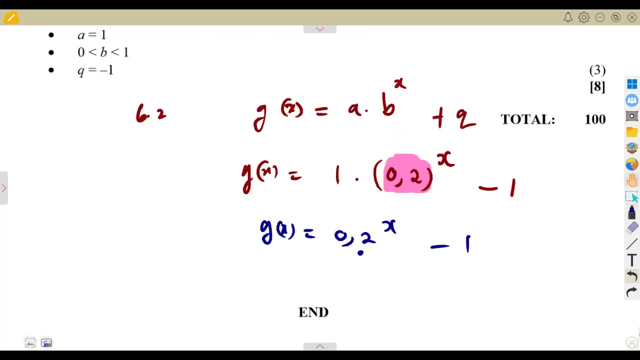 q is minus one. so this is our function. we, how do we sketch the function of this nature? maybe zero comma two to the exponent. as we can see, guys, this is an exponential function, but because it's a decimal it means it is going to. okay. the first thing, the asymptote is what minus one? this graph cannot pass through minus one. so 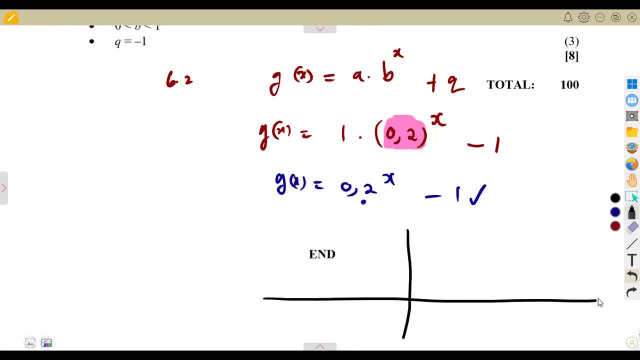 remember what we had before on the asymptotes. so this is our x, this is our y, so the asymptote is going to be at minus one. that's one thing that we are sure about. y is equal to minus one. so you're going to find your x intercept and so forth. uh, if you were to check if x is equal to zero. 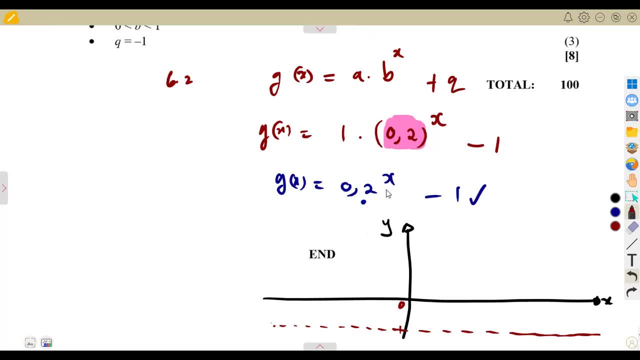 there we are going to have. what if x is a zero? they're going to have one minus one, which is a zero. meaning to say, when x is a zero, this function was going to pass through the origin. when x is, it's no longer passing through a one, just like what we are used when x is a zero, whether think of any. 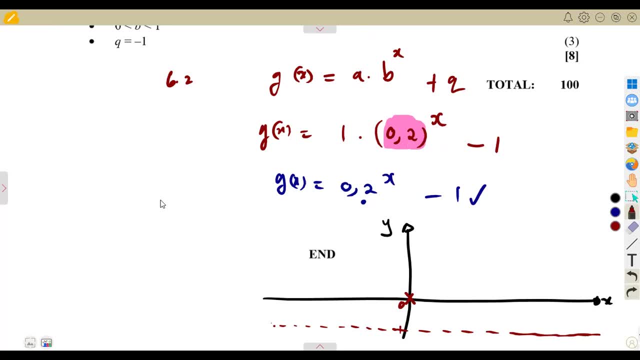 value you put here, any number to the power of zero is what one and one minus one is a zero. so meaning to say, where x is equal to one minus one is a zero. so we are going to have one minus one equal to zero. it was going to be a zero, so that is the most important part and this being a positive